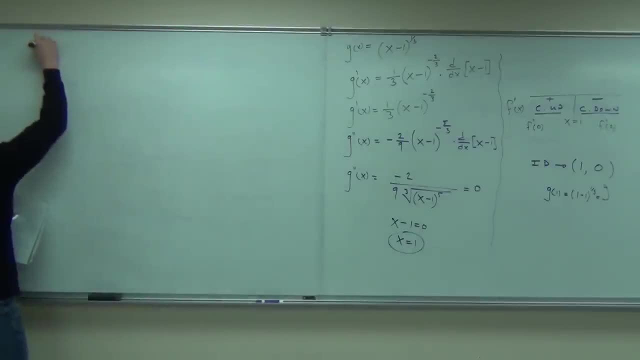 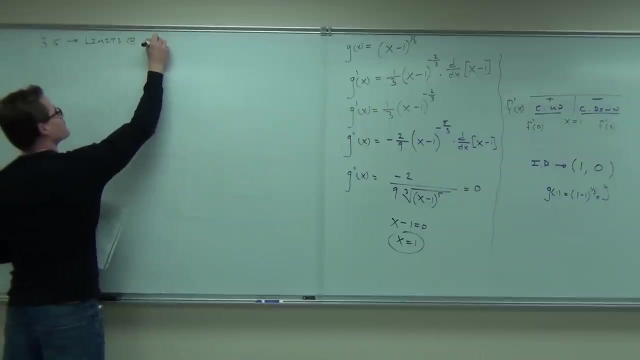 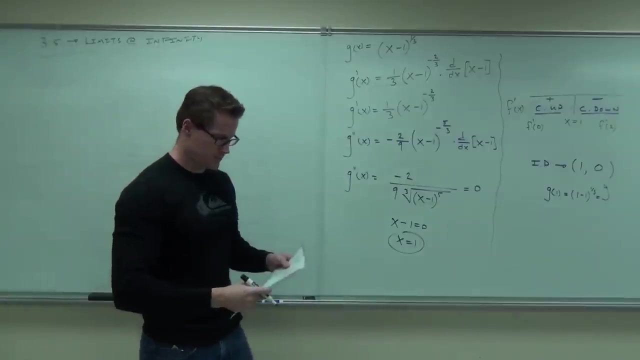 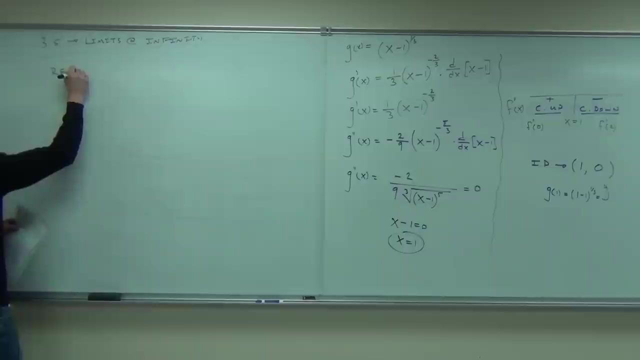 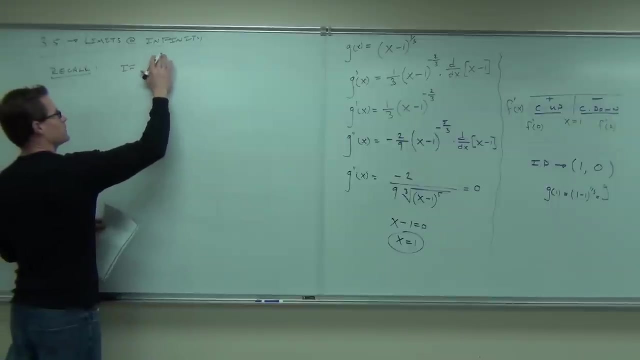 3.5,. we're going to talk about limits at infinity. I'll start off with just a little bit of a recall here. Do you remember If the limit as x approaches a number of f of x equals plus or minus infinity? 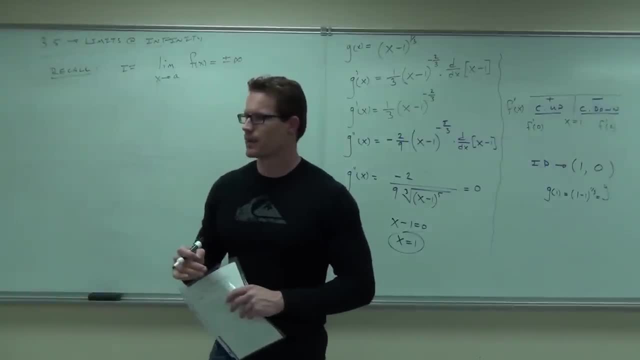 do you remember that? that gave us an asymptote. So basically, when you could not cross out the problem on your limit, you had an asymptote When you could cross it out. it's called a removable discontinuity, it's called a hole. 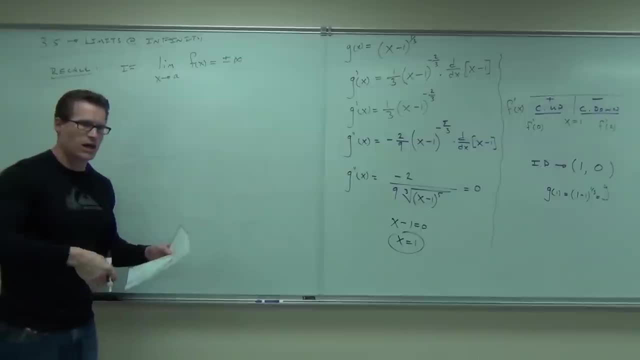 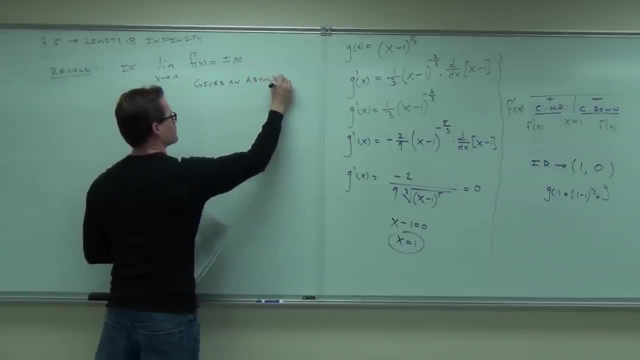 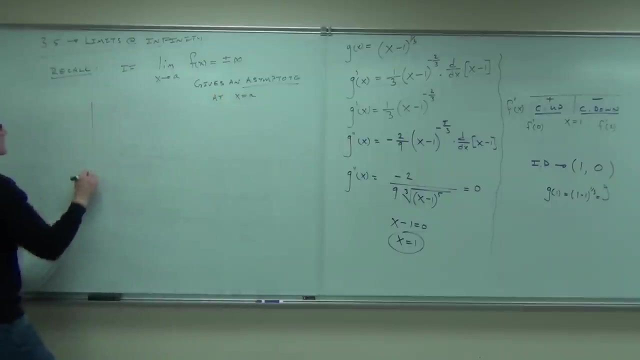 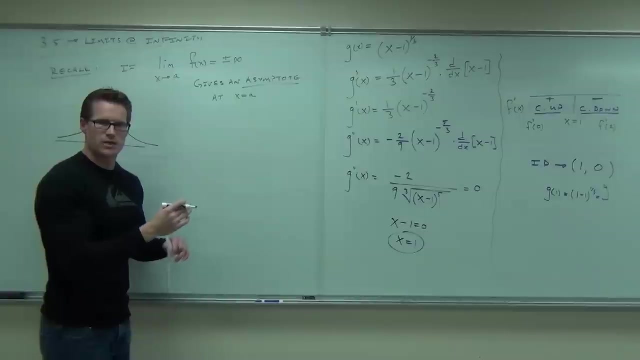 This right here will give you an asymptote at the limit, So we'll value it. And we had two cases really. We had this case Where we went to the same infinity- positive infinity on both sides- and said the limit existed. 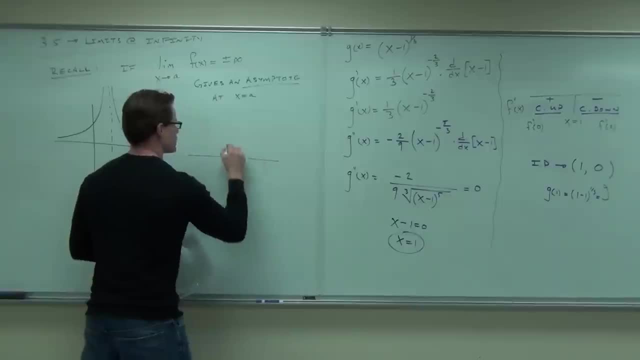 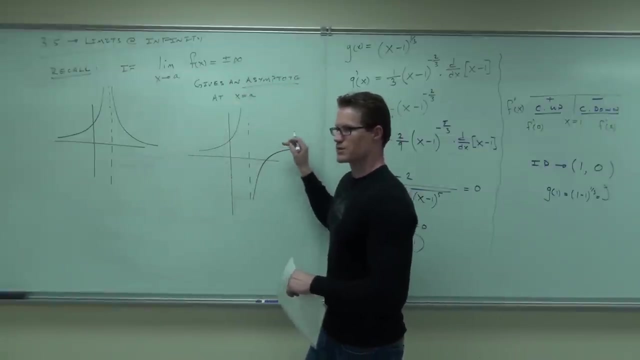 The limit was positive infinity there. Or we had this case Where one went up, another went down. We said the limit didn't exist there. One's going to positive infinity as we go from the left, One's going to negative infinity as we go from the right. 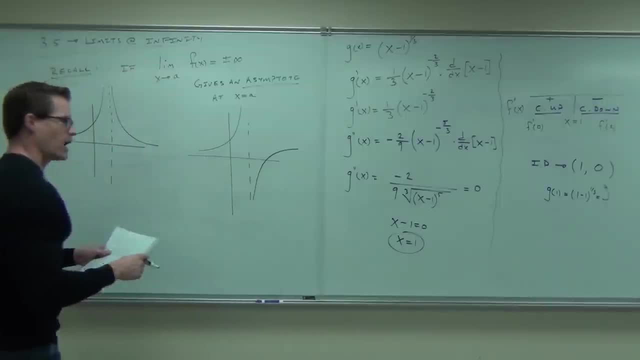 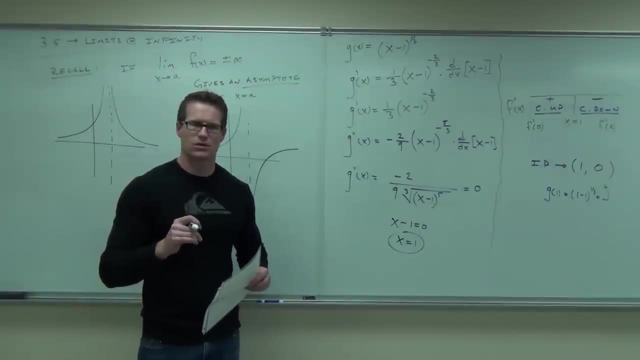 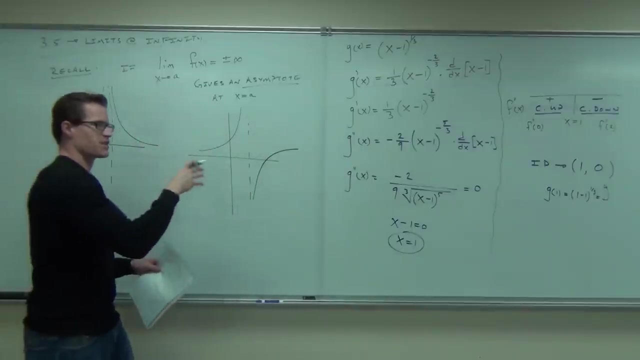 And we had a way to actually determine this. if you remember, How did we determine where we had holes or asymptotes? Sine tests would do this, But how do we find out where all this stuff happens? Let's pretend we had a rational function. 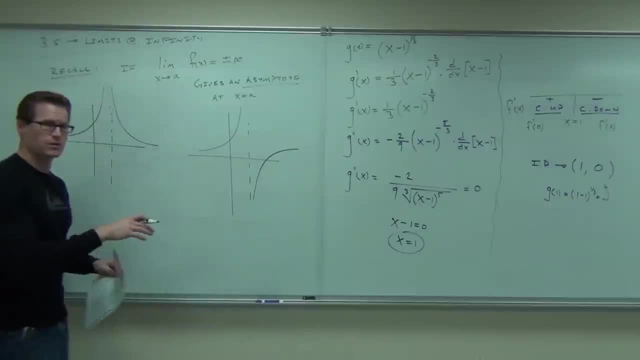 Rational functions have denominators. How do you find these things? You can cross out the denominator and it's a hole, And if you can't, it's an asymptote. Okay, The cross cancel. Let me give you an example. 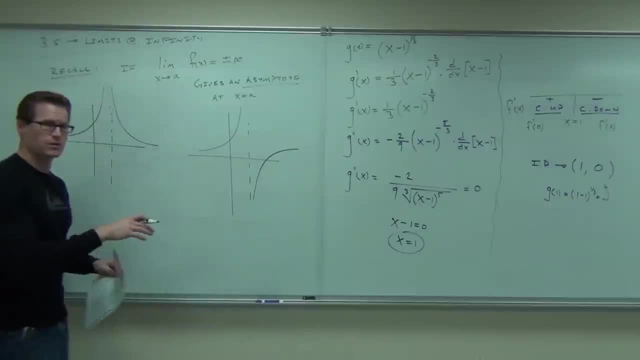 Rational functions have denominators. How do you find these things? You can cross out the denominator and it's a hole, And if you can't, it's an asymptote. Okay, The cost cancels. Let me give you an example. 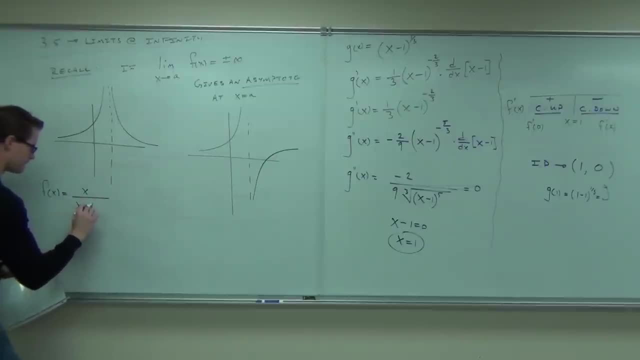 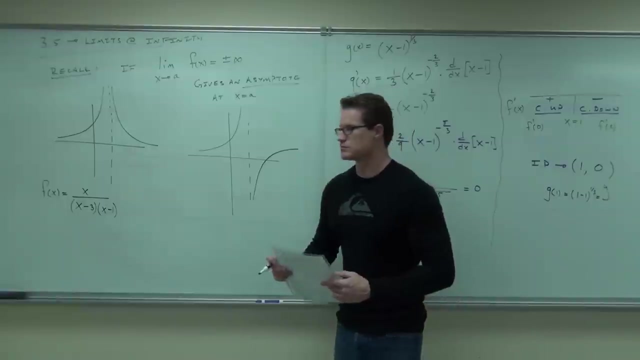 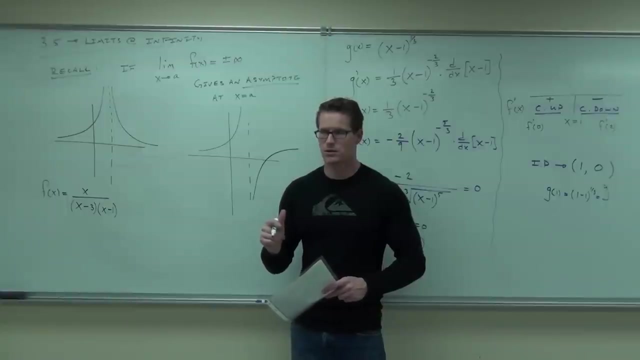 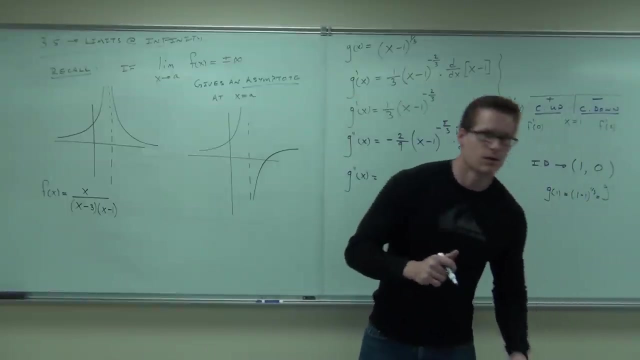 Will this have some discontinuities to it? Yes, Absolutely. Where At zero? one three, Which ones? One one zero Is zero going to be a discontinuity? What do you think? Zero, No, Zero's fine. 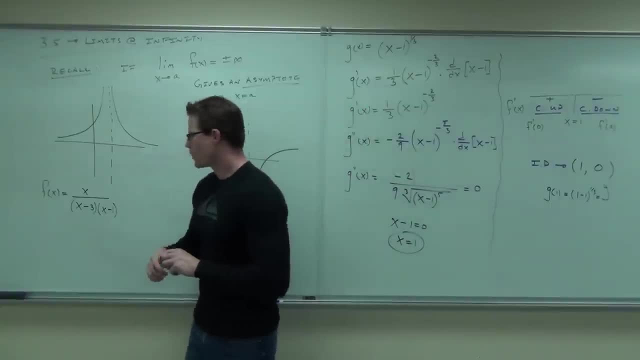 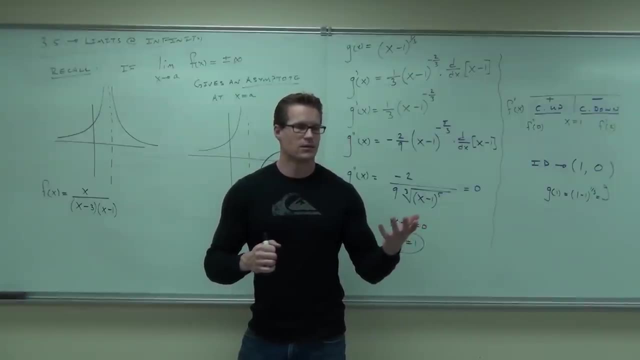 Zero over a number. Zero over a number's okay, That's okay. Where are discontinuities going to exist? Three and negative one. Three and negative one Why? Because it equals zero. Good, Because if a denominator equals zero, you have a problem, right? 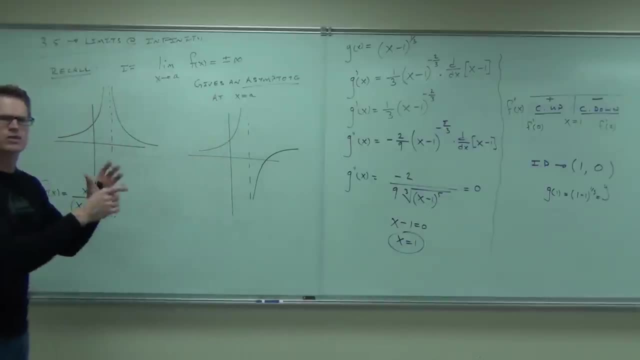 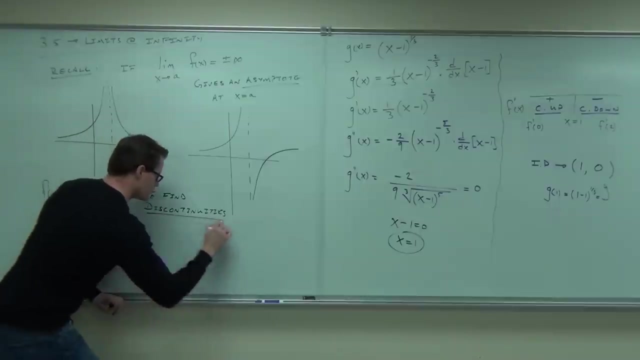 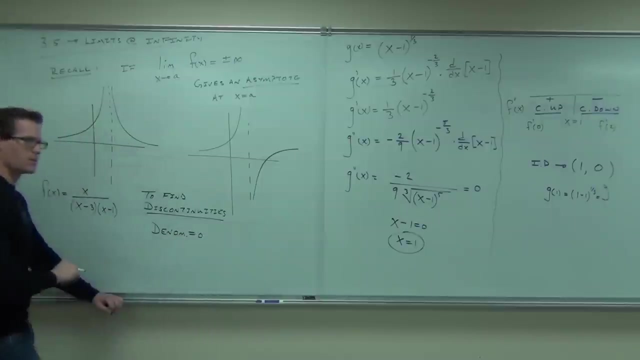 That's how you find discontinuities. That's why I told you a domain from a long time ago. So what do we do to find discontinuities? Denominator equals zero. That's how we do it. We set denominator equals zero. 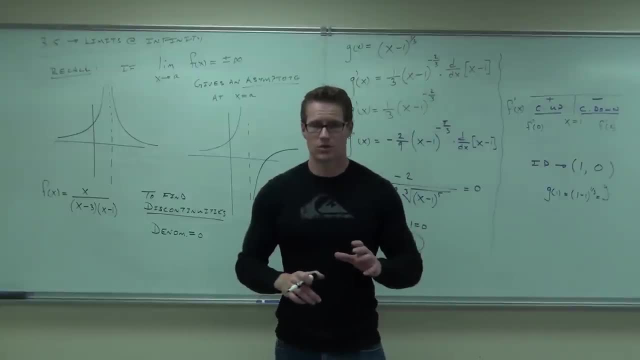 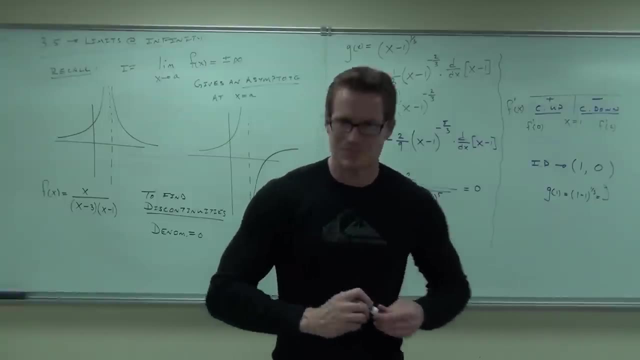 We solve it down, We're going to get either wholes or asymptotes. Do you remember when we get wholes and when we get asymptotes? Okay, Maybe we'll refresh your memory on that next time. So, if you'll recall when we take a limit of a function, 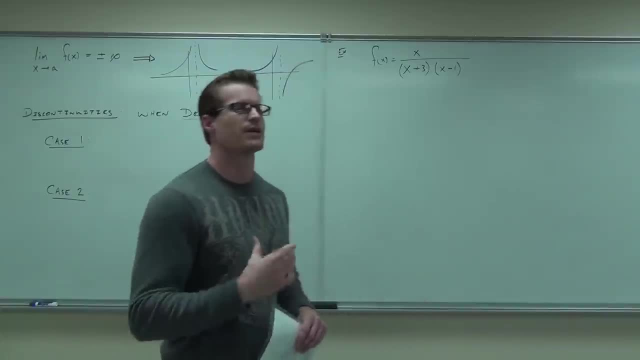 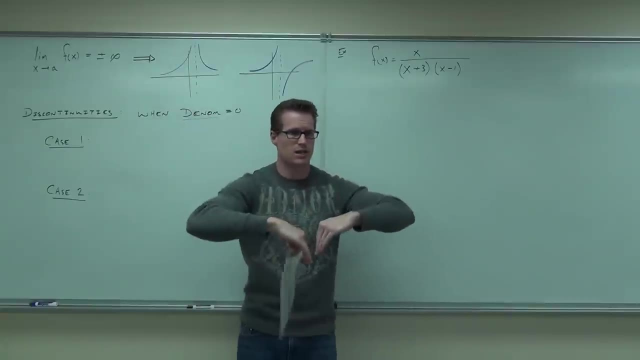 as we approach some number and it goes to infinity, we're going to have an asymptote. We're going to have either an asymptote where the limit exists, as they both go to positive infinity. I didn't draw the case where they both go to negative infinity. 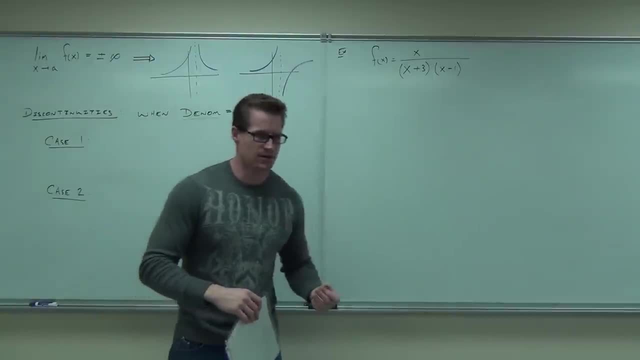 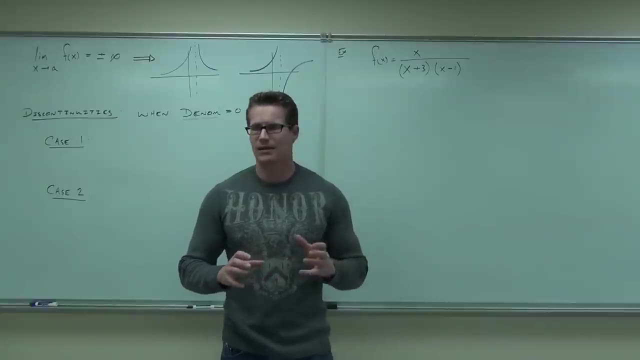 or where one goes to positive and one goes to negative. and then we'd find that with the sine analysis test, Now there were two cases where discontinuities existed. We had wholes and we had asymptotes. Do you remember those, the wholes and the asymptotes? 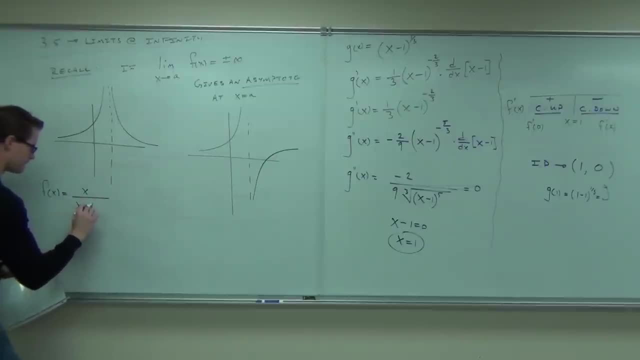 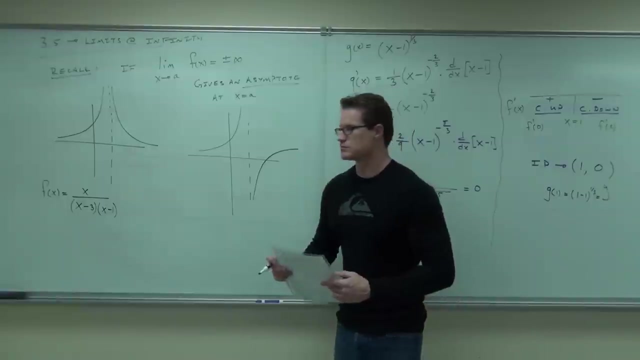 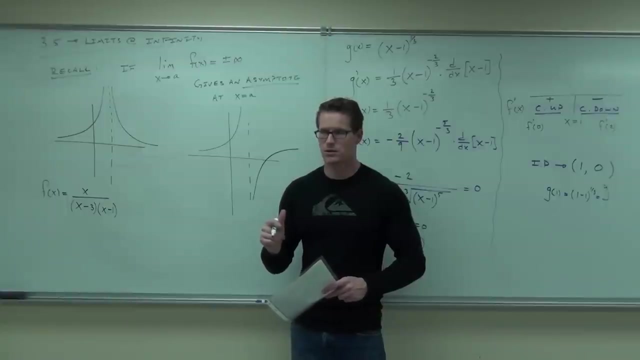 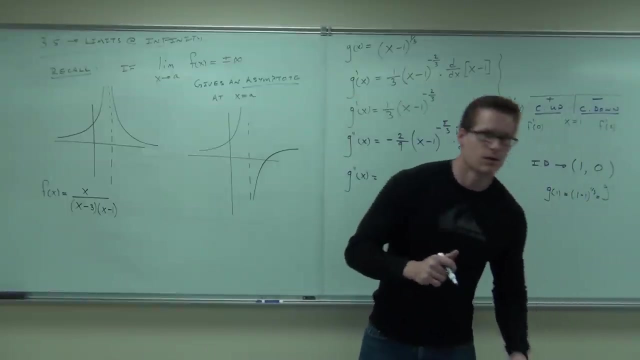 Will this have some discontinuities to it? Yes, Absolutely. Where At zero? one three, Which ones? One One Zero Is zero going to be a discontinuity? What do you think? Zero, No, Zero's fine. 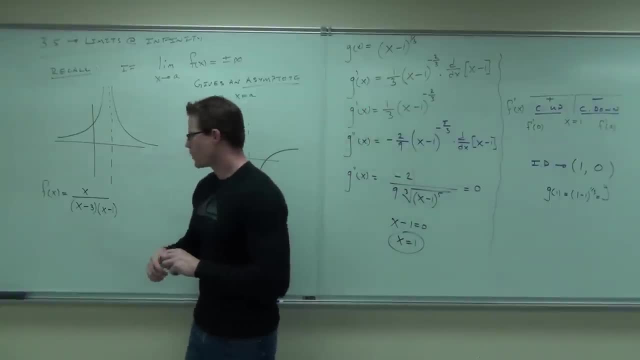 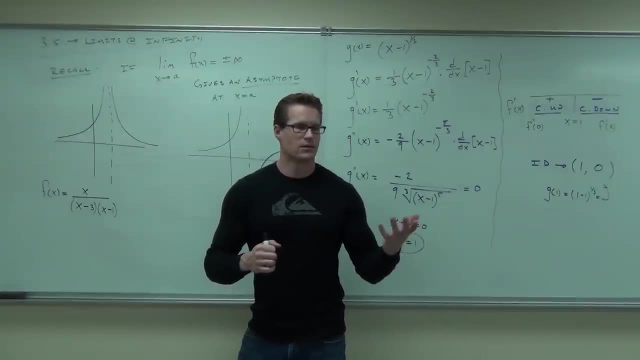 Zero over a number. Zero over a number is okay, That's okay. Where are discontinuities going to exist? Three and negative one. Three and negative one Why? Because it equals to zero. Good, Because if a denominator equals zero, you have a problem, right? 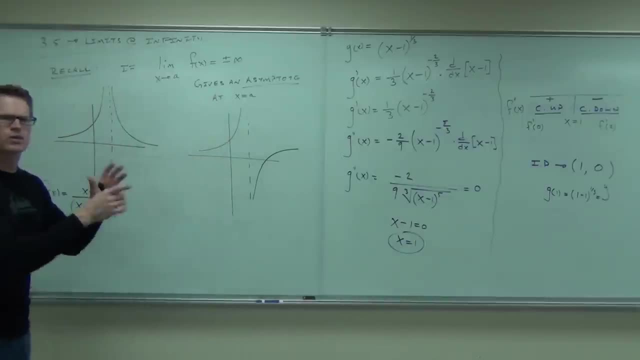 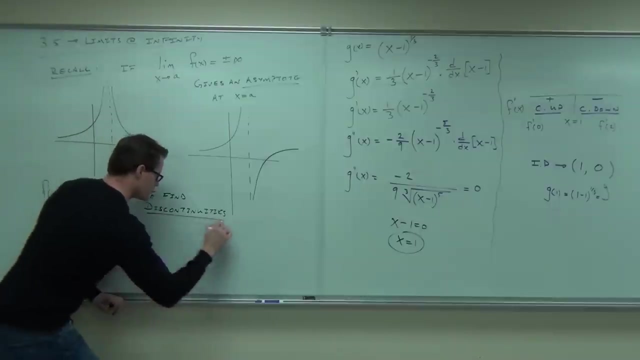 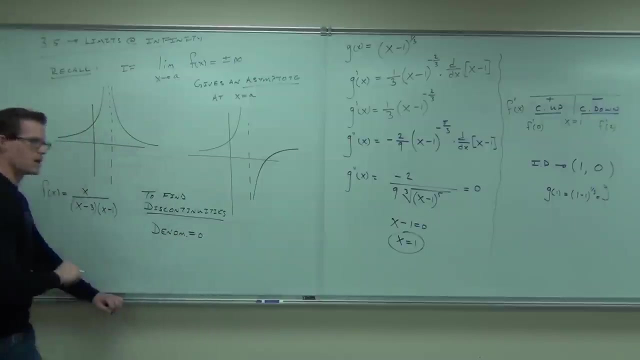 That's how you find discontinuities. That's why I told you a domain from a long time ago. So what do we do to find discontinuities? Denominator equals zero. That's how we do it. We set denominator equals zero. 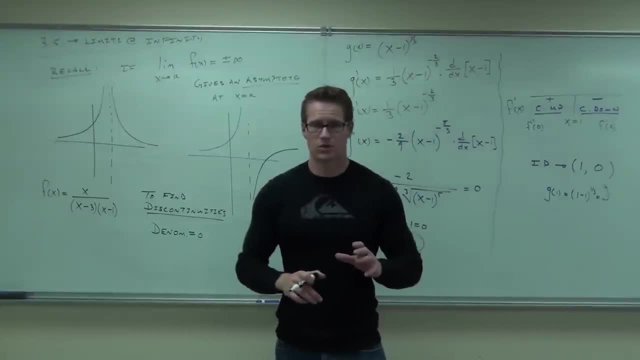 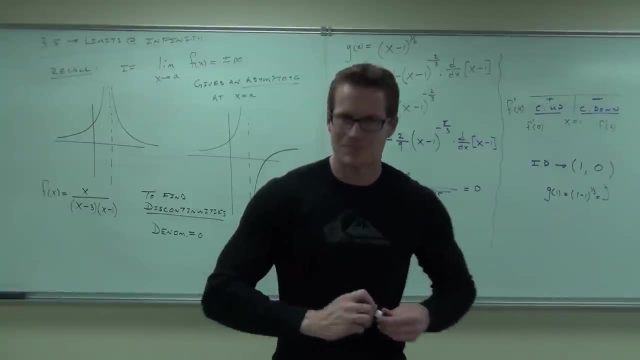 We solve it down, We're going to get either wholes or asymptotes. Do you remember when we get wholes and when we get asymptotes? Okay, Maybe we'll refresh your memory on that next time. So, if you'll recall when we take a limit of a function, 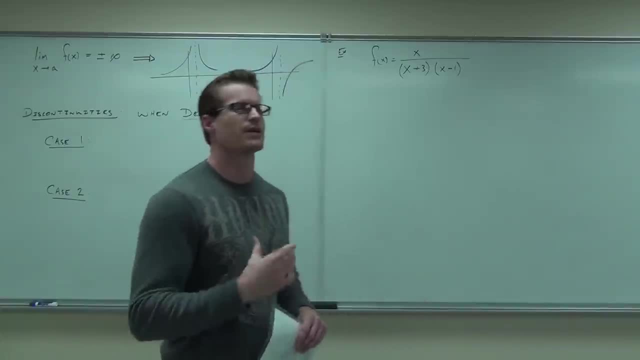 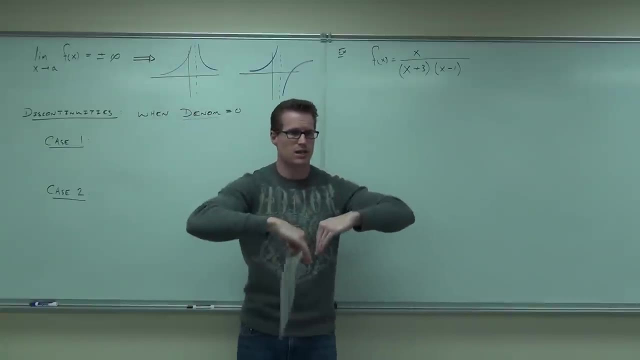 as we approach some number and it goes to infinity, we're going to have an asymptote. We're going to have either an asymptote where the limit exists, as they both go to positive infinity. I didn't draw the case where they both go to negative infinity. 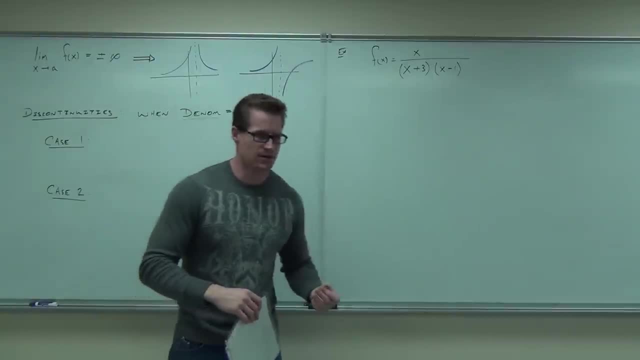 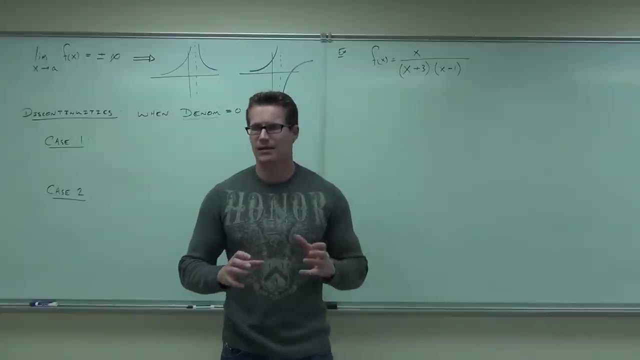 or where one goes to positive and one goes to negative. and then we'd find that with the sine analysis test, Now there were two cases where discontinuities existed. We had wholes and we had asymptotes. Do you remember those, the wholes and the asymptotes? 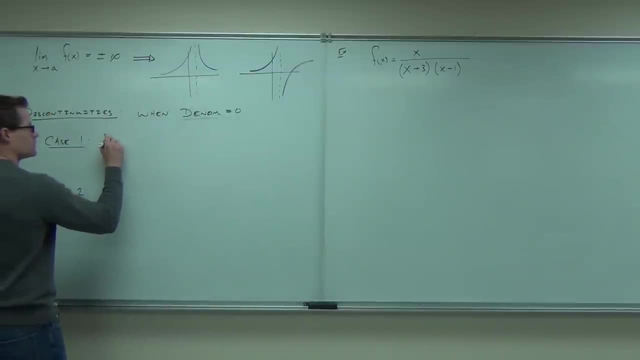 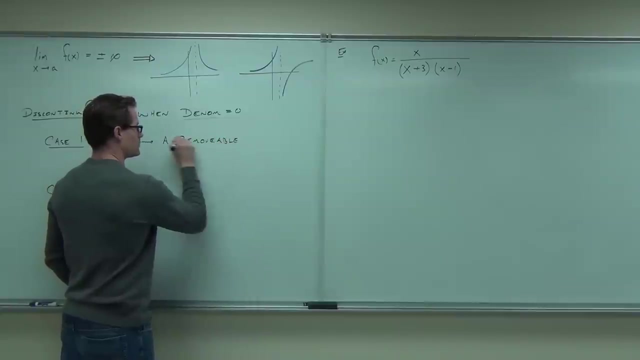 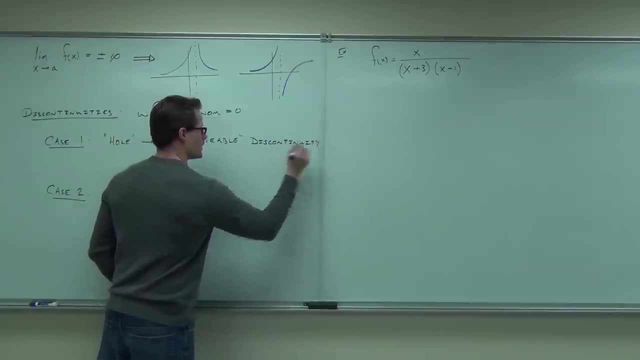 The wholes. So the wholes and the asymptotes was what was called a removable discontinuity. What it meant was that only a single point is missing from that function, One little single point. That was what defined a removable discontinuity, and it exists. 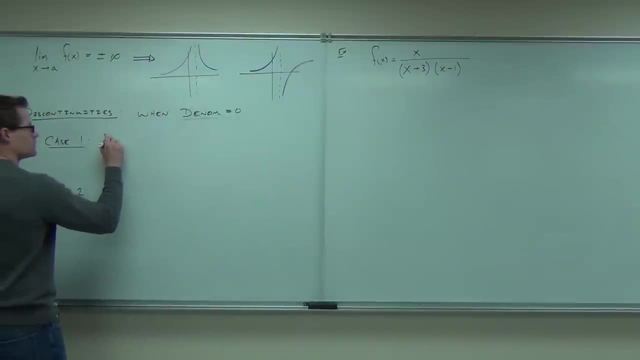 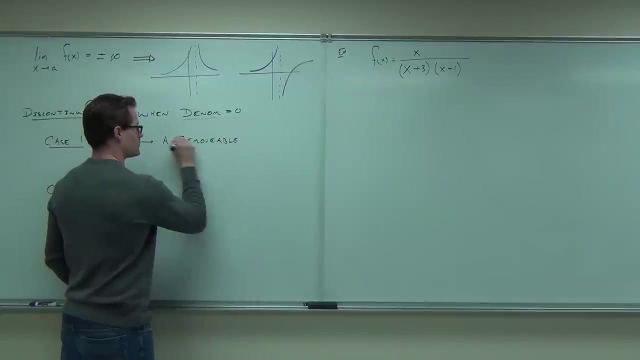 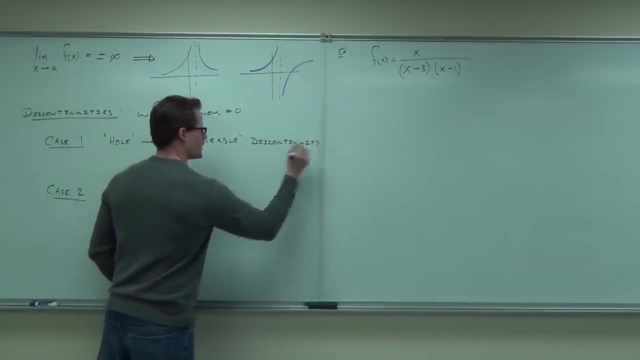 The wholes Okay. So we have two cases where discontinuities existed. The first case was what was called a removable discontinuity. What it meant was that only a single point is missing from that function, one little single point. That was what defined a removable discontinuity, and it exists. 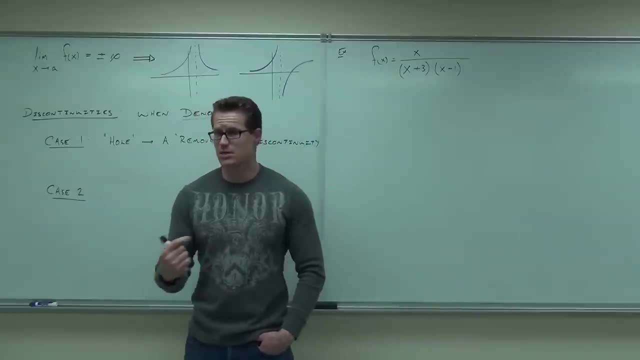 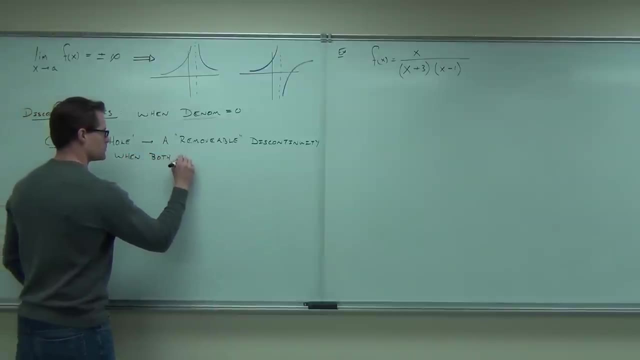 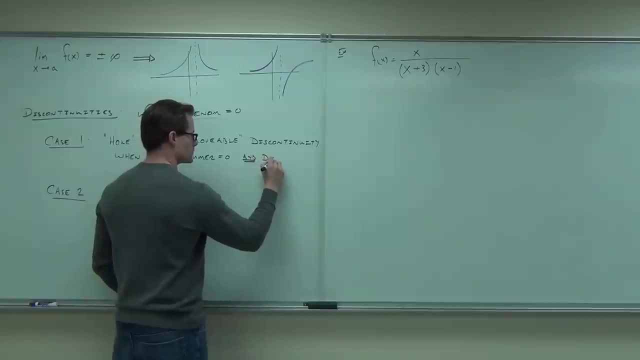 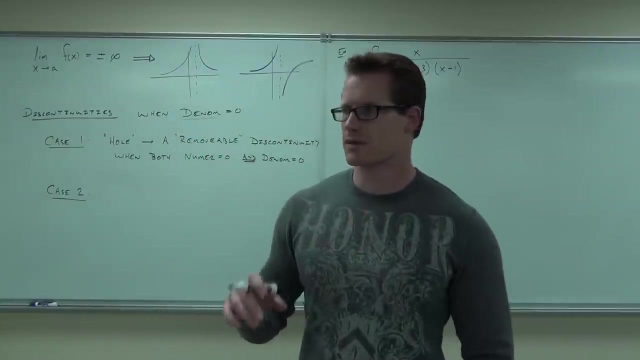 when the numerator is negative, The denominator and the denominator equals zero at the same time. Why was that the case? Well, if both the numerator and denominator equals zero at the same point, you're going to have a factor of x minus that value that you could cross out. 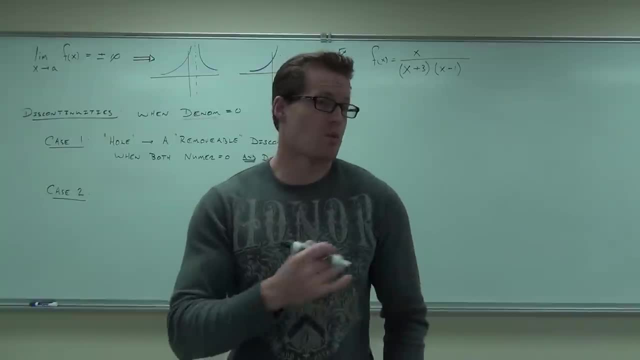 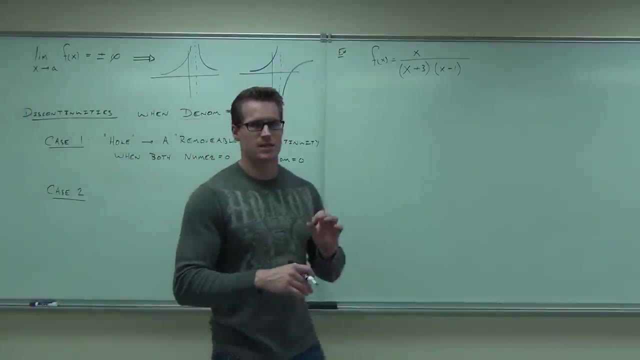 Remember crossing out those, Those problem areas. That was a removable discontinuity Now, or a whole. If we don't have that, if the numerator equals a number and the denominator equals zero and you cannot cross it out and you can't simplify it, it's not removable. 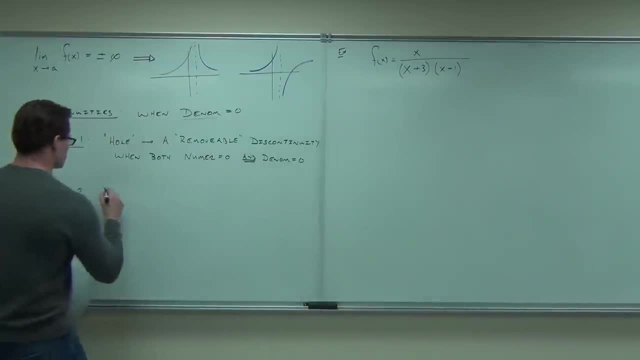 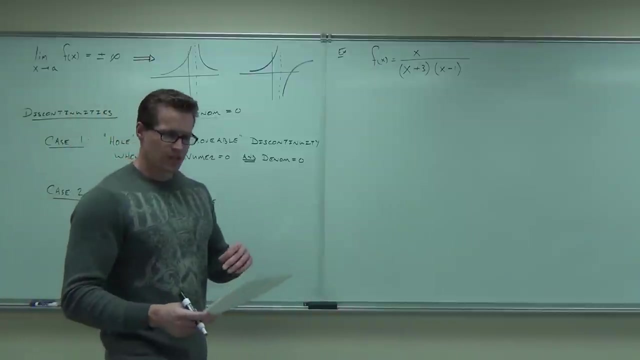 That means we have an asymptote. So case two is where we had the asymptote, a vertical asymptote, A vertical asymptote. This is when you can't cancel out. I know you love to use that word: cancel out, right. 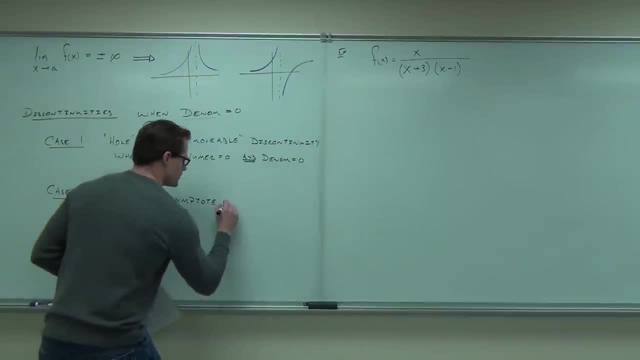 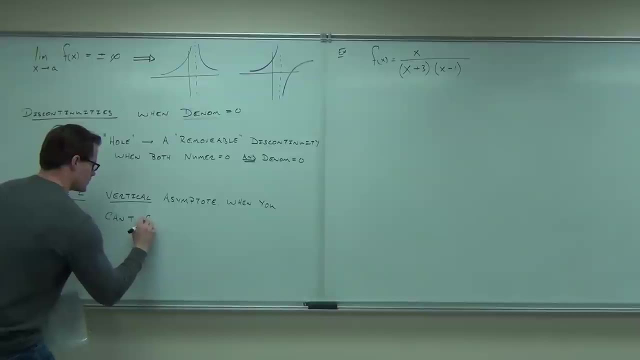 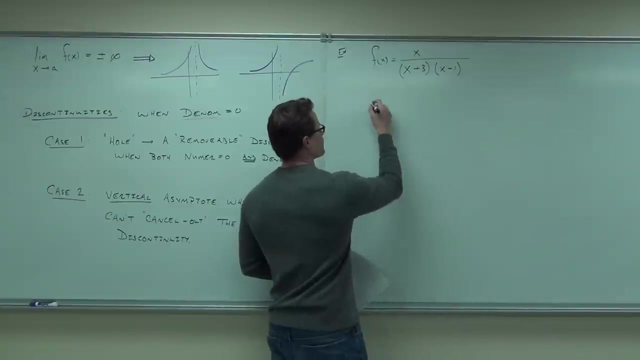 Where you can't cancel out the discontinuity or you can't remove it. Let's do an example here, real quick, okay, Let's do an example. Can you tell me where discontinuities exist? So any discontinuities? How about? x equals zero. 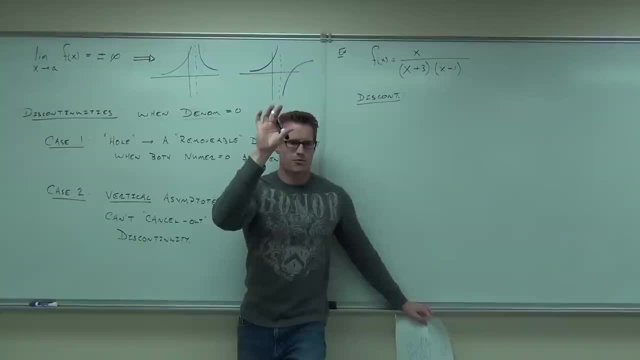 Is that a discontinuity or not? Is it okay to have zero on the top of a fraction? Sure, that's zero, That's a point. Give me one discontinuity. One One would work. sure, because if I plug in one, 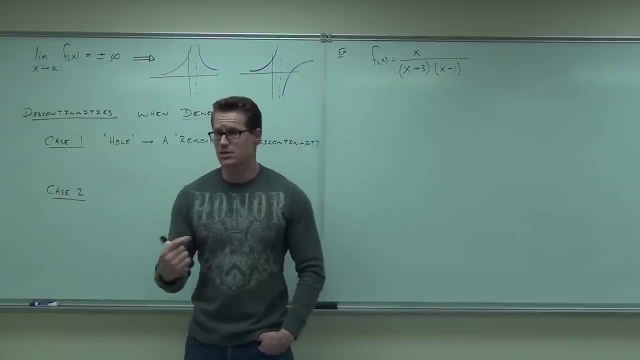 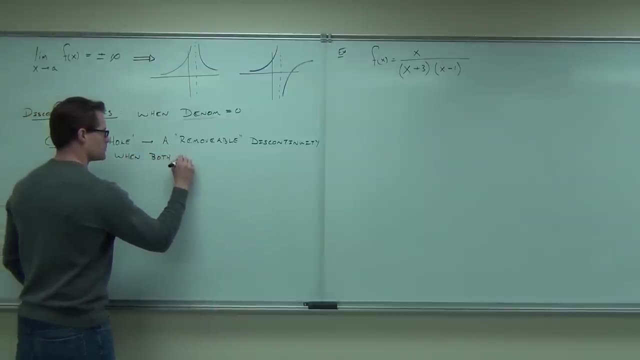 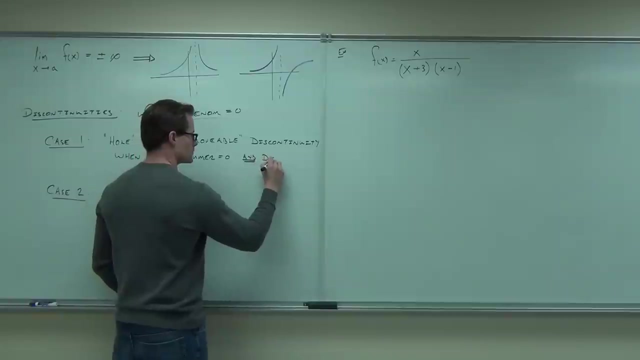 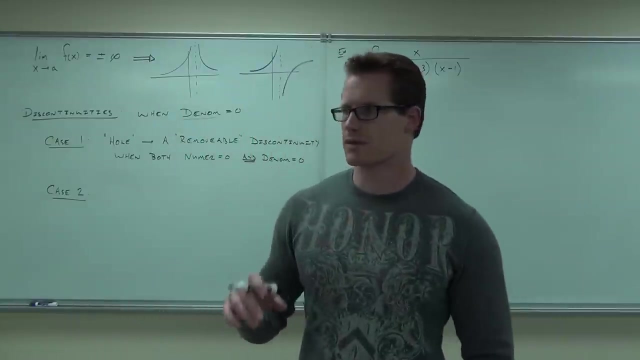 when the numerator is negative, The numerator and the denominator equals zero at the same time. Why was that the case? Well, if both the numerator and denominator equals zero at the same point, you're going to have a factor of x minus that value that you could cross out. 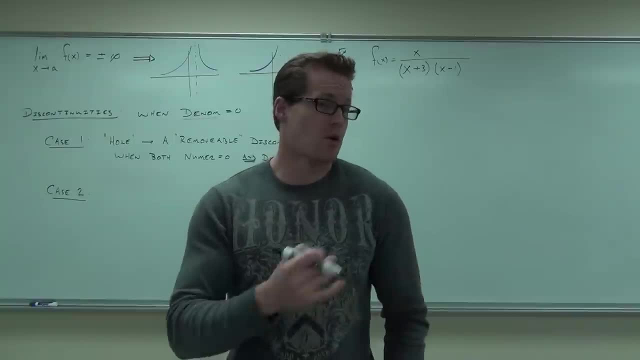 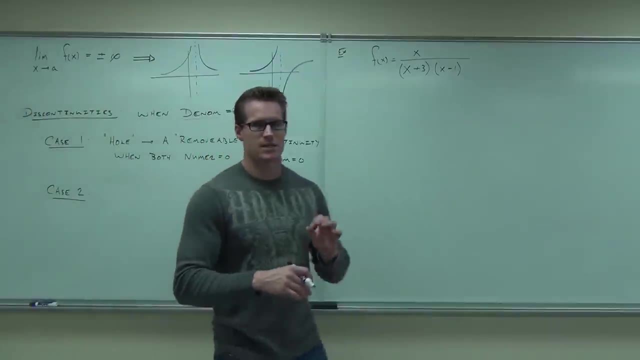 Remember crossing out those, Those problem areas. That was a removable discontinuity Now, or a whole. If we don't have that, if the numerator equals a number and the denominator equals zero and you cannot cross it out and you can't simplify it, it's not removable. 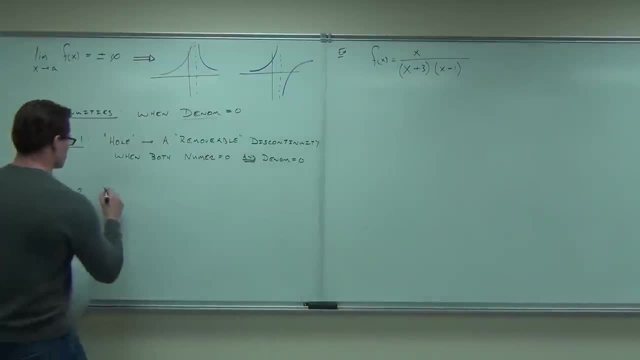 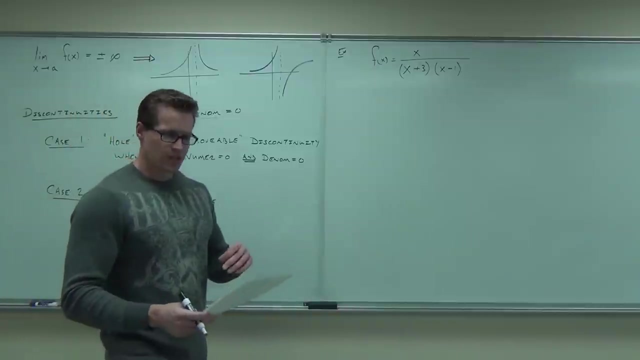 That means we have an asymptote. So case two is where we had the asymptote: a vertical asymptote. A vertical asymptote, All right, all right. so the vertical asymptote is here. It's not removable, It's a removable asymptote. 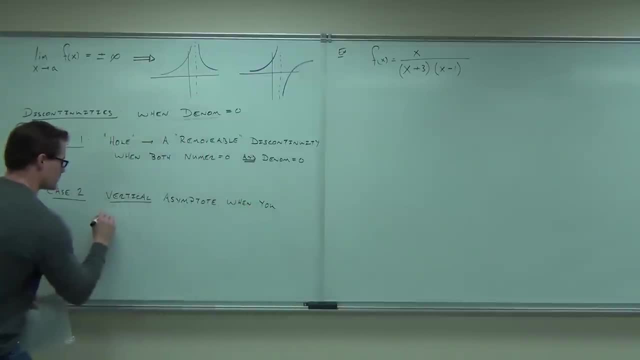 So the vertical asymptote? what's a vertical asymptote? It's a hierarchical DY, right? Okay, so that's when you can't cancel out- I know you love the use of the word cancel out- right Where you can't cancel out the discontinuity or you can't remove it. 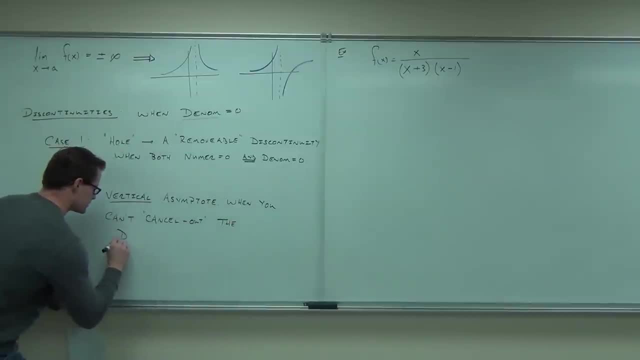 Okay, Okay. so the difference between: okay, so this is the vertical asymptote, all right, and then this is the vertical asymptote, All right, Let's do an example here real quick. okay, Let's do an example. 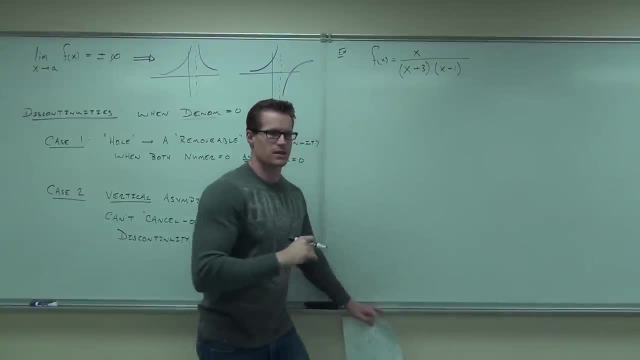 Can you tell me where discontinuities exist? So any discontinuities. How about? x equals zero. Is that a discontinuity or not? Is it okay to have zero on the top of a fraction? Sure, that's zero. That's a point. 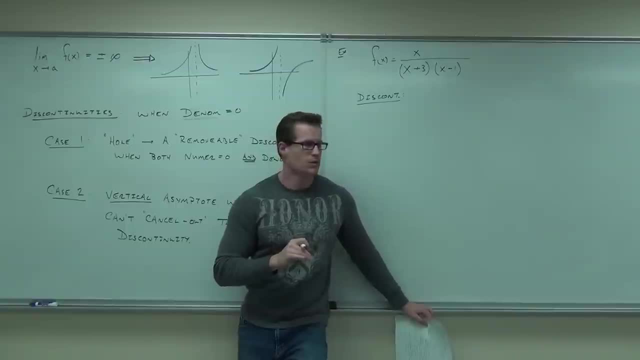 Give me one discontinuity. One One would work, sure, Because if I plug in one, I'm going to get zero in the denominator. That's a discontinuity. You follow me. So x equals one will be a spot in which we will have a discontinuity. 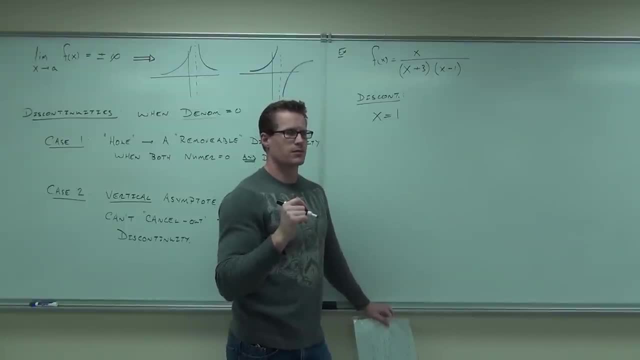 Give me another one, Someone on the left-hand side of the room. What do we have? Negative three would be another one, Sure. Now let me ask you a question about x equals one and x equals negative three. Are they wholes, Are they asymptotes? 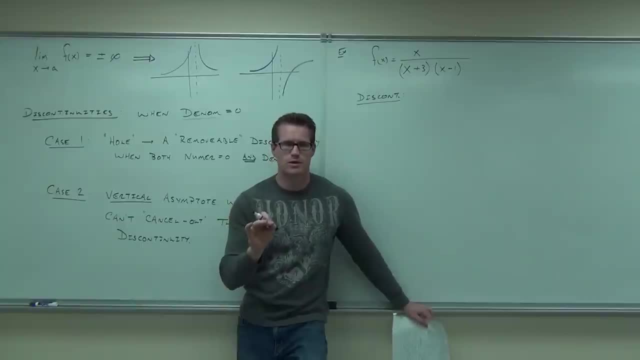 I'm going to get zero. I'm going to get zero on the denominator. That's a discontinuity. You follow me. So x equals one will be a spot in which we will have a discontinuity. Give me another one, Someone- left hand side of the room. 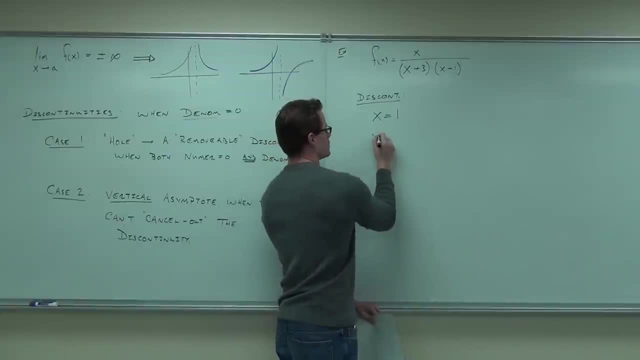 What do we have? Negative three would be another one, sure? Now let me ask you a question about x equals one and x equals negative three. Are they wholes? Are they asymptotes? Is one a whole? Is one an asymptote? 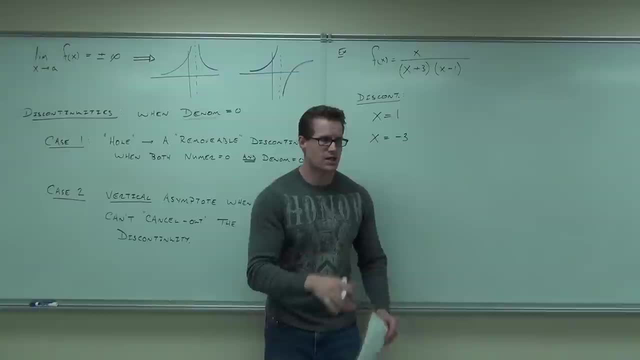 What do you think? And the answer to the question is: can you cross out where the discontinuity happens? So basically, can you cross out, Can you cross out the x minus one, Can you cross out the x plus three. So are those wholes or asymptotes? 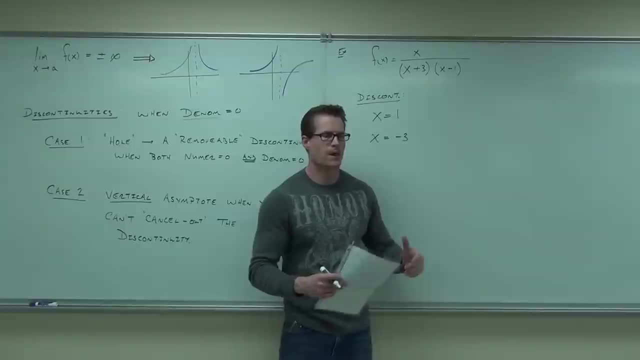 Those are both asymptotes, both of them. Now stop for a second, Just watch. What if I had done this, please? Which one would be the asymptote in this case? That would be the asymptote here, and that would be a removable discontinuity, or 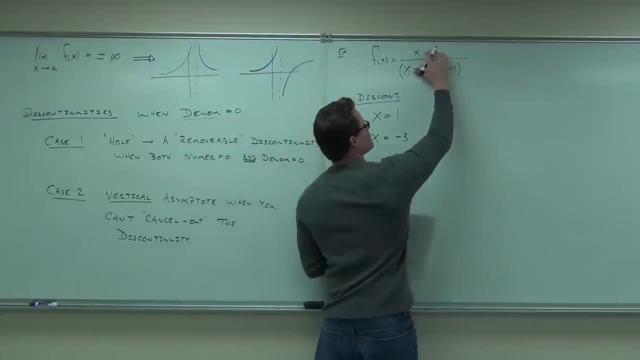 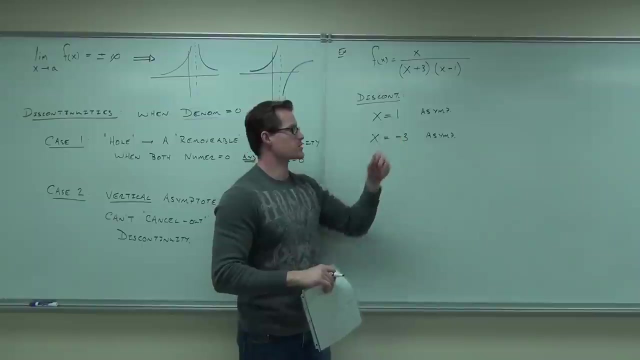 in other words a whole. Do you follow that? Okay, good, So I'm going to change it back to this. This is an asymptote, And that's an asymptote if I have just x over x plus three and x minus one. 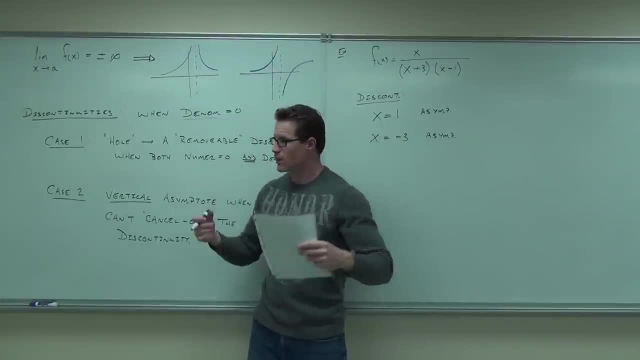 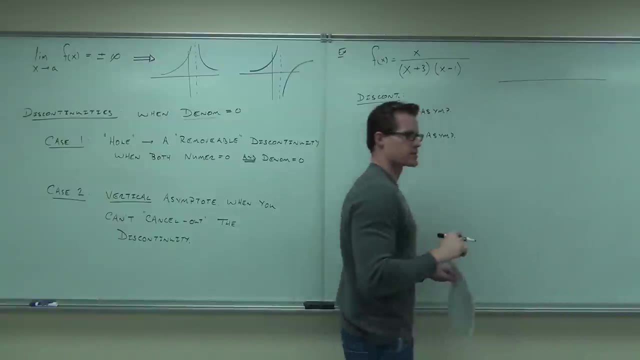 Those are vertical asymptotes. Do you recall how to find out what the limit is around those? Do you remember that Yep sine analysis is how you do it? You'd put the negative three And you know it's going to be asymptote. 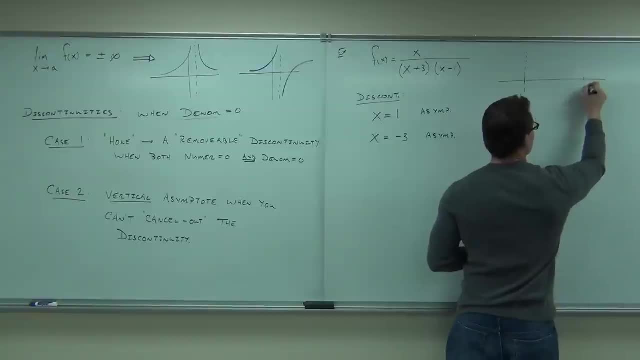 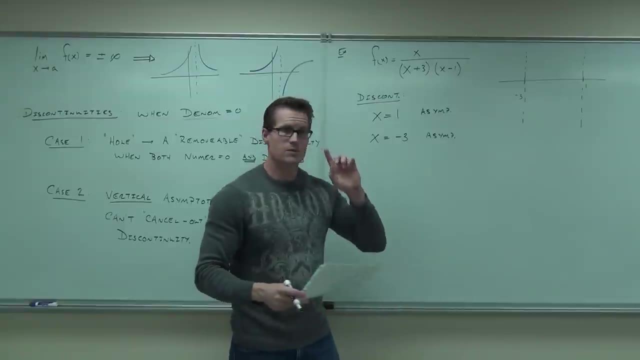 because we just talked about that. It's going to be an asymptote there And you put the positive one And you know it's going to be an asymptote, And then all you have to do is plug in some numbers for those intervals because, look at it, 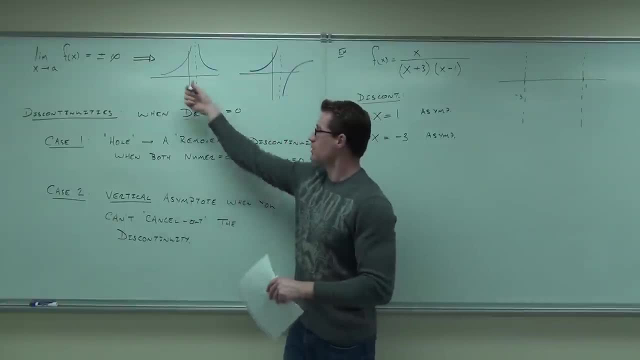 Look If it's an asymptote. look at the board here real quick. You know it's going to be one of these cases, right, It's either going to go this, that or be opposite. So it's going to be one of those. 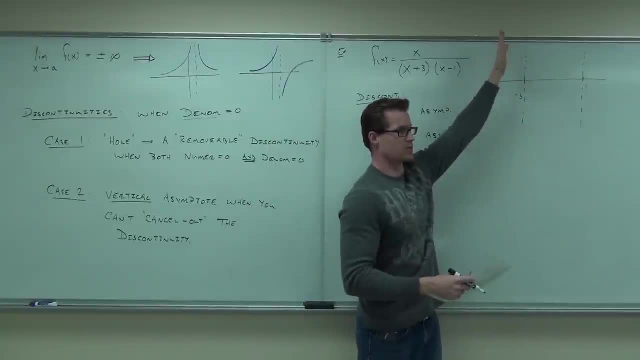 All you have to do is plug in numbers. If it's positive, it's going positive. If it's negative, it's going negative. Same thing in here: Positive, positive, negative, negative. Same thing here, Positive or negative. 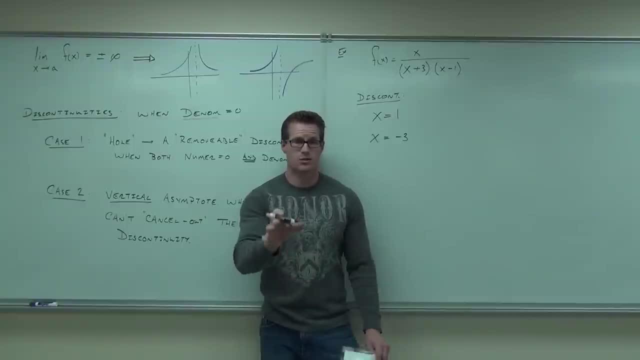 Is one a whole? Is one an asymptote? What do you think? And the answer to the question is: can you cross out where the discontinuity happens? So, basically, can you cross out the x minus one? Can you cross out the x plus three? 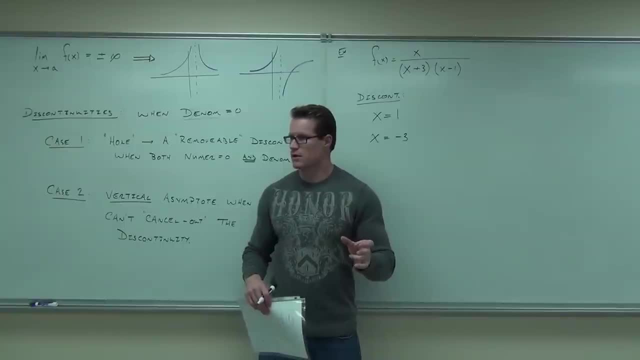 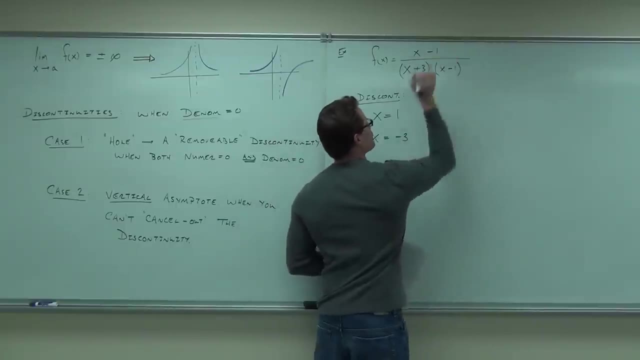 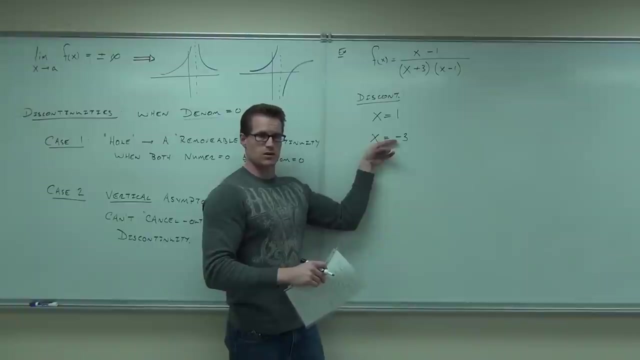 So are those wholes or asymptotes? Those are both asymptotes, Both of them. Now stop for a second, Just watch. What if I had done this, please? Which one would be the asymptote in this case? That would be the asymptote here. 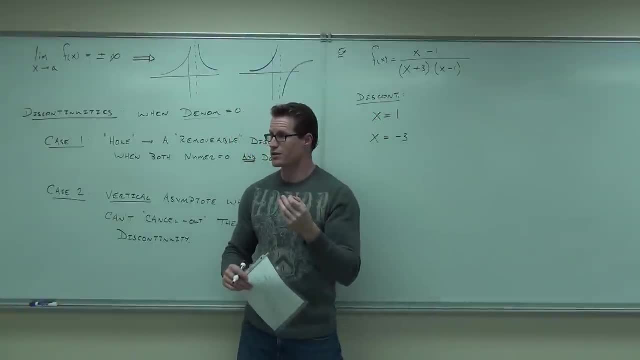 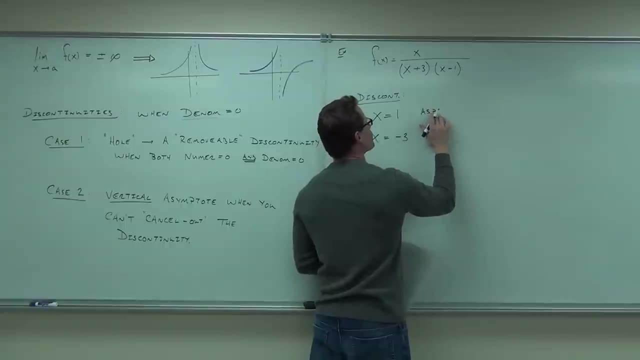 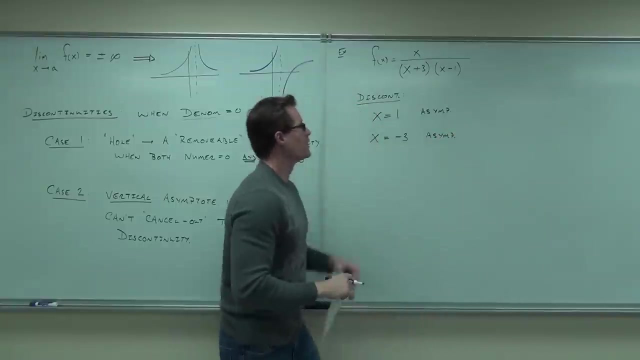 And that would be a removable discontinuity, or in other words, a whole. Do you follow that? Okay, good, So I'm going to change it back to this. This is an asymptote And that's an asymptote If I have just x over x plus three and x minus one. those are vertical asymptotes. 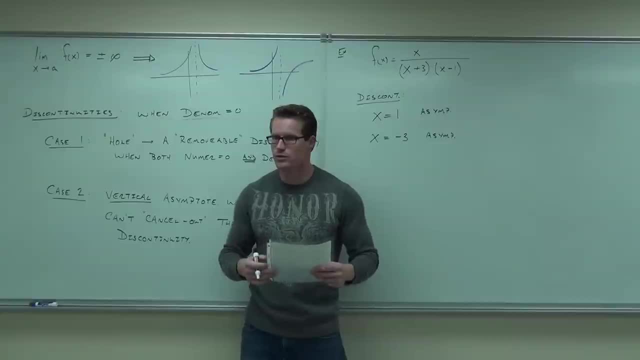 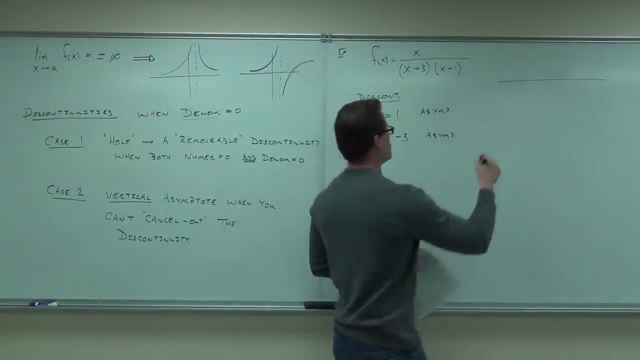 Do you recall how to find out what the limit is around those? Do you remember that Yep sine analysis is how you do it. You'd put the negative three And you put your negative three And your plus one And you know what's going to be: negative three. 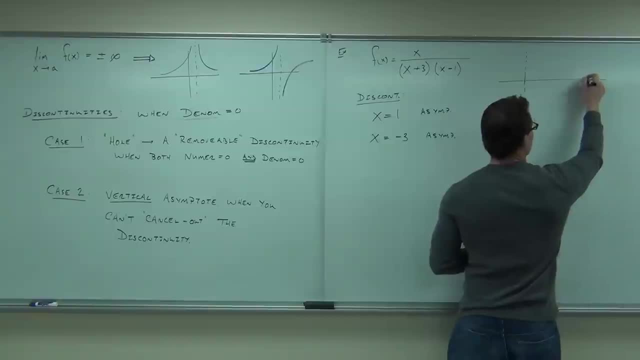 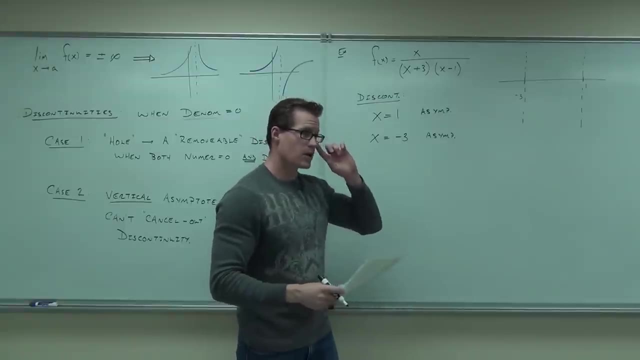 And you know what's going to be an asymptote, because we just talked about that. It's going to be an asymptote there And you put the positive one And you know what's going to be an asymptote, And then all you have to do is plug in some numbers for those intervals. 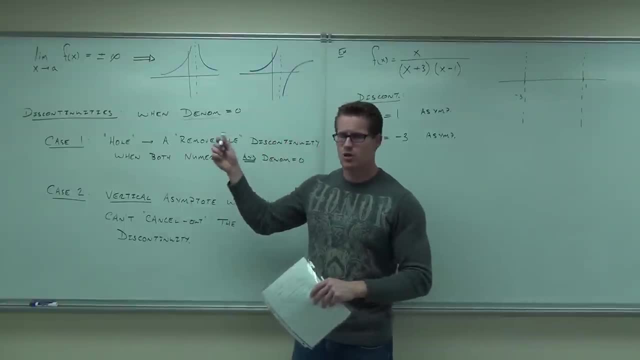 Because look at it, Look If it's an asymptote, look at the board here. real quick, You know what's going to be one of these cases. right, It's either going to go this, that or be opposite. So it's going to be one of those. 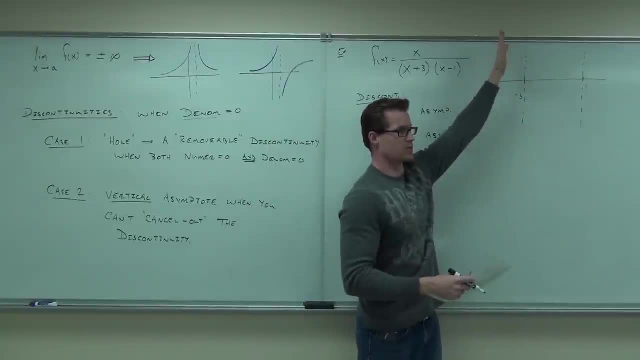 All you have to do is plug in numbers. If it's positive, it's going positive. If it's negative, it's going negative. Same thing in here: Positive, positive, negative, negative. Same thing. Same thing here, Positive or negative. 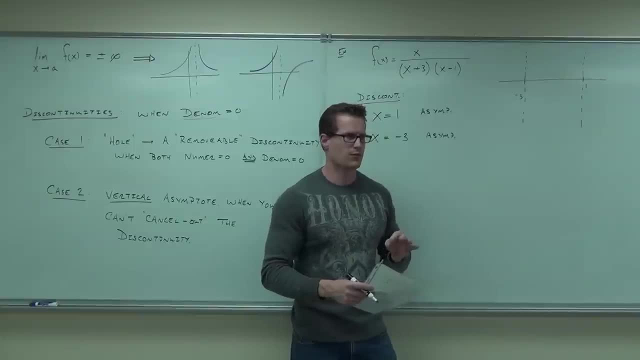 Now there's one thing you have to be careful of, One very important thing for us right now. Do you see that the numerator will equal zero at zero? That point's not going to be an asymptote, but it will. It will change the sign of your fraction. 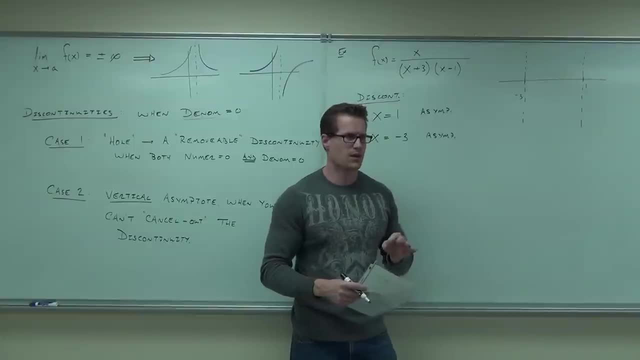 Now there's one thing you have to be careful of, One very important thing for us right now. Do you see that the numerator will equal zero at zero? That point's not giving me an asymptote, but it will. It will change the sign of your fraction. 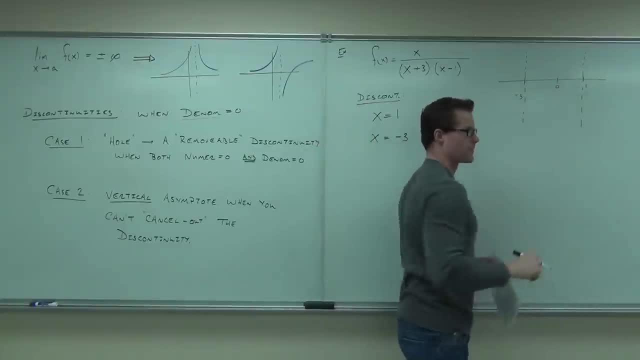 So you're going to put a little marker in here at zero, And the only reason why you're going to do it is because a number in this region could potentially be different than a number in this region concerning the sign. Does that make sense to you? 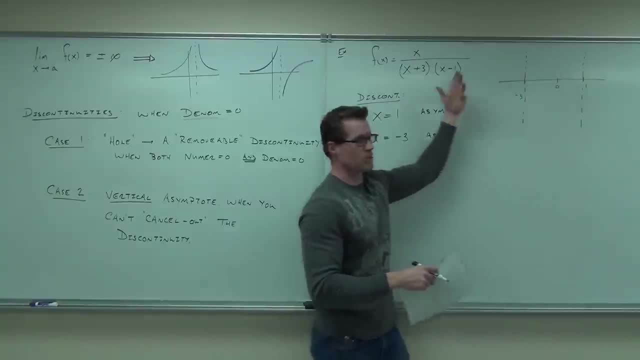 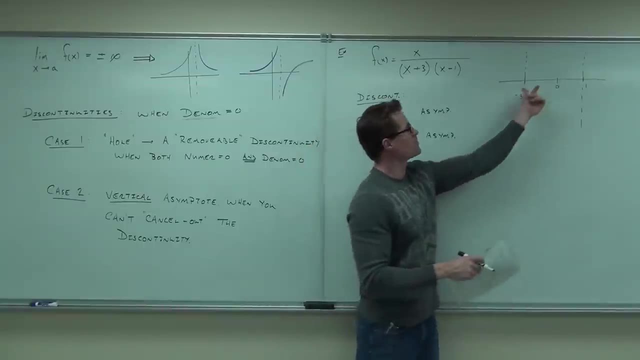 So that's a separator, Because if you just plug in zero, you're going to get zero, right, That doesn't tell you positive or negative. That could be a case where you're switching from positive to negative, So you have to put that plug in a number here and plug in a number here. 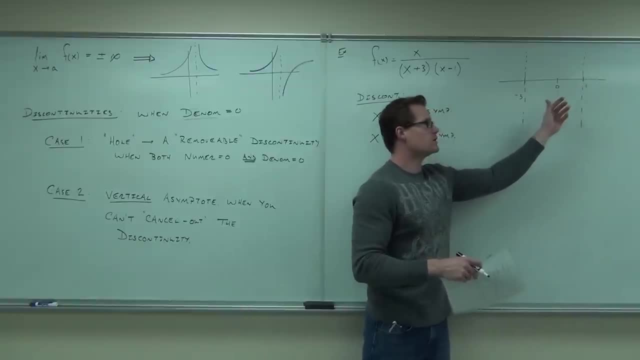 And that'll tell you. So it's like having four intervals instead of two or three. You have just three intervals. but that's a separating marker which says I can't plug in just one number here. I need to plug in two different numbers. 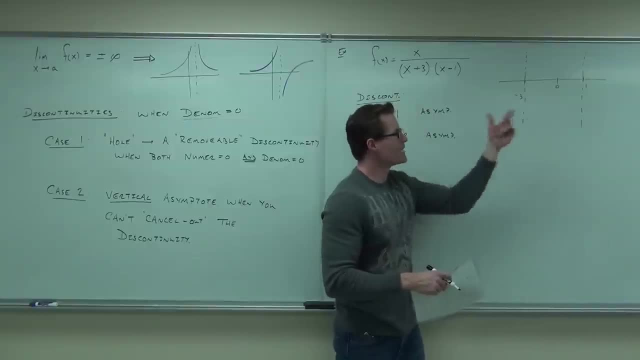 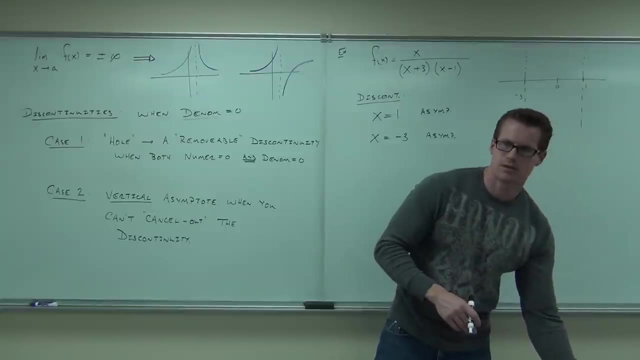 So you only have two asymptotes, There's not three asymptotes. But it's like, yes, like you're testing four intervals, Okay, Feel okay with this. Why don't we see what happens? Why don't you plug in negative four? 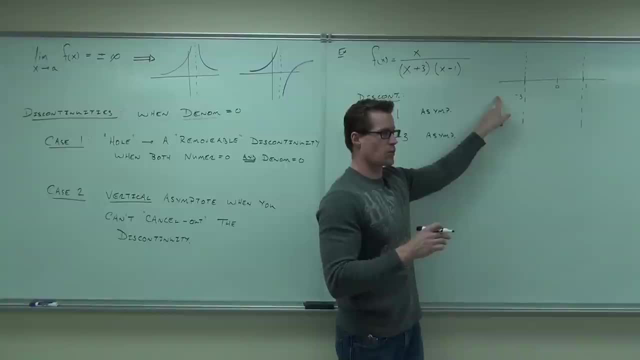 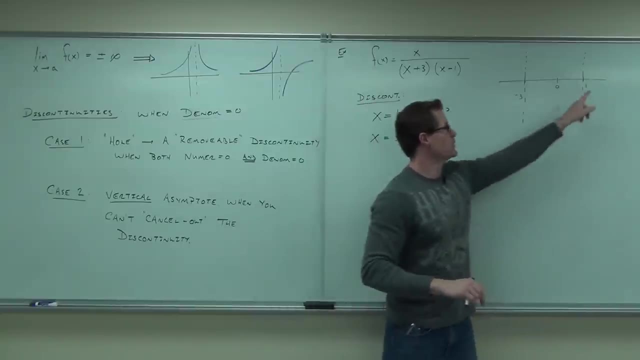 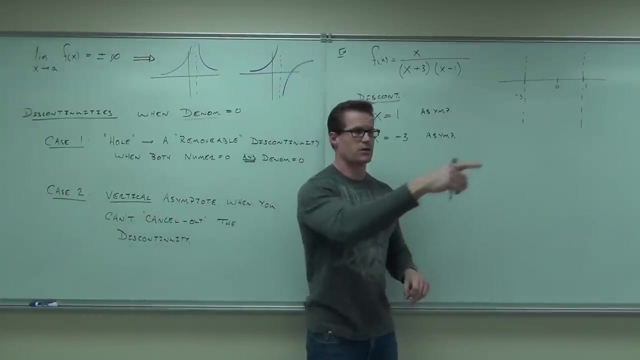 So how about this? U2 rows do negative, four, U2 rows do negative one, U2 rows do .5. And U2 rows do two. Okay, Can you tell me that? Have you already done the two? When you have them, let me know. 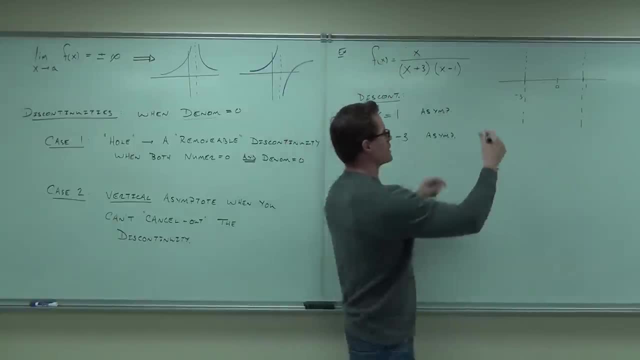 It's negative. So you plug it into here, right, And you get negative. I don't care what the value negative, It's going to be that one, These two rows. have you plugged in negative one here, Negative, Negative. 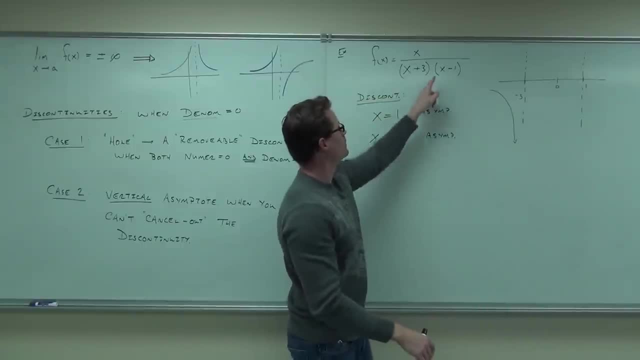 Really Positive, Positive, Negative, positive, negative, positive, Positive. How about .5?? Positive, positive, Negative. How about two? Positive, Negative, Negative, Positive, Negative, Positive Negative. Here's my question: Will the limit exist? will the limit exist as we approach negative three? 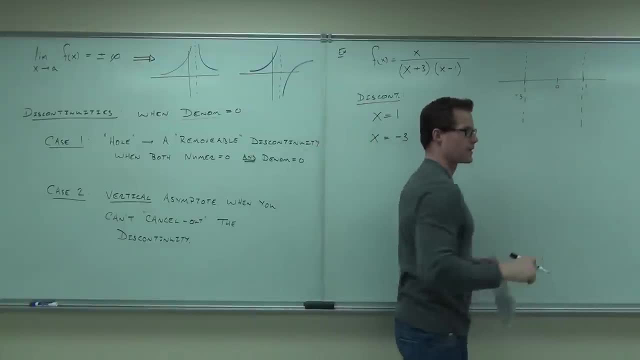 So you're going to put a little marker in here at zero, And the only reason why you're going to do it is because a number in this region could potentially be different than a number in this region. Does that make sense to you? So that's a separator. 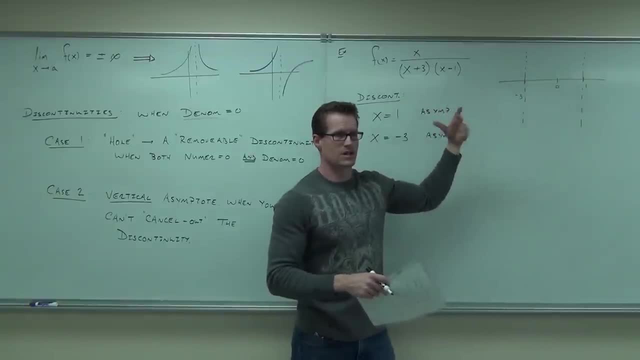 Because if you just plug in zero, you're going to get zero, right, That doesn't tell you positive or negative. That could be a case where you're switching from positive to negative, So you have to put that plug in a number here. 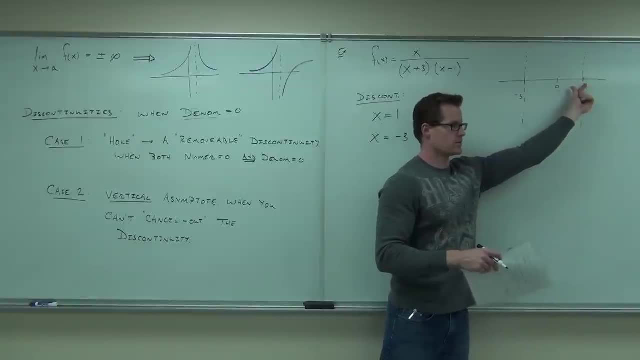 and plug in a number here and that'll tell you. So it's like having four intervals, except for two Or three. You have just three intervals, but that's a separating marker which says I can't plug in just one number here. 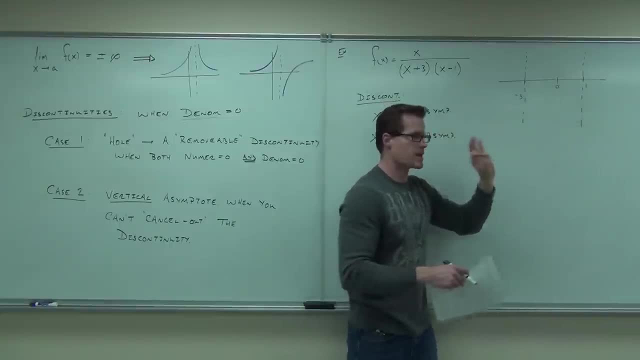 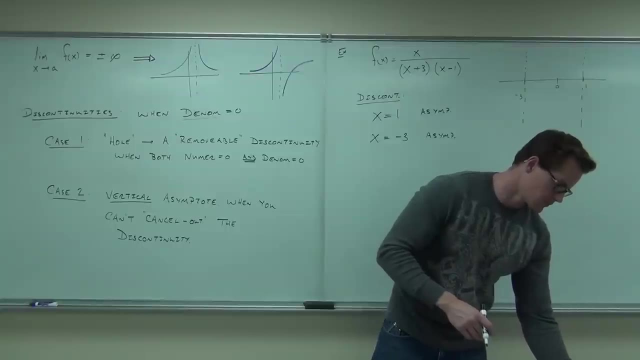 I need to plug in two different numbers, So you only have two asymptotes. There's not three asymptotes. but it's like, yes, it's like you're testing four intervals. Okay, Feel okay with this. Why don't we see what happens? 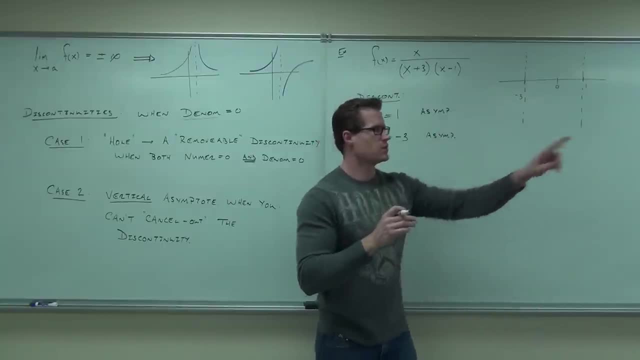 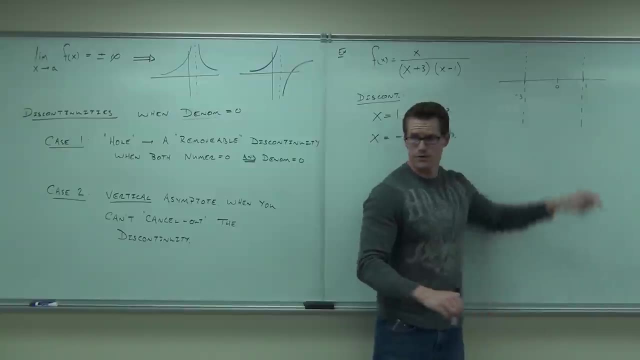 Why don't you plug in negative four? So how about this? U2 rows do negative four, U2 rows do negative one, U2 rows do .5, and U2 rows do two. okay, Can you tell me that? Have you already done the two? 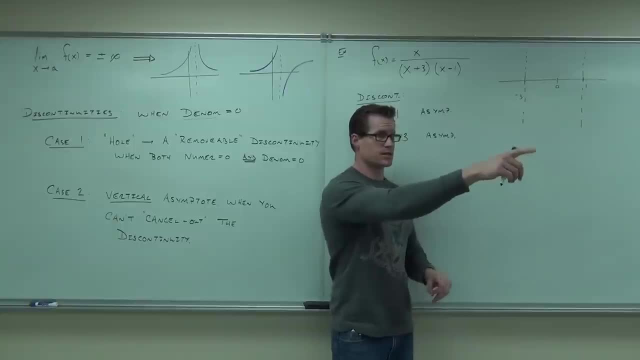 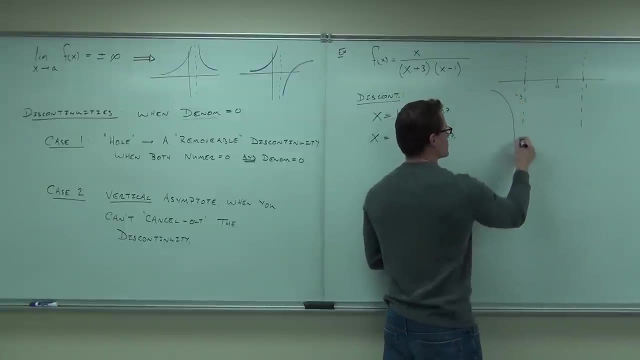 When you have them, let me know It's negative, So you plug it into here. right, You got negative. I don't care what the value negative, It's going to be. that one, These two rows. have you plugged in negative one yet? 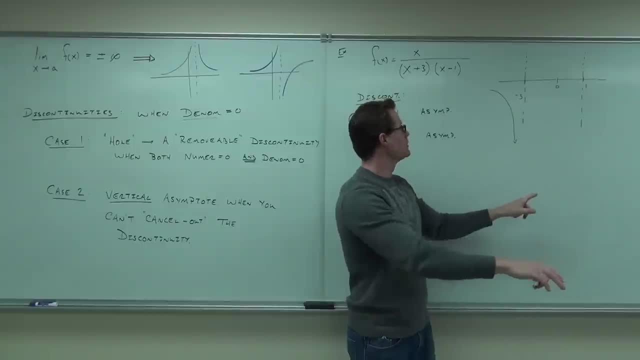 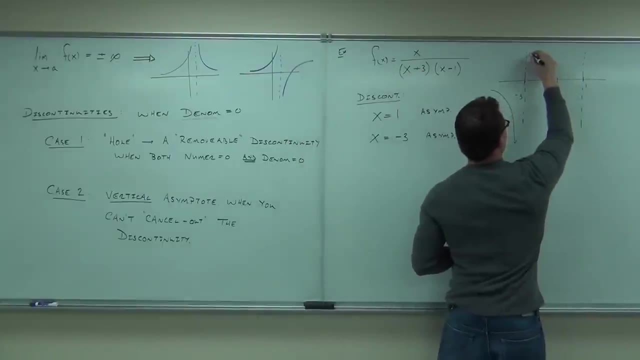 Negative, Negative, Really Positive, Negative, positive, negative, positive, Positive. How about .5? Positive positive, negative? How about .5? Negative? How about .5? Positive, Positive, Negative, Positive, Positive. 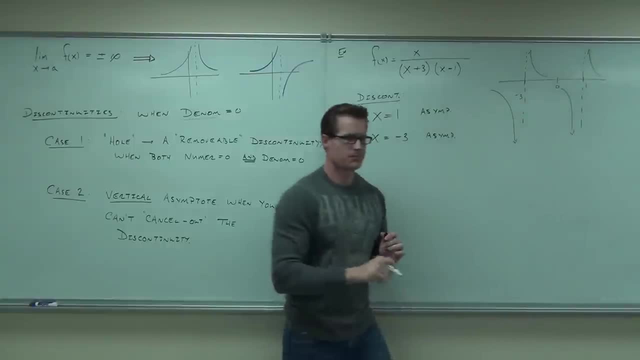 Positive, Negative, Positive, Positive, Negative, Positive, Positive. Here's my question: Will the limit exist? will the limit exist as we approach negative three? From the left we're going down, from the right we're going up. Does it exist? 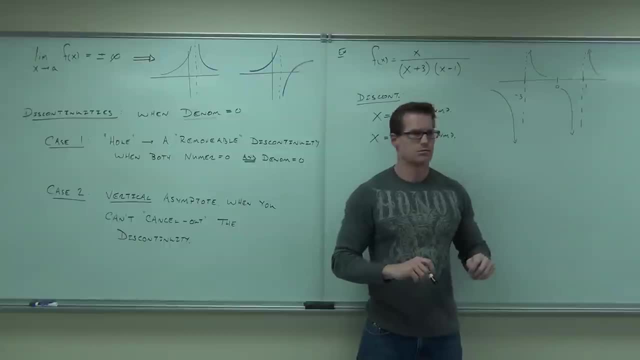 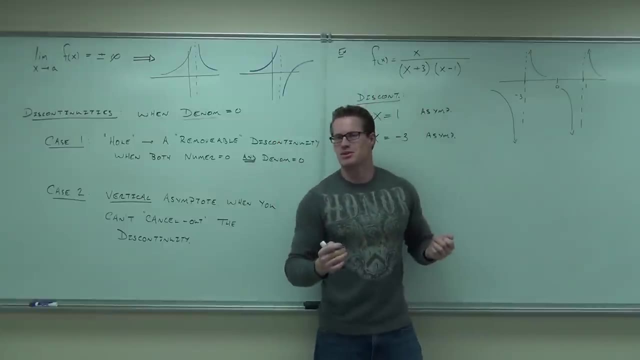 No, I think no. How about at one, No, No, No. From the left we're going down, from the right we're going up. If they had been like this, both going up, both going down, Sure, How about this question? trick question. 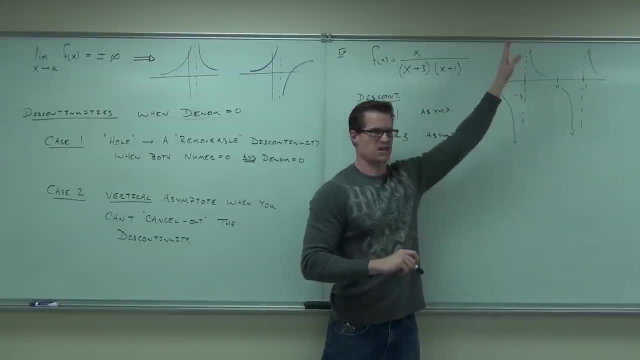 From the left we're going down, from the right we're going up. Does it exist? Heck? no, How about? at one Nope. From the left we're going down, from the right we're going up. If they had been like this- both going up, both going down- sure. 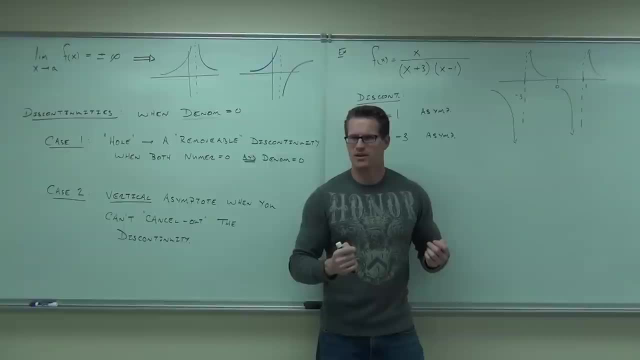 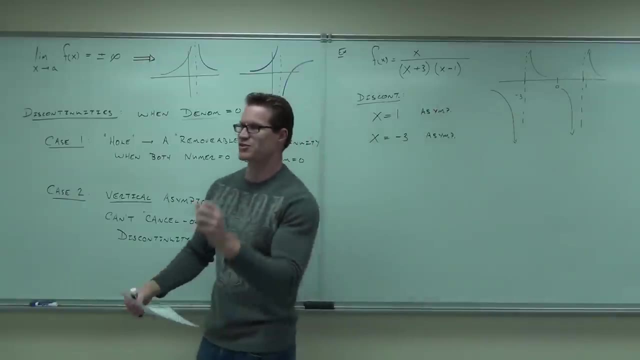 How about this question, trick question: Does the limit exist at zero? Yeah, Absolutely, That's a point. There's no asymptote there. Right, That's a point. The limit does exist at zero. Ah, trick job. Thank you, Joe. 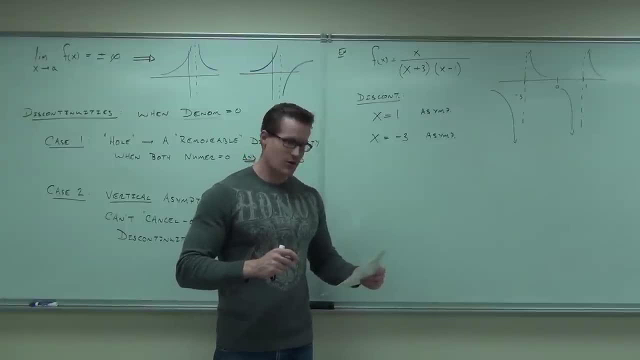 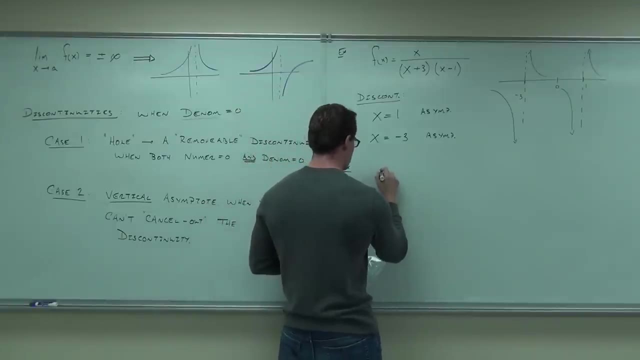 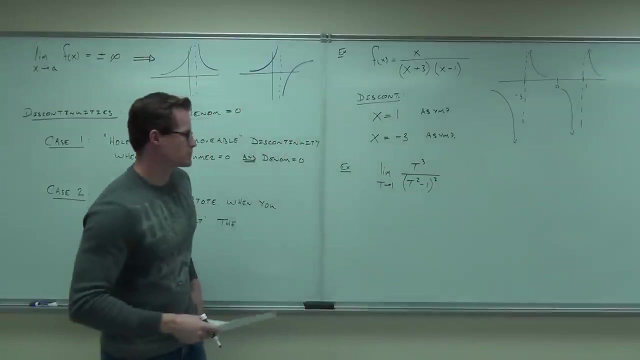 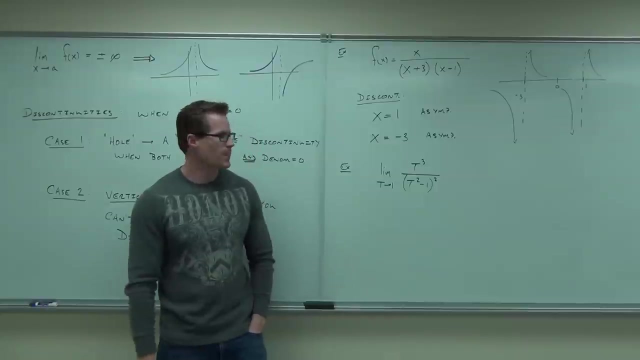 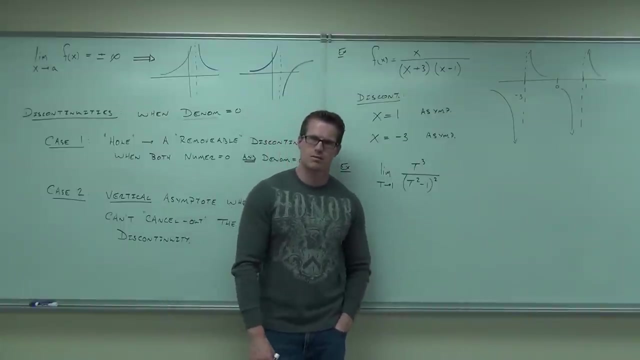 Hopefully. yeah, Feel okay with this so far. Could you do the same thing with something like this: Can you tell me where discontinuities exist on this problem? Where would they exist on this problem? Do you need to distribute all this out to tell that? 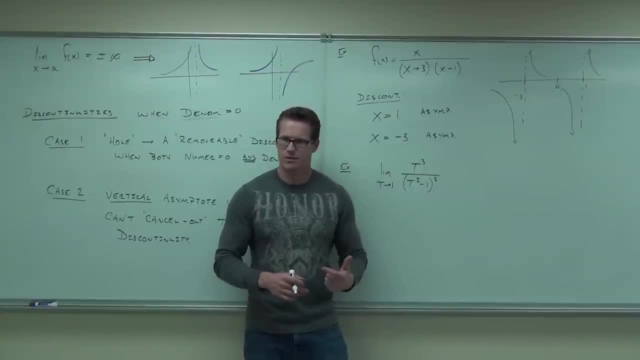 No, The only place where discontinuities are going to exist is where the denominator equals zero. True, So where the denominator equals zero is where this little piece equals zero. You follow: Where is that going to equal zero? Where is that going to equal zero? 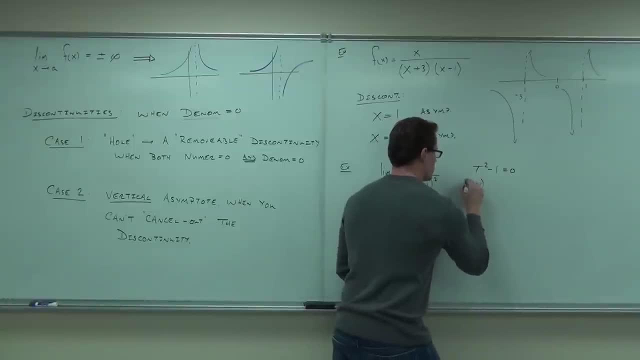 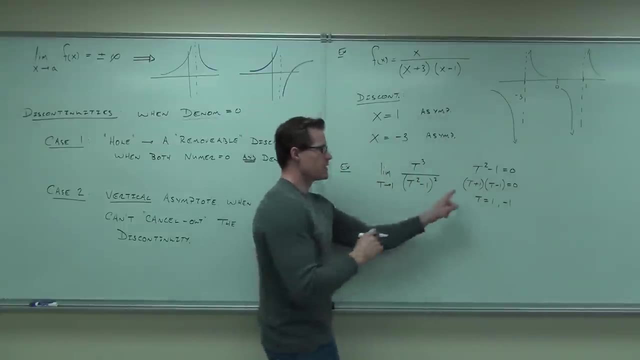 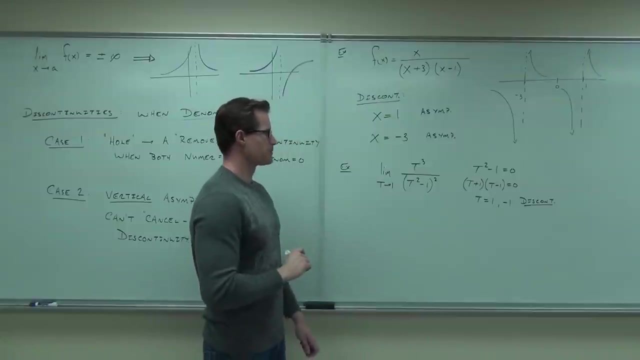 Uh-huh. So these are my discontinuities. Would you say that those are wholes or asymptotes? Explain why they're asymptotes. Yes, Because they can't be deleted. Okay, They can't be removed. That's exactly right. 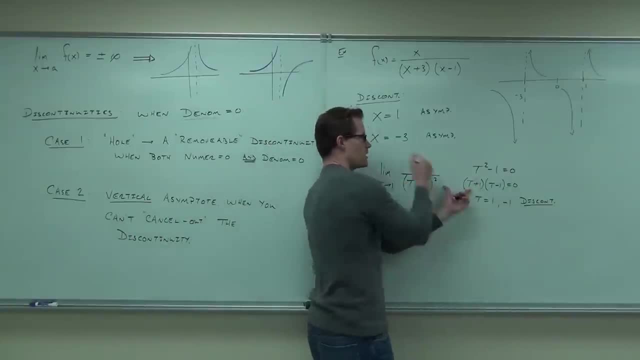 Can't be deleted is what you said. but absolutely, And even if you factored that, could you cross it out at all? Definitely not. So these are non-removable discontinuities, Those are asymptotes. So how could you find out where those asymptotes go? 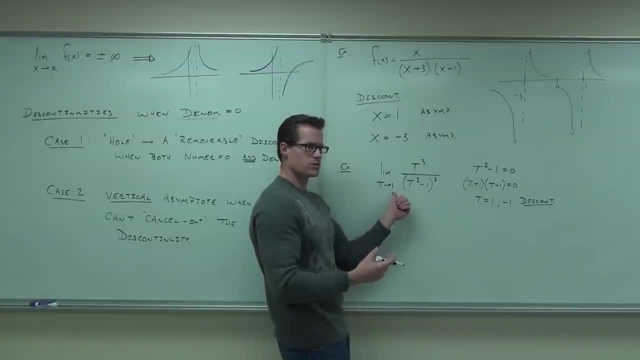 Well, this says really what we're concerned about is around the one. Do you see what I'm talking about? So from our chart here we've got two discontinuities, We've got negative one, We've got one, We've got two. 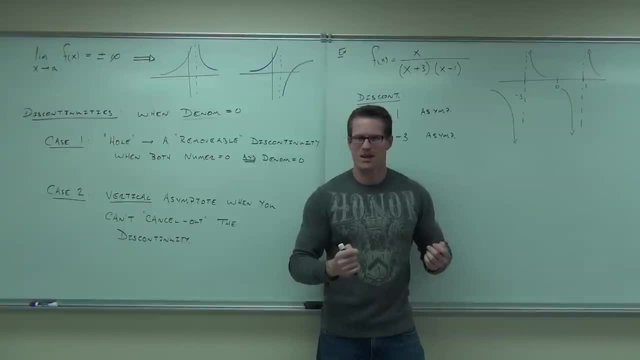 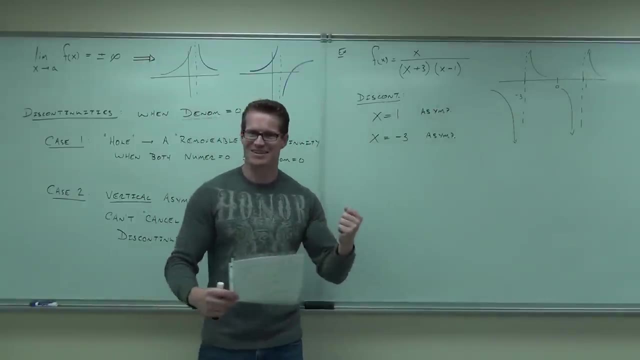 Does the limit exist at zero? Yes, Yes, Absolutely. that's a point. There's no asymptote there. right, That's a point. limit does exist at zero. Ah, trick job. thank you, Joe, Feel okay with it so far. 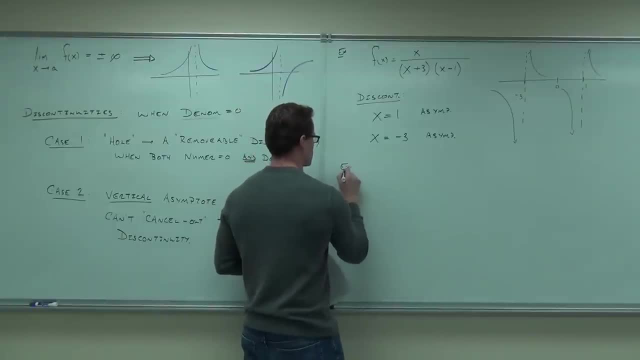 Could you do the same thing with something like this, Do the same thing with something like that? Can you tell me where discontinuities exist on this problem? Where would they exist on this problem? Do you need to distribute all this out to tell that? 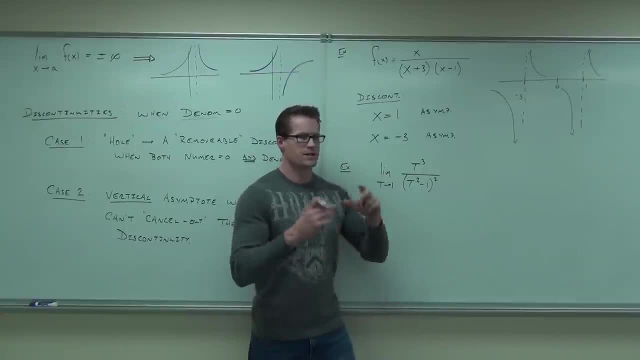 The only place where discontinuities are going to exist is where the denominator equals zero. true? So where the denominator equals zero is where this little piece, this little piece, equals zero. you follow, Where is that going to equal zero? Uh-huh. 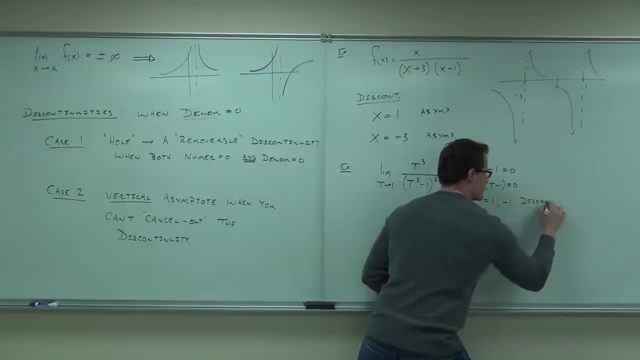 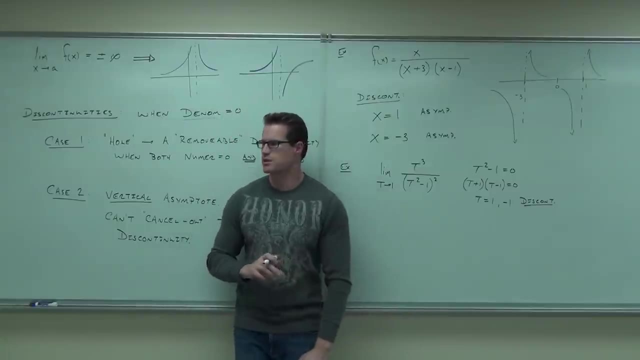 So these are my discontinuities. Would you say that those are holes or asymptotes? Explain why they're asymptotes. Because they can't be deleted. Okay, they can't be removed. that's exactly right. Can't be deleted is what you said, but absolutely. 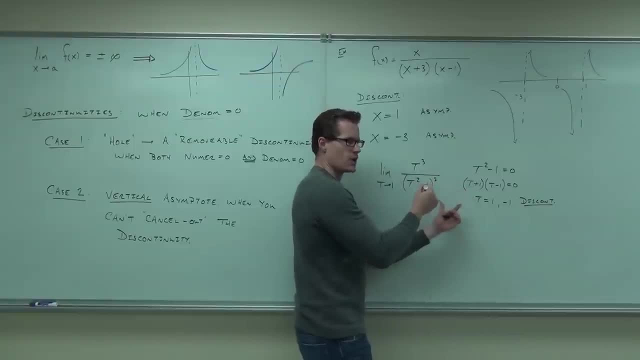 Even if you factored that, could you cross it out at all? Definitely not. So. these are non-removable discontinuities, Those are asymptotes. So how could you find out where those asymptotes go? Well, this says really what we're concerned about. 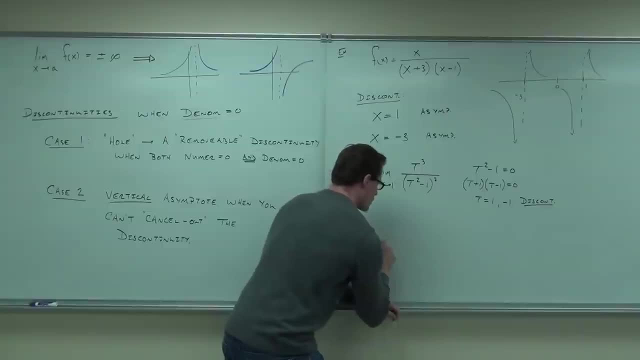 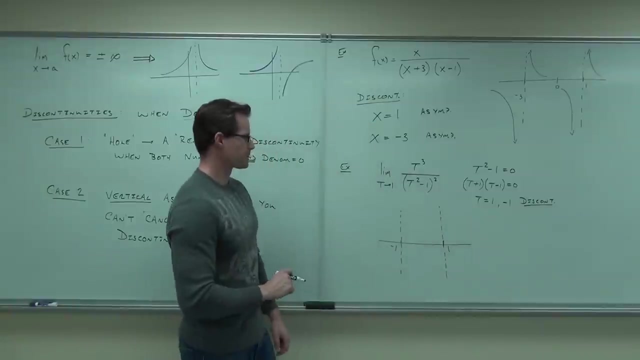 is around the one. Do you see what I'm talking about? So from our chart here, we've got two discontinuities, We've got negative one, We've got one, We've got one One and negative one, And what we're gonna do is check where these asymptotes go. 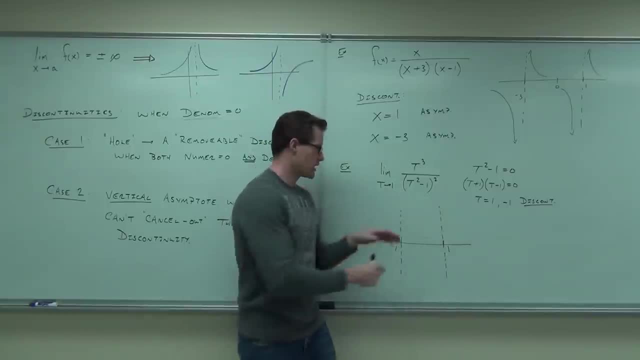 Now look up here at the board here real quick. Normally we would check all the asymptotes follow, But which one do I really care about? Do I care about the negative one? No, Why not? I don't care about the negative one. 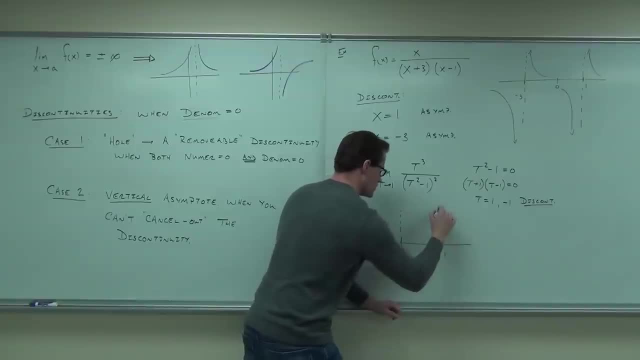 What do you think? One and negative one, And what we're going to do is check where these asymptotes go. Now look up here at the board here real quick. Normally we would check all the asymptotes Follow, But which one do I really care about? 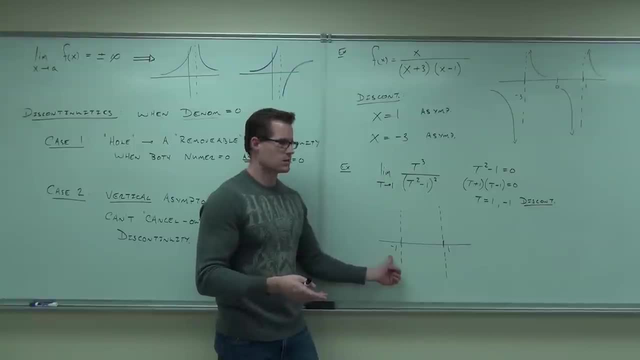 Do I care about the negative one? Why not izers one, Then it says one, Then it says one. So I don't care about that, I care about this. Sure, tell me one more point that I absolutely must have up here right now. 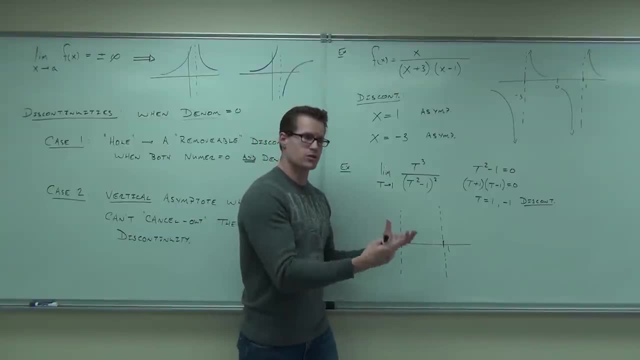 That's zero. That zero could be a change of sign. So where the numerator equals zero, that could also be a place where you wanna at least separate your interval. It's not gonna be an asymptote, but you definitely wanna plug in just to be safe. 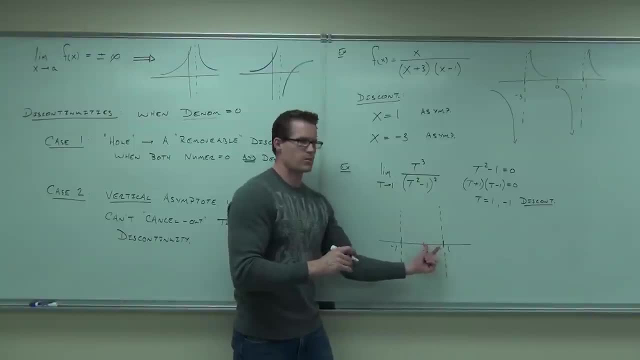 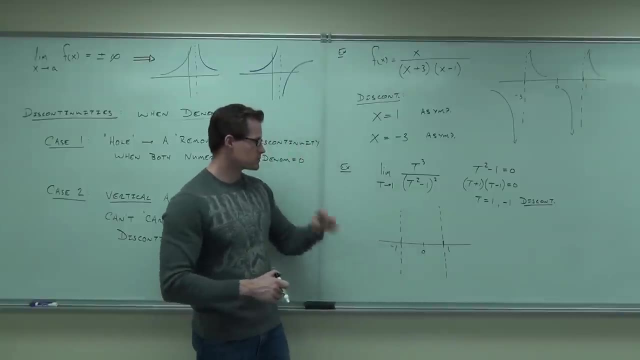 a number between zero and one. That's what you wanna do, So try that. People on the left-hand side, why don't you try .5?? Right-hand side, why don't you try two for me? We'll see what happens around that. 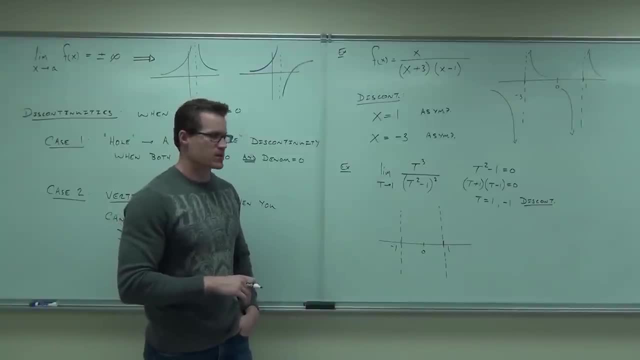 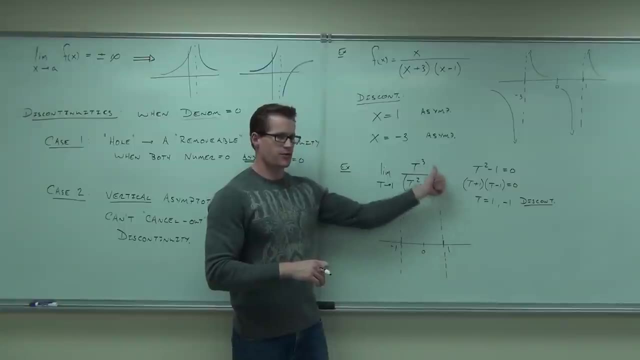 You shouldn't really be able to do it without a calculator, honestly, because when you think about it, this is gonna be a positive number, right? Positive, it doesn't matter, that's positive. Positive over positive is positive Up. 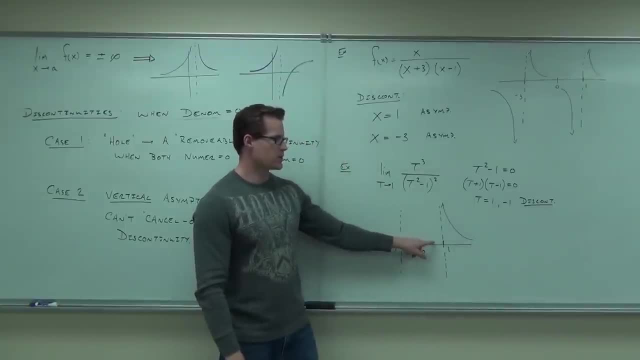 Up Really Positive number. 0.5 is a positive number. You didn't check negative, did you? Because we should be checking between this little interval. That's why we have that interval. Yeah, yeah, yeah positive. 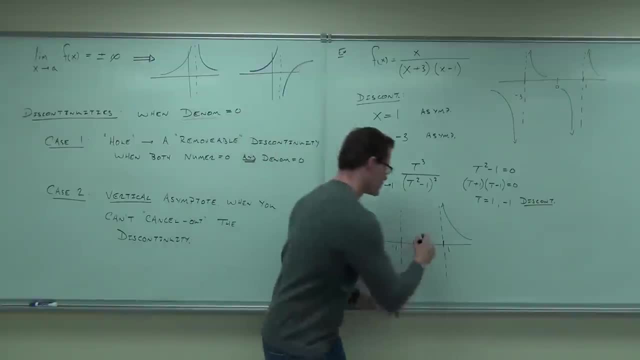 0.5 is positive. this is positive. positive over positive, positive Positive, Positive over positive. Aha aha, We did this the first time. I think we've had one of these. Does the limit exist? Yes, 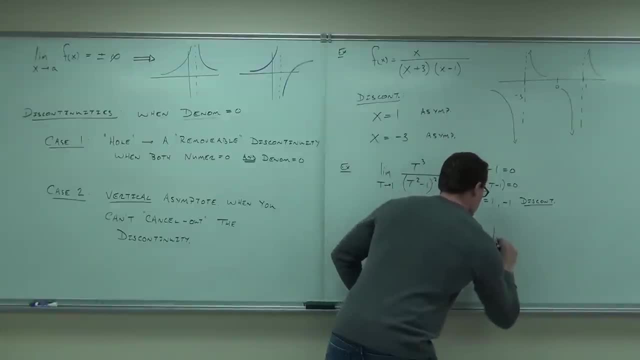 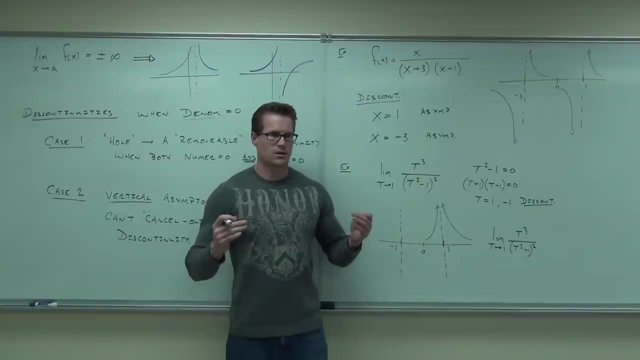 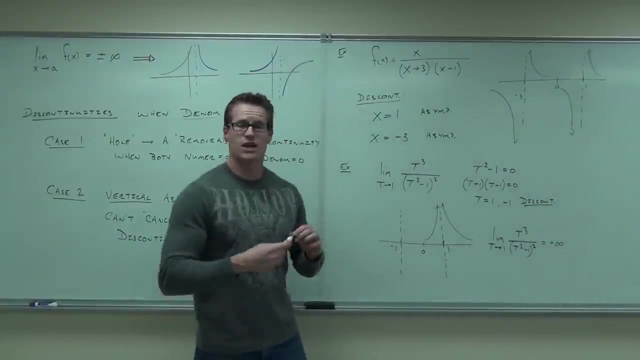 Yes, it does. This limit as t approaches. one of that nasty-looking function is: what can you tell me? Positive or negative, Positive or negative, Positive or negative? So are sine analyses important? Are sine? is that a sound, an alici? 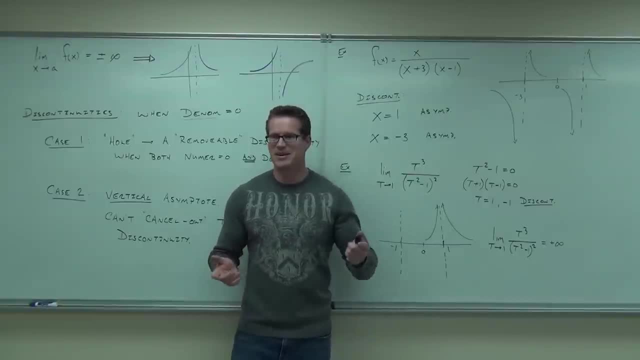 How do you say that Analysis is Analyses? Analyses, oh, that's better. Are sine analyses important for you? Are they important? Yeah, you gotta know how to do those. So when you can cross out, it's very easy. 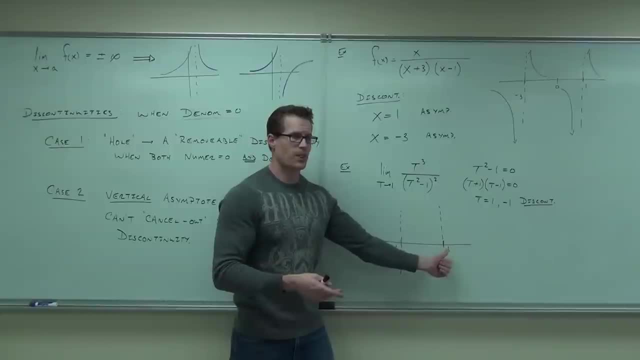 Then it says one. so I don't care about that, I care about this. Sure, Tell me one more point that I absolutely must have up here right now: Zero, That's zero. That zero could be a change of sign. So where the numerator equals zero, 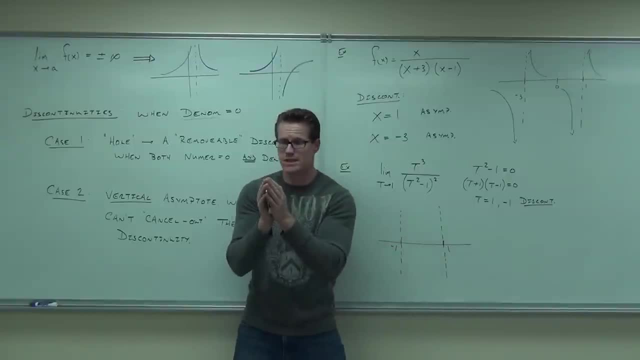 that could also be a place where you want to at least separate your interval. It's not going to be an asymptote, But you definitely want to plug in, just to be safe, a number between zero and one. That's what you want to do. 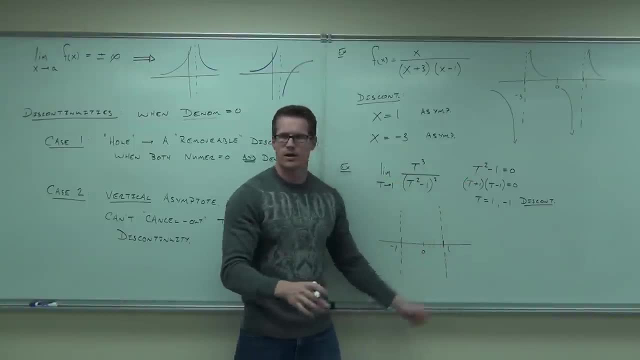 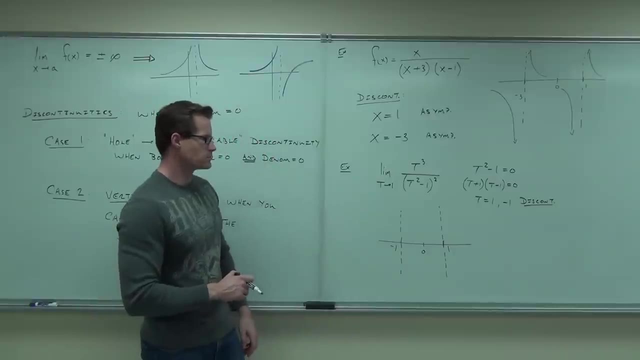 So try that. People on the left-hand side, why don't you try 0.5?? Right-hand side, why don't you try 2?? Try 2 for me. See what happens around. that Shouldn't really be able to do it without a calculator. honestly. 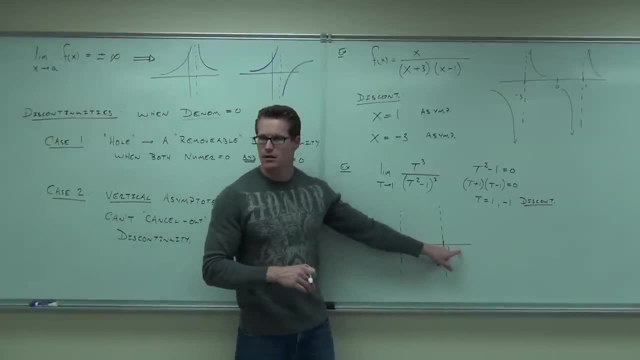 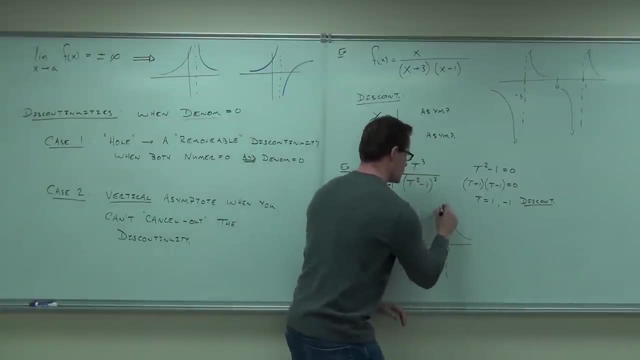 Because, when you think about it, this is going to be a positive number, right? Positive, it doesn't matter, That's positive. Positive over positive is positive. Up 0.5 is negative. Really Positive number: 0.5 is a positive number. 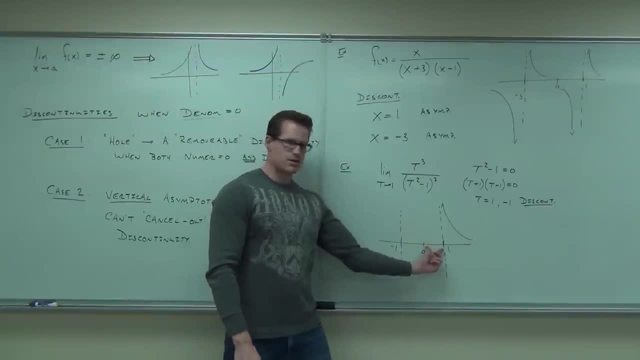 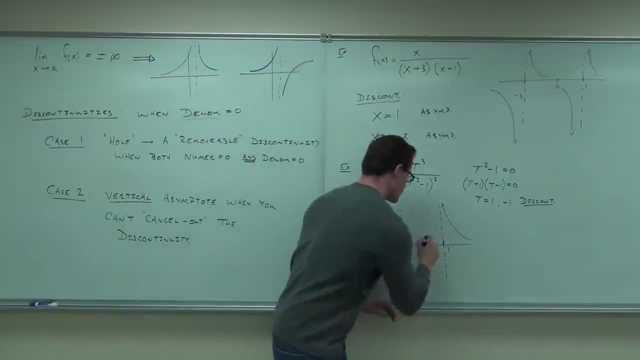 You didn't check negative, did you No? Because we should be checking between this little interval. That's why we have that 0.5 is positive. This is positive, Positive over positive, positive. I can't do it. 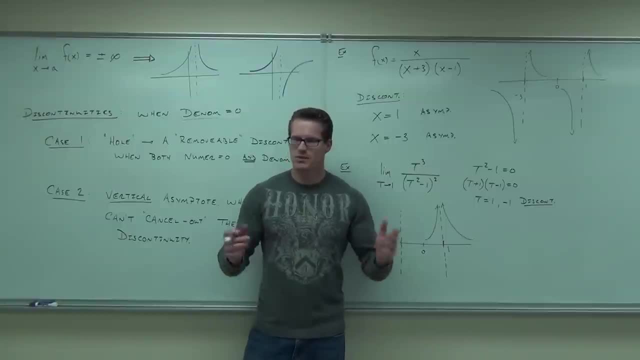 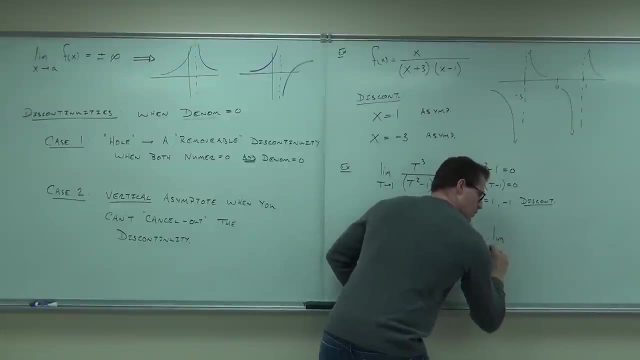 Aha, Aha. This is the first time, I think, we've had one of these. Does the limit exist? Yes, Yes, it does. This limit as t approaches 1.. So the limit of that nasty looking function is what? 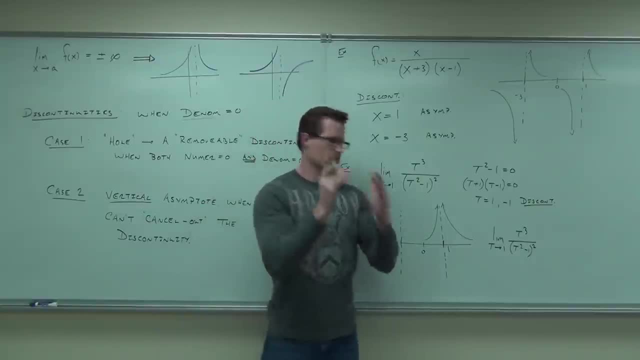 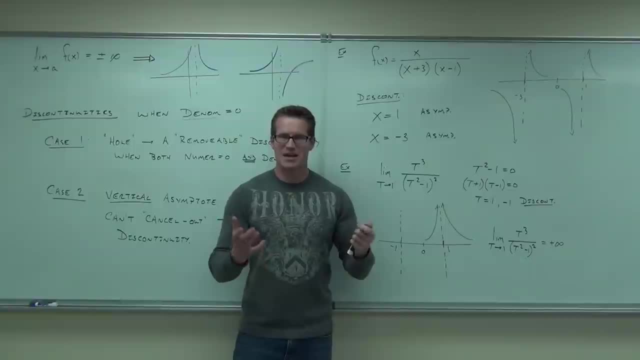 Analysis is Analyses, Analyses- Oh, that's better. Are sine analyses important for you? Are they important? Yeah, You've got to know how to do that. You've got to know how to do those. So when you can cross out, it's very easy. 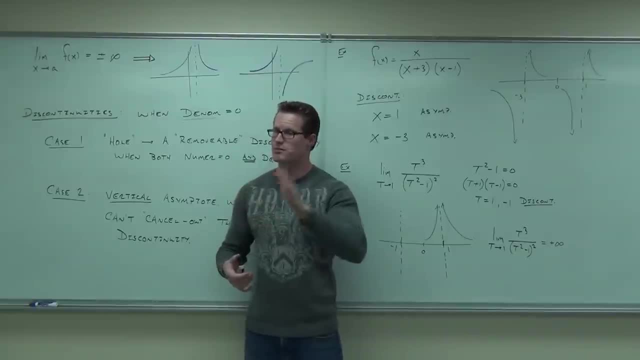 those are holes, no problem. When you can't cross them out, you have to have some way to determine where they're going. And the way you do that is with a sine analysis, just like that. Don't worry about all the ask-and-quotes. 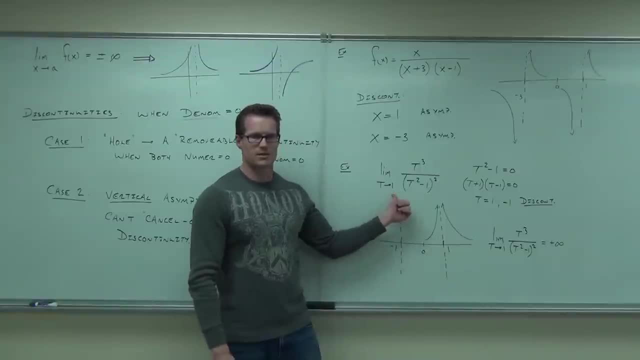 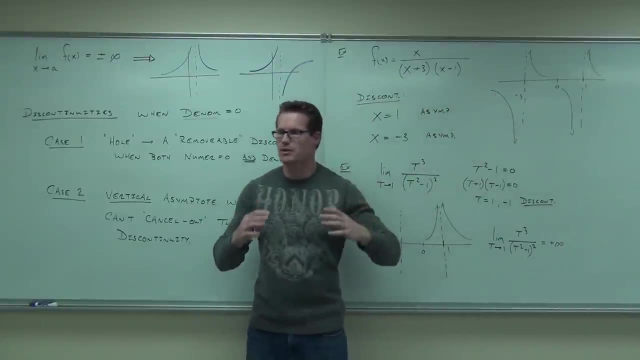 if I don't ask them for you. Worry about just where the limit says. If I'm asking for all the discontinuities, I'm just asking for the points, right? This was a little extra for us in that case. just wanted to see what happened. 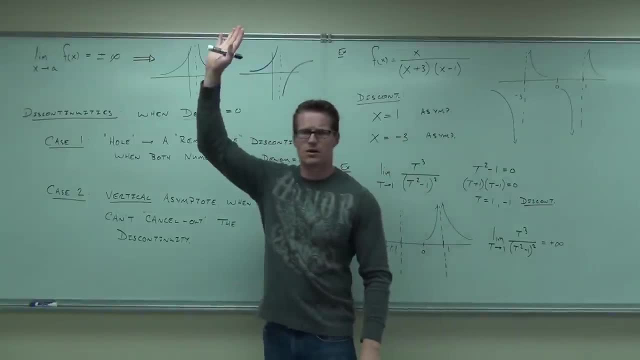 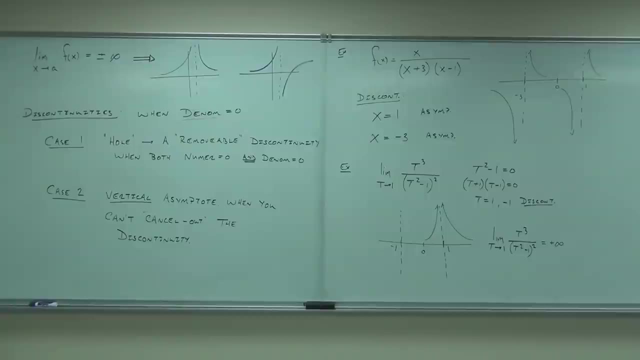 This is the application for a limit Question. I feel okay with this so far, All right, good. Now the next question we have to answer is what happens with a limit if x doesn't actually go to a number. So, for instance, x goes to one here, right? 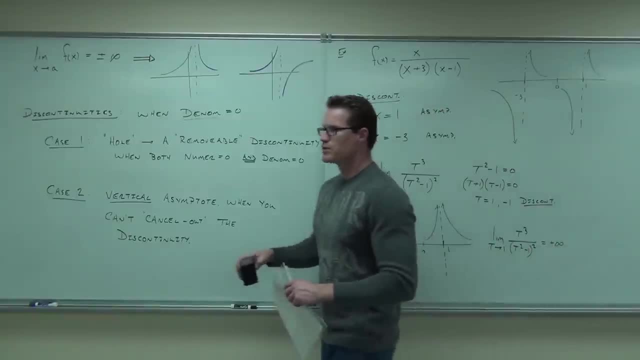 Or t. in this case, a variable goes to one. What if we say: I don't want to go to one, I don't want to go to two, I want to go to infinity. What happens to our function? I don't want to go to negative three. 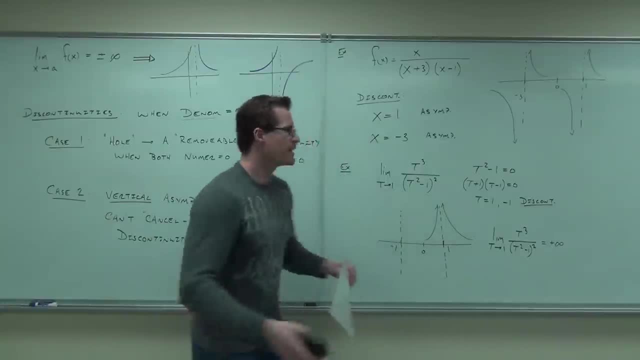 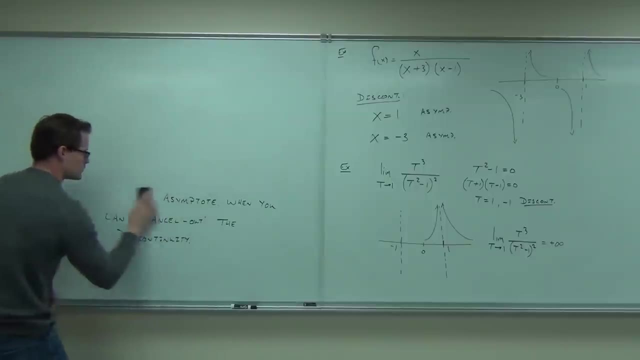 I don't want to go to negative four. I want to go to negative infinity. What happens to our function? That's what this next part of the question is. That's what this part is all about. It's all messed up. So the question is: what happens in a limit or to a function? 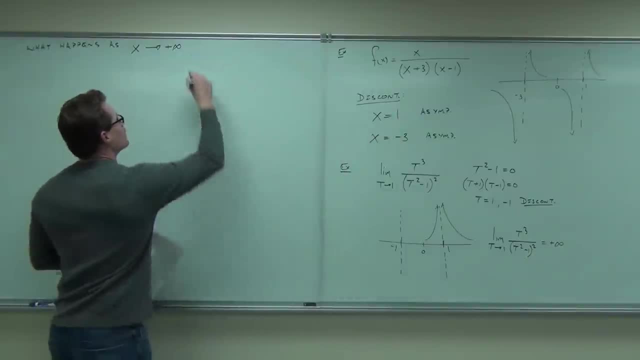 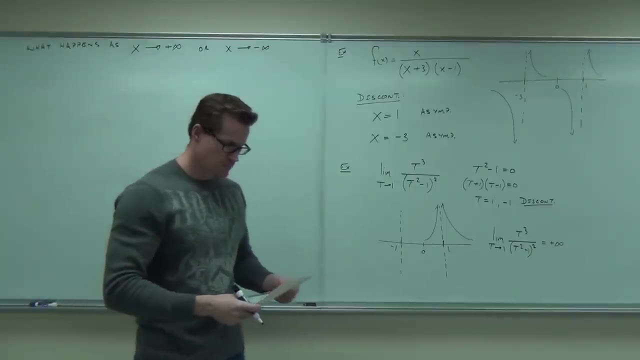 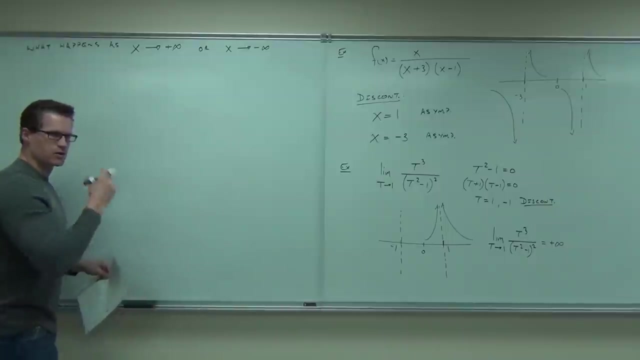 As x approaches positive infinity, as far as we can go, right, As x approaches positive infinity, as far as we can go, or negative infinity. Basically, x increases forever or decreases forever. What happens to our function? Let's take a look at two examples that are going. 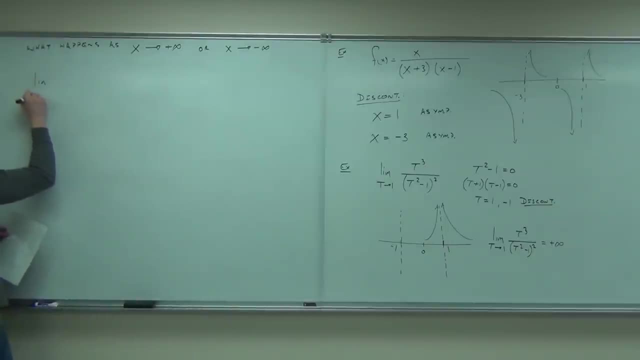 to give us insight as to this. Let's take one example. Let's take a look at a table. Here you have an x minus a, minus a, and let's say that x is positive infinity. So we have a x plus a minus a, which is negative infinity. 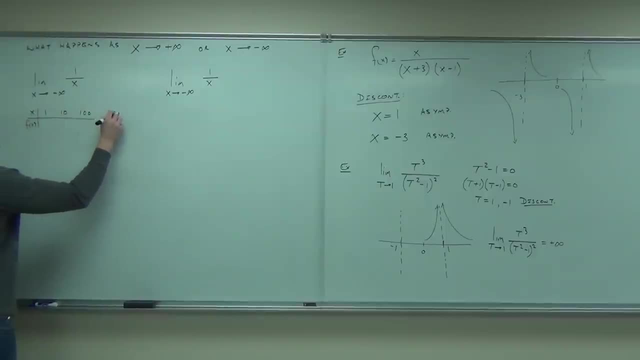 So we know that x is positive infinity, So we don't have to figure out how many. What's the и? Well, it's not. Let's make a table, We'll see what we find. What's the y? What's the z? 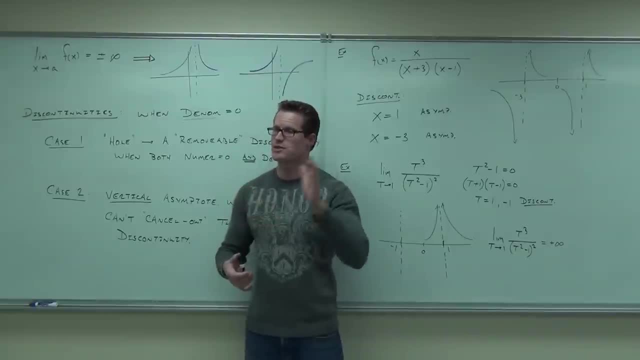 Those are holes, No problem. When you can't cross them out, you have to have some way to determine where they're going. And the way you do that is with a sine analysis, just like that. Don't worry about all the asymptotes. 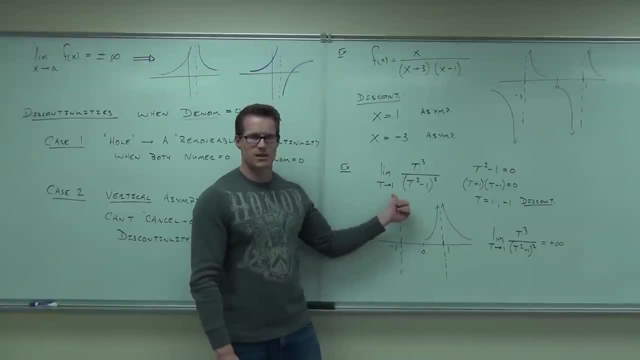 if I don't ask them for you. Worry about just where the limit says. If I'm asking for all the discontinuities, I'm just asking for the points. This was a little extra for us in that case. I just wanted to see what happened. 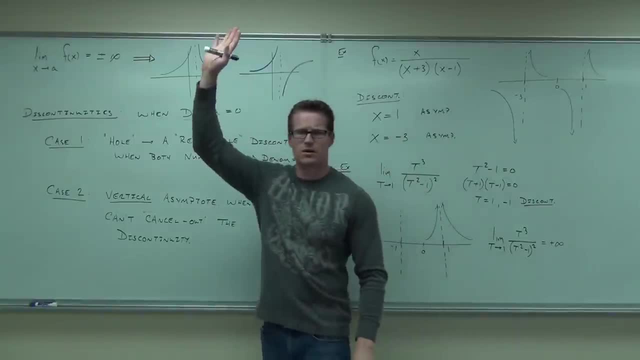 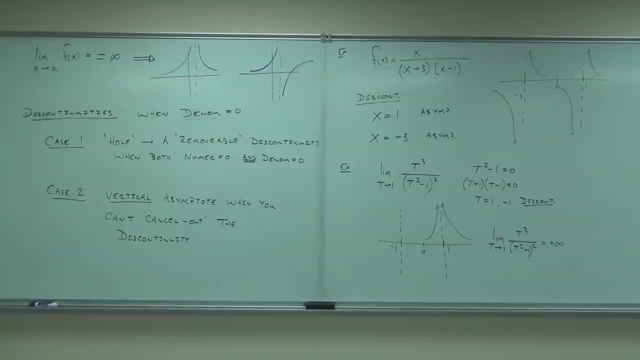 This is the application for a limit Question. I feel OK with this so far, All right, good. Now the next question we have to answer is what happens with a limit if x doesn't actually go to a number. So, for instance, x goes to 1 here, right? 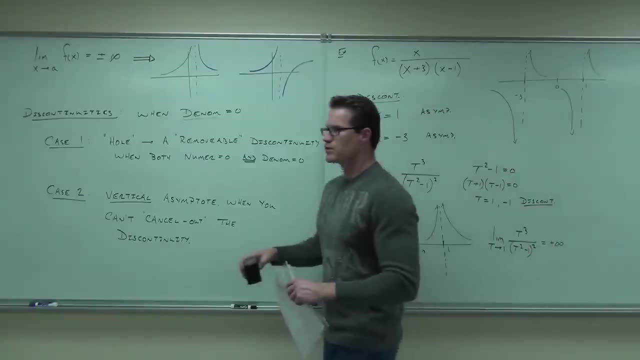 Or t. in this case, A variable goes to 1. What if we say: I don't want to go to 1.. I don't want to go to 2.. I want to go to infinity. What happens to our function? 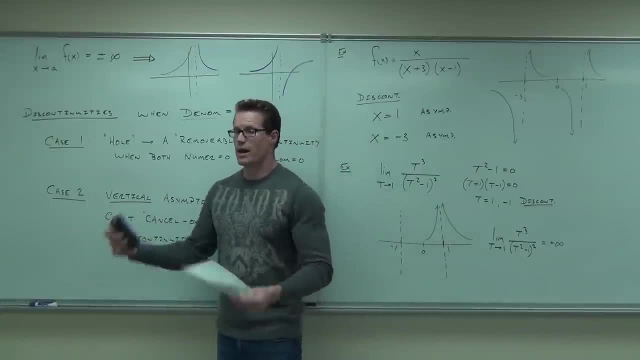 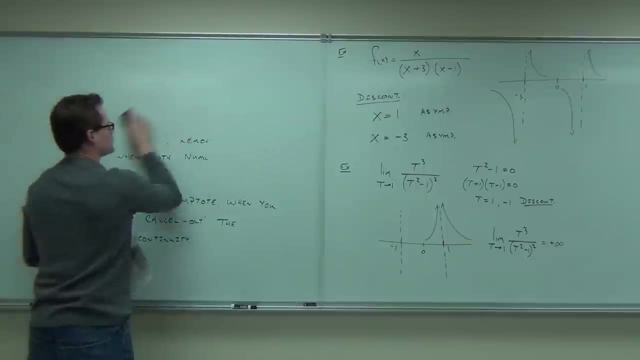 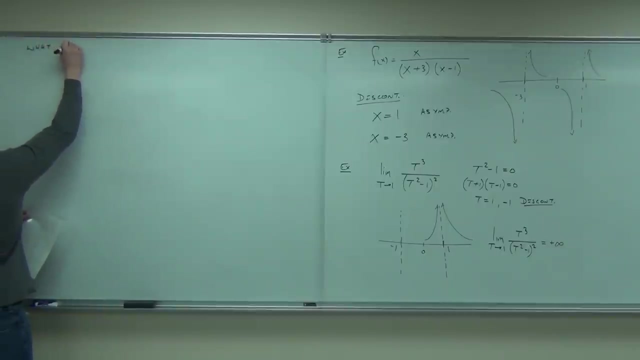 I don't want to go to negative 3. I don't want to go to negative 4. I want to go to negative infinity. What happens to our function? That's what this next part is all about. So the question is: what happens in a limit or to a function? 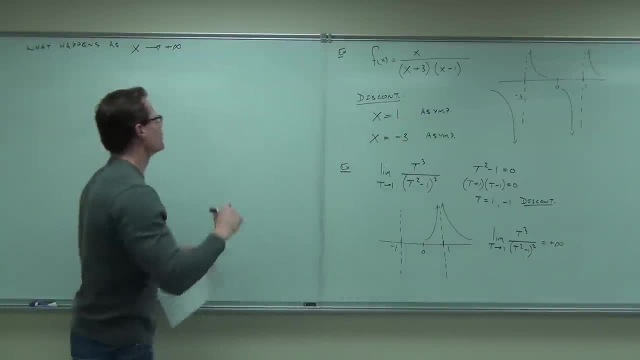 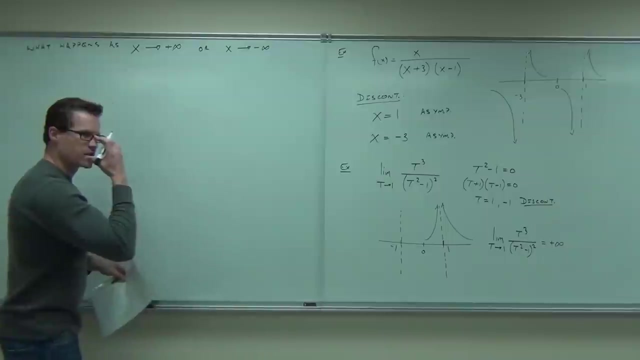 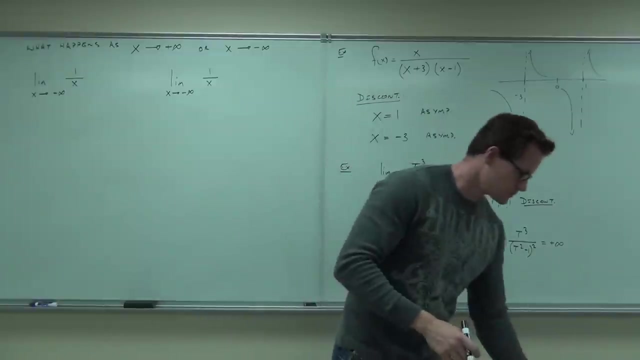 as x approaches positive infinity- As far as we can go- or negative infinity. Basically, x increases forever or decreases forever. What happens to our function? Let's take a look at two examples that are going to give us insight as to this. You know what? 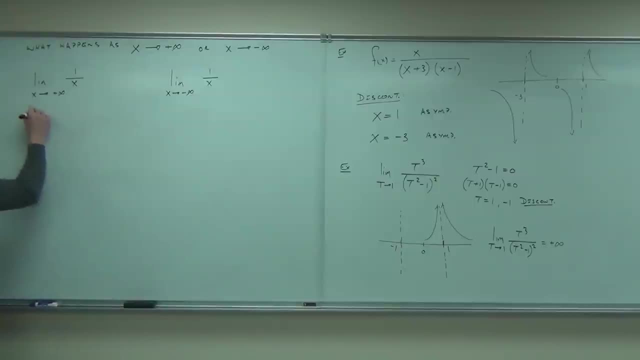 just to kind of get a picture of what's going on. We'll have x and f of x. We'll start very easily. We'll start at one, ten, a hundred and then a million. Let's do it for this one. 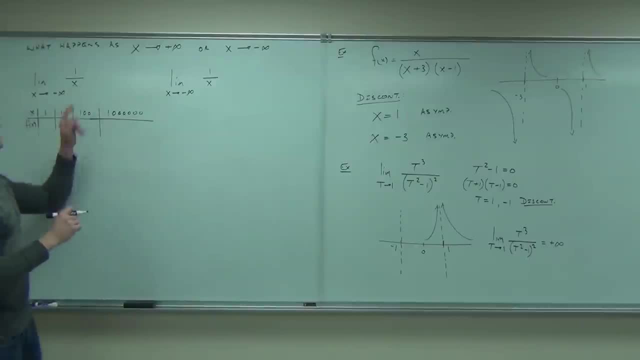 Let's see what we find. Let's make a table. Let's do it for this one. What would happen, please, if x equal to 1, what would we get? 1.. How about if x equal to 10,? what would we get? 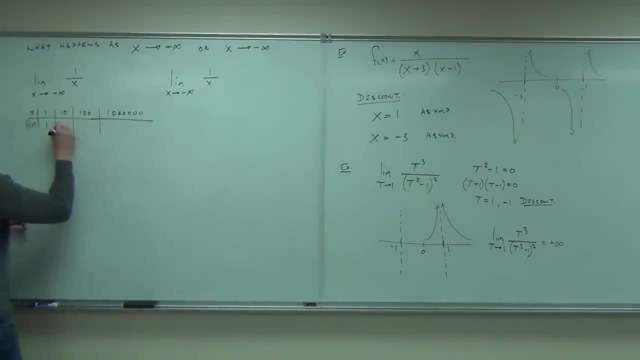 0.1.. 0.1.. Very good. Or 110.. Yeah, clearly right. 1 over whatever that number is. How about 100? 0.01.. 0.01.. How about a million? 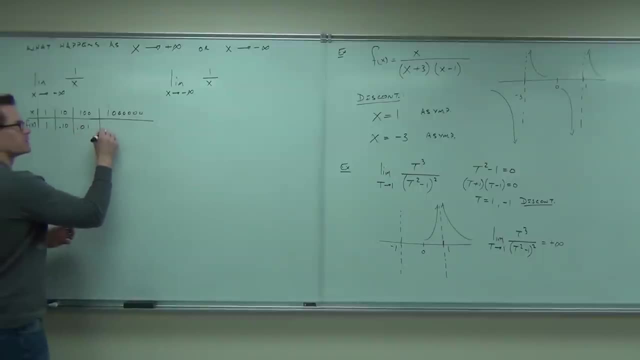 0.501.. 0.501.. 0.501.. 6 zeros, right, 5 zeros. 5 zeros, Yeah, 5 zeros. What if x equaled a trillion? would it get bigger or smaller, Smaller? 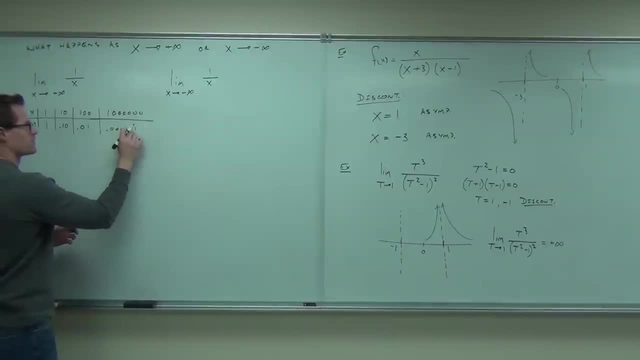 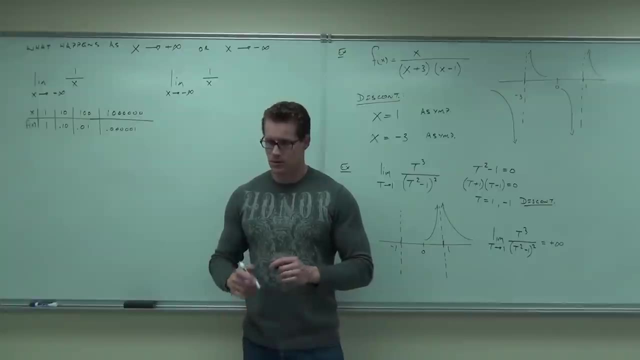 What's it going to Zero? Is it ever going to reach zero? No, But think about this: You're dividing a constant number by infinity. What's it going to do? Zero, Zero, Zero, Zero, Zero, Zero. 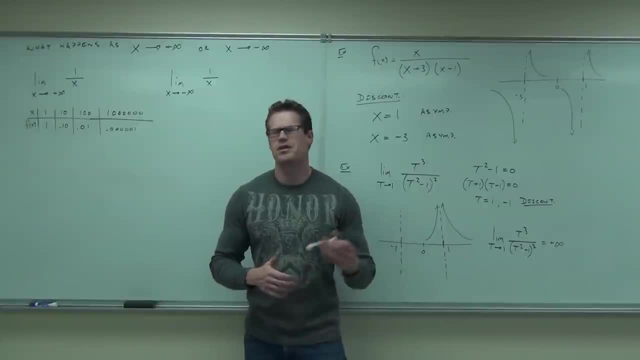 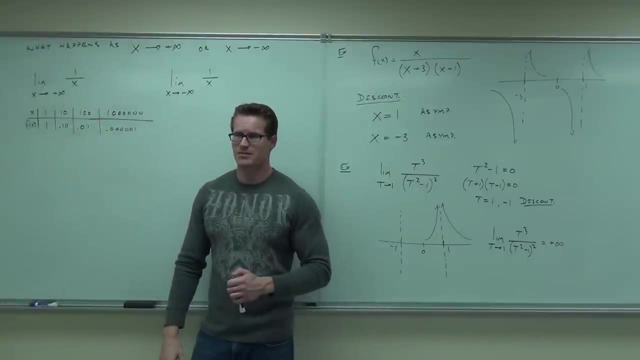 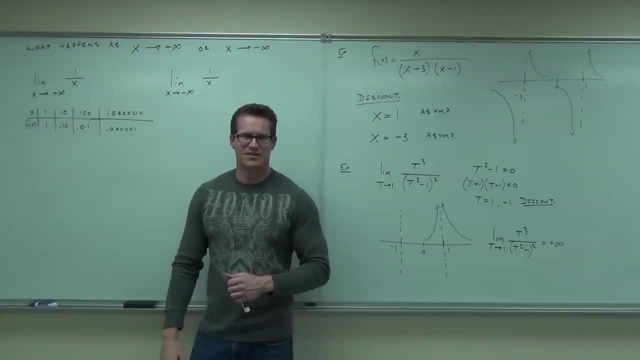 You're wrong plus 10.. Well, you're wrong times infinity. Ha ha, ha, ha ha ha, Right. Well, if you did divided by infinity, you'd have- like you'd have- zero. You keep dividing it by a bigger and bigger number, you're going to get zero. 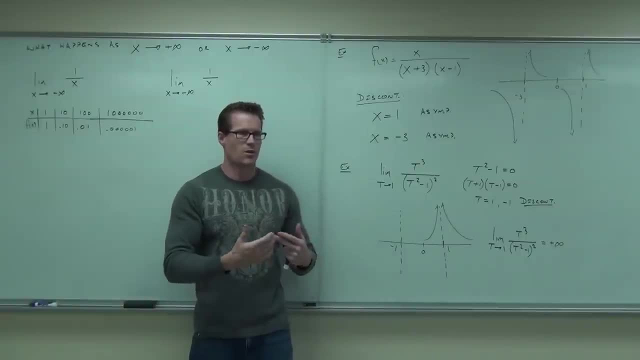 Right. One divided by a billion is very close to zero. One divided by a zillion- and you have to take number like a number- is very close to zero. But you keep getting bigger and bigger. This quantity is closer and closer to zero. 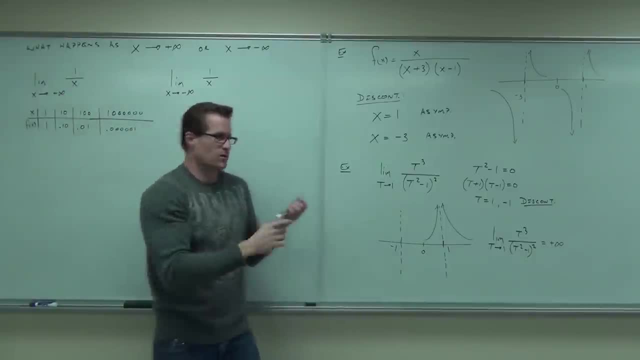 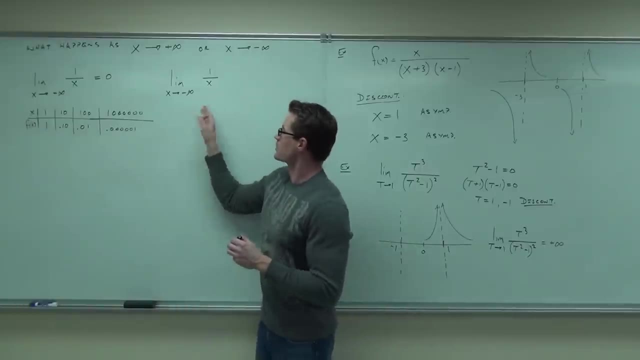 zero. Are you with me on that Zero? Let's look at negative infinity. What happens as you go closer to negative infinity? Well, that would be- I'm just going to change this. that would be negative, negative, negative, negative, True, Negative, negative, negative. 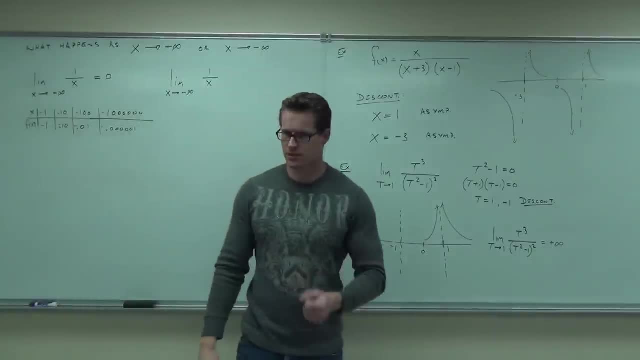 negative. Is it still approaching zero? Yes, As we go to negative infinity, we're also approaching zero. What this says is that if f of x, our function, gets really, really close to a number as we approach infinity, then the limit exists, So we can take limits. 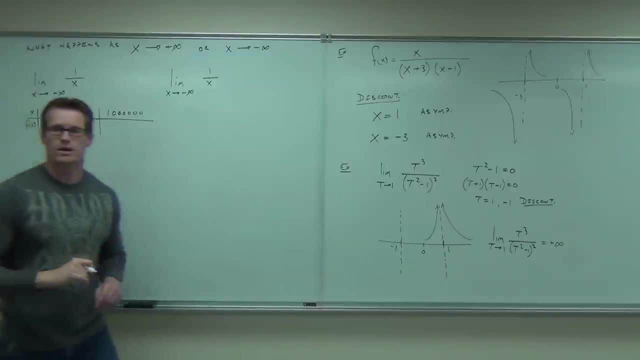 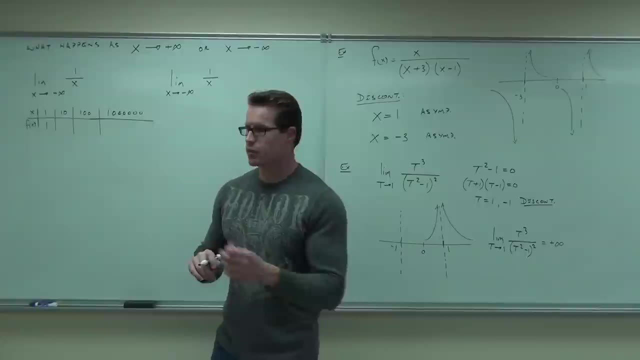 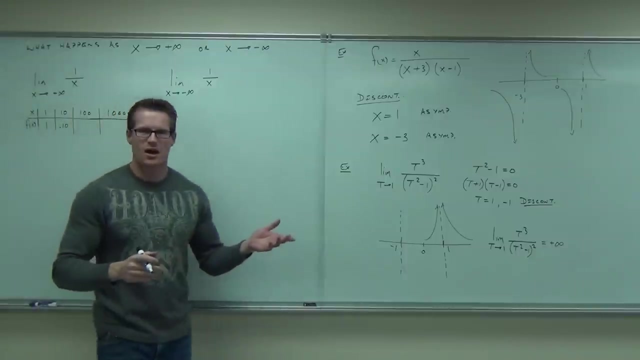 What would happen, please, if x equal to one? What would we get One? How about x equal to ten? what would we get? Point one, okay, Point one, very good. or one-tenth, Yeah, clearly right. one over whatever that number is. 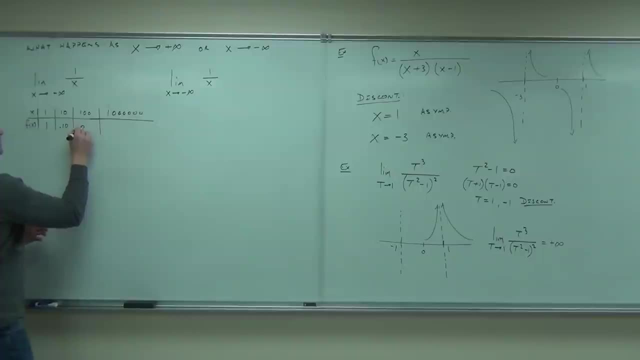 How about a hundred Point zero one Point zero one. How about a million Point five zero zero one? Six zeroes, right, Five zeroes, Five zeroes, Yeah, five zeroes. What if x equaled a trillion? would it get bigger or smaller? 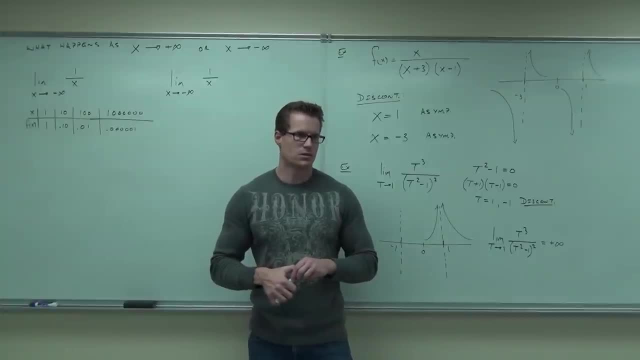 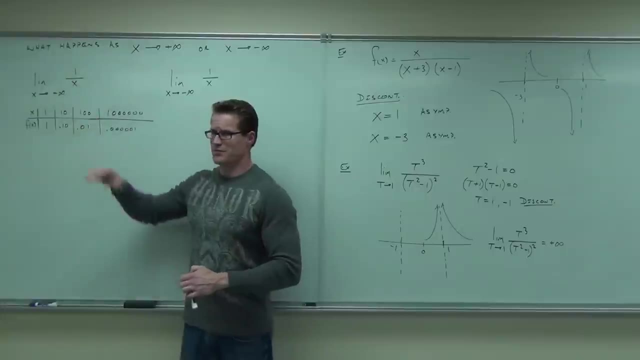 Smaller, Smaller. What's it going to? Zero? Zero? Is it ever going to reach zero? Never. But think about this: You're dividing a constant number by infinity right Like when you're a little kid and you go. you're wrong. 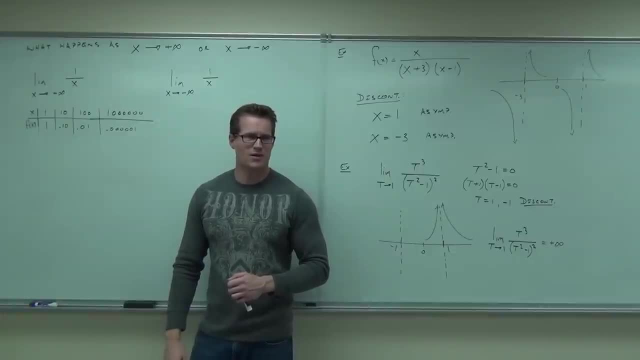 Well, you're more wrong. Well, you're wrong. plus ten. Well, you're wrong times: infinity. Ha, ha, ha, ha, ha, Right. Well, if you did divide it by infinity, you'd have like ten. 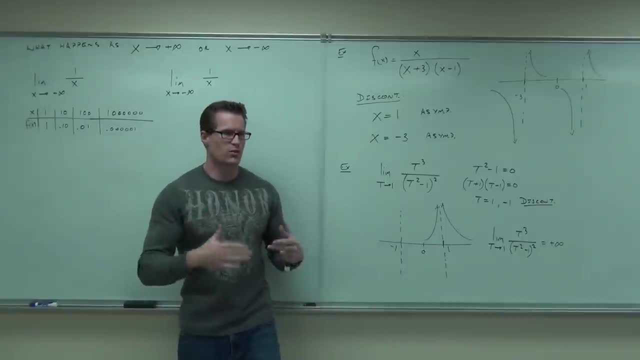 Right, You'd have zero. You keep dividing it by a bigger and bigger number. you're going to get zero, Right? One divided by a billion is very close to zero. One divided by a zillion is very close to zero, But you keep getting bigger and bigger. this quantity is closer and closer to zero. 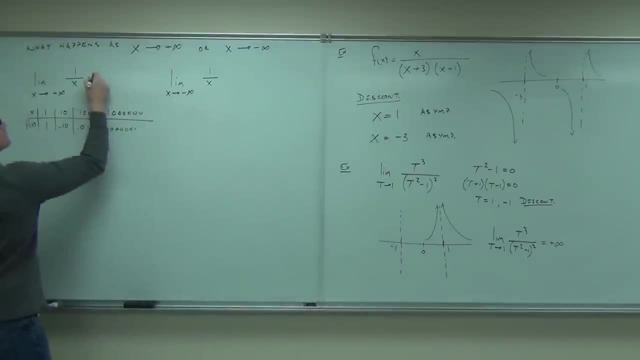 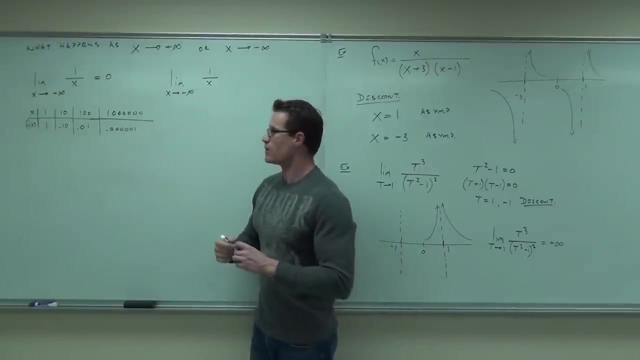 Are you with me on that Zero? Let's look at negative infinity. What happens as you go closer to negative infinity? Well, that would be. I'm just going to change this. That would be negative, negative, negative, negative. 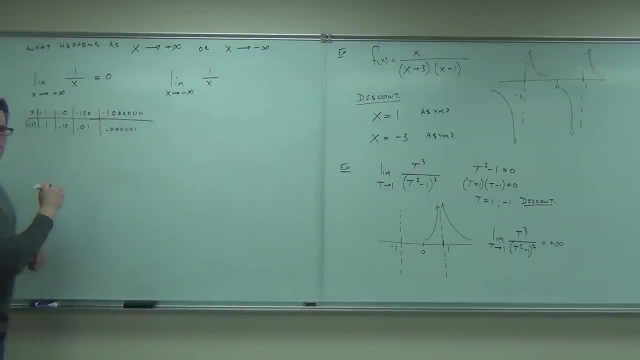 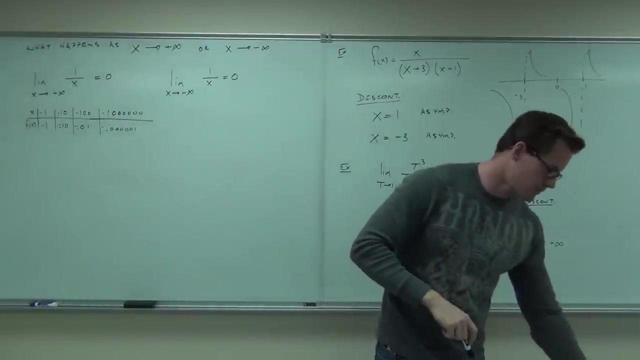 True, Negative, negative, negative, negative. Is it still approaching zero? Zero, Yes, As we go to negative infinity, we're also approaching zero. What this says is that if f of x, our function, gets really, really close to a number, as we 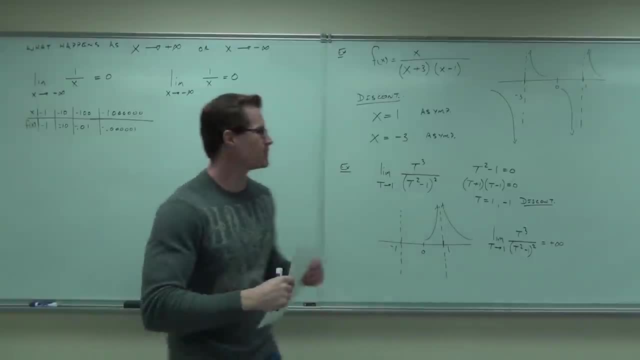 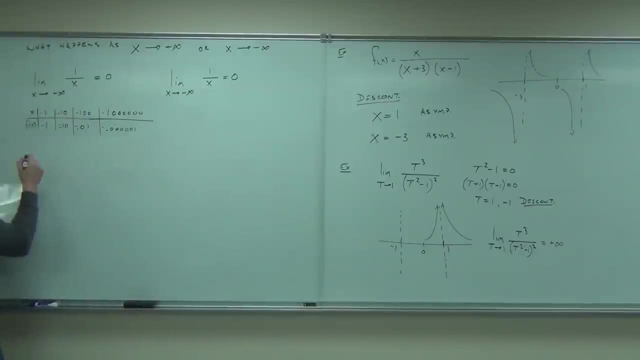 approach infinity, then the limit exists. So we can take limits as x approaches one of these infinities. if x approaches an actual number- Remember that idea of really close to, That was the idea of that limit- If f of x gets really close to a number, 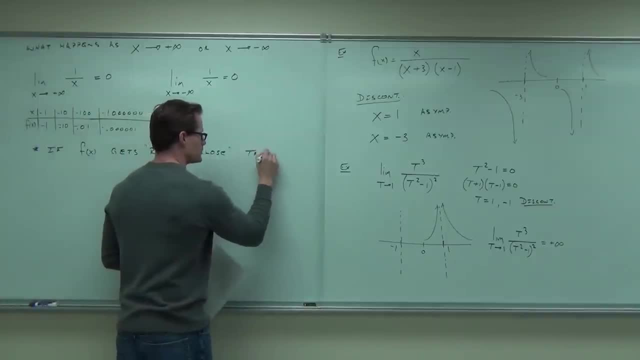 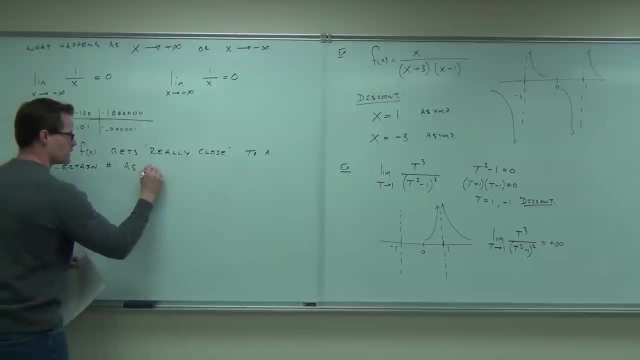 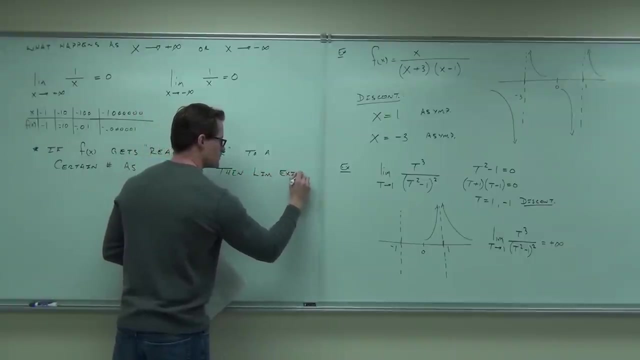 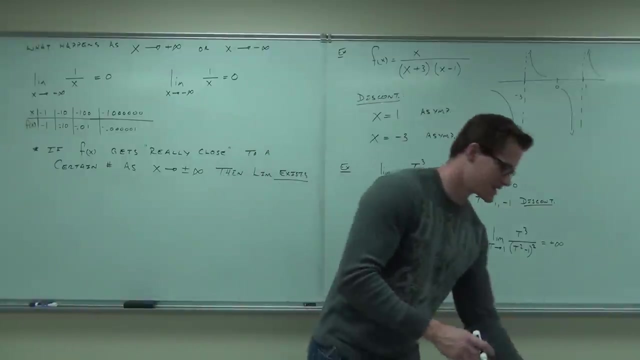 What's the limit? Zero, Zero, Zero, Zero, Zero, Zero. As x approaches infinity- plus or minus, whichever one- then the limit exists, Okay. well, if the limit exists, what's it stand for? What's it mean? Think about this. 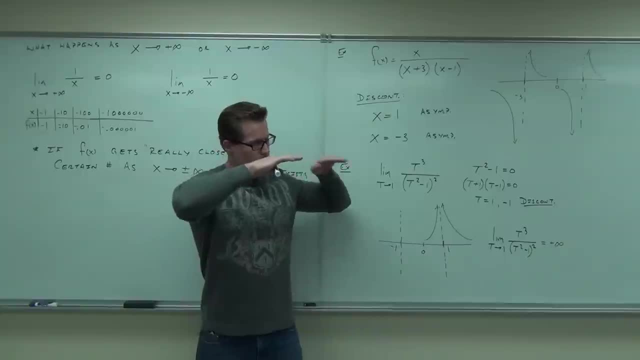 Let's say that you start taking your function and you start going forever in that direction. Well, it's almost like a karate move. I've never taken karate, I don't know, but it kind of feels like it, Whatever The limit move. 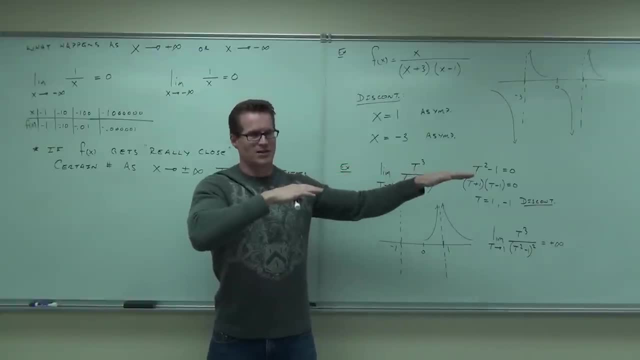 So, by the way, if you ever try to do the math karate, you're going to beat up. Never do math karate. So you go this way forever and ever and ever, and your function is going to the same number. 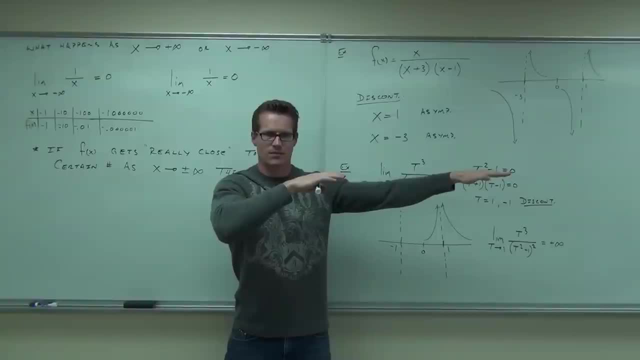 Is it ever going to get to that number? No, Let's get very, very, very, very close, right? What idea do we have? What idea do we have that represents that, But not a vertical one. A vertical one says: you're getting really close to that, right. 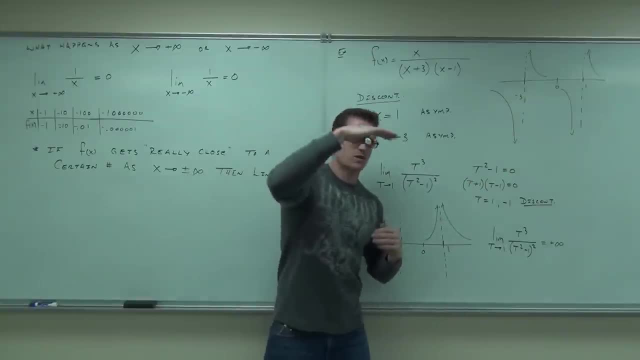 You'll never reach it. That's the same idea. we have going this way, Really close to that. but we don't have this idea. We only have one, because otherwise we don't have a function. But we have this idea: We're going to get close to a number or close to a number, close to a number or close to a number. 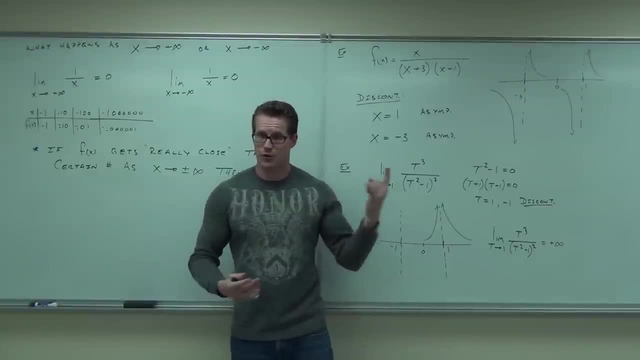 That's a horizontal asymptote. So now we have two types of asymptotes. Vertical happens when you have discontinuities that are not real and full. Shake your head or nod your head if you're okay with that. Horizontal happens when you take a limit of your function to infinity. 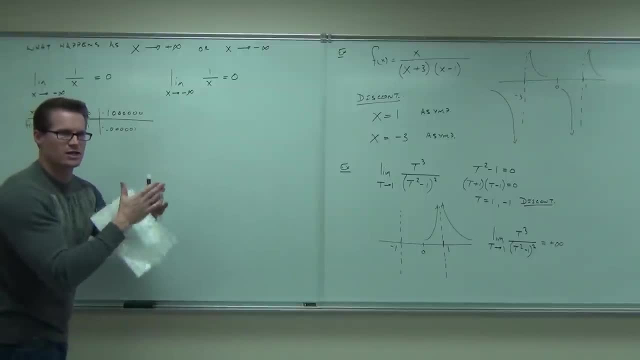 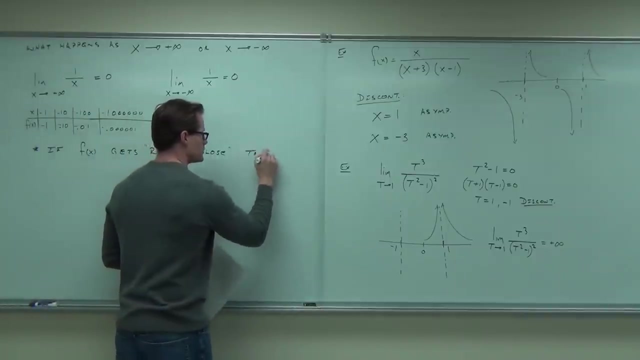 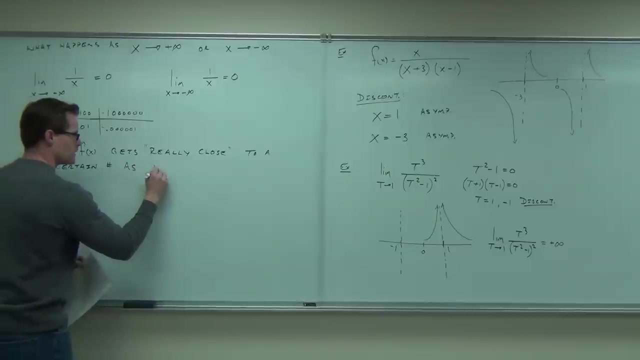 as x approaches one of these infinities. if x approaches an actual number- Remember that idea of really close to, That was the idea of that limit- If f of x gets really close to a number, as x approaches infinity, plus or minus, whichever one, then the limit. 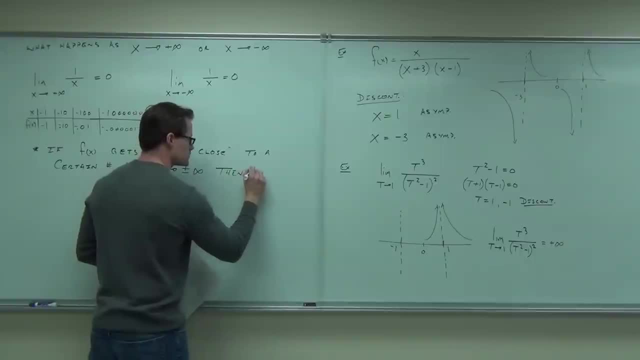 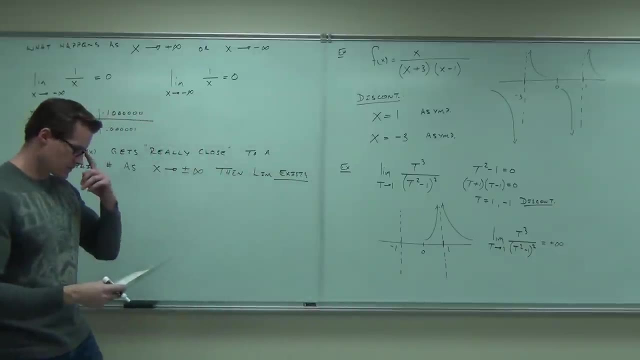 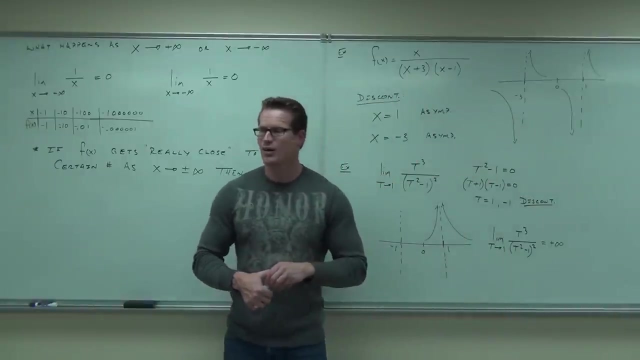 exists? OK. Well, if the limit exists, what's it stand for? What's it mean? Think about this. Let's say that you start taking your function and you start going forever in that direction. It's almost like a karate move. I've never taken karate, I don't know, but it kind of. 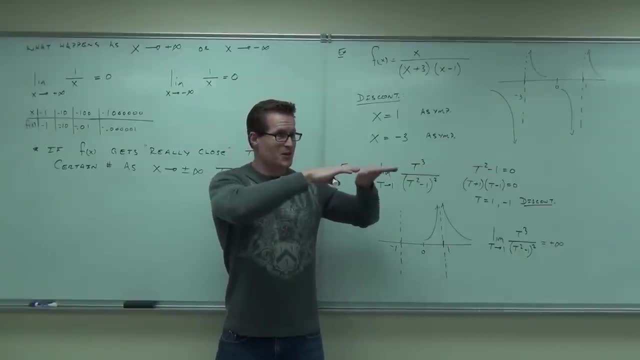 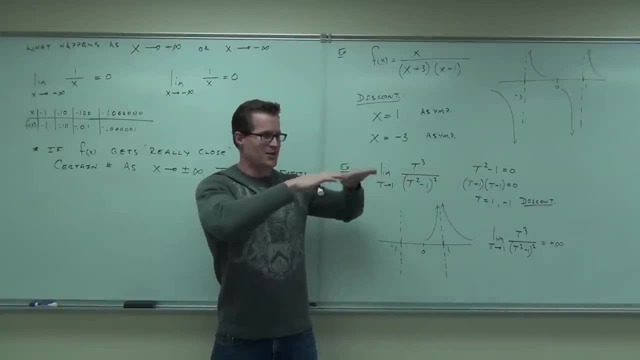 If you ever try to do the math karate, you're going to get your feet, You're going to beat out. You'll never be a math karate. So you go this way forever and ever and ever, and your function is going to the same number. 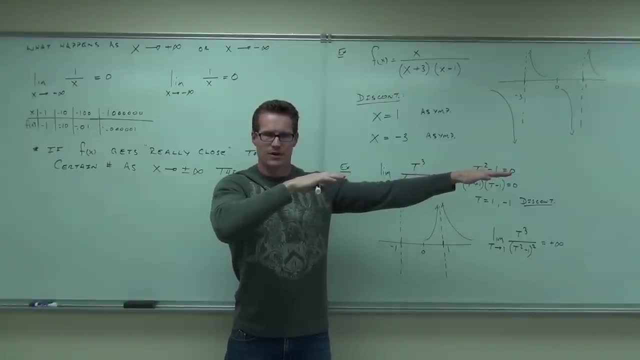 Is it ever going to get to that number? Never. It's going to get very, very, very, very, very close right. What idea do we have? that represents that Math, But not a vertical one. A vertical one says: you're going to get really close to that. 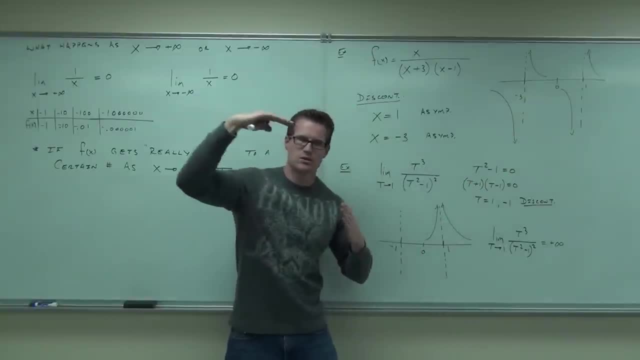 right, You'll never reach it. That's the same idea. we have going this way, Really close to that, but you're going. we don't have this idea. We only have one, because otherwise not a function. but we have this idea. 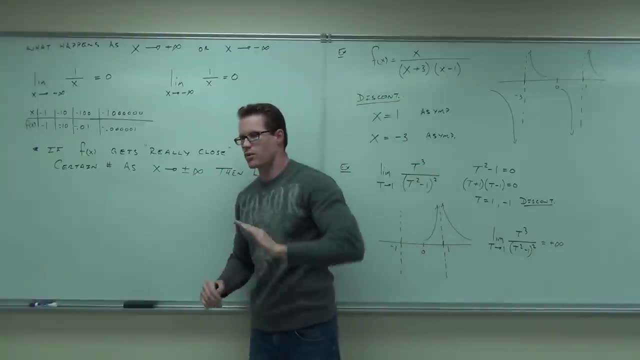 We're going to get close to a number or close to a number. close to a number or close to a number, That's a horizontal asymptote. So now we have two types of asymptotes. Vertical happens when you have discontinuities that are not roomful. 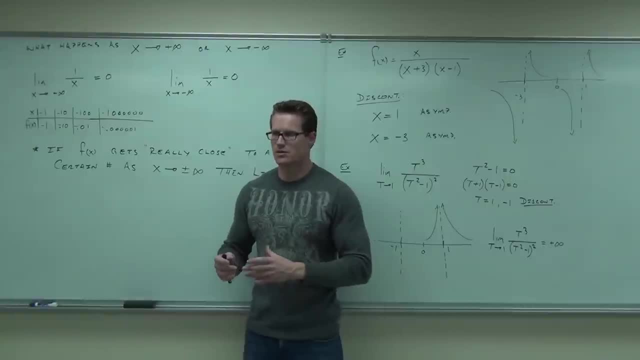 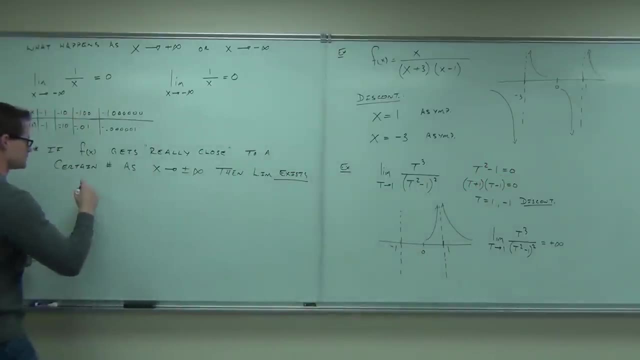 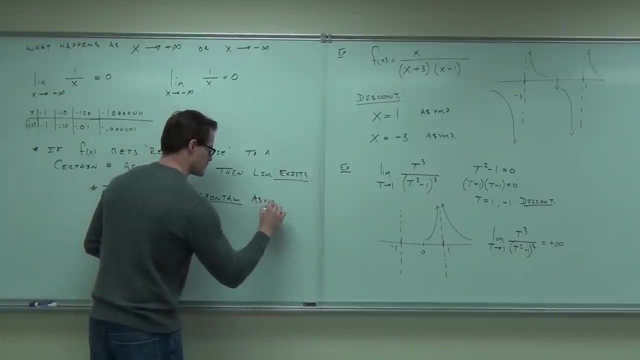 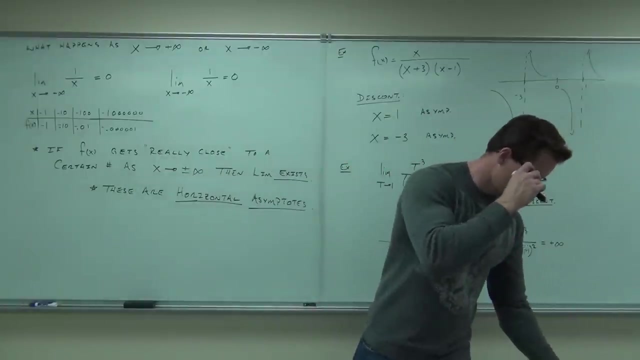 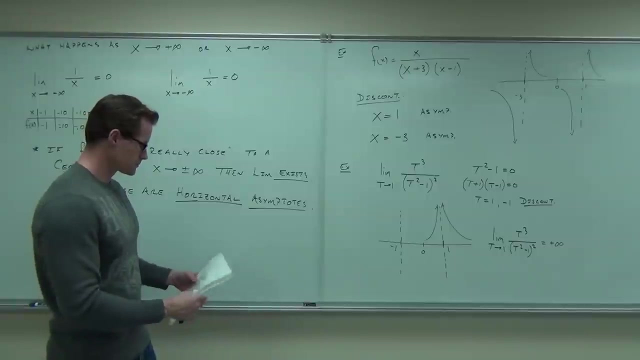 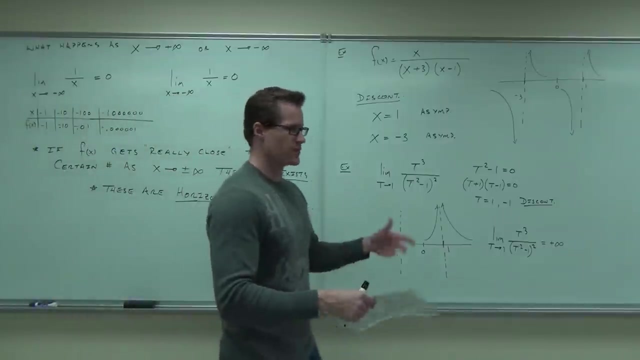 Shake your head or nod your head if you're okay with that. Horizontal happens when you take a limit of your function to infinity, and that's the idea: Horizontal asymptotes. By the way, the same rules apply to these limits we're about to do. 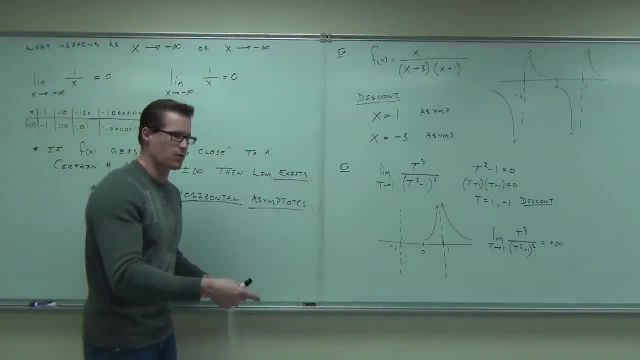 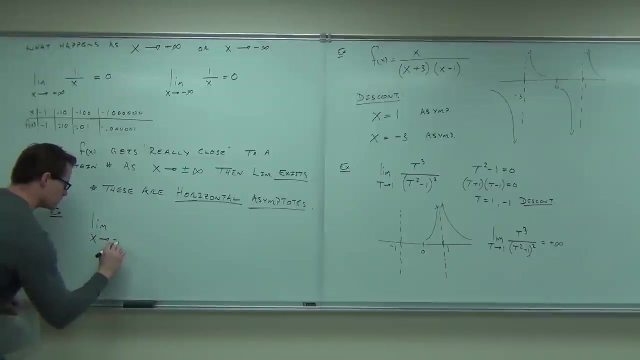 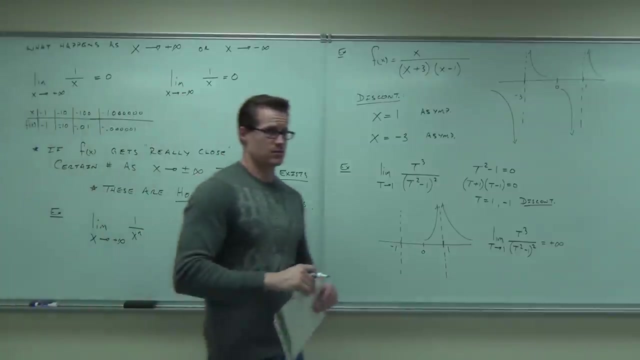 The rules for limits as x approaches negative and positive infinity are the same as before, So the same rules apply. Everything holds the same, which means one thing for us. Consider this: What if we take any any one over x to the n power? 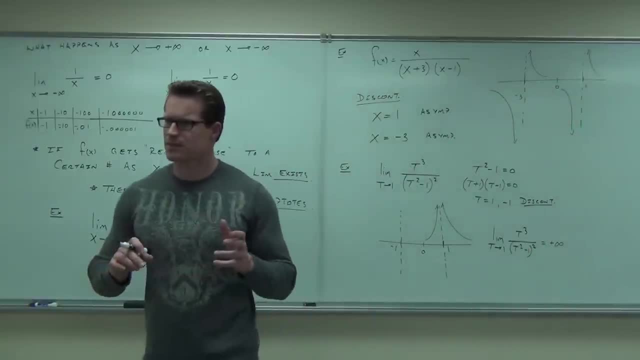 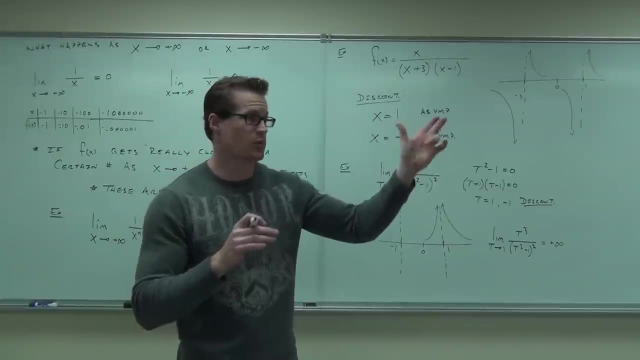 Do you recall from limits that I can take the limit of the function and then raise it to the power? Do you remember that that we could pull out the exponent? That was one of our prime rules. that helped us a lot. Well, notice how 1 to the n is always just going to be 1, right. 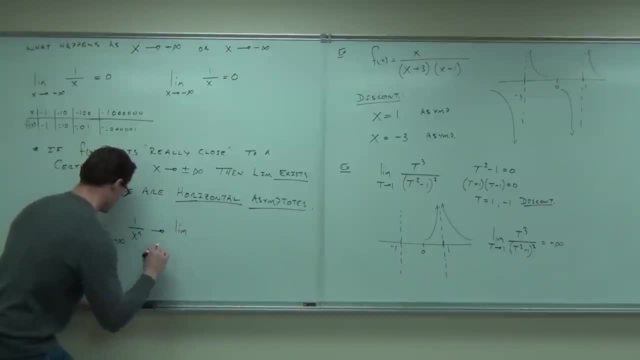 So then, this is true. That's a true statement. That's 1 over n. I'm sorry. 1 to the n, that's 1.. This is x to the n. That's x to the n. Are you guys OK with that statement? 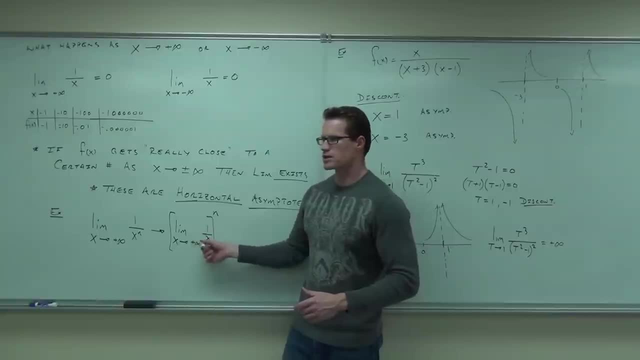 Well, tell me something then. How much is the limit of 1 over x as we approach infinity? What's 0 to the nth power? So what this says in English is that any function where you're dividing a constant 1, because you can pull a constant out. 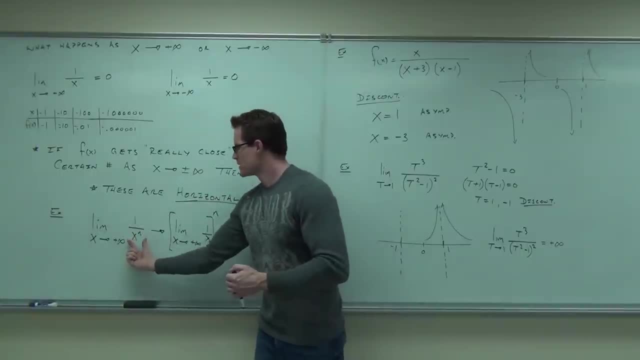 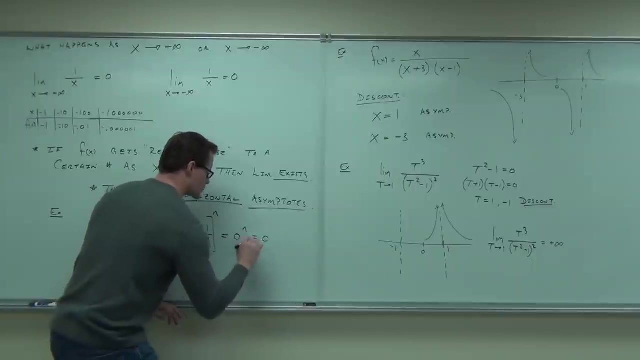 any constant can be pulled out of that limit. any constant by some variable that's being raised as x approaches to that infinity is going to end up being 0. It's going to have a horizontal asymptote at 0.. 0 to the n or 0. 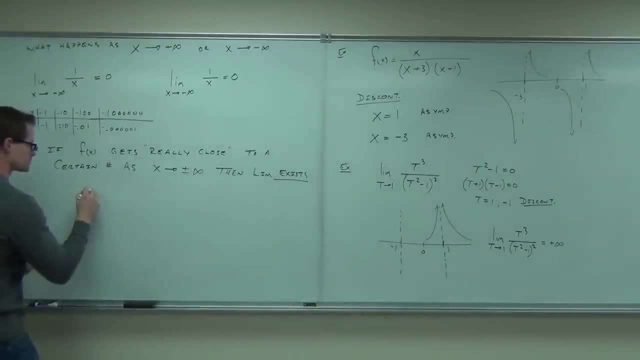 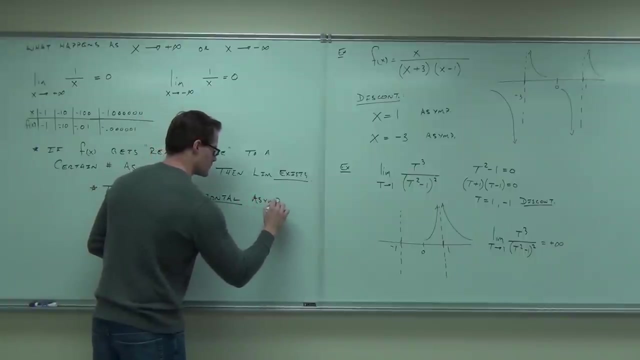 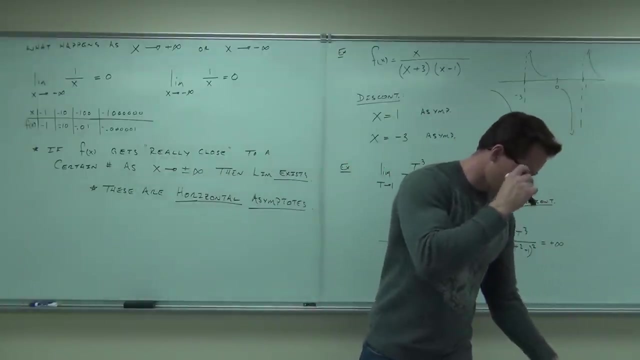 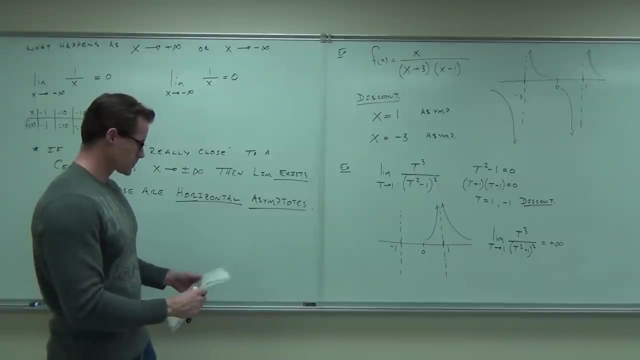 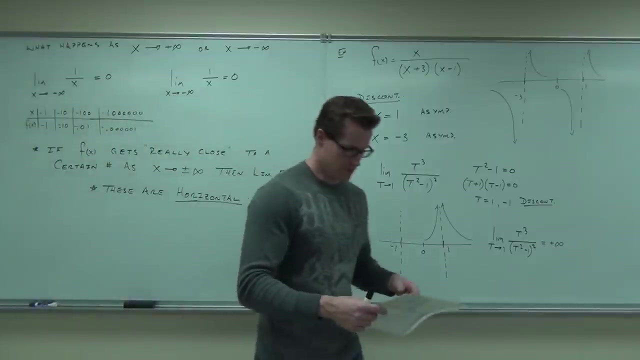 And that's the idea: Horizontal asymptotes. By the way, the same rules apply to these limits we're about to do. The rules for limits as x approaches negative and positive infinity are the same as before, So the same rules apply. 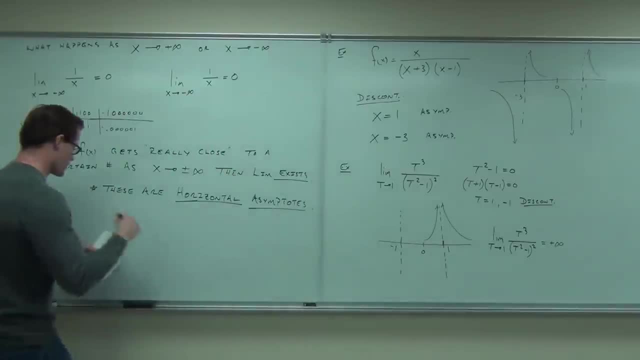 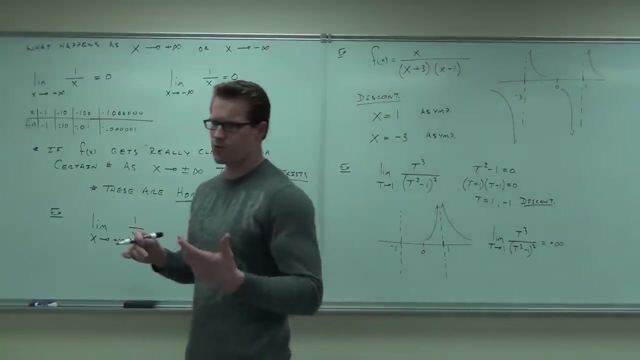 Everything holds the same, Which means one thing for us. Consider this: What if we take any any one over x to the n power? Do you recall from limits that I can take the limit of the function and then raise it to the power? 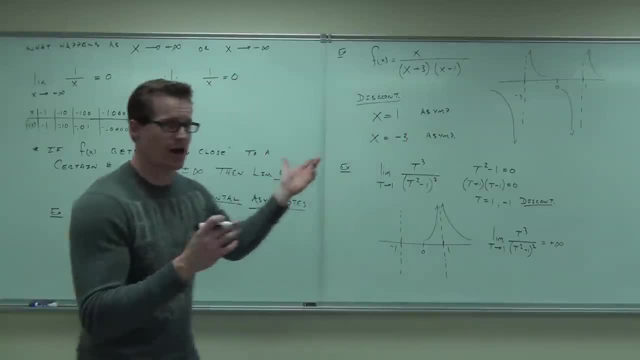 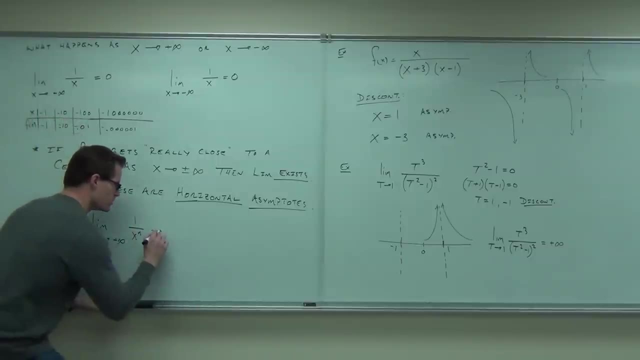 Do you remember that? That we could pull out the exponent? That was one of our prime rules. that helped us a lot. Well, Notice how one to the n is always just gonna be one, right? So then, this is true, That's a true statement. 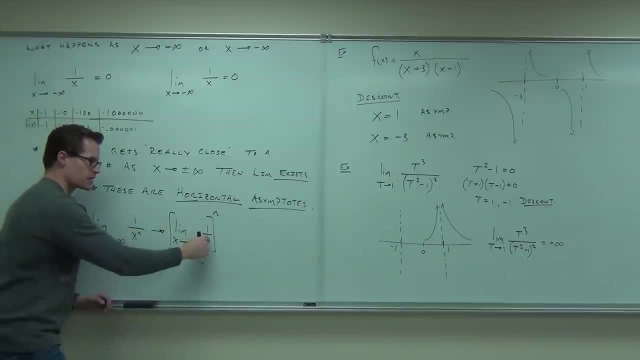 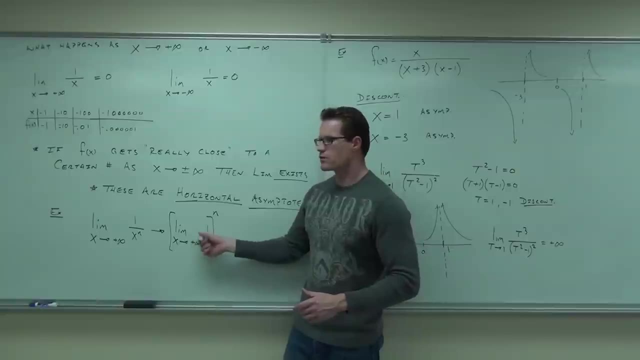 That's one over n. I'm sorry, one to the n, that's one. This is x to the n, That's x to the n. Are you guys okay with that statement? Well, tell me something then: How much is the limit of one over x? 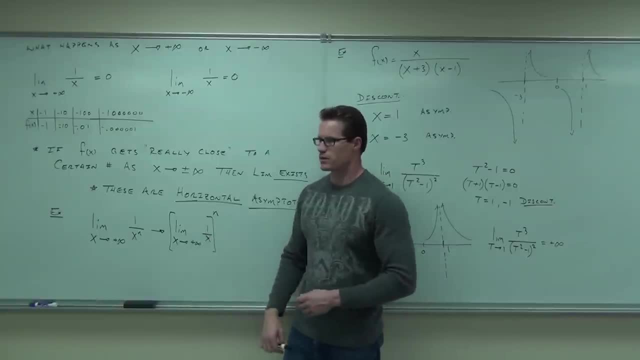 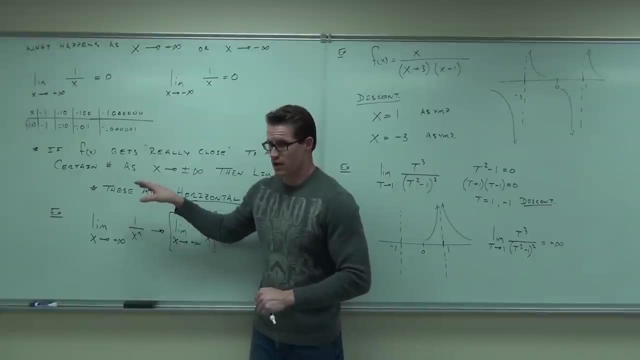 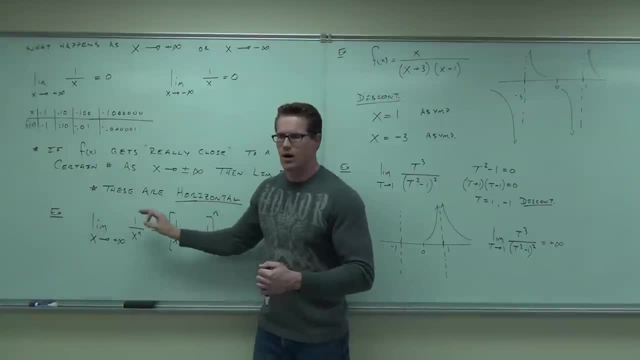 because you can pull a constant out. any constant can be pulled out of that limit. any constant by some variable that's being raised as x approaches to that infinity, is gonna end up being zero. It's gonna have a horizontal asymptote at zero. 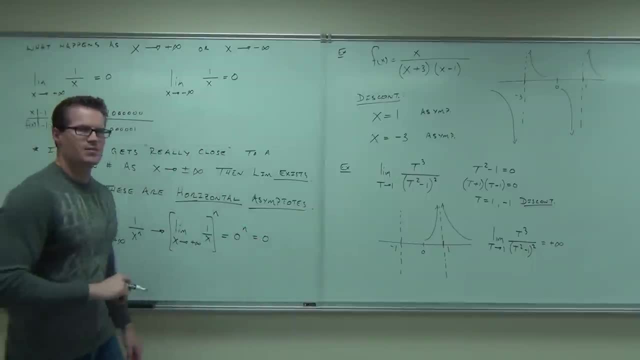 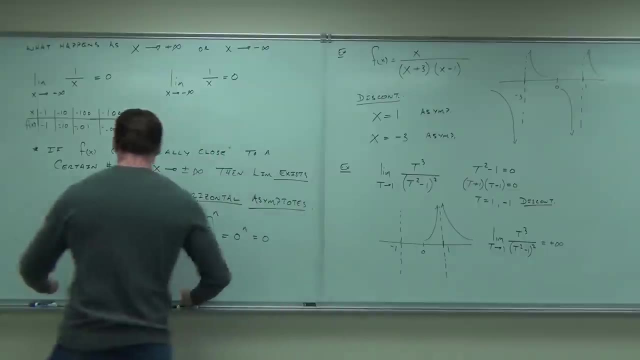 Zero to the n or zero, Does it make a difference? It makes a difference. if we're talking about negative infinity, Let's consider that Let's go to negative infinity. Negative infinity, That means- is this still true for negative infinity? 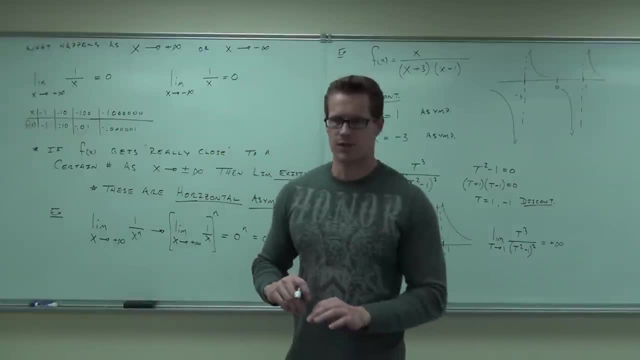 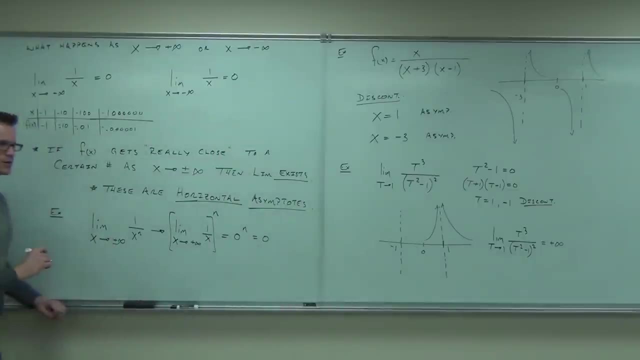 Does it make a difference if we're talking about negative infinity? Let's consider that. Let's go to negative infinity. Negative infinity, That means. is this still true for negative infinity? Absolutely, Is this still true? Is 1 over x as x approaches negative infinity? 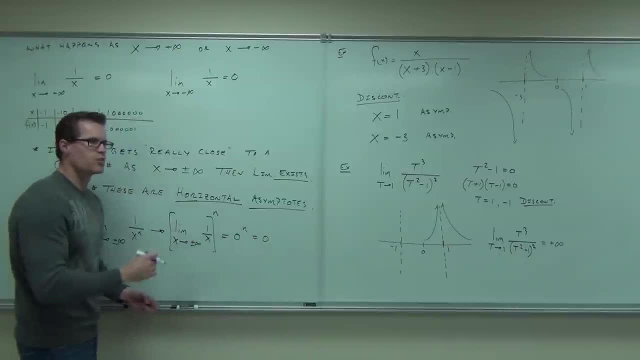 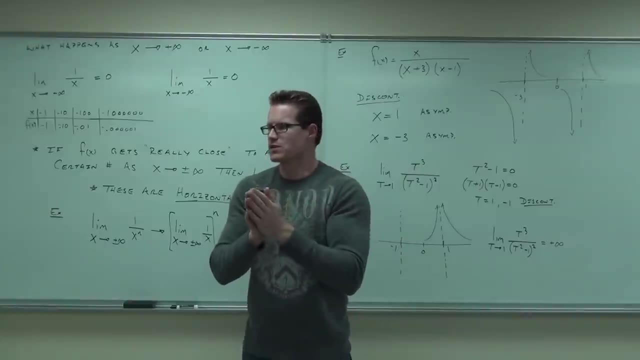 is that still 0? 0 to the n? that holds true for both of them. What this says is that 1, a constant over any variable that's being taken to infinity, is going to give you a horizontal asymptote. How many people feel OK with that, with that idea? 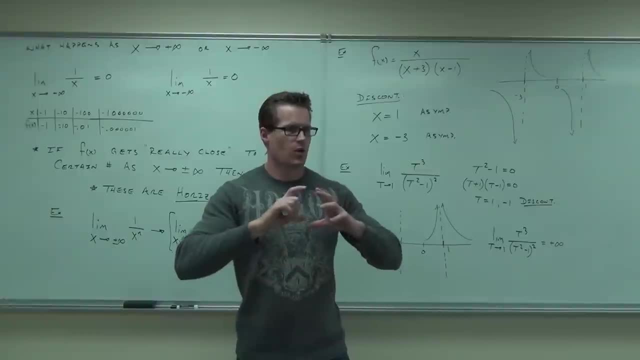 No matter what the power is squared, cubed doesn't matter, because you're always taking that 1 over x to that power, 1 over x as x approaches infinity. either positive or negative, it's going to be 0.. 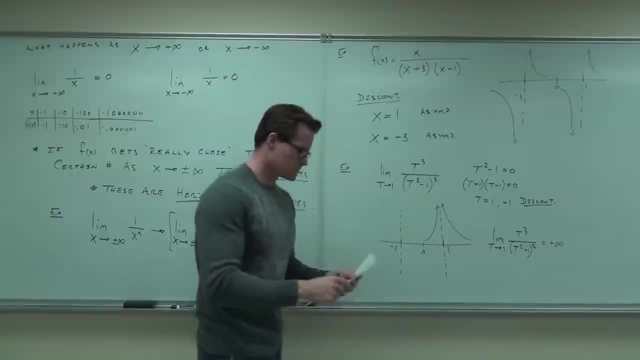 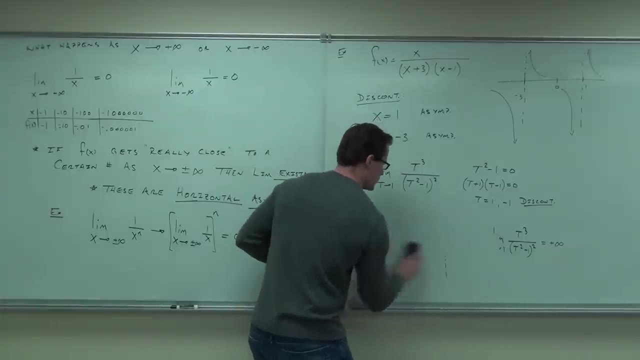 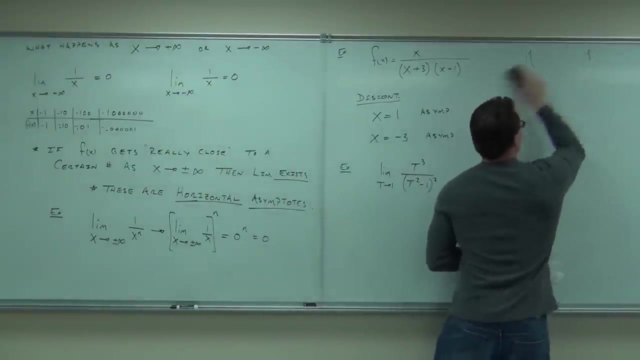 0 at any power is still 0.. Interesting thing: Horizontal asymptotes in each case at 0.. Now, before we get into some other computational stuff, let me show you one more idea Right now. we've done a lot of theory so far. 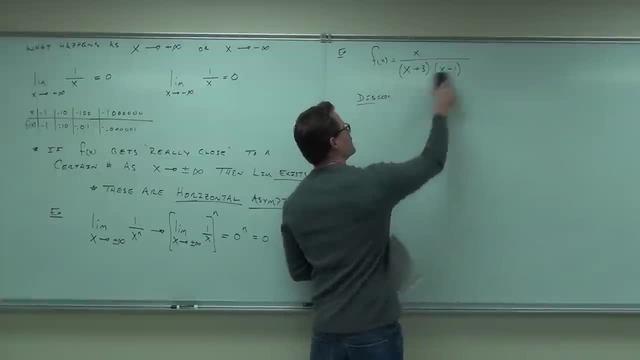 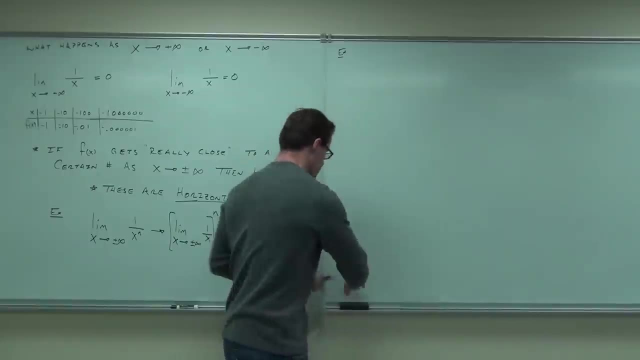 So there's not really a whole lot of examples. We're going to change that in just a minute, But I've got to talk about one more. I want you to think of polynomials. Let's talk about the limit of a polynomial. 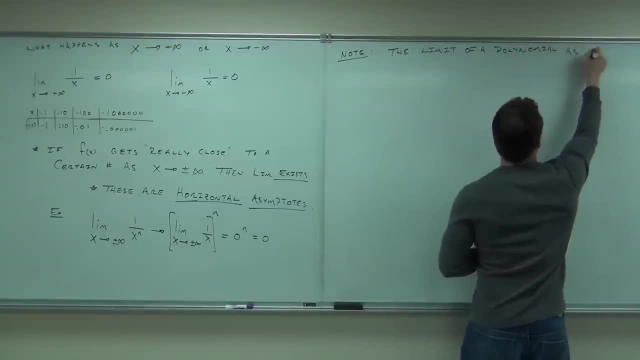 Let's talk about the limit of a polynomial. Let's talk about an asymptote. I want you to think of the ratio between the intercept Theнюc number. You can put 1 over 1 here. Do a little t there. 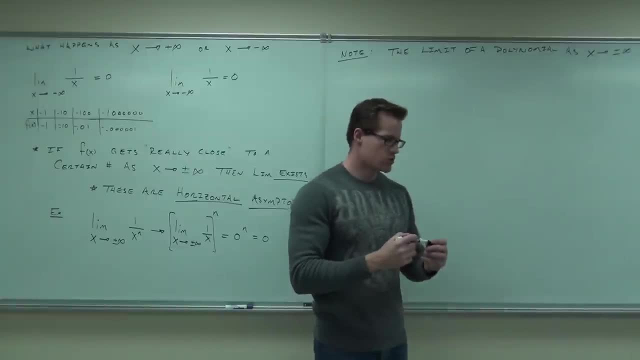 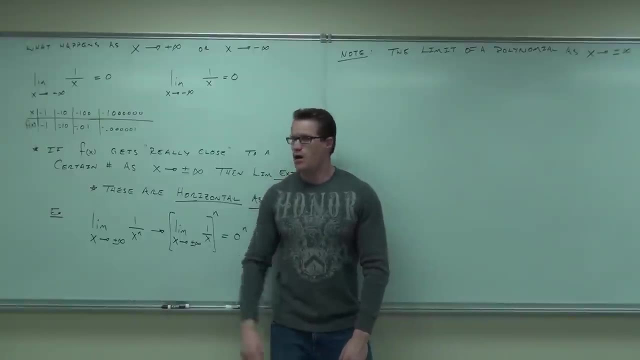 which is positive or negative infinity. Think about what you know. think about what you know about polynomials. Would you agree that polynomials are in one of these four? one, two, three, one of these four cases? Polynomials are either like this: 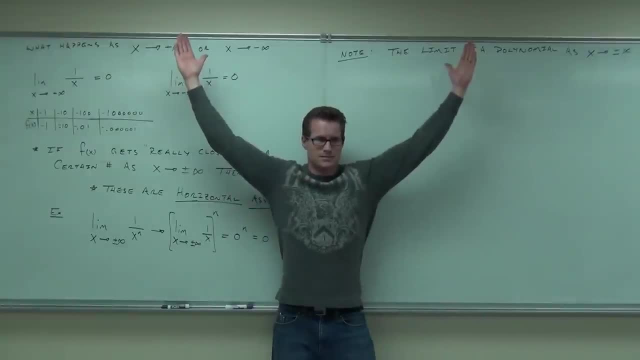 like this, like this or like that True. Think about x squared. x squared like this. Does it ever go to an actual number as we go this way? Does it ever go down or up and go to no polynomials? don't do that. 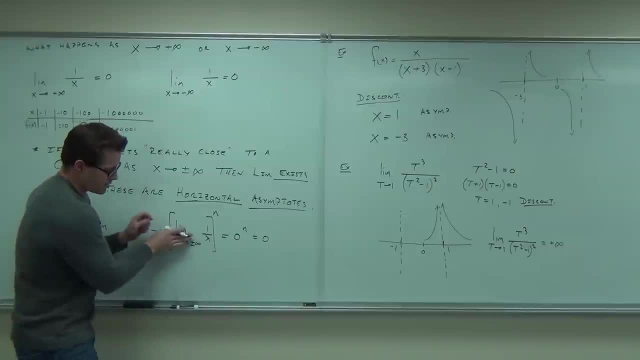 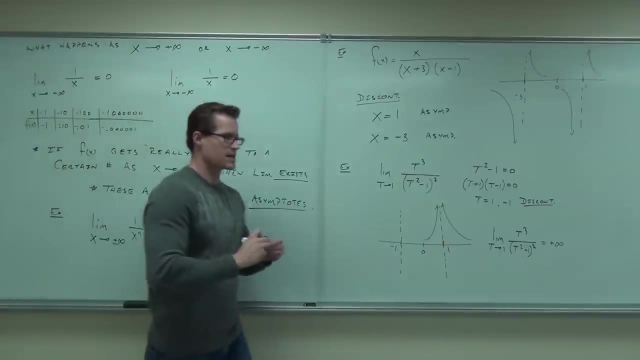 Absolutely. Is this still true? Is one over x as x approaches negative infinity? is that still zero? Zero to the n. that holds true for both of them. What this says, is that one a constant over any variable that's being taken to infinity, it's gonna give you. 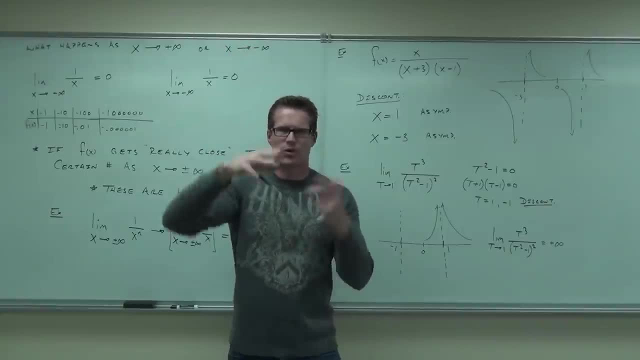 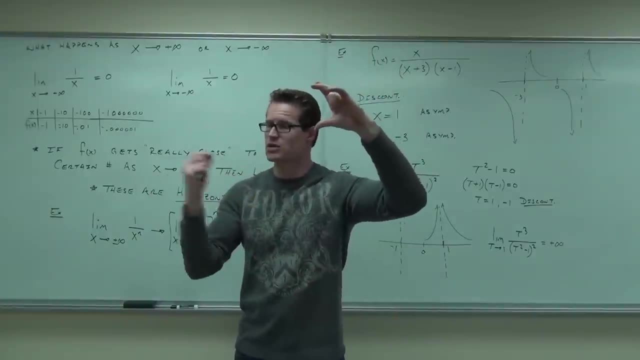 a horizontal asymptote. How many people feel okay with that, with that idea, No matter what the power is, square cube doesn't matter, because you're always taking that one over x to that power, One over x as x approaches infinity. 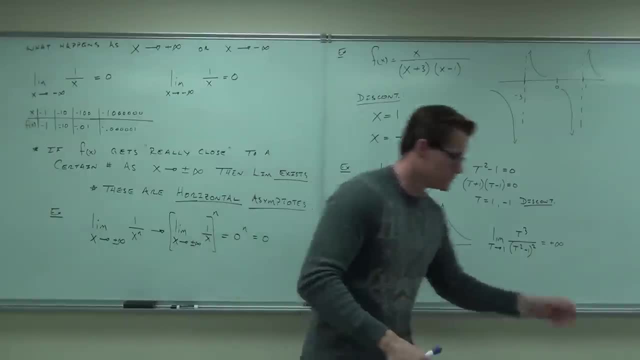 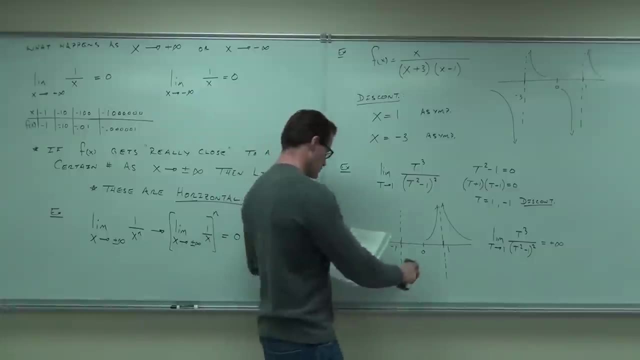 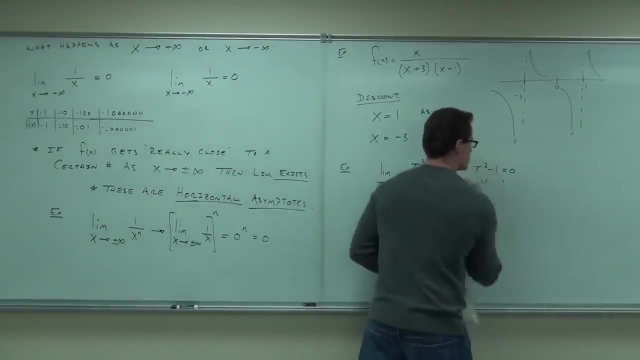 either positive or negative, it's gonna be zero. Zero to any power is still zero. Interesting thing: Horizontal asymptotes, in each case at zero. Now, before we get into some other computational stuff, let me show you one more idea Right now. we've done a lot of theory so far. 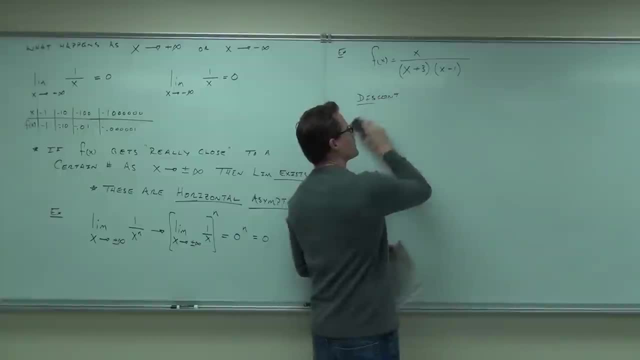 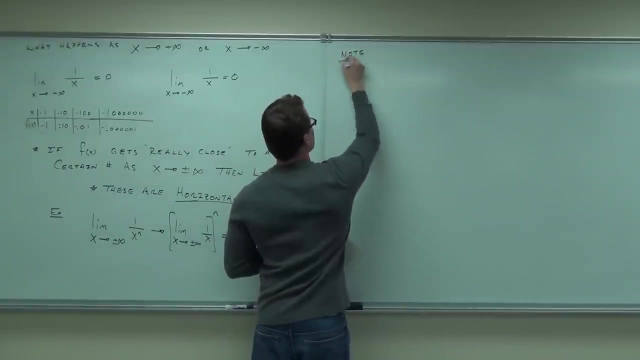 so there's not really a whole lot of examples. We're gonna change that in just a minute, But I gotta talk about one more. I want you to think of polynomials. Let's talk about the limit of a polynomial that approaches x. 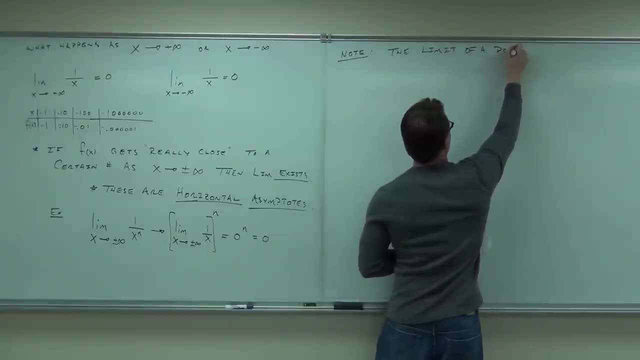 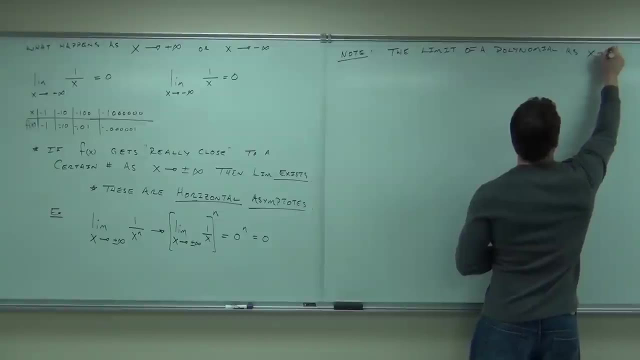 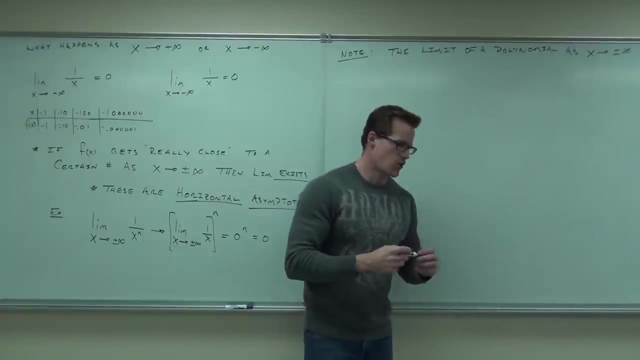 So, if x approaches positive or negative infinity, think about what you know. think about what you know about polynomials. Would you agree that polynomials are in one of these four? one, two, one of these four cases? One, two, three, four, five, six, seven, eight, nine, 10,. 11,, 12,, 13,, 14,, 15,, 16,, 17,, 18,, 19,, 20,, 21,, 22,, 23,, 24,, 25,, 26,, 27,, 28,, 29,, 20, and 25.. 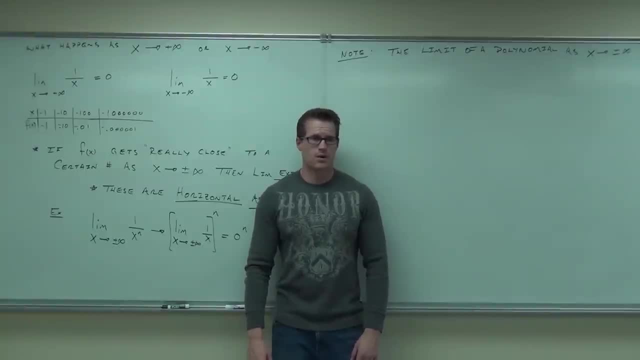 All right, let's go to polynomials. Polynomials are, in one of these four, one, two, three. one of these four cases, Polynomials are either like this, Like this, Like this Or like that. True, Think about x squared, x squared like this. 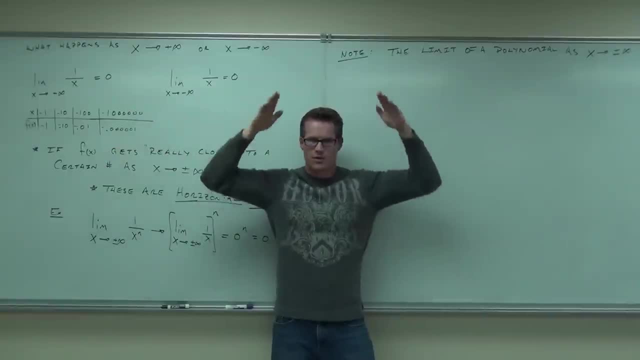 Does it ever go to an actual number as we go this way? Does it ever go down or just up and go to? no Polynomials don't do that. Polynomials always have a cradle somewhere. An x cubed would go this way to that way, right. 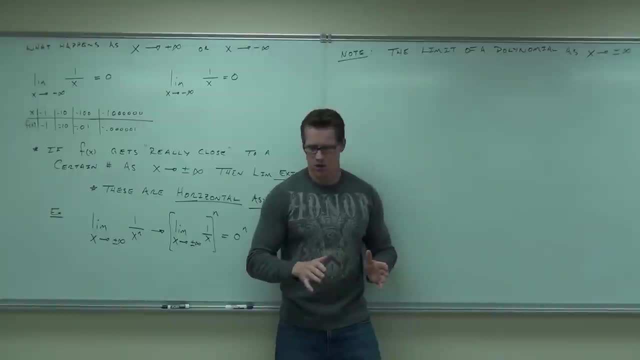 Polynomials always have a cradle somewhere. An x cubed would go this way, to that way, right. Negative x cubed goes this way, to this way. X squared goes this way. Negative x squared goes this way. They never actually go to an actual number. 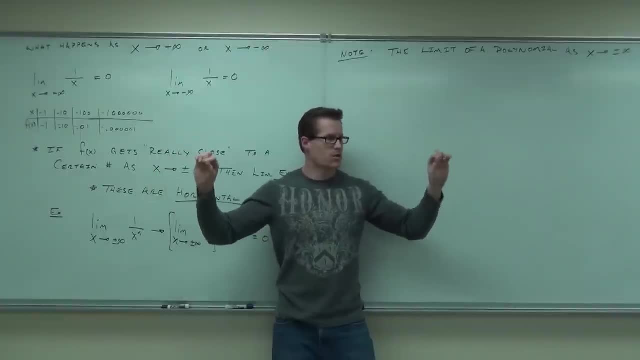 They're all either going to positive or negative infinity. So as we approach for any polynomial, positive or negative infinity on the x-axis, the function itself approaches positive or negative infinity on the y-axis. Let me say that one more time because I think I lost something. 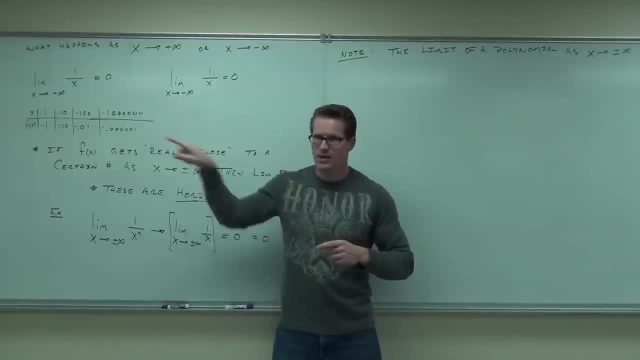 As you travel this way on the x, your function is doing one of two things: going this way forever or going this way forever. You follow me on that one. That's what I just said. okay, If you're going this way on the x-axis. 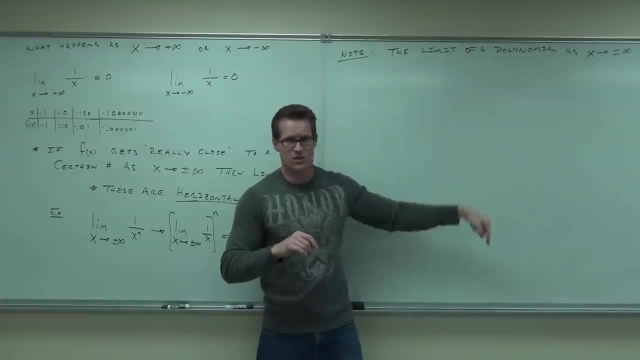 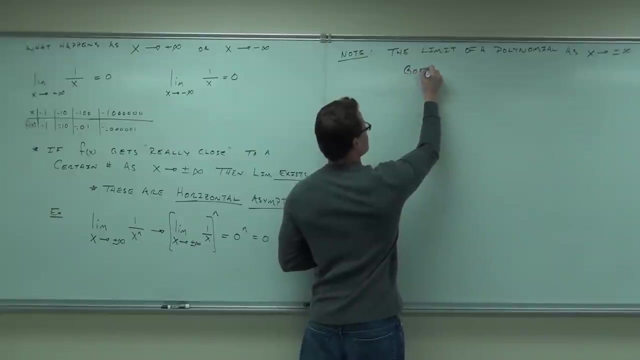 your function is doing one of two things: Going this way Forever, Going this way Forever. we're going this way forever. that's what this says. the limit of a polynomial as X approaches negative infinity or positive infinity goes to positive or negative infinity itself. I'll give you some examples of this. 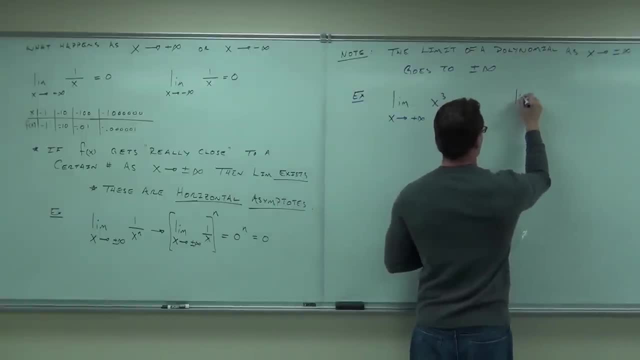 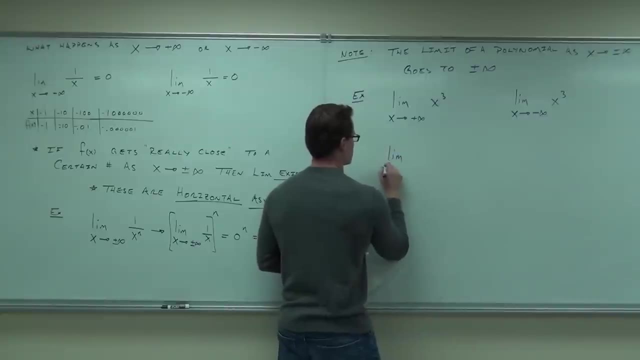 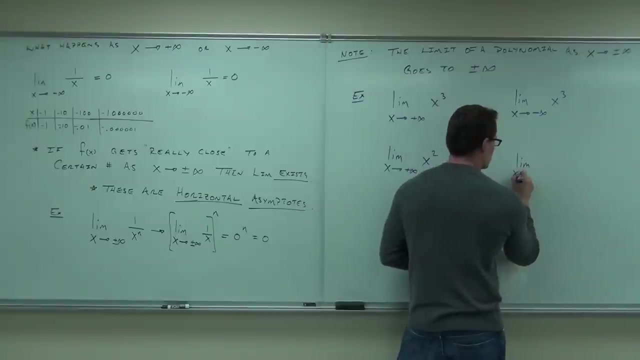 by the way, you're going to notice that I always use positive and negative infinity. that's something I do because I don't like to get confused. if I say positive, I write the positive. that's just the way I do it. do you have to do it that? 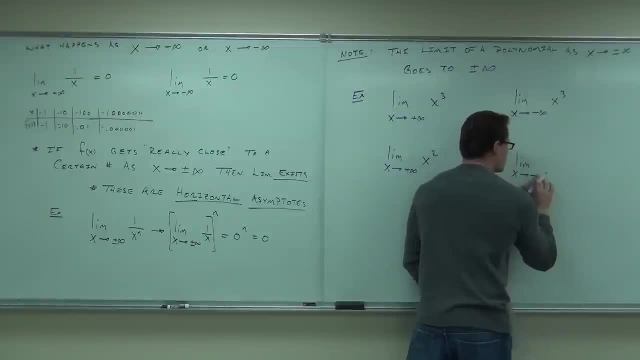 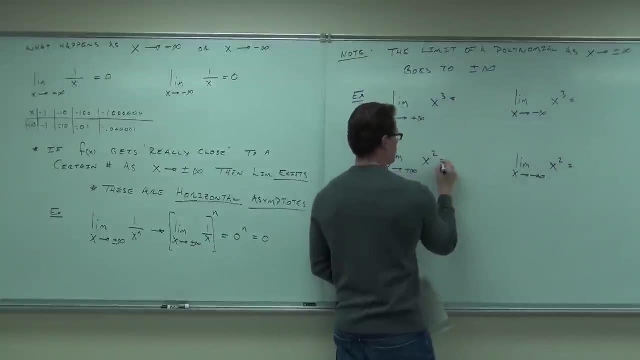 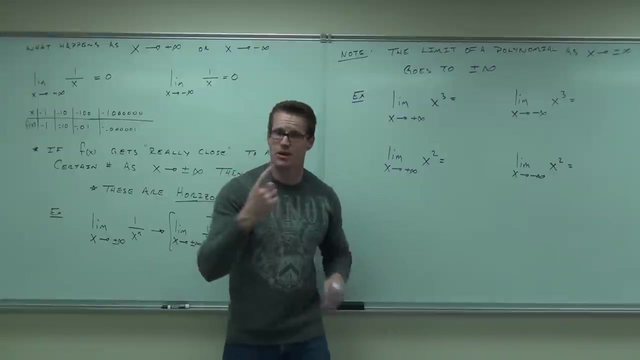 way. no, not necessarily helps me. let's get, let's consider this. okay now, infinity is not something we can actually plug in, but something we can think about. in fact, this one guy actually went crazy thinking about the sizes of infinity, because there's different sizes of infinity, which is pretty interesting itself. but so thinking 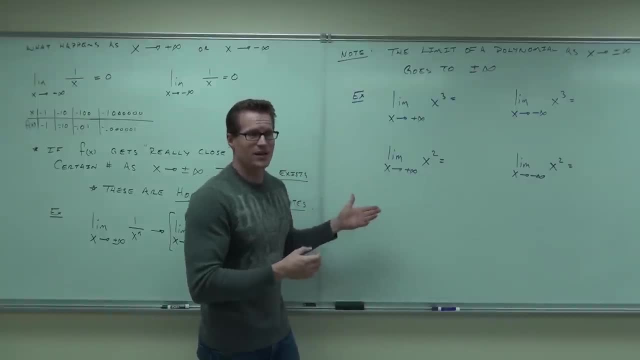 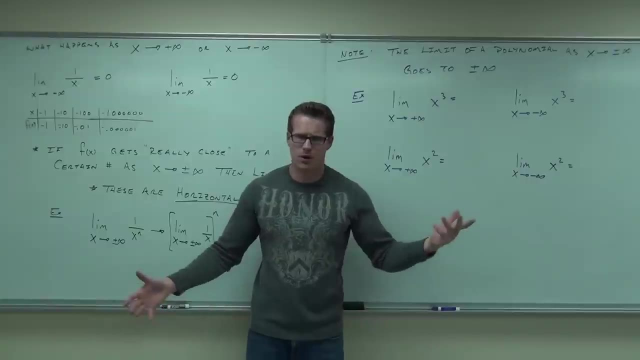 on infinity is kind of weird to think about, but we can do it. think about this: take a big point, positive number, plug it into x cubed. You know the shape of x cubed. right, It's a polynomial. it's gonna be like this: 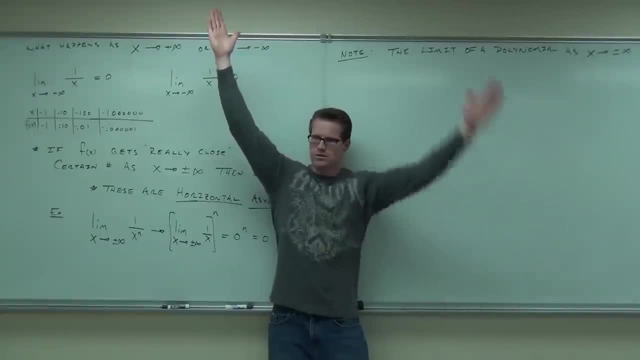 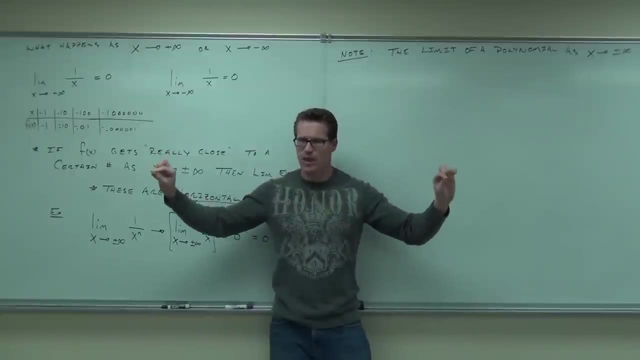 Negative x cubed goes this way, to this way X squared goes this way. Negative x squared goes this way. They never actually go to an actual number. They're all either going to positive or negative infinity. So as we approach, for any polynomial, the positive 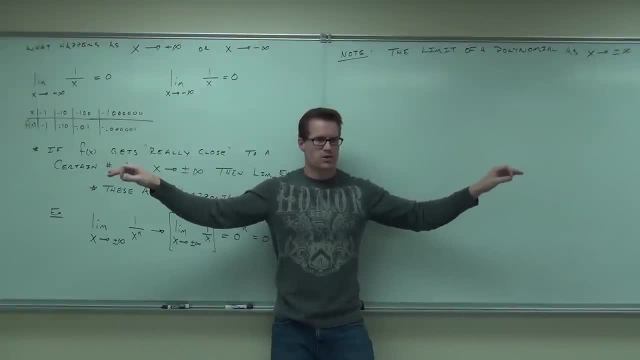 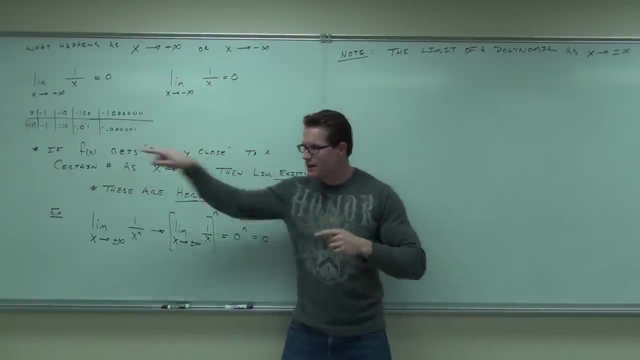 or negative infinity on the x axis, the function itself approaches positive or negative infinity on the y axis. Let me say that one more time because I think I lost it As you travel this way. on the x, your function is doing one of two things. 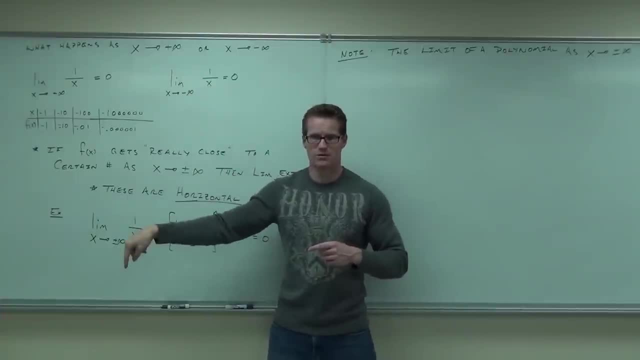 going this way forever or going this way forever? You follow me on that one. That's what I just said. okay, If you're going this way on the x axis, your function is doing one of two things: going this way forever or going this way forever. 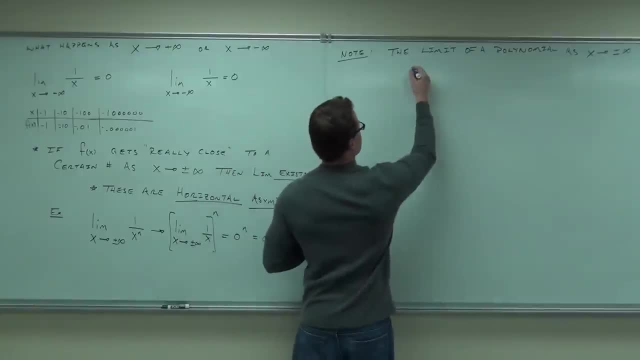 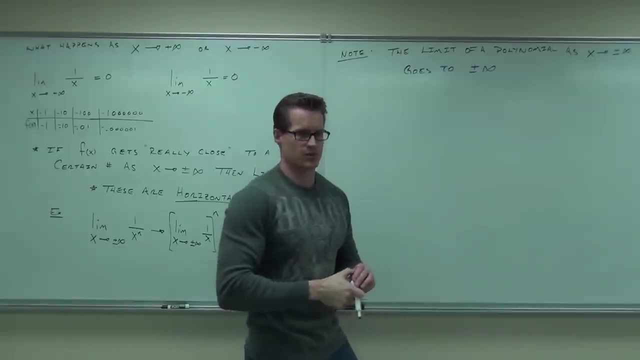 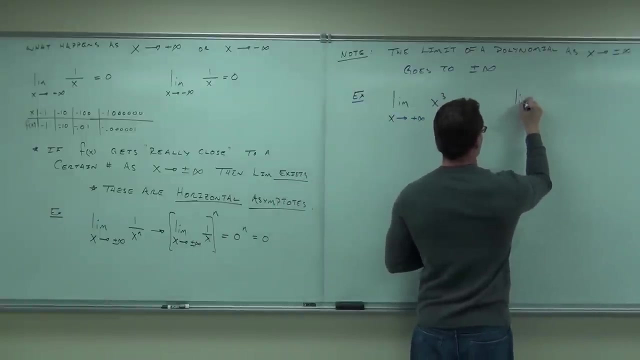 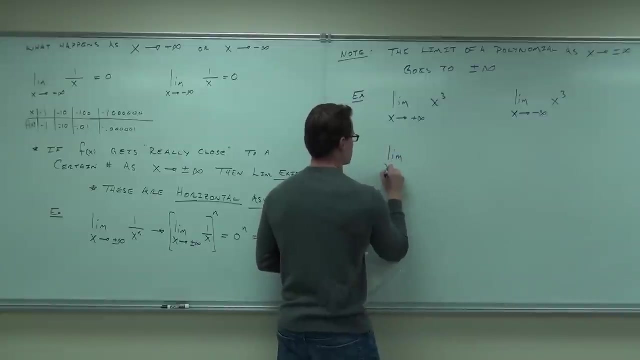 That's what this says. The limit of a polynomial as x, as x approaches negative infinity or positive infinity goes to positive or negative infinity itself. I'll give you some examples of this. Let me write it down here. I'll leave it at that for now. 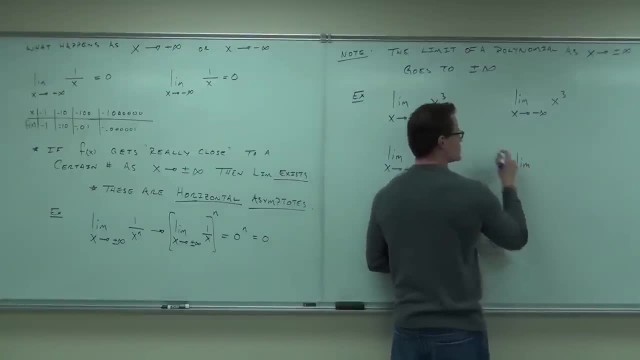 We always use positive forever for allนะคะ. when we find ourStanОt Ş out, It's only because we know that all contractions have ways to make them work. By the way, you're going to notice that I always use positive and negative infinity. 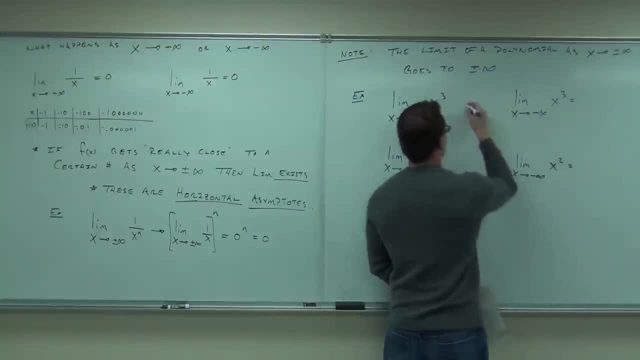 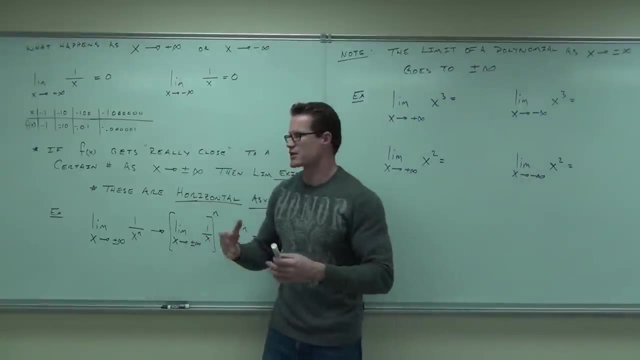 That's something I do because I don't like to get confused. I buy, say positive, I write the positive. That's just the way I do it. Let's consider this. okay Now, infinity is not something we can actually plug in. 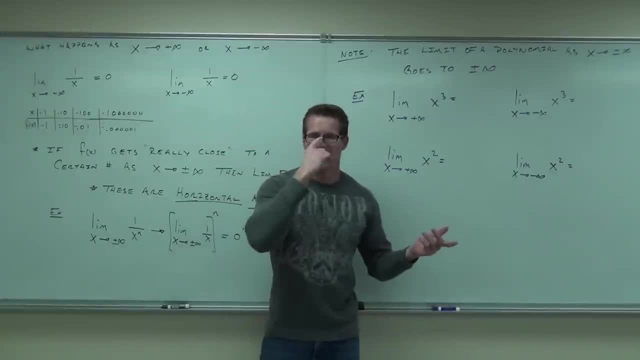 but it's something we can think about. In fact, this one guy actually went crazy thinking about the sizes of infinity, because there's different sizes of infinity, which is pretty interesting in itself. So thinking about infinity is kind of weird to think about. 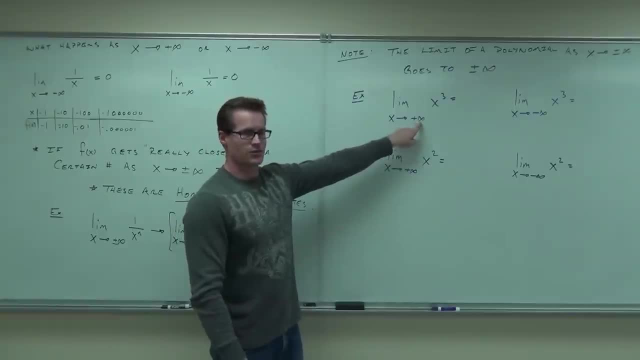 but we can do it. Think about this: Take a big positive number, plug it into x cubed. You know the shape of x cubed. right, It's a polynomial. it's gonna be like this: Take a positive number and plug it in. 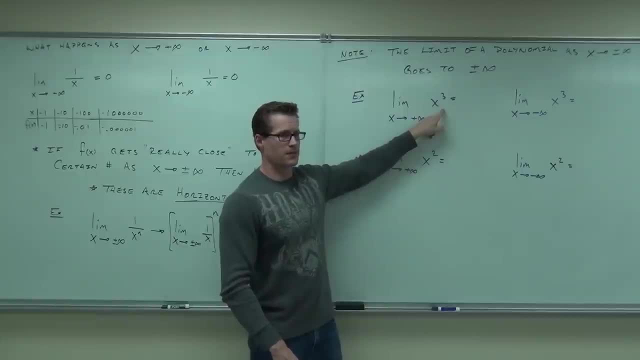 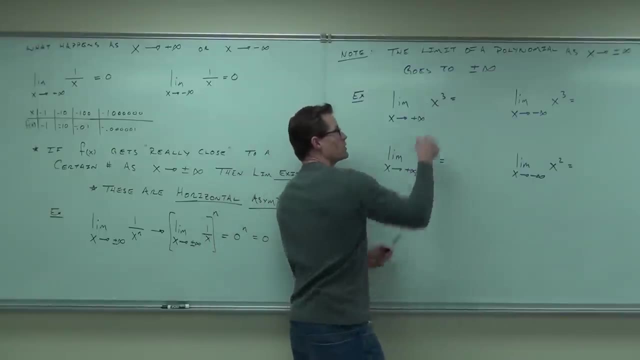 Take a positive number and plug it in. Do you get a positive or negative? Positive: Take a bigger number. Is it still positive? Take a bigger number: Is it still positive? In fact, it's getting bigger and bigger. This is going to go to positive infinity. 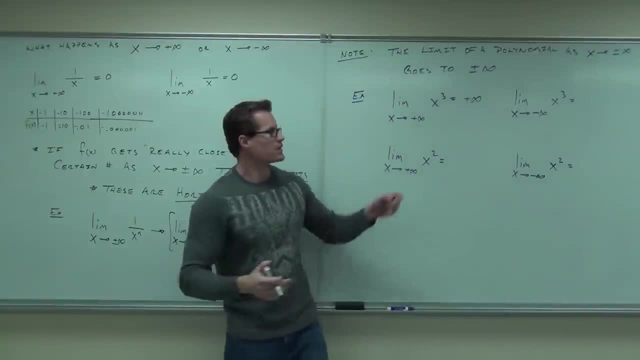 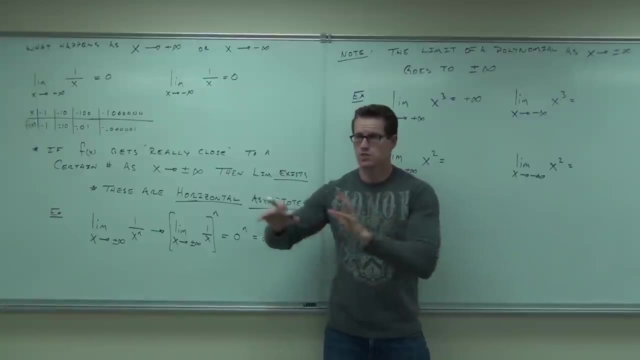 The bigger the positive number I plug in, the bigger the positive number I get out. Let's try this one: Negative infinity. Take a negative number, plug it in. What do you get? Negative? Take a smaller negative number, even more negative. 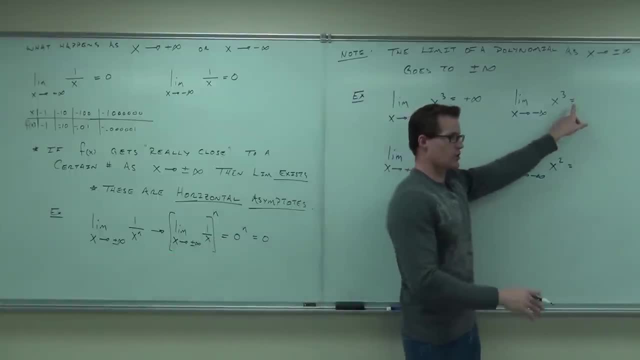 Plug it in. Do you still get negative? Do you see that this one's actually going to negative infinity? The further we go left on the number line, the further we go down on the y-axis- Negative infinity, And that's what that says. 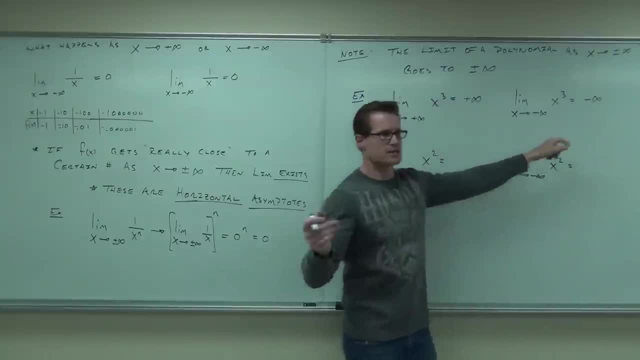 The further you go left, the further your function drops. That's what that's saying. Does that make sense to you? How about this one X squared? Take a positive number, Plug it in X squared. Where are you going? 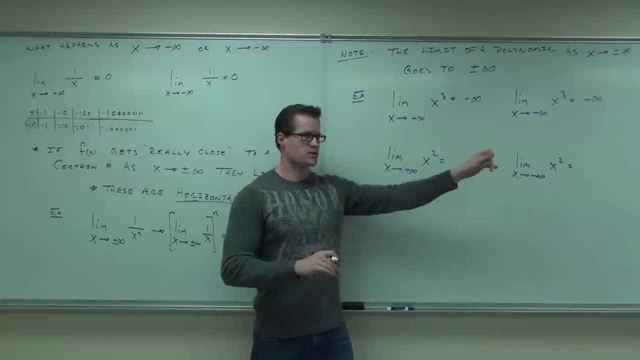 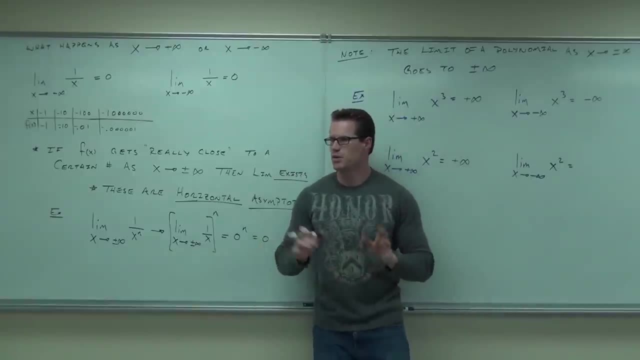 Up or down. Up, Up, Positive infinity. So the bigger the positive number, the bigger the positive number. Try that one, though. Take a negative number, plug it in. What do you get? A positive, Uh-huh. 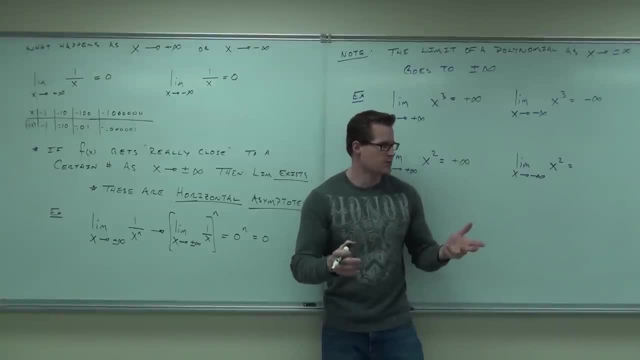 A positive Because x squared takes that number and makes it positive. So even though we're going to the left, our function is going up. That's why x squared looks like that It's going to go up on both sides. This is also positive: infinity. 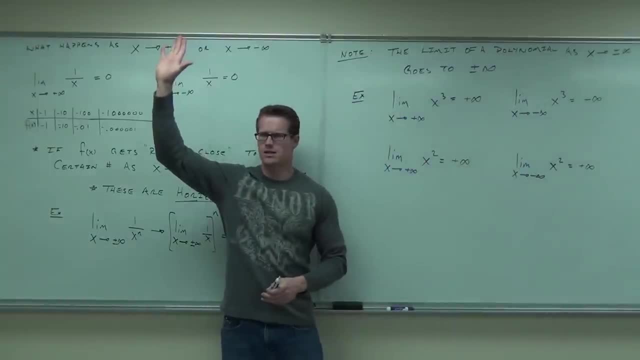 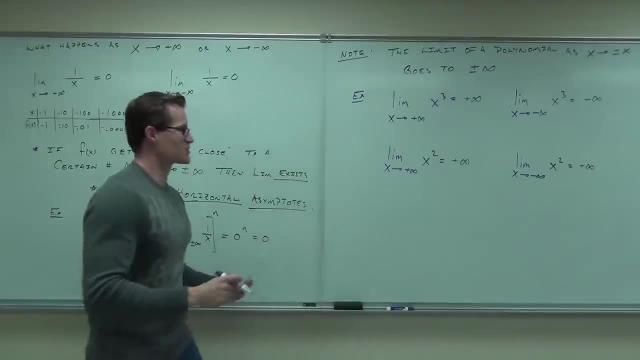 Show of hands how many people feel OK with our limit ideas. so far, Good, All right, All right. By the way, this is kind of an interesting little note. Did you know that the behavior of the polynomial itself will follow the behavior of the leading term? 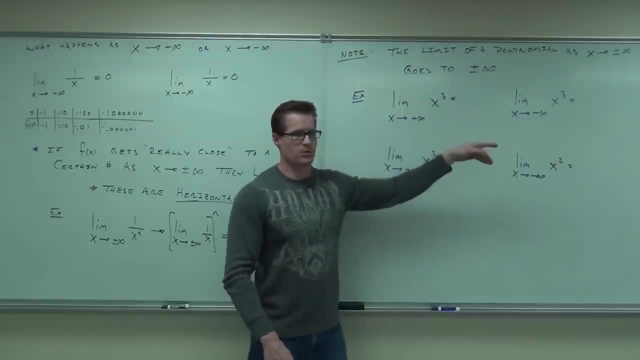 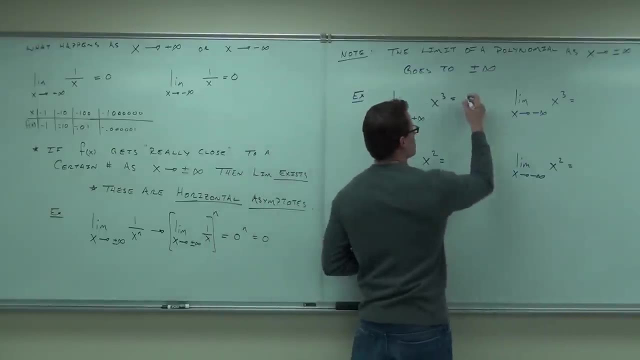 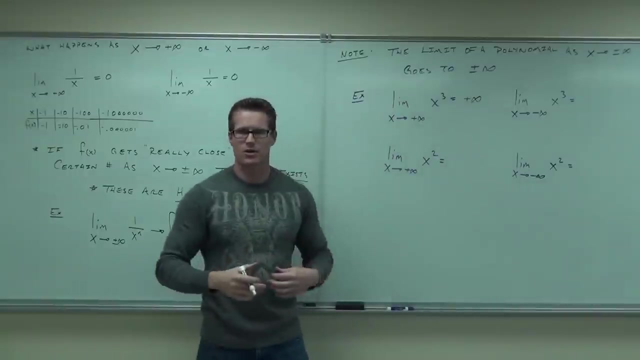 Do you get a positive or negative? Positive: Take a bigger number. Is it still positive? Take a bigger number: Is it still positive? In fact, it's getting bigger and bigger. This is going to go to positive infinity. The bigger the positive number, I plug in. 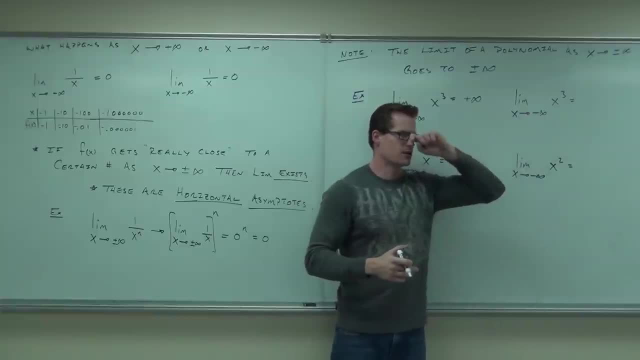 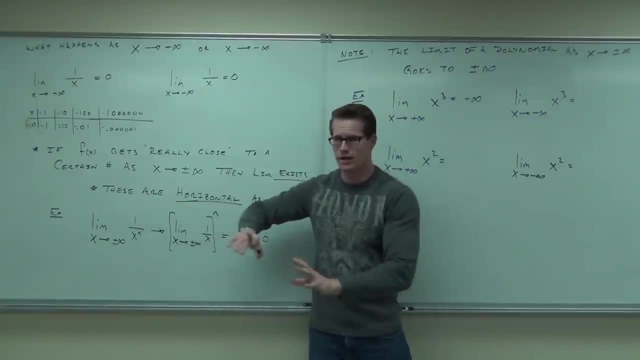 the bigger the positive number I get out. Let's try this one: negative infinity. Take a negative number, plug it in. what do you get? Take a smaller negative number, even more negative, Plug it in, do you still get negative? 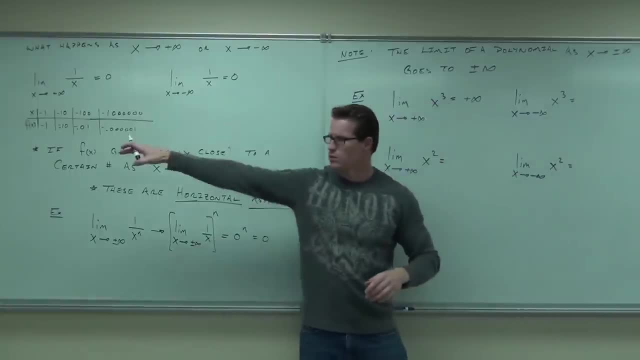 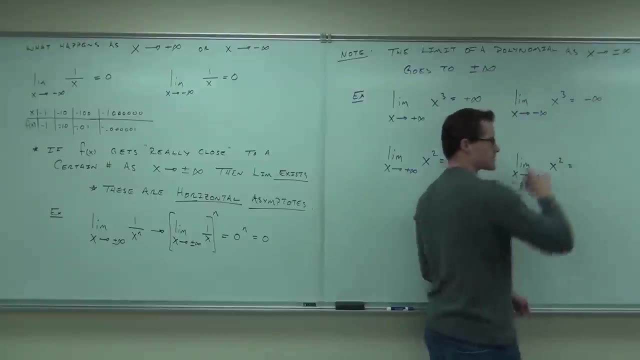 Do you see that this one's actually going to negative infinity? The further we go left on the number line, the further we go down on the y-axis- Negative infinity, And that's what that says. The further you go left, the further your function drops. 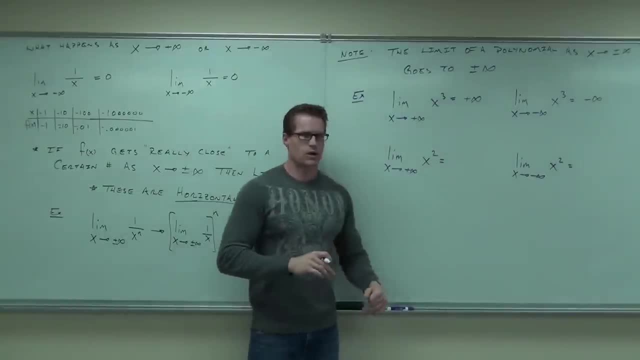 That's what that's saying. Does that make sense to you? How about this one x squared? Take a positive number, plug it in x squared. Where are you going? up or down? Up, Up positive infinity. So the bigger the positive number. 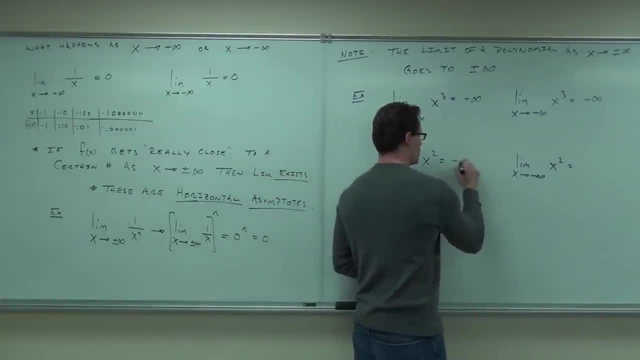 the bigger the positive number. Try that one, though. Take a negative number, plug it in. What do you get? A positive. Uh-huh, a positive, Because x squared takes that number and makes it positive. So, even though we're going to the left, 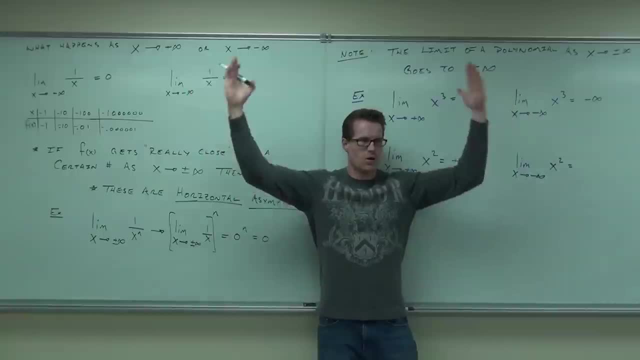 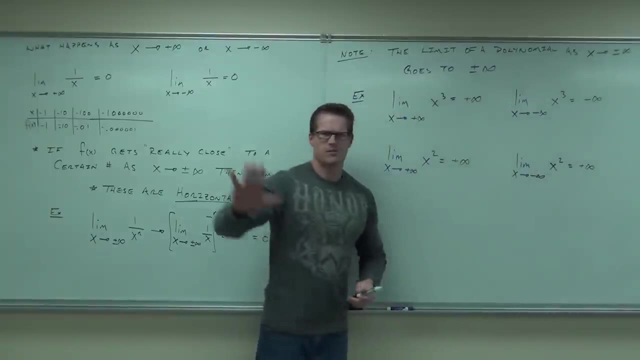 our function is going up. That's why x squared looks like that. Right, It's going to go up on both sides. This is also positive infinity Show of hands. how many people feel okay with our limit idea? so far, Good, all right, all right. 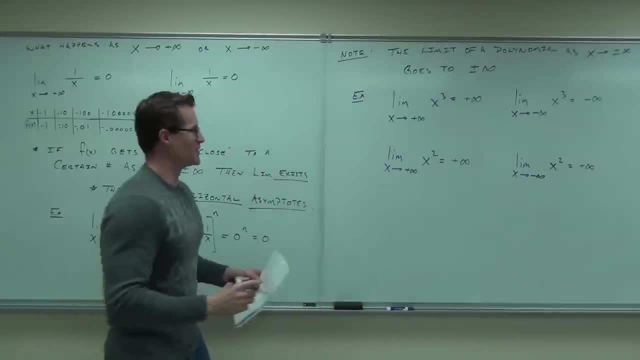 By the way, this is kind of an interesting little note. So did you know? did you know, that the behavior of the polynomial itself will follow the behavior of the leading term? Did you know that? I'll explain that in a second. Sorry, I'll say it this way: 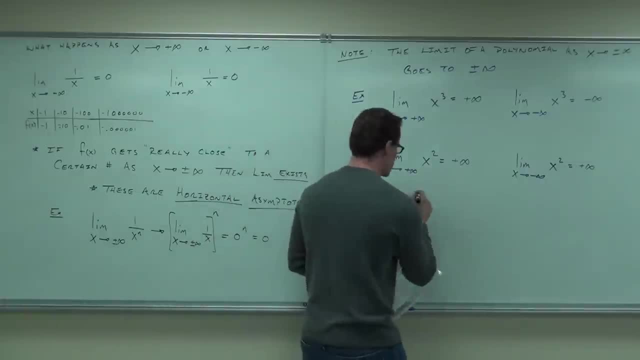 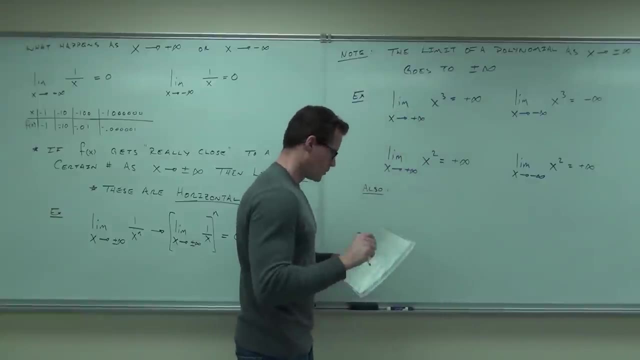 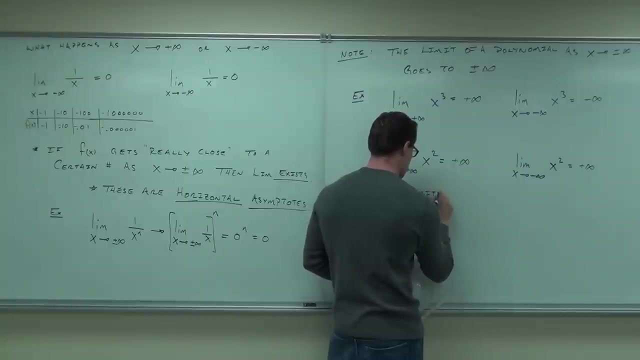 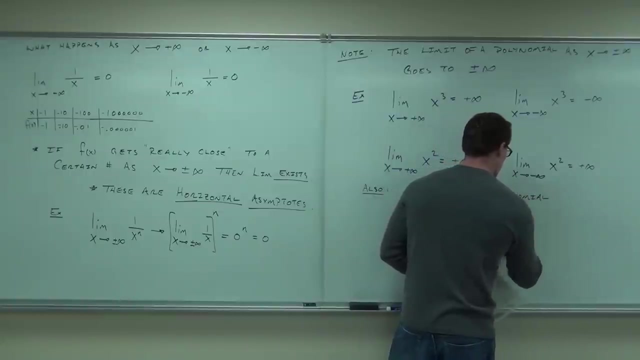 Did you know that? No, No, I'll explain that in a second. Sorry, I'll say it this way: Limits of a polynomial will follow the behavior of the highest power of a term. No, The polynomial, nothing else polynomial. 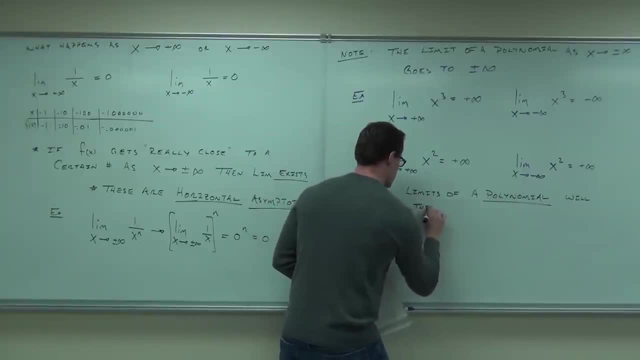 There are no rules Again. the polynomial is only a formula. I don't know if you've followed that. That's a good question, So you can use that When you heard the formula. I'm sorry to interrupt. I'm not sure that the word polynomial works. 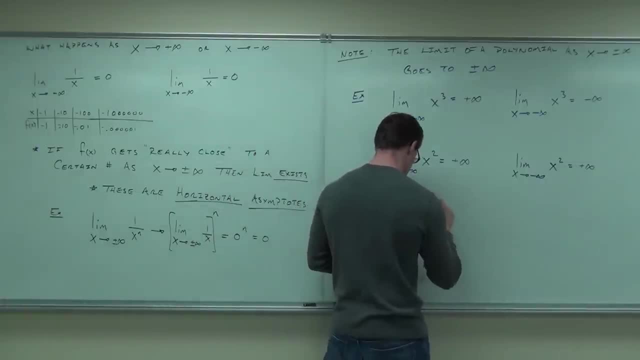 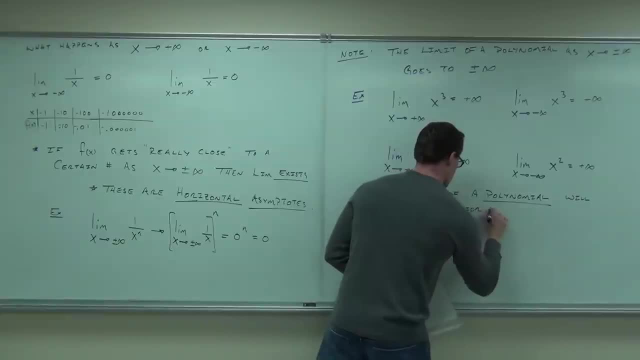 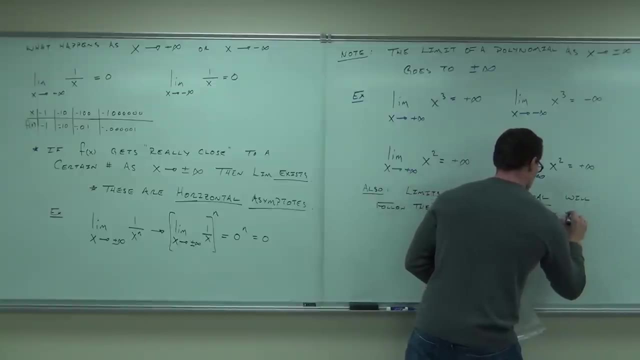 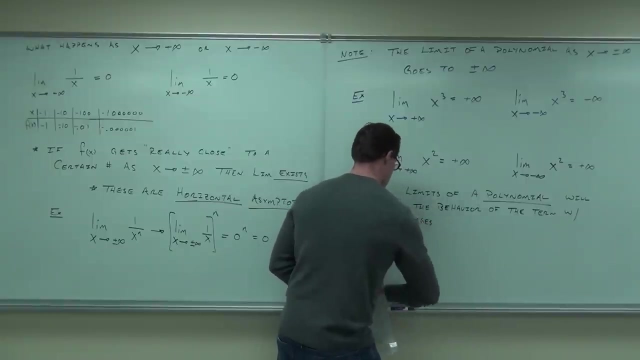 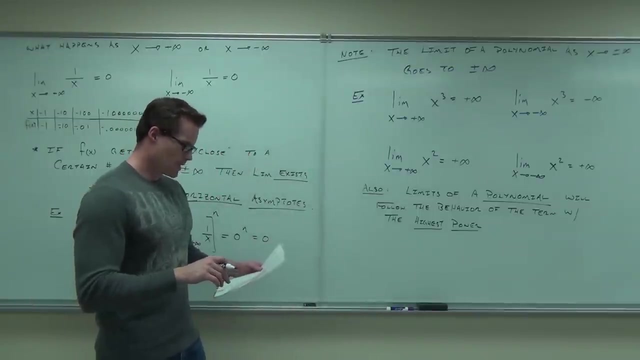 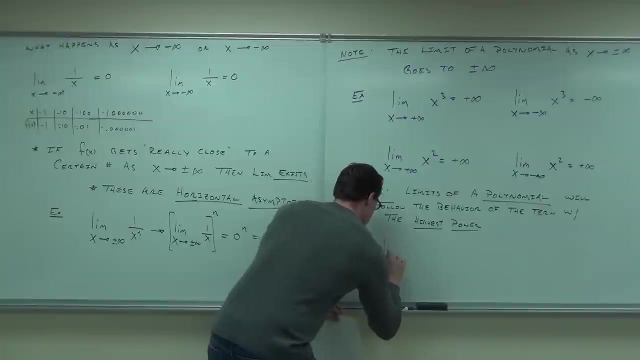 Thank you. Let me give you one quick example, because I think you'll really handle this pretty well. Let's say that I want to talk about the limit as x approaches. negative infinity of negative: 3x cubed minus 2x, squared minus x. 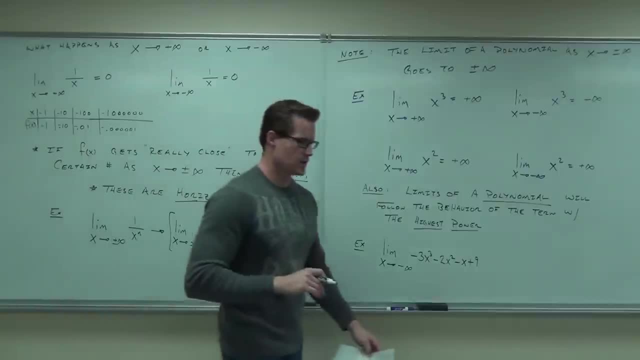 Well, it's not Now. here's what you can't do. What you can't do is go. oh, let's see Negative infinity cubed negative, infinity times negative. that's positive infinity minus a positive infinity, that's oh man. 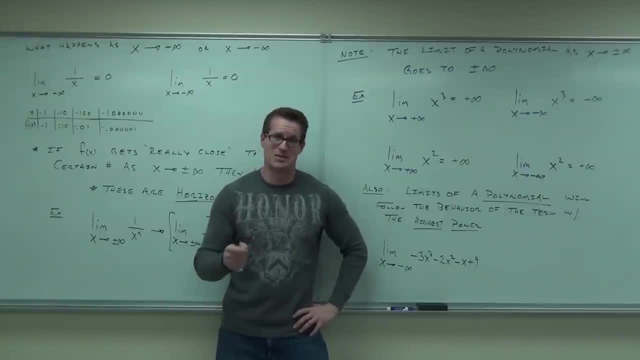 If you start doing stuff like that, subtracting infinities, that is going to make you go crazy. What you need to understand is that all this subtracting and subtracting and adding the infinities are meaningless. The behavior of this polynomial is going to follow the term that has the largest power. 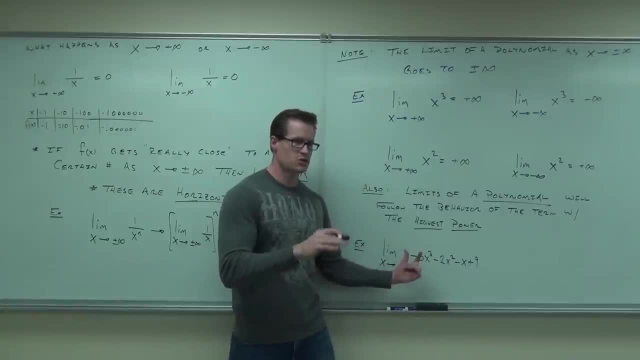 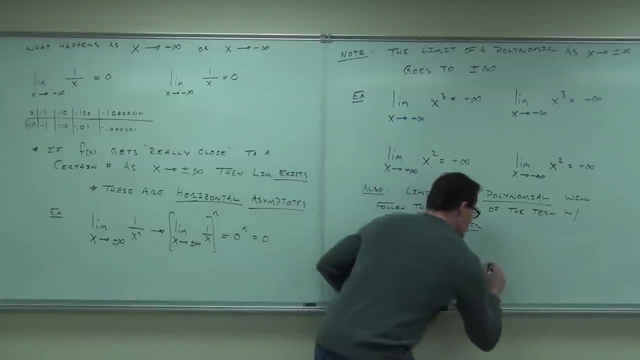 The term that has the largest power is usually in front. It doesn't have to be, but it's usually in front of your polynomial, It's this one. Here's what this little corollary says, what this action theorem says. It says this is going to be equal to the limit as x approaches. negative infinity of just the negative 3x cubed. 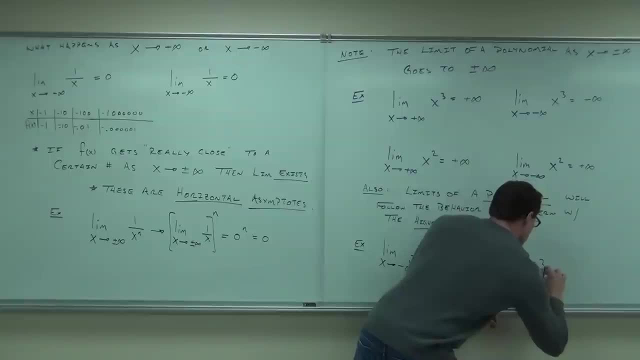 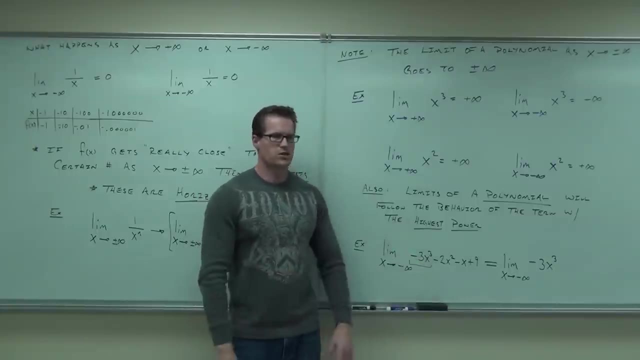 Don't forget that. Don't forget the negative. that's important, but the negative 3x cubed. You know this intuitively. In fact, when you think about it. look at that. The power is 3.. Don't you automatically know it's going to be s-curve? 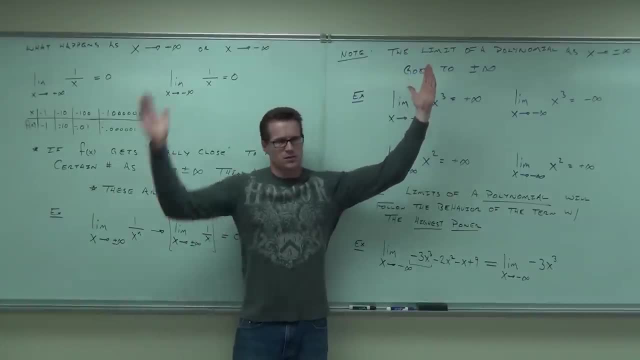 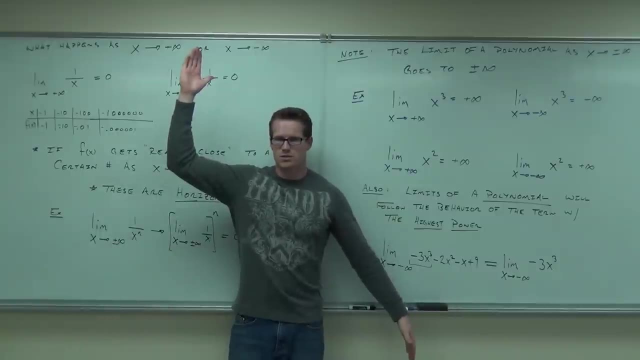 For sure it's going to be doing this. A power of 4 would look like this: 5,, 6,, 7,, 8, you know that right Now negatives would be opposite, so negative x cubed negative. oh, I did it wrong. 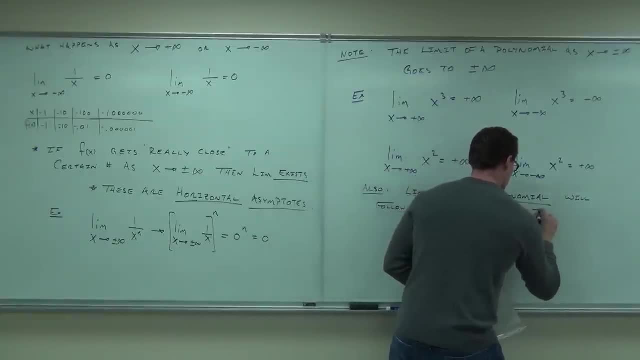 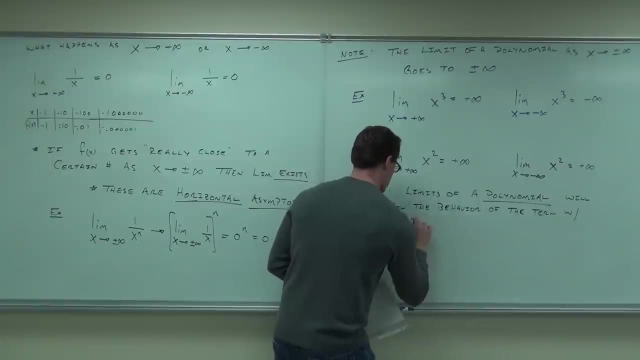 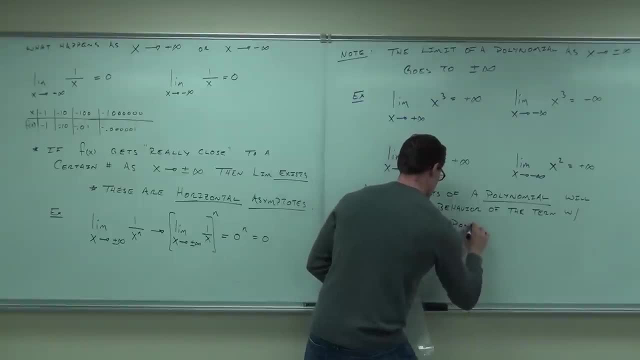 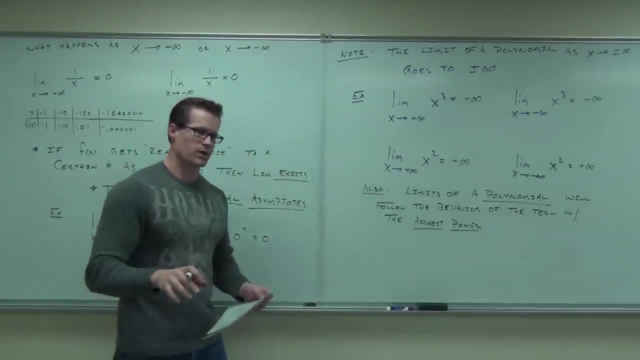 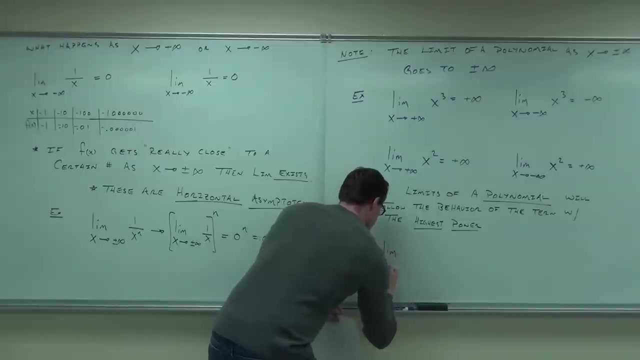 Thank you, Thank you, Thank you. Let me give you one quick example, because I think you'll really handle this pretty well. Let's say that I want to talk about the limit as x approaches negative infinity of negative 3x cubed minus 2x, squared minus x plus 9.. 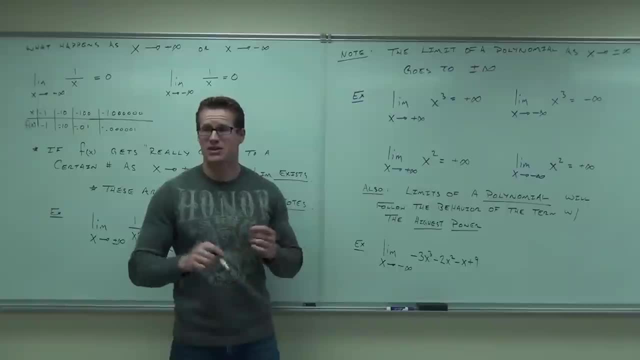 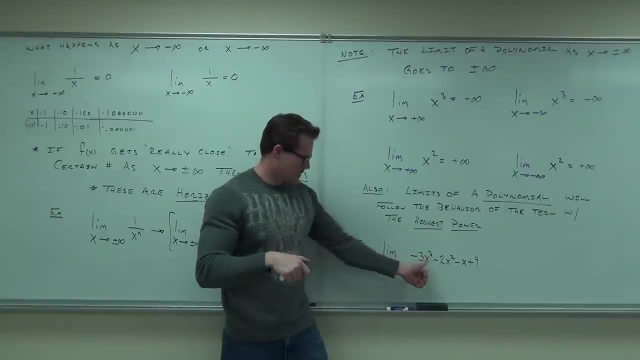 Now here's what you can't do. What you can't do is go: Oh, let's see Negative infinity cubed negative, infinity times negative. that's positive infinity minus a positive infinity. that's- oh, man, I don't know. 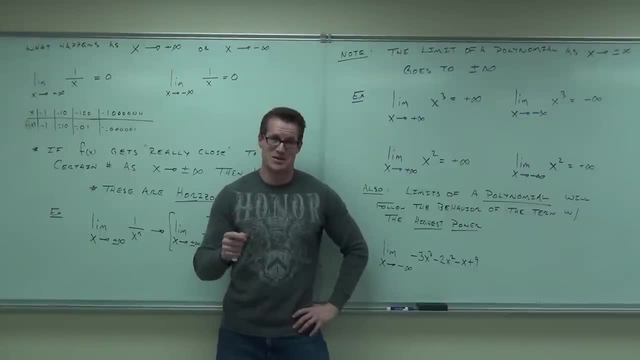 If you start doing stuff like that- subtracting infinities- that is going to make you go crazy. What you need to understand is that all this subtracting and adding the infinities are meaningless. The behavior of this polynomial is going to follow the term that has the largest power. 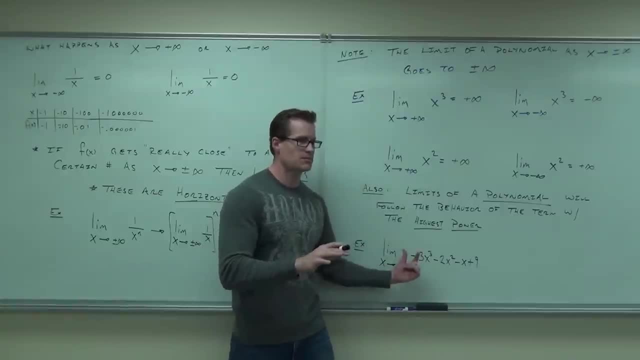 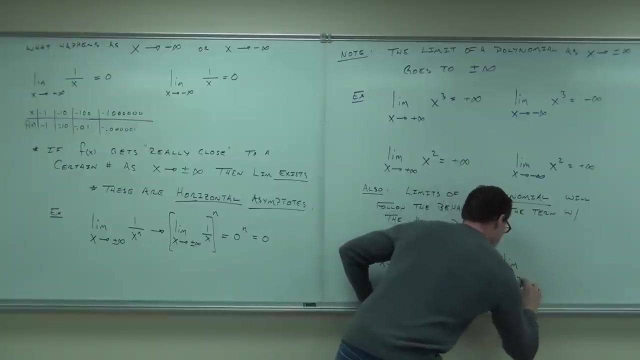 The term that has the largest power is usually in front. It doesn't have to be. It's usually in front of your polynomial, It's this one. Here's what this little corollary says, what this action theorem says. It says this is going to be equal to the limit as x approaches. negative infinity of just the negative 3x cubed. 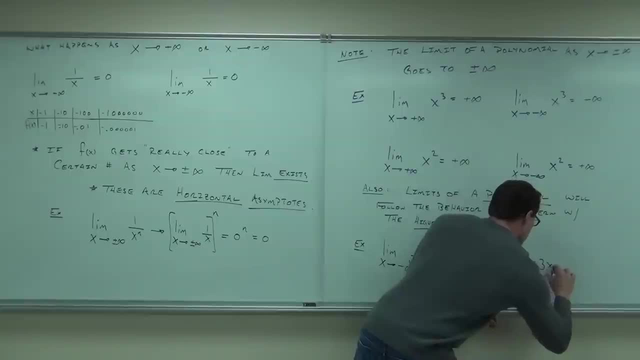 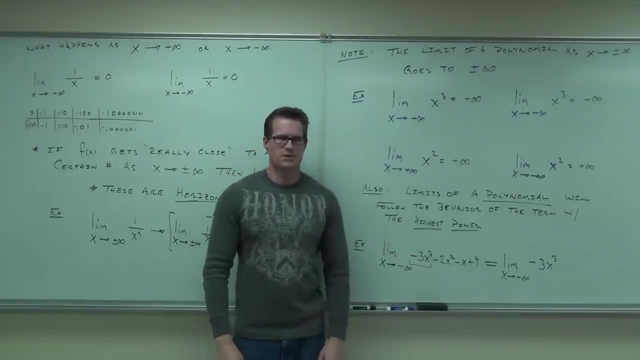 Don't forget the negative. That's important, But the negative 3x cubed. You know this intuitively, In fact, when you think about it. look at that, There's 3.. Don't you automatically know it's going to be s-curve? 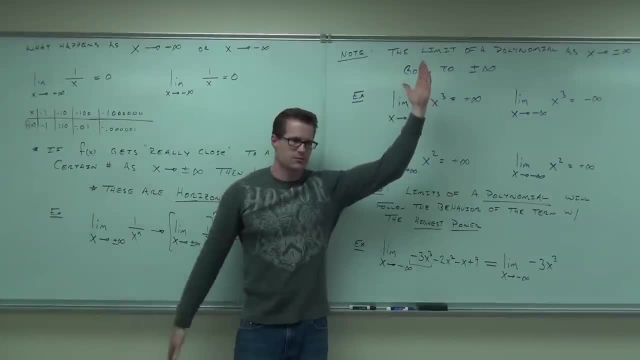 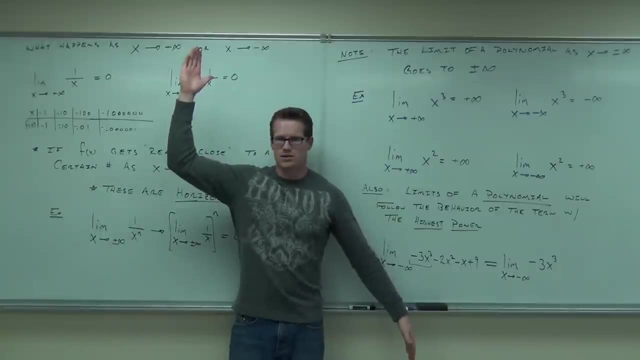 For sure it's going to be doing this. A power of 4 would look like this: 5,, 6,, 7, 8.. You know that right Now negatives would be opposite. So negative x cubed. 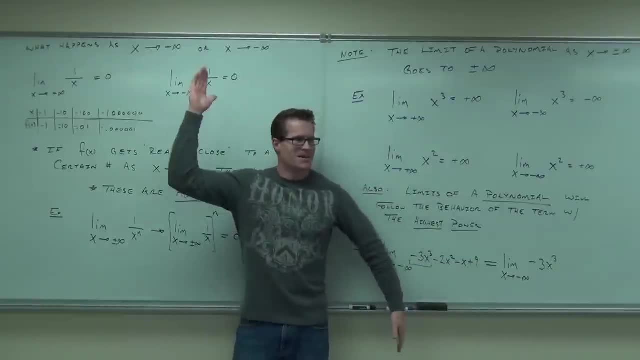 Negative of that dude, right? No, I'm going to go with Nancy. Negative x, cubed. negative x to the fourth, Negative x to the fifth. It's going to do that, right, You know that, intuitively, It follows that leading term. 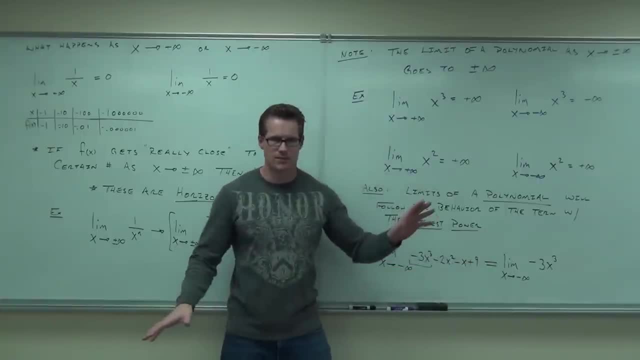 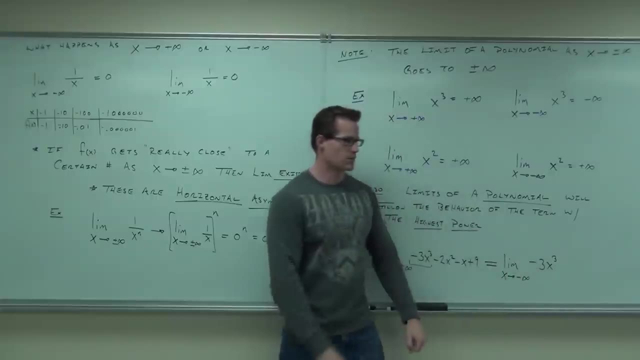 All the rest of this is garbage as far as I'm concerned. Really, when you talk about infinity, Now, normal limits, no, it's not garbage, But for infinity that's something that matters. So consider the leading term, That negative 3x to the third. 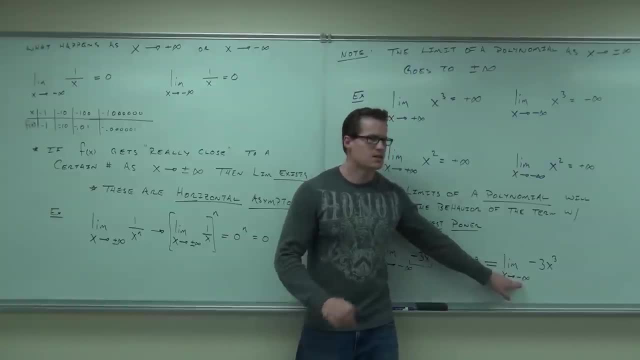 Take, we're going to negative infinity, mind you. Take and do this. Negative means negative, right, It means a negative number. Take a negative number, plug it in here. What do you get out? Negative minus 3.. And then multiply it by negative 3.. 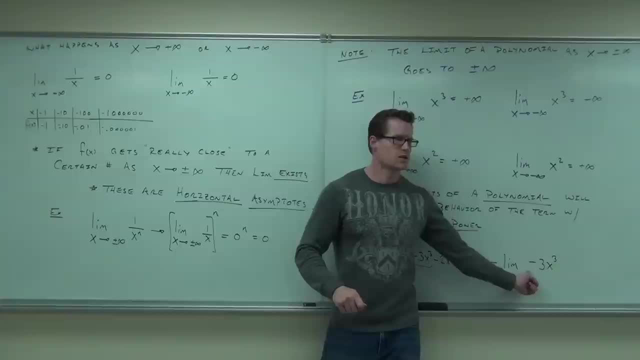 What do you get? a positive or negative? Positive, That's a positive. So, as we're approaching negative infinity, that approaches positive infinity. It's a polynomial. We'll go to one infinity. Let me do this one more time so you really catch the song. 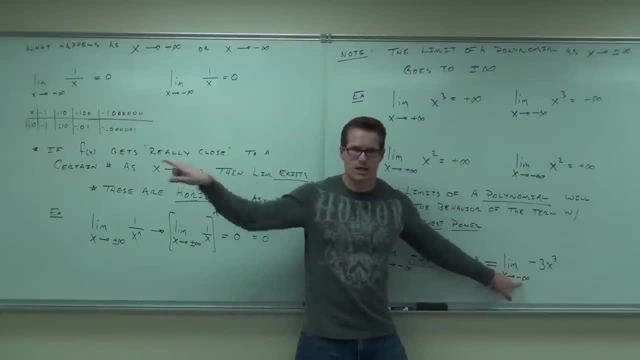 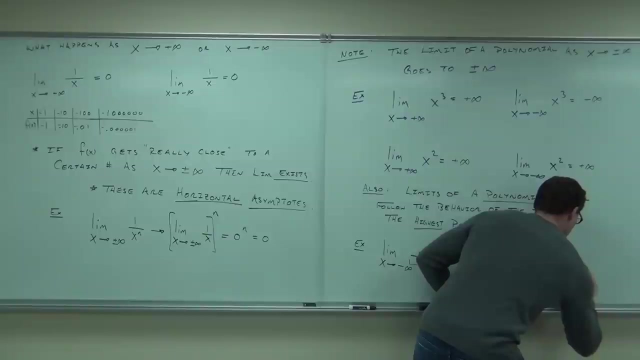 You're talking about going to really negative numbers, right, Really negative. Plug in negative numbers to that. You're going to get out negative numbers, right, But then you're multiplying it by negative 3, which makes them positive numbers. That's positive infinity. 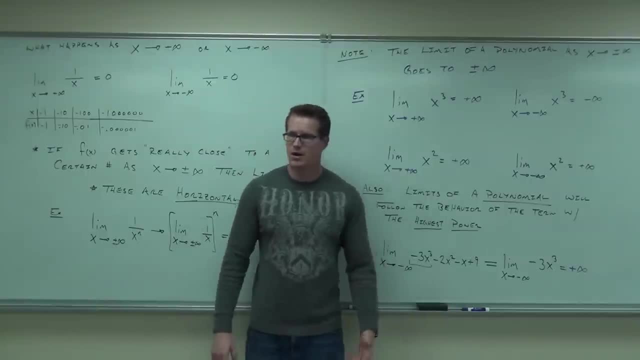 Think about negative x cubed. If you think about negative x cubed, it looks like this, doesn't it About like that? Let's see if I can move my arms a little bit There. It looks about like that. I think you're doing dance, dance revolution, or something. 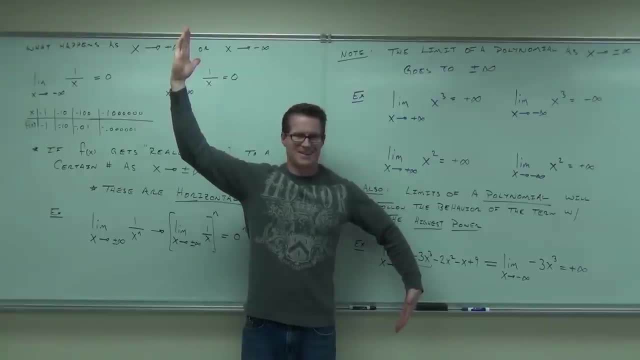 It's this: As you go left, it goes higher, doesn't it? As you go right, it goes low. That's what this is saying. That's what it's saying. How many people feel okay with that one? I'm not trying to show limits here. 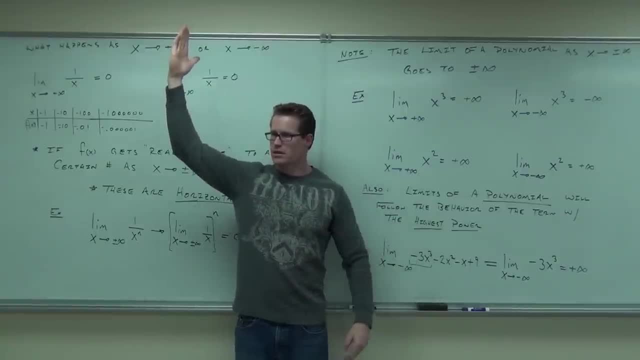 I'm just asking: Okay, Now we're going to start using these ideas that we've been talking about. We're going to start using these ideas that we've been talking about? We're going to start using these ideas that we've been talking about? 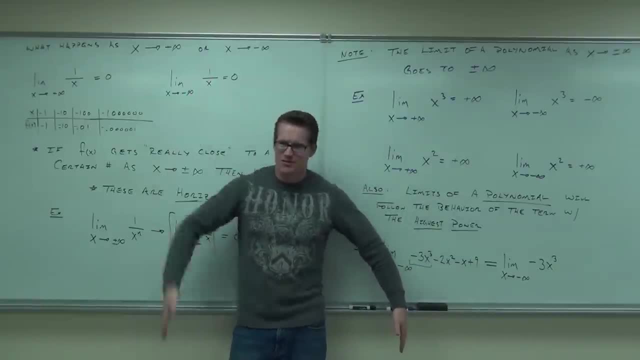 No, I'm doing what Nancy needs: Negative x, cubed. negative x to the 4th, negative x to the 5th, negative x to the 6th. it's going to do that right. You know that intuitively. 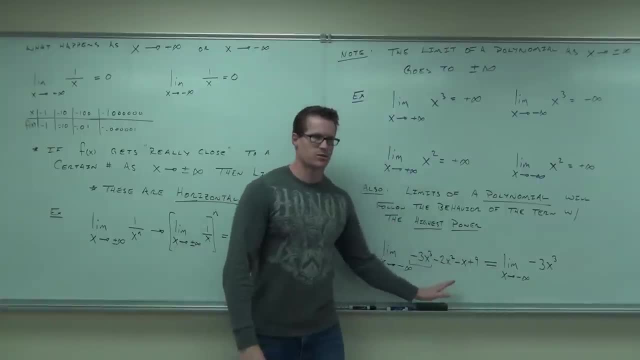 It follows that leading term. All the rest of this is garbage. as far as the limit's concerned, really, when you're talking about infinity, Now, normal limits, no, it's not garbage, but for infinity, that's the one that matters. 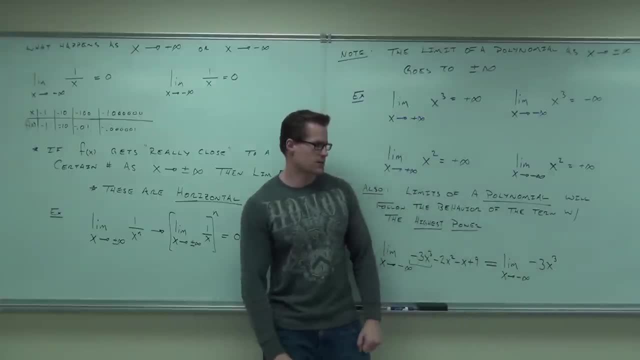 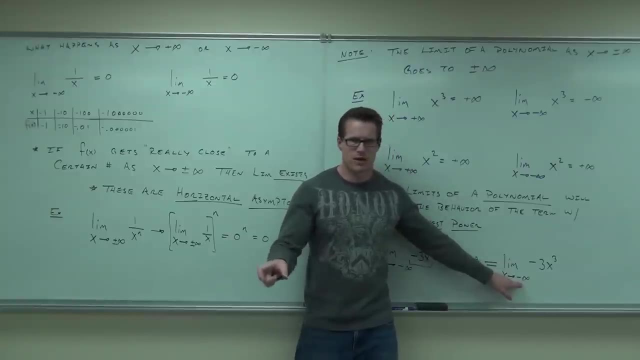 So consider the leading term, that negative 3x to the 3rd. Take we're going to negative infinity, mind you. Take and do this. Negative means negative, right, It means a negative number. Take a negative number, plug it in here. 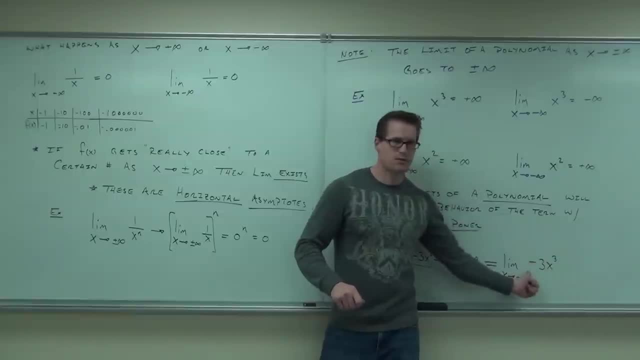 What do you get out? And then multiply it by negative 3. What do you get? a positive or negative? That's a positive. So, as we're approaching negative infinity, that approaches positive infinity. It's a polynomial. We'll go to one infinity. 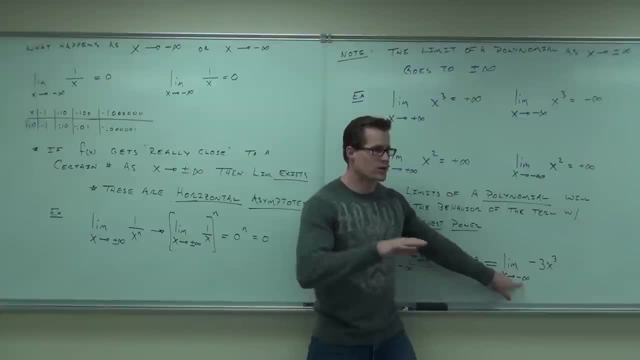 Let me do this one more time so you really catch the song. You're talking about going to really negative numbers, right, Really negative- Plug in negative numbers to that. you're going to get out negative numbers, right, But then you multiply it by negative 3, which makes them positive numbers. 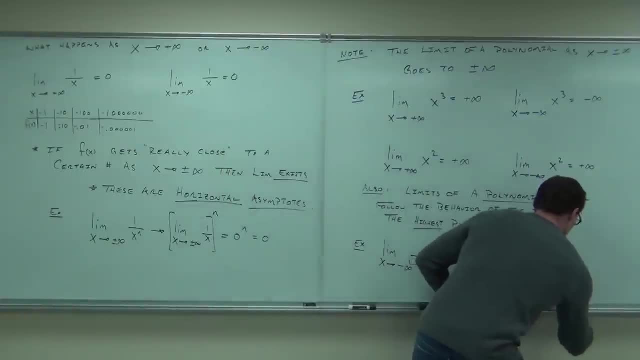 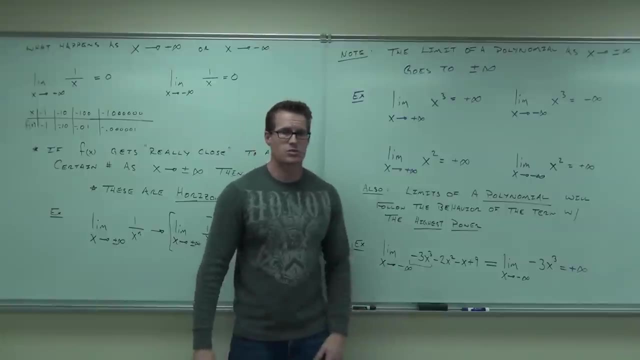 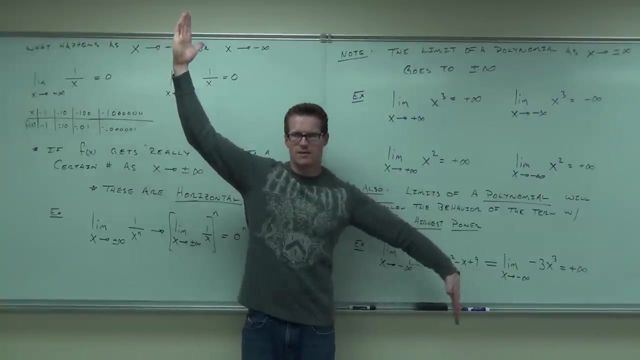 That's positive infinity. Think about negative x cubed. If you think about negative x cubed, it looks like this, doesn't it About like that? Let's see if I can move my arm a little bit there. It looks about like that. 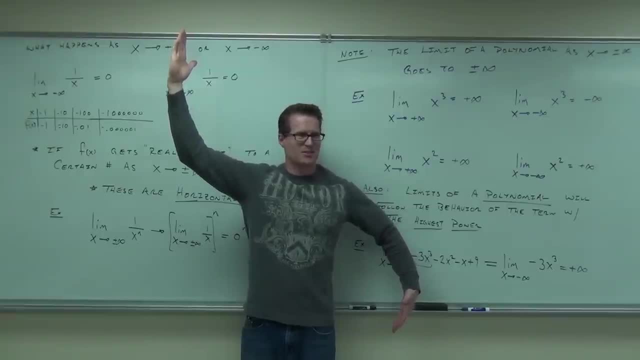 I think you're doing dance, dance revolution or something. It's this: As you go left, it goes higher, doesn't it? As you go right, it goes low. That's what this is saying. That's what it's saying. 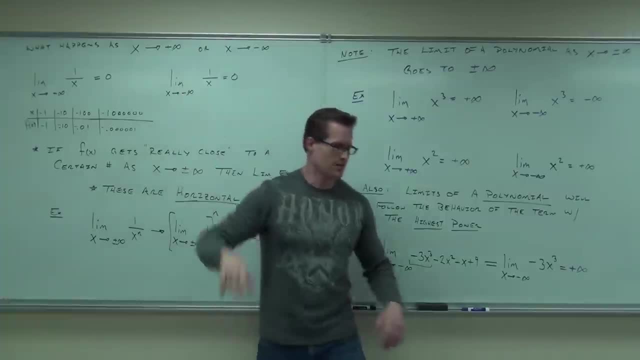 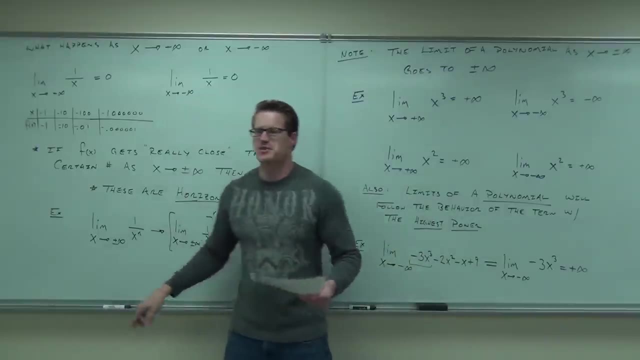 How many people feel okay with that one? I'm not trying to show limits here, I'm just asking: Okay, Now we're going to start using these ideas to actually compute some limits. This is where kind of the fun comes in. 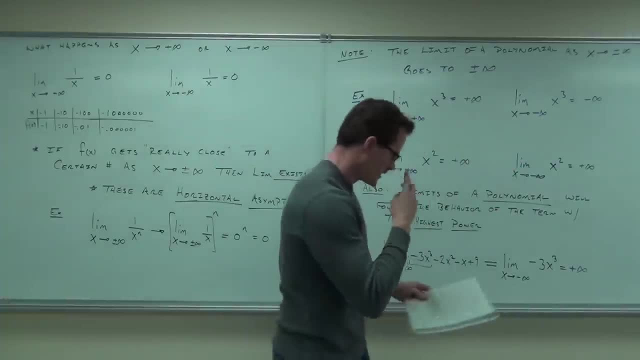 We're going to start using these ideas to actually compute some limits. This is where kind of the fun comes in. We're back to computing limits. Are they hard? Not really, But you need to know not tricks but some mathematical manipulations. 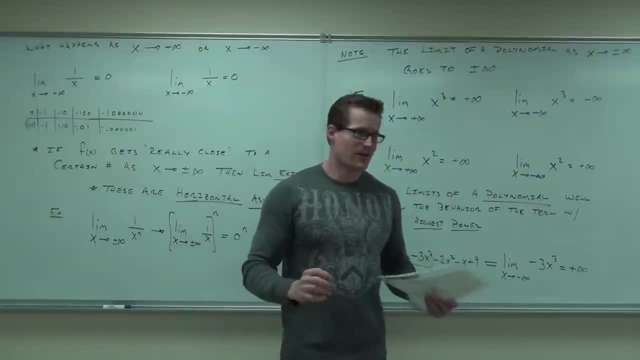 to do them correctly. There's going to be a lot of rationalization, A lot of that. There's going to be a lot of dividing by things. There's a lot of that. Not hard, though. You just got to see it a few times. 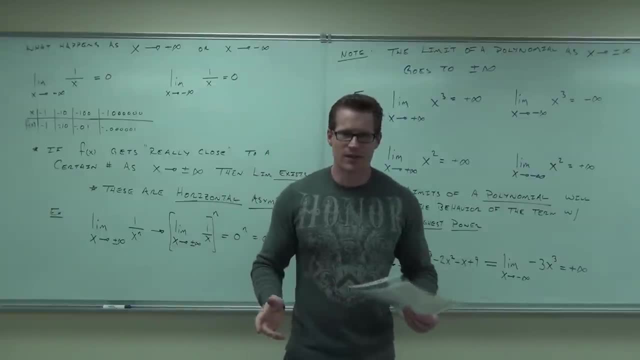 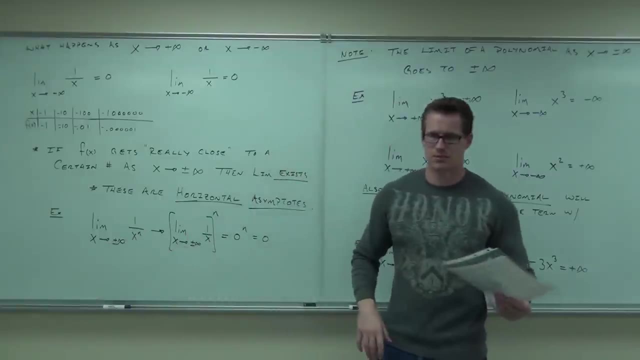 We're back to computing limits. Are they hard? Not really, but you need to know, not tricks but some mathematical manipulations to do them correctly. There's going to be a lot of rationalization, a lot of that. There's going to be a lot of dividing by things. 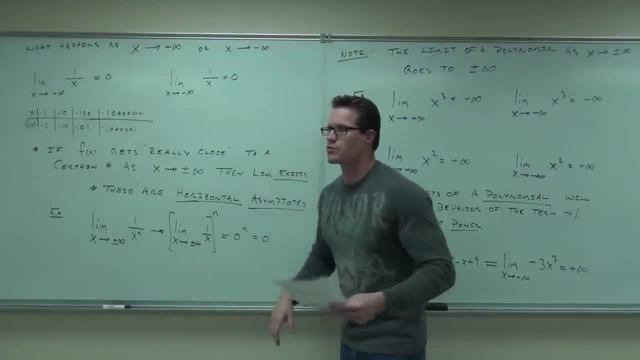 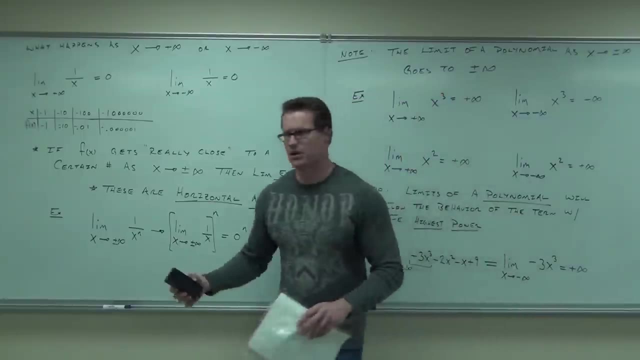 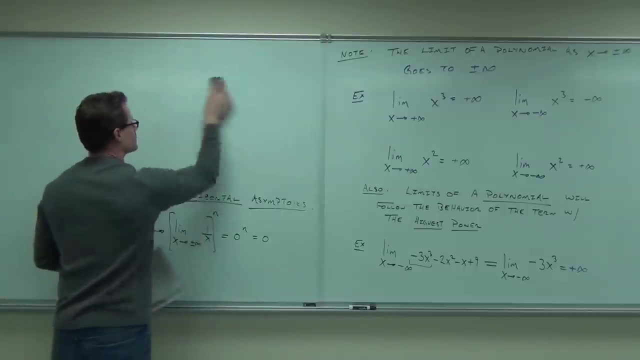 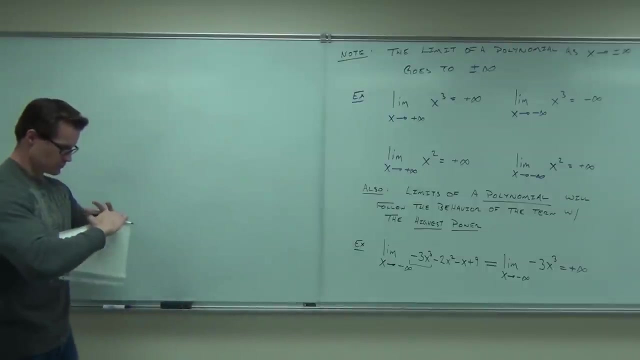 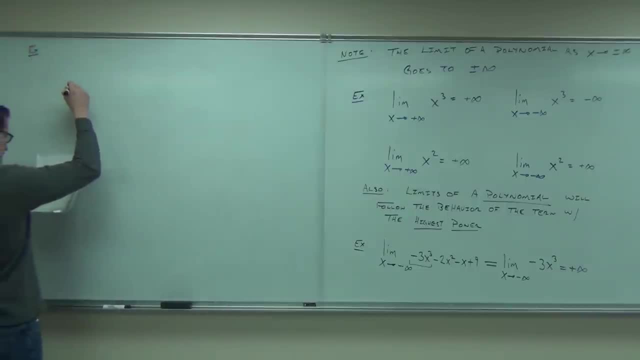 Okay, Okay, Okay Okay, Thank you. All right, All right, Thank you. Thank you, Mr Duke Fucking lick. Hey, Rick, You know you're fromroddehhhh, fique in, Remember about this miss. 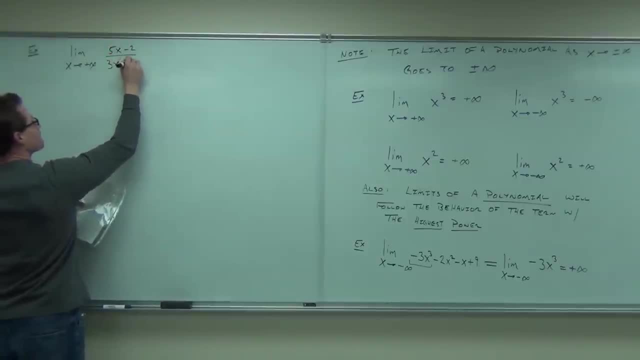 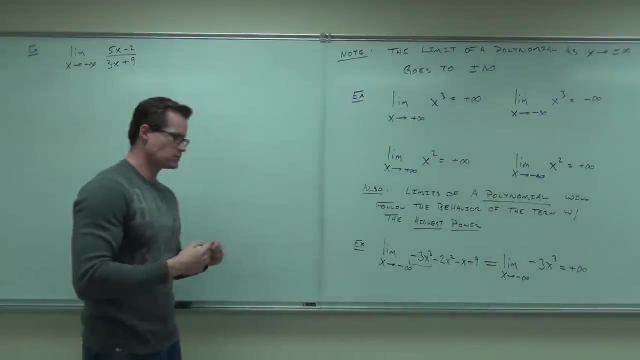 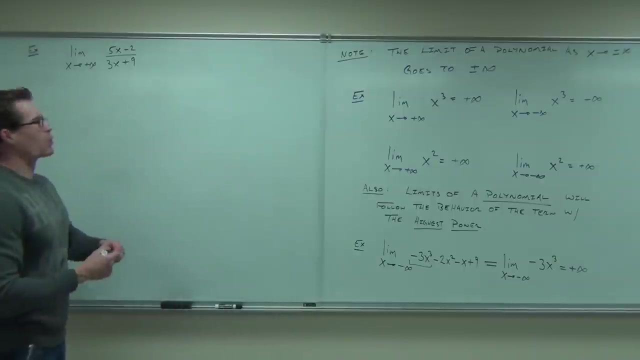 Back in the day when we had after. What about that one? Let's see if we can do that. What about that? Where are we going? Positive infinity- Really big numbers. So plug in positive, What's 5 times positive infinity? 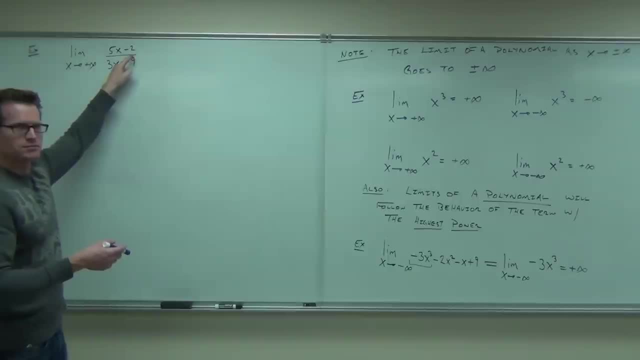 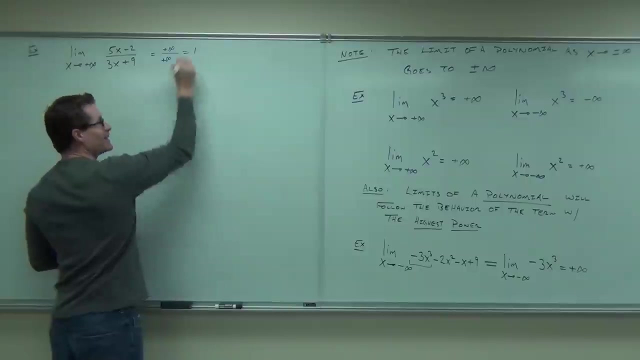 Infinity, Positive right Minus 2. Infinity: What's 3 times infinity Plus 9.. We got you infinity plus 1. What Infinity over infinity? 1. Yes, No, No, you can't do that. 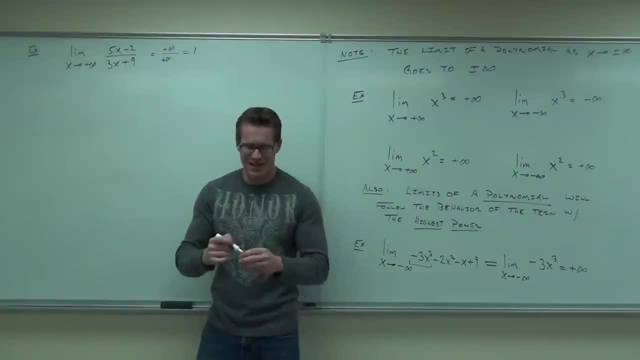 Do you know how big infinity is? Me neither. So how are you supposed to divide it and get 1?? You can't do that, But maybe we can manipulate this in such a way that this stuff is possible. Now, here's the idea. 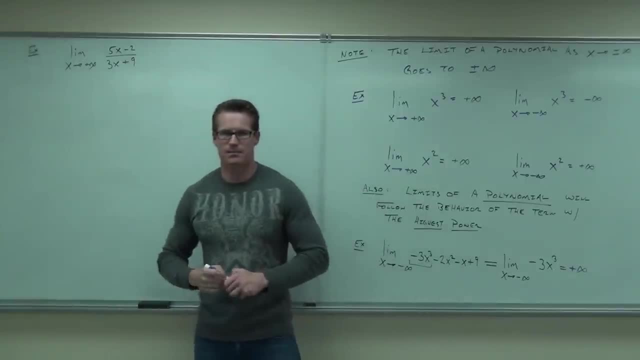 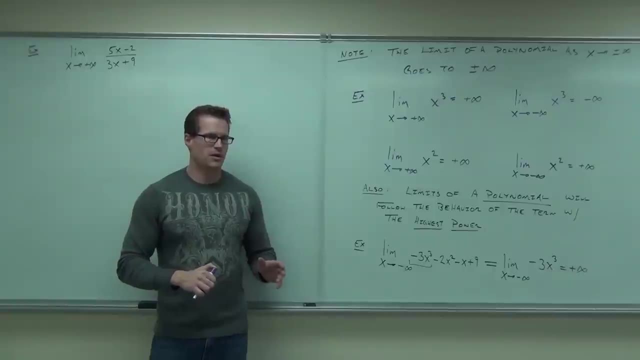 Did you know that you can multiply both the top and the bottom of a fraction by anything that you want? Sure, And if you multiply both the top and the bottom of a fraction by anything you want, it goes to both of those terms, true. 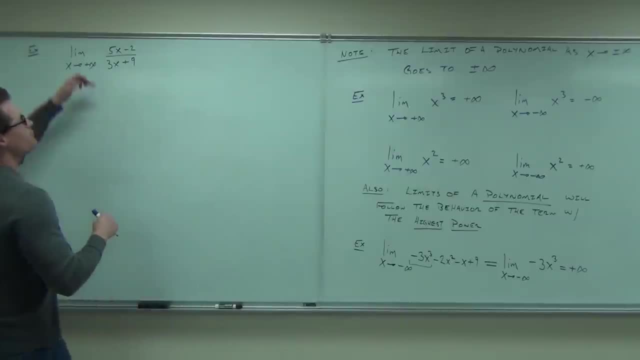 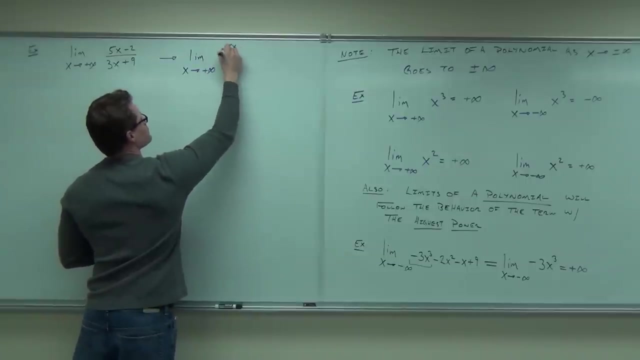 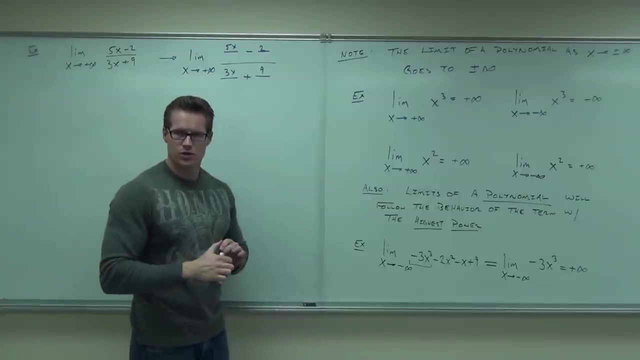 What that says is this: What if I divided every term by x? Could I do it Mathematically? is that legal? Sure? Mathematically that's fine. So 5x minus 2,, 3x plus 9, let's divide all those terms by x. 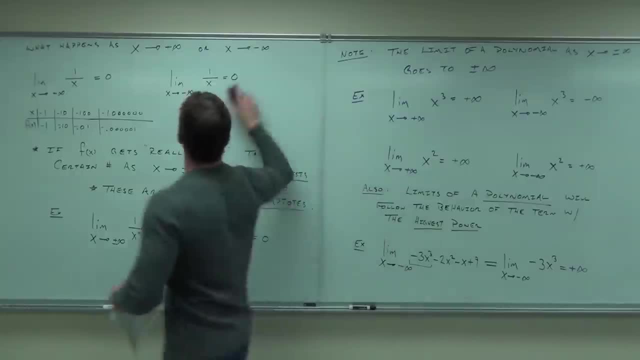 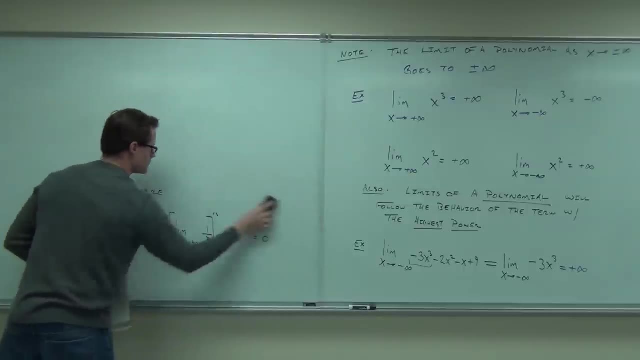 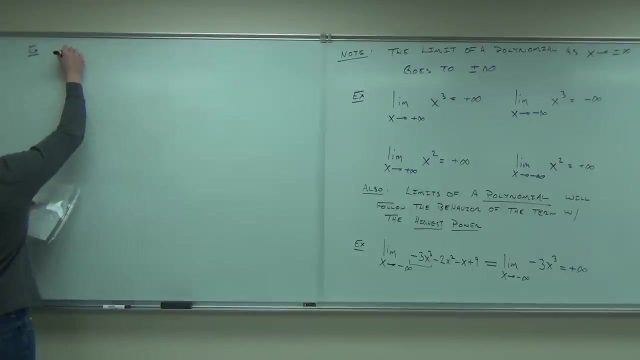 There's a lot of that, Not hard, though. You just got to see it a few times. The 51st one is called the 起來 Wereherth. Like even just luck is there. I could as well do two like these all together. 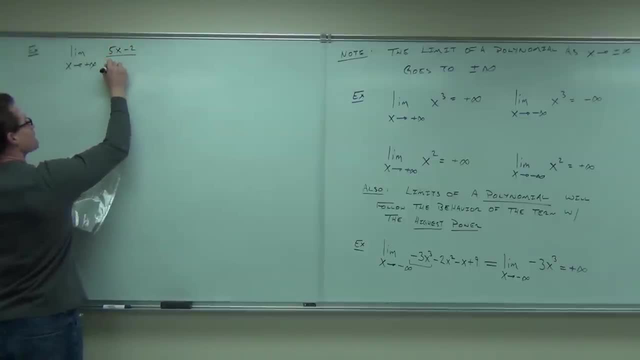 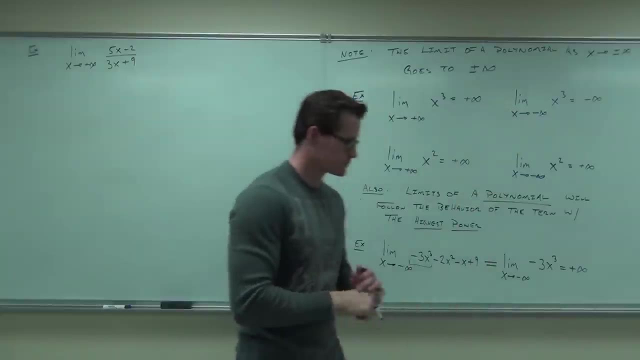 There's a lot of times I would say four, 2x. Okay, I'll do four, three, Three, 2x, Four, 2x, Four, 3x, Three, 4x. What about that one? Let's see if we can do that. 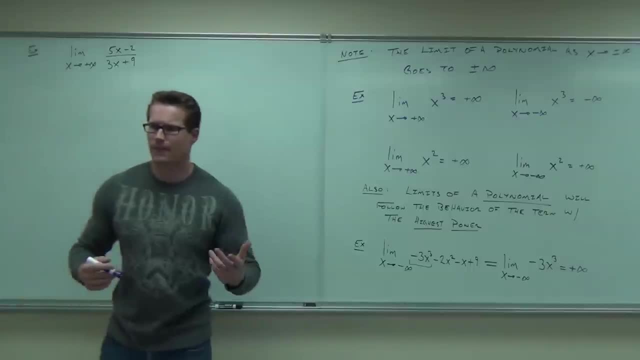 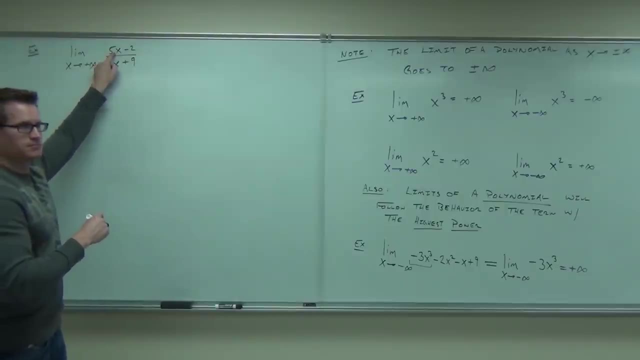 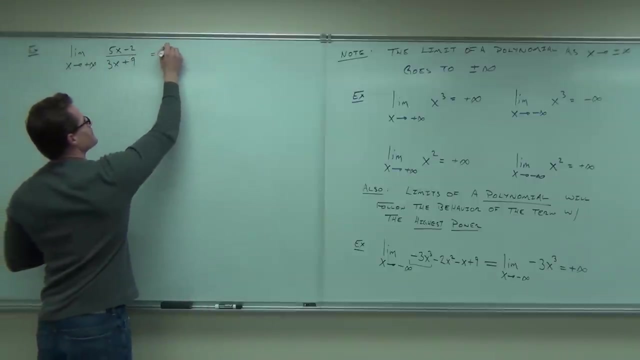 What about that? Where are we going? Positive infinity, Positive infinity- Really big numbers. So plug in positive: what's five times positive infinity. Positive Infinity, Positive right Minus two Positive Infinity: Okay, What's three times infinity? 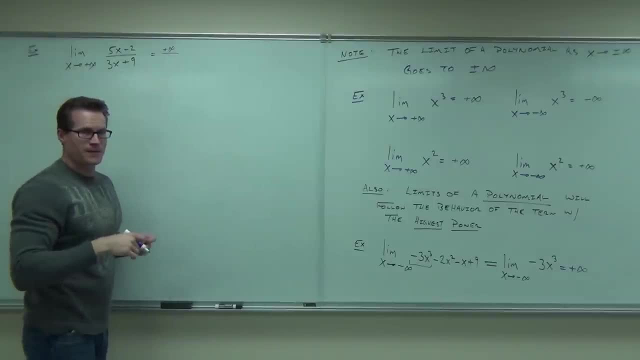 Positive Plus nine, We got you infinity plus one. Ha ha, ha ha. What Infinity over infinity? One, Yes, No, No, You can't do that. Do you know how big infinity is? Me neither, So how are you supposed to divide it and get one? 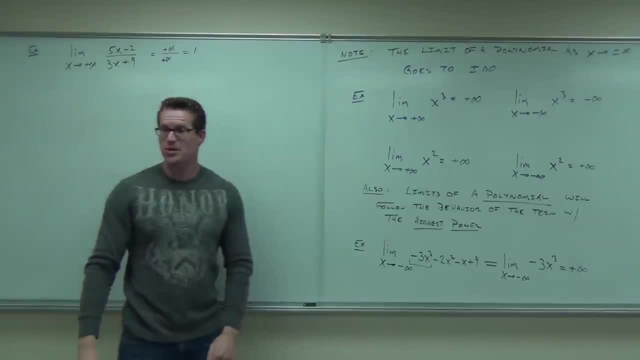 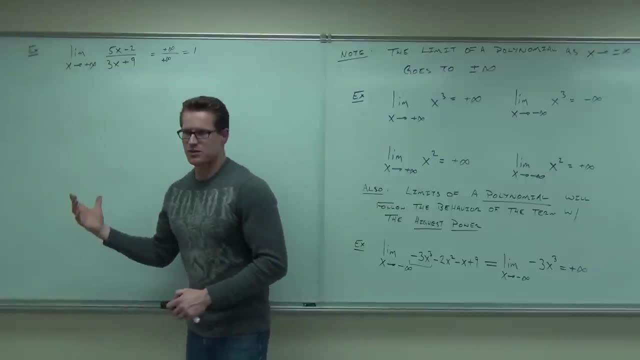 You can't, You can't, You can't. I was thinking one testing will be completely possible, But I'm kind of afraid this stuff is possible. Now here's the idea. Did you know that you can multiply both the top and the bottom of a fraction by anything? 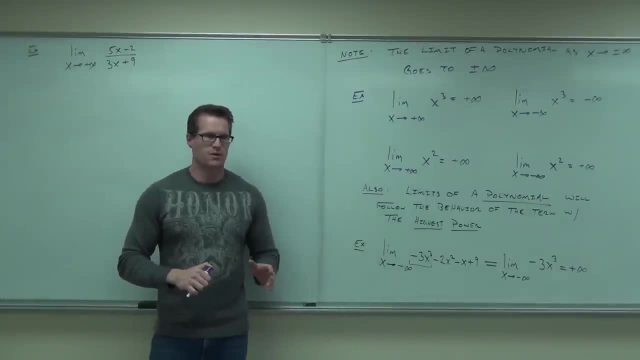 that you want? Sure, And if you multiply both the top and bottom of the fraction by anything you want, it goes to both of those terms true. What that says is this: what, if I divided every term by x, Could I do it? 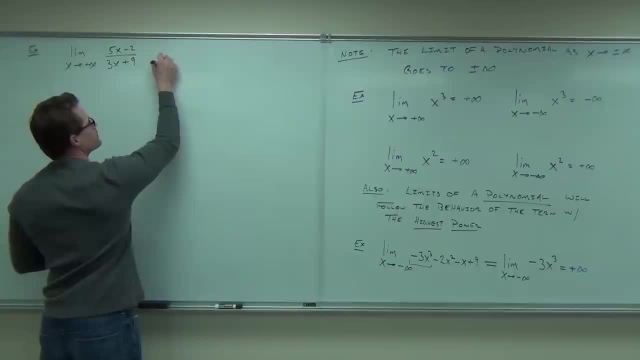 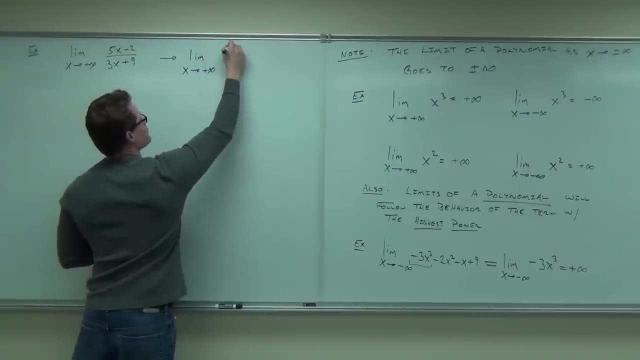 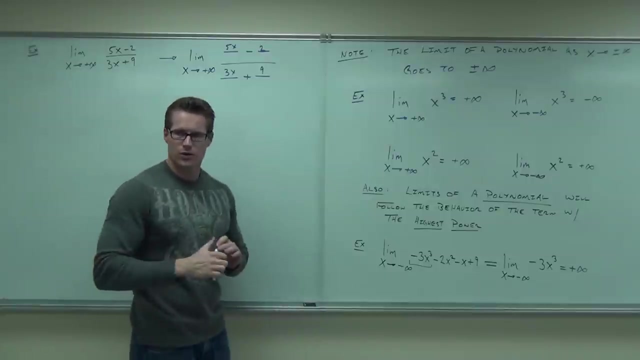 Mathematically is that legal. Sure. mathematically that's fine. Okay, 5x minus 2,, 3x plus 9.. Let's divide all those terms by x. I'll explain where I'm getting the x from in just a minute. 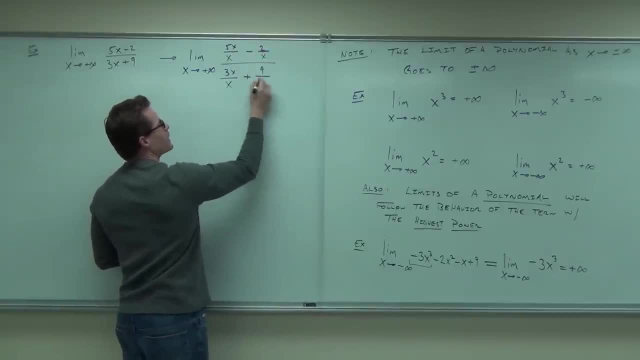 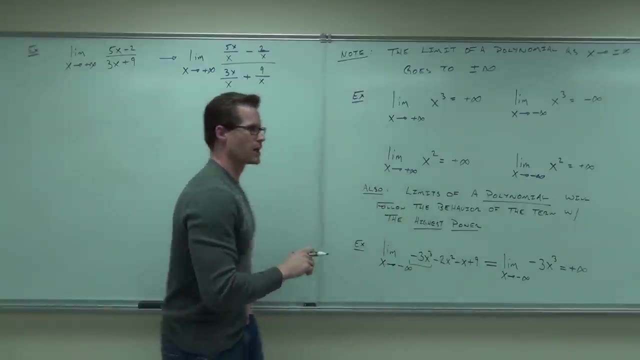 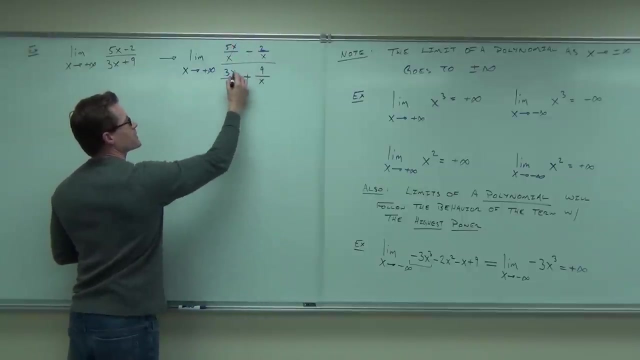 Some of you can probably see it. I'll explain why in a bit. Are you okay with that so far, Are you sure? Okay, Now simplify What happens here. Same thing happens here, right? Do they cancel out or cross out here? 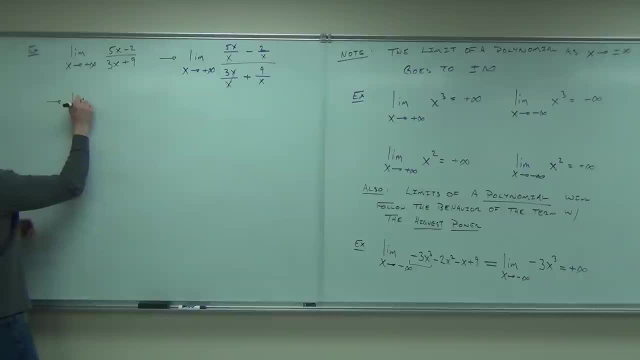 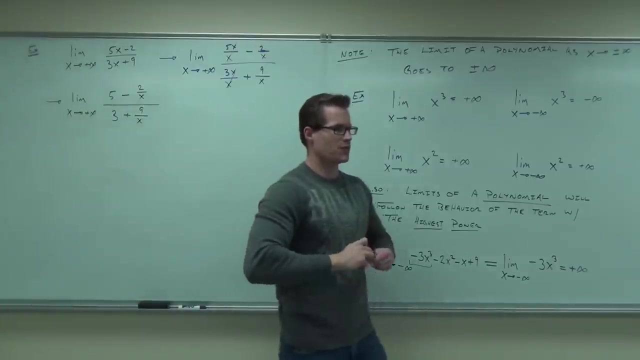 So I get the limit. Okay. This becomes 5 minus 2 over x, 3 plus 9.. 9 over x By a show of hands. how many people can follow that algebra now? Now watch, Let's take x to infinity. 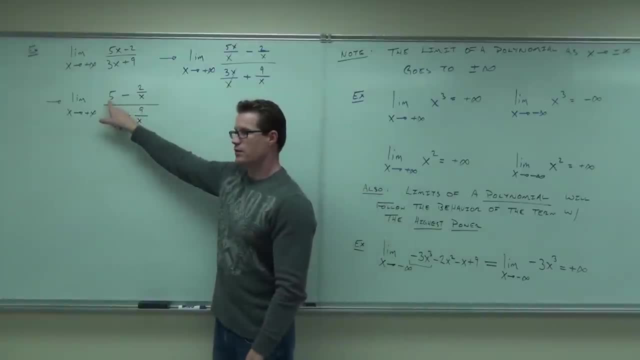 If I take x to infinity, what happens to the 5? It's 5.. Nothing, Nothing. There's no x, It doesn't change at all. The 5 is 5.. What happens to the 3?? Nothing. 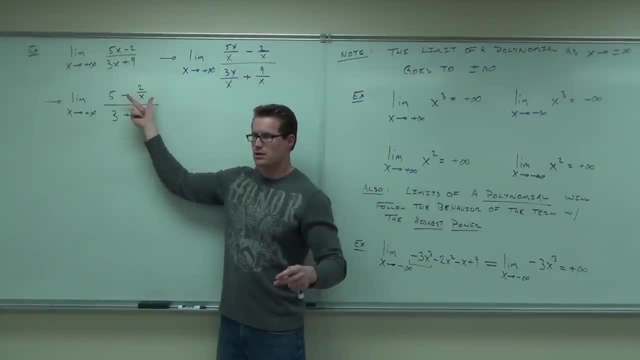 What happens to 2 over x? Really small, Really small, How small, Zero, Zero. Remember the definition of our limit, Our limit said: as we take x approaches infinity. a constant over x is the first thing I gave you today. 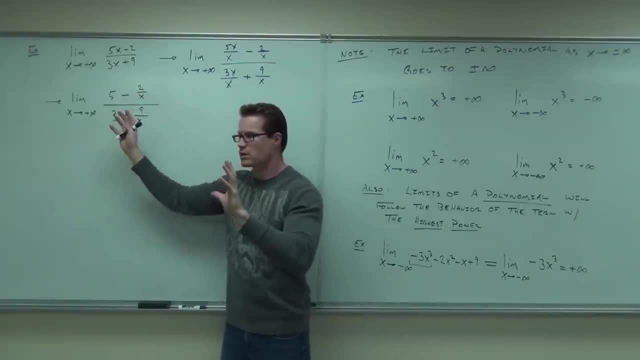 Really the first new thing It said: a constant over x to any power goes to what Zero? That was important. We needed that. This becomes: how much folks, Everybody, How much does this become Constant over infinity? Whether it's positive or negative, it doesn't matter. 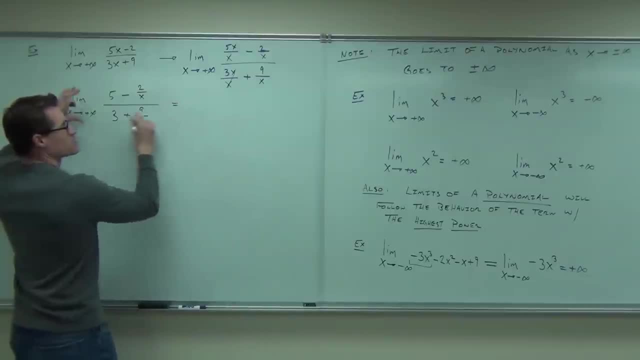 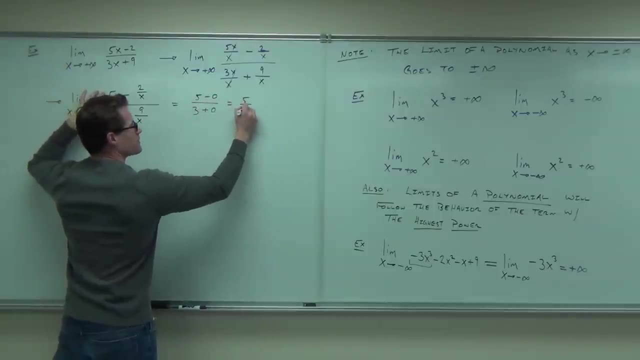 It's going to zero. So what this says is this limit. notice how I'm going to stop right in the limit now. I've written limit till here: 5.. Minus zero over 3 plus zero, That's 5 thirds. 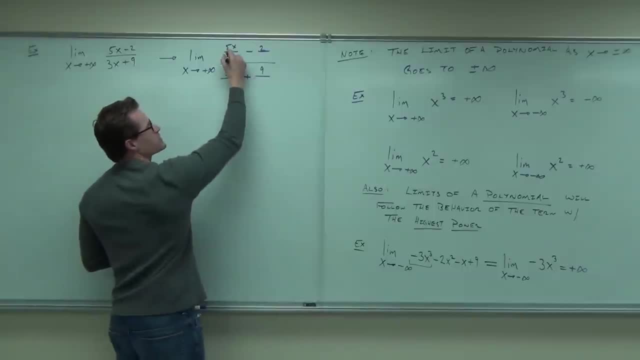 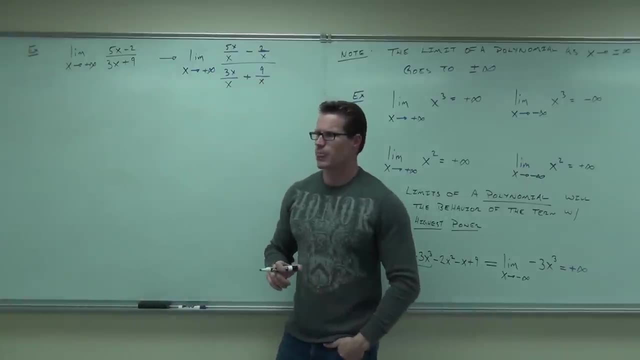 I'll explain where I'm getting the x from in just a minute. Some of you can probably see it. I'll explain why in a bit. You okay with that. so far, You sure Okay. Now simplify it. What happens here? 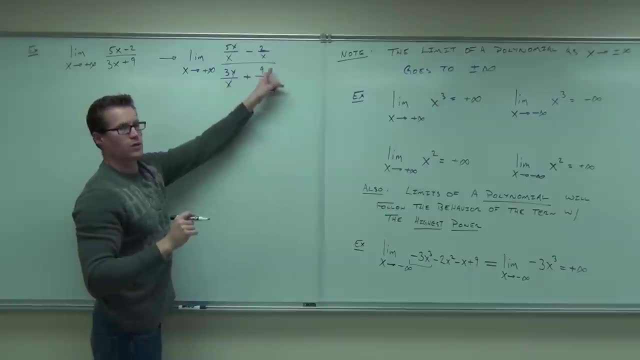 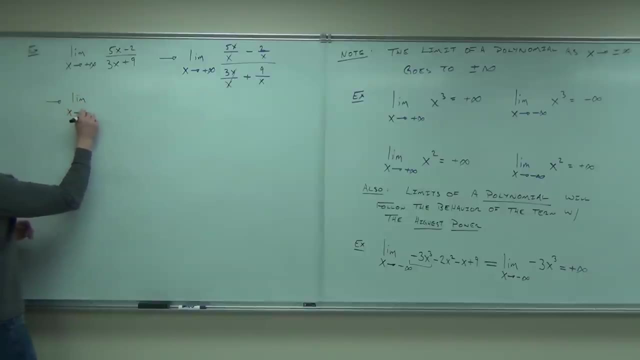 X is canceled. Same thing happens here, right? Do they cancel out or cross out here? No, So I get the limit. This becomes 5 minus 2 over x, 3 plus 9 over x. But a show of hands, how many people can follow that algebra down? 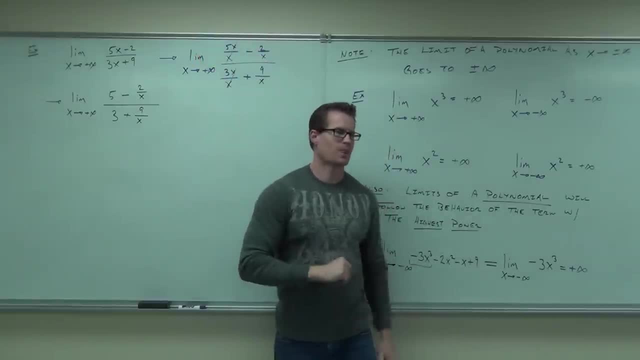 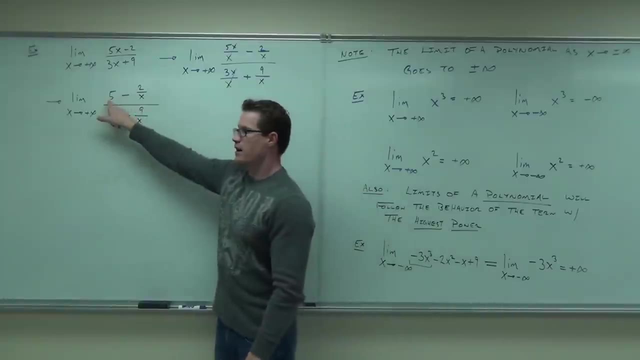 Now, now watch. Let's take x to infinity. If I take x to infinity, what happens to the 5?? Nothing, Nothing. There's no x. It doesn't change at all. The 5 is 5.. What happens to the 3?? 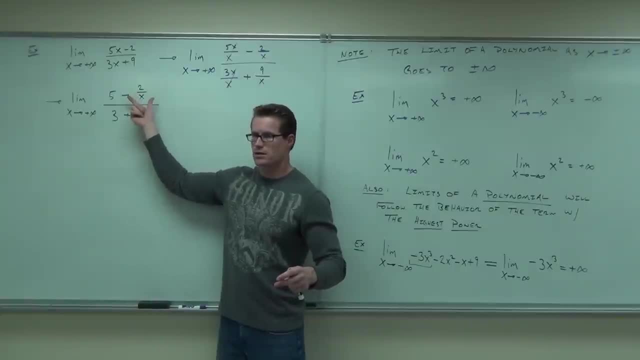 Nothing. What happens to 2 over x? Really small, Really small, How small, Zero, Zero. Remember the definition of our limit, Our limit's set As we take. x approaches infinity. a constant over x is the first thing I gave you today. 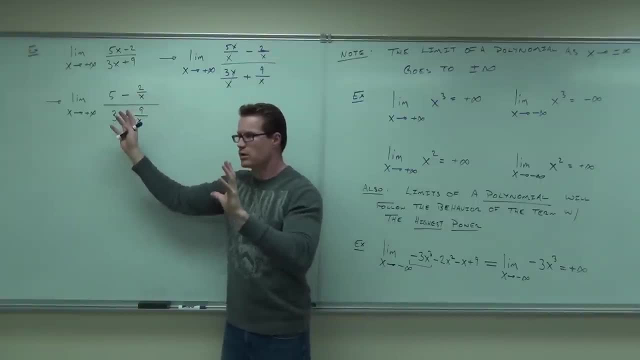 Really, the first new thing is that a constant over x to any power goes to what Zero? That was important. We needed that. This becomes. how much folks, Everybody, Zero. How much has this become Zero? 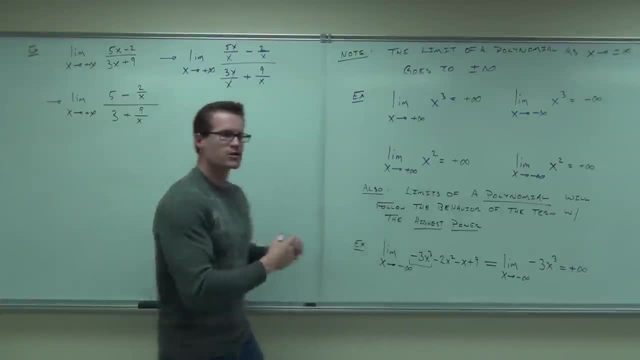 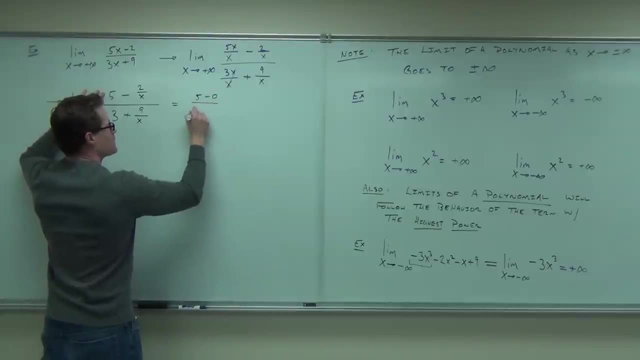 Constant over infinity. Whether it's positive or negative, it doesn't matter, It's going to zero. So what this says is this limit. notice how I'm going to stop right in the limit now. I wrote in the limit tail here: 5 minus 0 over 3 plus 0, that's 5 thirds. 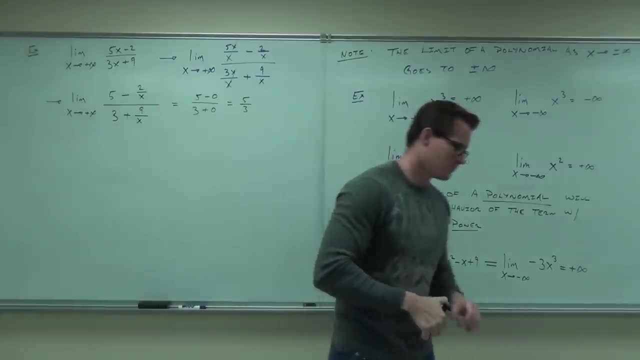 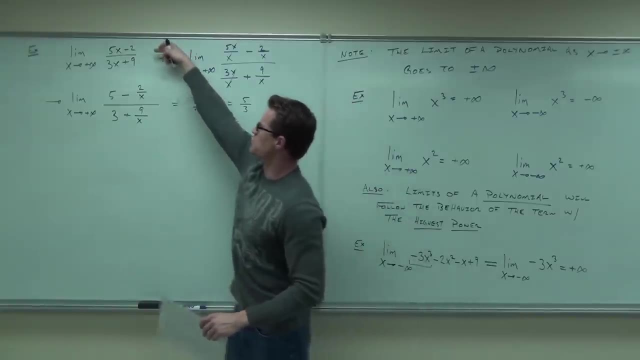 Not 1,, 5 thirds? Now, is it coincidental? is it coincidental that, by the way this works, because you do 1 over x over 1 over x? Do you guys see what I'm talking about there? 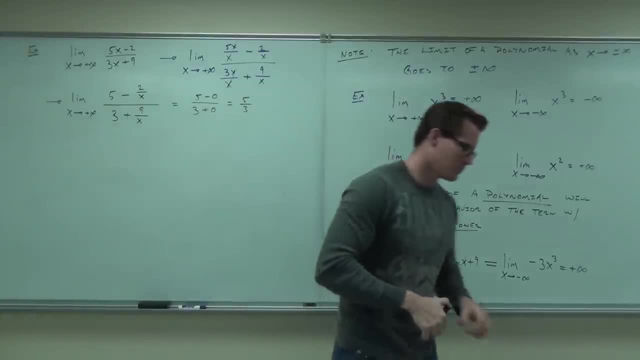 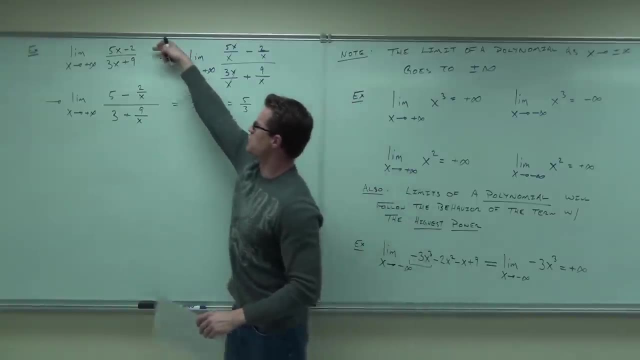 Not 1. 5 thirds. Now, is it coincidental? is it coincidental that, by the way, this works because you do 1 over x over 1 over x? Do you guys see what I'm talking about there? 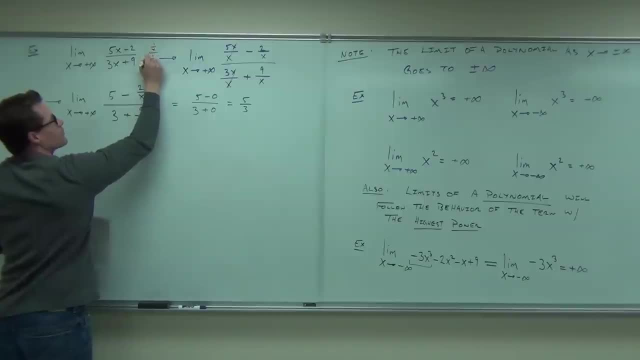 What I really did mathematically was this: over that, Do you see it? 1 over x, over 1 over x. And I distributed and I basically divided every term by x, And that's the mathematical way you'd show that. 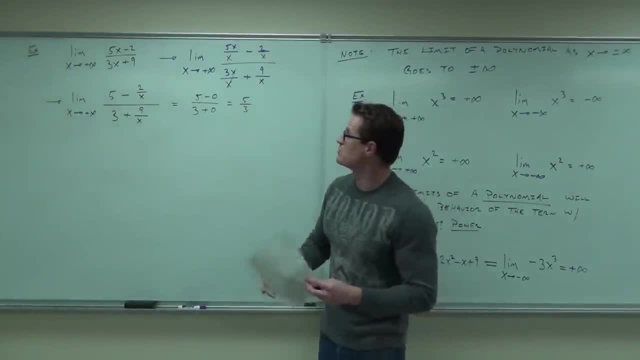 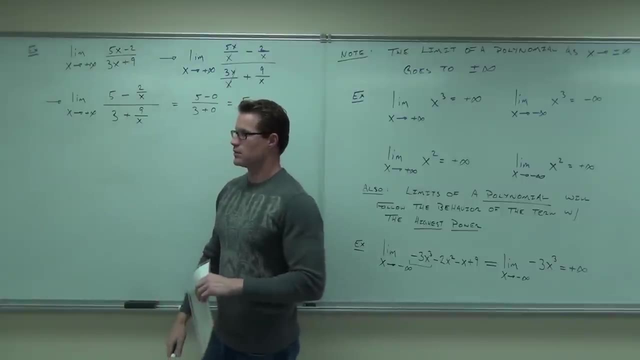 Look at the first, look at the first expression, The limit. So 5x minus 2 over 3x plus 9.. What's the leading term here? 5x is the leading term. What's the leading term here? 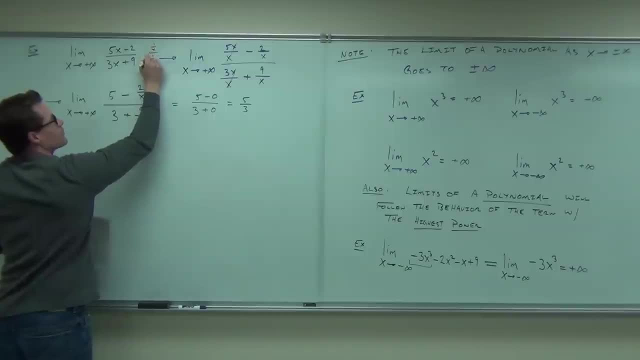 What I really did mathematically was this: over that, Do you see it? 1 over x, over 1 over x. And I distributed and I basically divided every term by x, And that's the mathematical way you'd show that. Look at the first, look at the first expression. 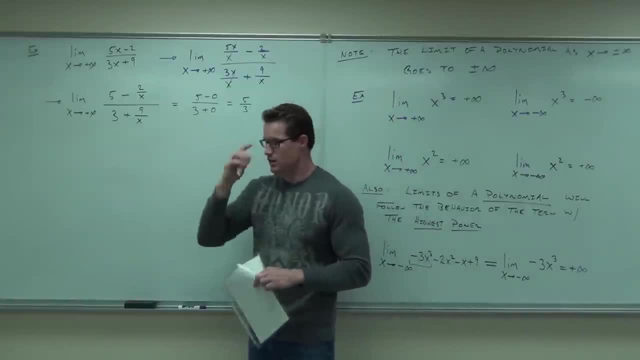 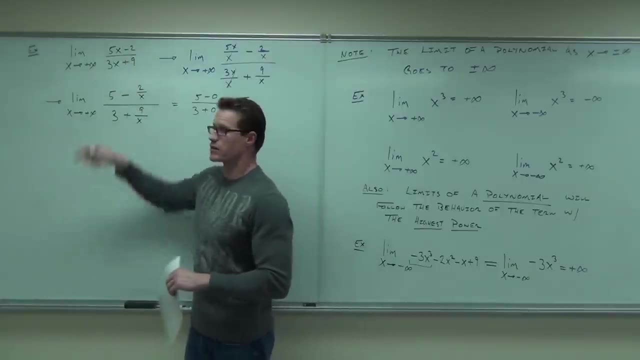 the limit of 5x minus 2 over 3x plus 9.. What's the leading term here? 5x? 5x is the leading term. What's the leading term here? 3. What are the coefficients? 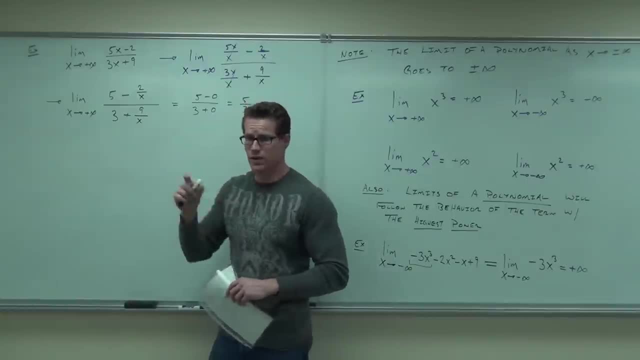 5 and 3.. Do you see that when I divide- excuse me, when I divide by that x, I'm going to get 5 thirds. Everything else is going to go to zero. So the lead, those are polynomials. 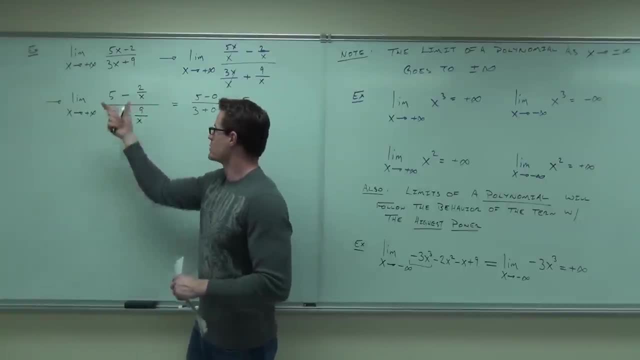 The leading term is all that really matters for us. for that, Now I'm going to go to the next one. Now, do you have to show it? Yeah, I'd like you to show it for right now. okay, As you're going on, you know later in math class. 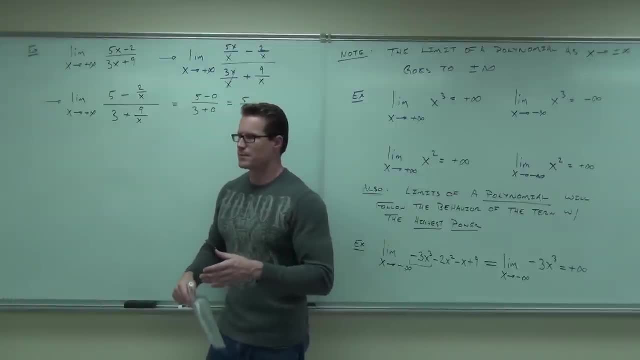 there's no problem. but show me that. Where are you getting the x from? It's not the common x here. You're actually only looking at the denominator, And what you're going to do is divide every term by the largest power of x in the denominator. 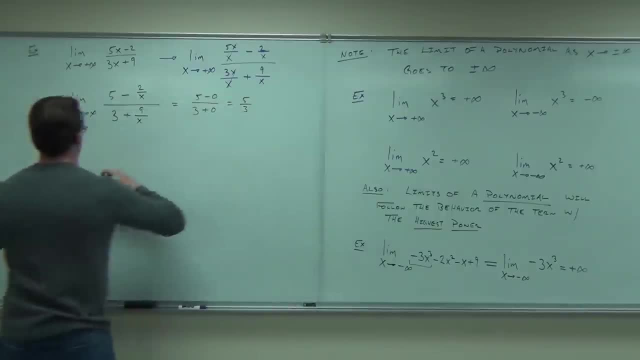 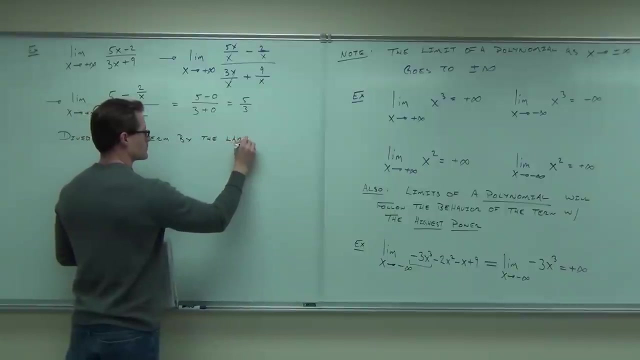 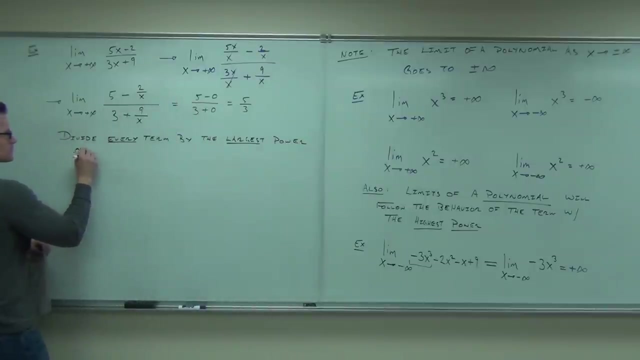 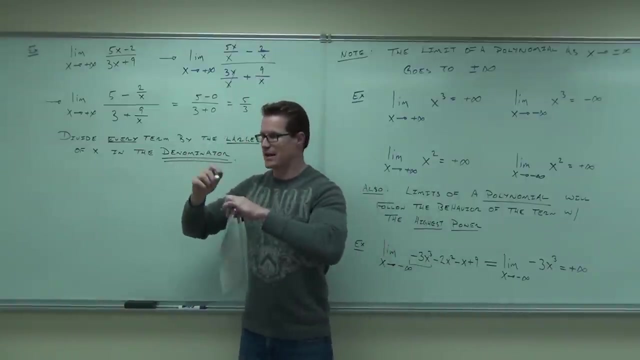 You should probably write that down. Okay, Now why not the numerator? Well, think about it. If your, if your exponents don't exactly match up, then you start dividing by the 162,000.. You're going to find that it's the reaction ratio will go up by one half of the denominator. 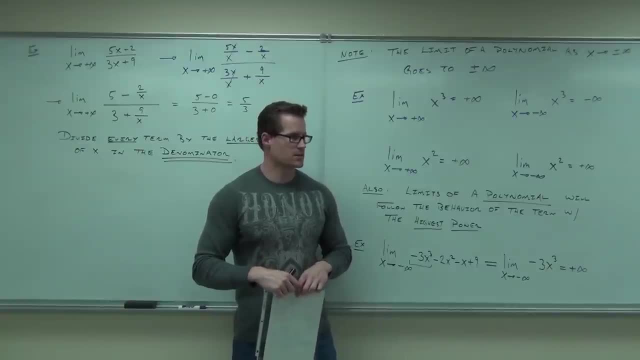 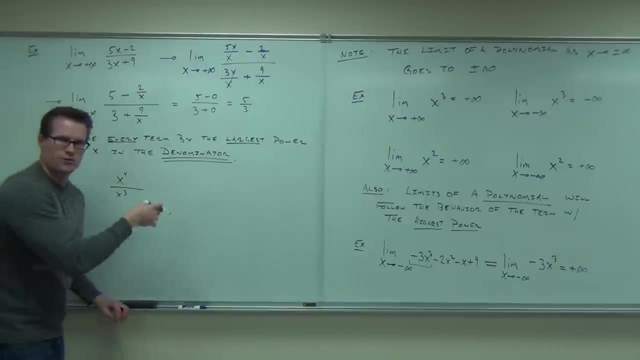 in the numerator, you could have a lot of undefined things. Does that make sense? For instance, if you had this x to the fourth over x cubed and you divide it by x to the fourth, you'd have other stuff here. 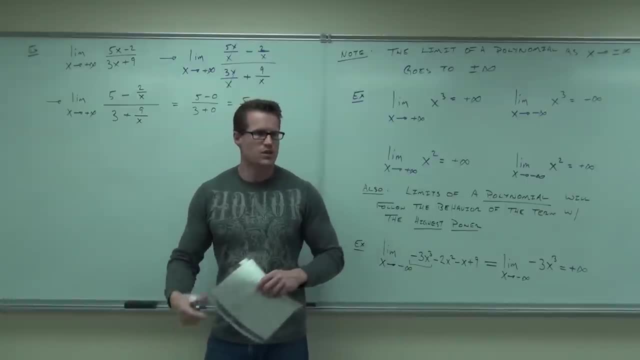 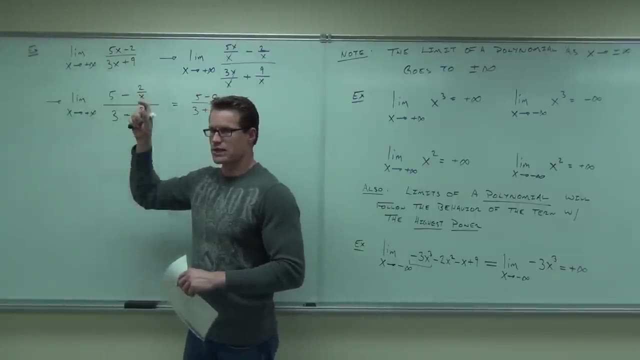 3.. What are the coefficients? 5 and 3.. Do you see that when I divide- excuse me, when I divide by that x, I'm going to get 5 thirds. Everything else is going to go to zero. So the lead, those are polynomials. 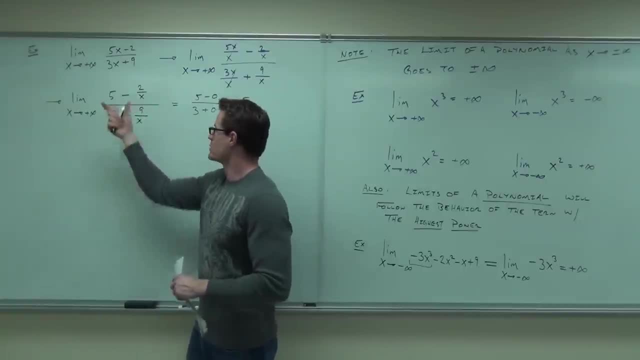 The leading term is all that really matters for us. for that, Now, do you have to show it? Yeah, I'd like you to show it for right now. OK, As you're going on, you know later, Math class is no problem. 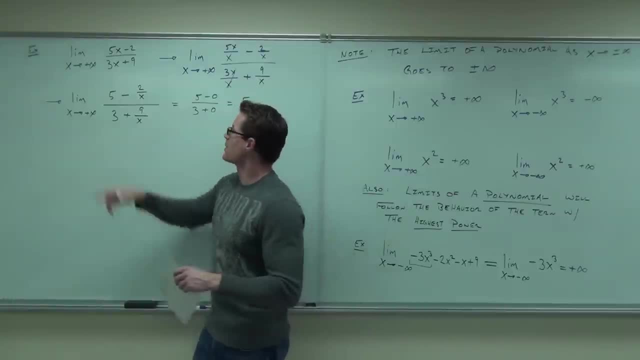 But show me that. Where are you getting x from? It's not the common x here. You're actually only looking at the denominator, And what you're going to do is divide every term by the largest power of x in the denominator. You should probably write that down. 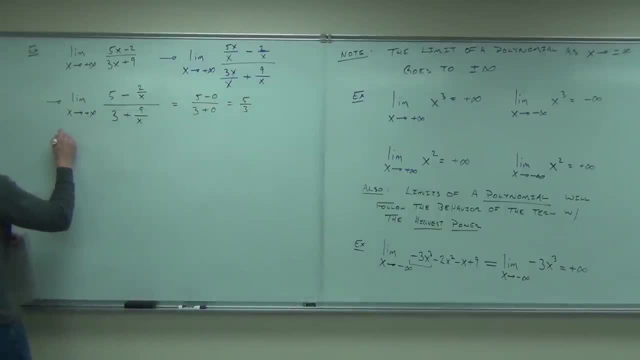 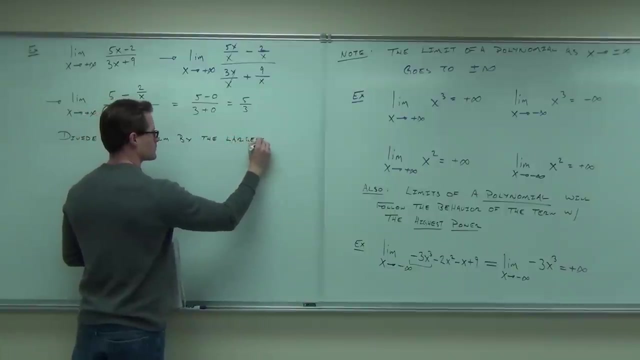 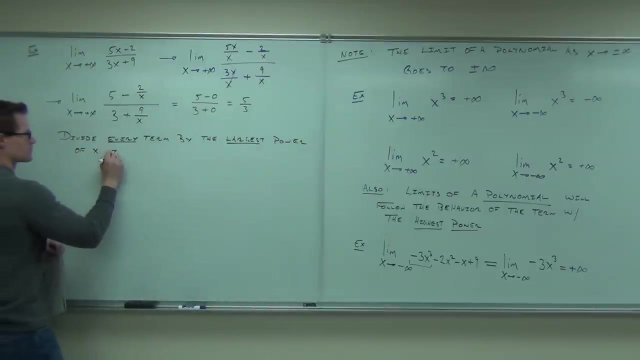 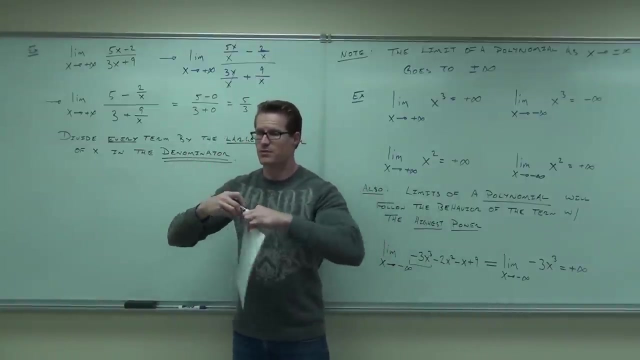 OK, Thank you. Now why not the numerator? Well, think about it. If your exponents don't exactly match up and you start dividing by the largest power in the numerator, you could have a lot of undefined things. Does that make sense? 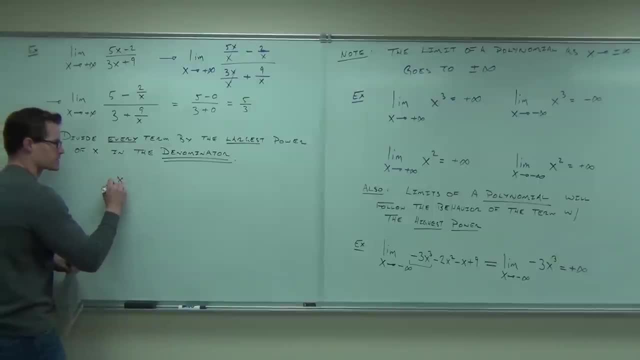 For instance, if you had this x to the fourth over x cubed and you divide it by x to the fourth, you'd have other stuff here. but if you divide it by x to the fourth, that's undefined. That's one over x. 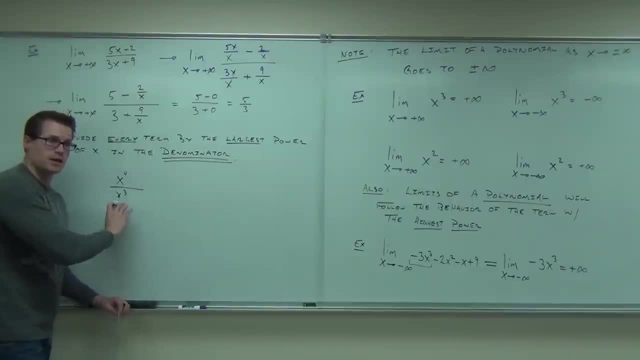 That's a bad thing. So it's always by the largest power in the denominator. That way you won't be undefined. You might be going too far. You might be going to infinity because you won't be undefined. Does that make sense to you? 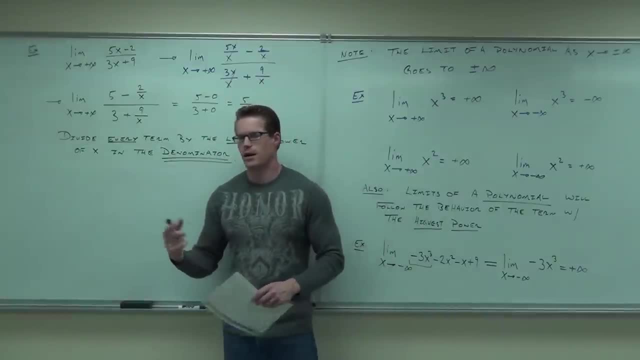 Okay, Another way people like to say this. I'm not going to write it down, It's a shortcut, But if your powers are equal to each other, you're going to the coefficient over the coefficient. That's what we have here. 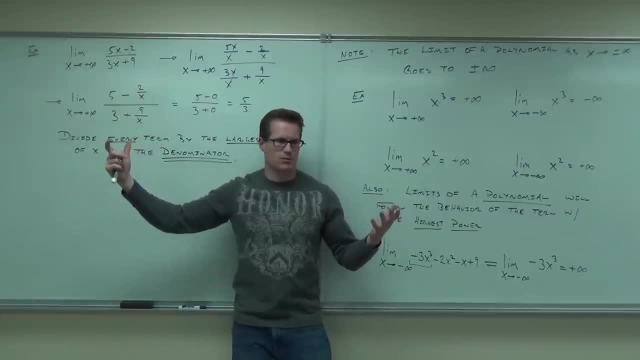 But you can see that that's going to work right. x squared over x squared, x cubed over x, no problem. So if the power is larger on the numerator than the denominator, well, you divide by this power. this is still going to have an x up there somewhere, right? 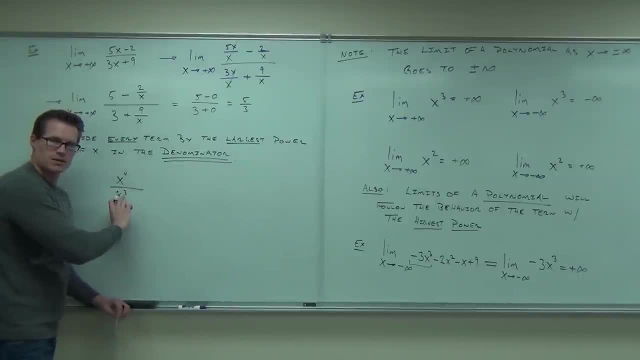 but if you divide it by x to the fourth, that's undefined. That's one over x. that's a bad thing. So it's always by the largest power in the denominator. That way you won't be undefined. you might be going to infinity. 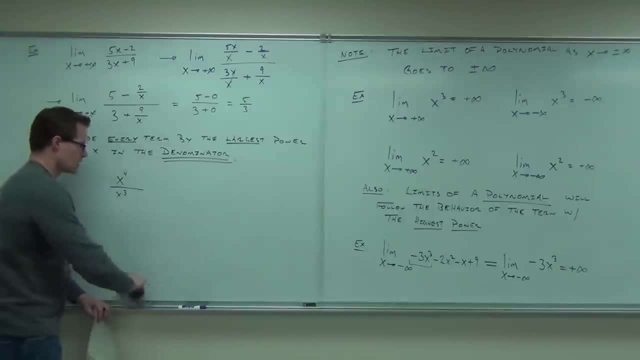 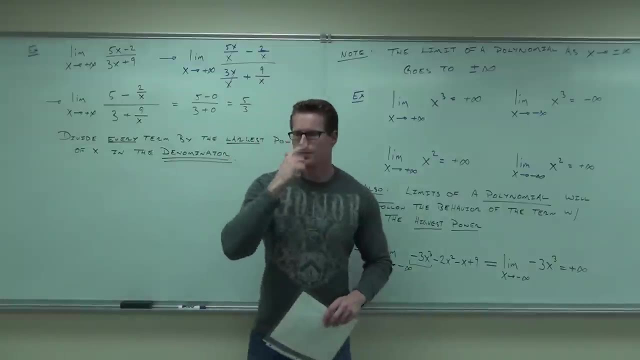 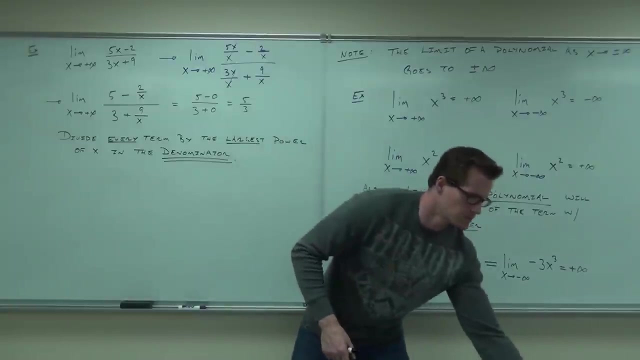 but you won't be undefined. Does that make sense to you? Okay, another way people like to say this. I'm not gonna write it down, it's a shortcut. but if your powers are equal to each other, you're going to the coefficient over the coefficient. 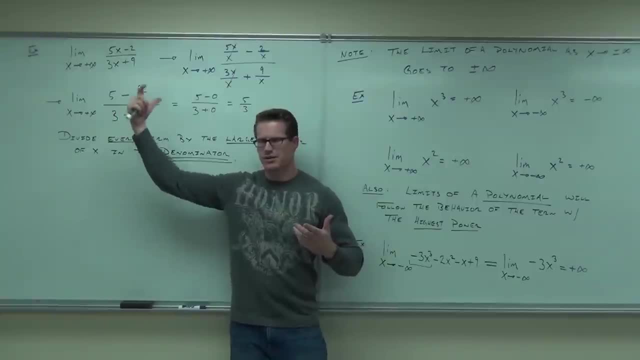 That's what we have here, But you can see that that's gonna work right. X squared over x squared, x cubed over x. no problem, If your power is larger on the numerator than the denominator. well, you divide by this power. 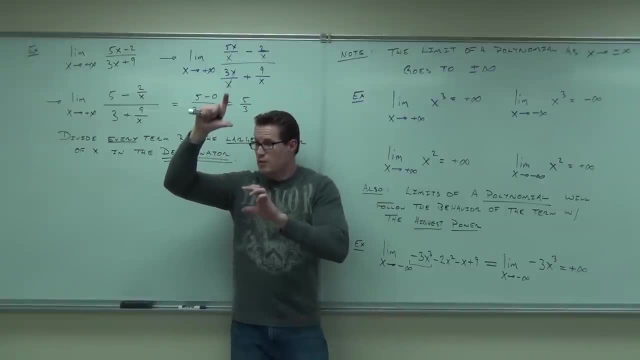 this is still gonna have an x up there somewhere. right, That's infinity. It's gonna be a positive or negative infinity. If this one is larger than- I'm sorry, smaller than this one, if this one's larger, well then you're gonna be going. 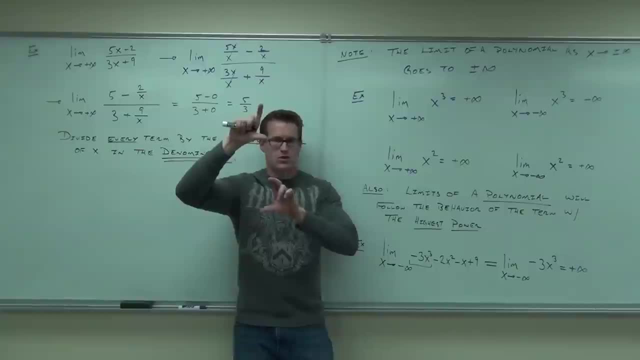 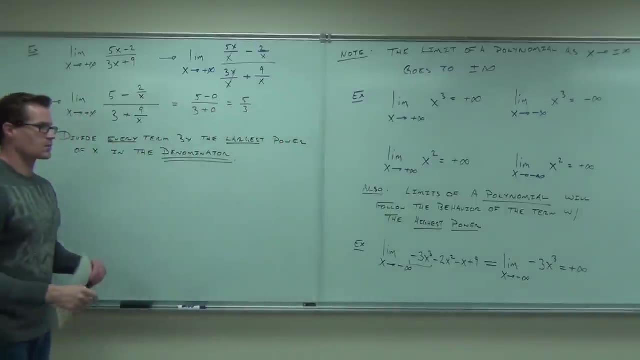 to zero, because you divide by this one. no x's here, x here, you're going to zero. That's one way you can look at that as well. So if the top still has an x, you're going to go to infinity. 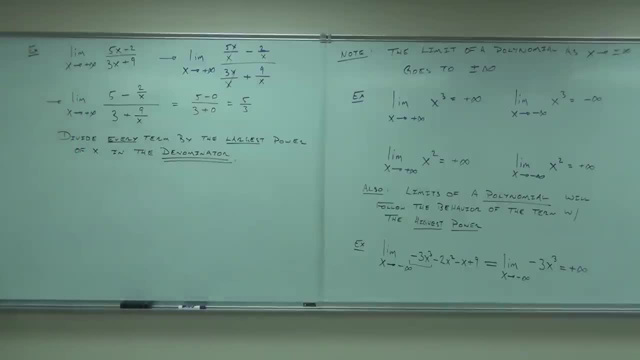 Of course, Let's try a couple more. You're gonna start seeing this very easily. It's not gonna be something super duper hard. Well, it's gonna be super duper hard is when we combine this with some other ideas in a little while. 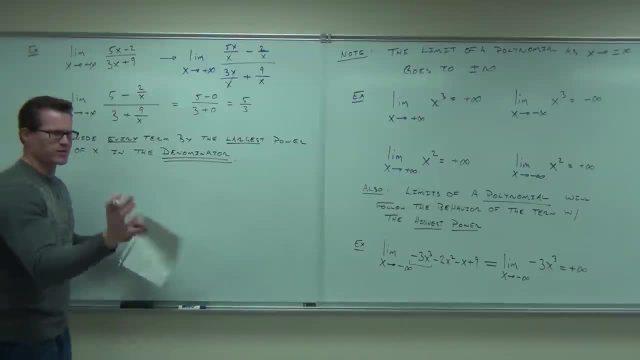 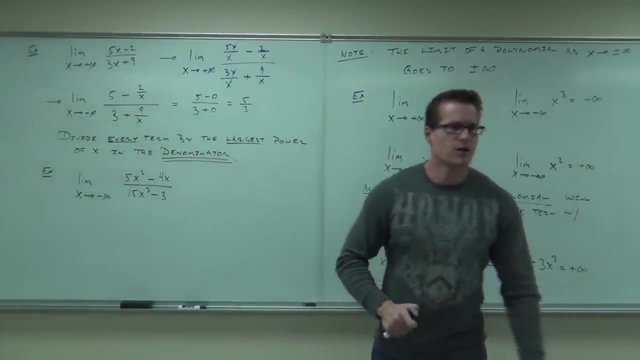 Actually it might be super duper hard then. just super hard, Not even the duper. Don't worry about the duper, Come on, that was funny. Yeah, it was pretty funny, Among others, If you were listening to what I was talking about, 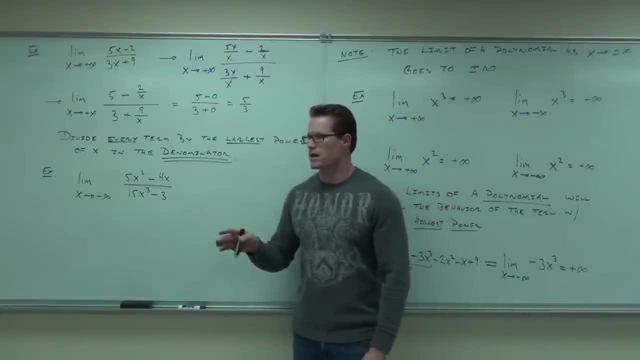 you could probably tell me where this limit is going right off the bat. Zero, Zero, Not 1 third Zero. If the powers matched up, it would: Where's the power the biggest? That means what we're gonna be doing here. 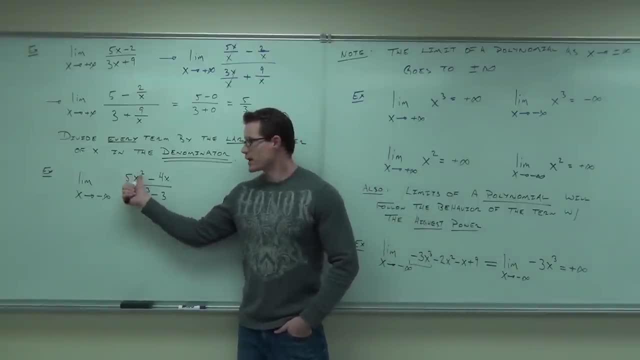 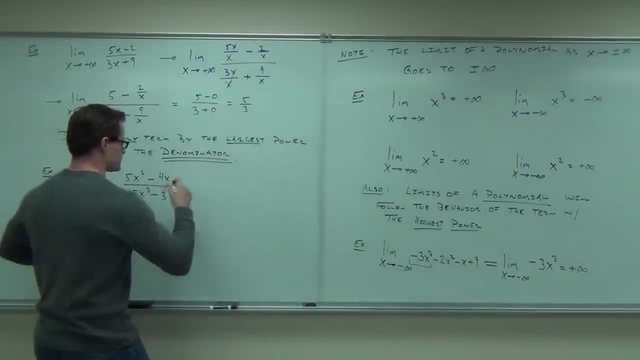 to show you work, you're gonna be dividing everything not by x squared mm-mm, but by x to the third power, X to the third power- Want me on that? So this would look just like this: You'd have 5x squared over x to the third. 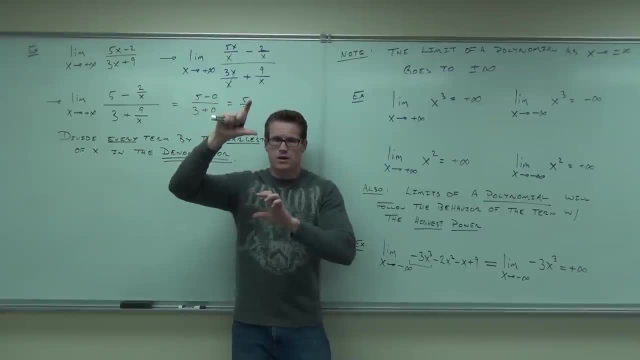 That's infinity, either positive or negative infinity. If this one is larger than- I'm sorry, smaller than this one, if this one's larger, well then you're going to be going to zero, because you divide by this one. 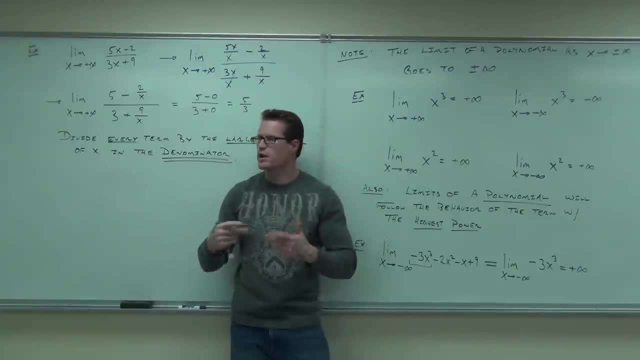 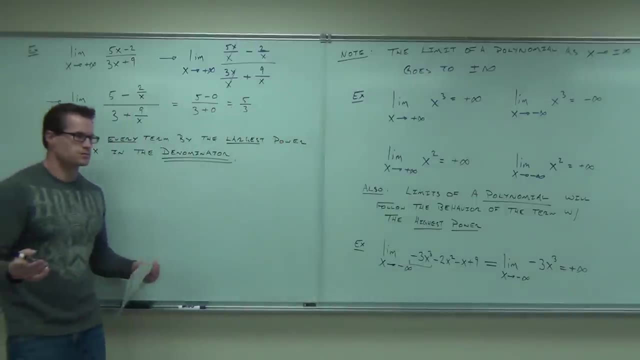 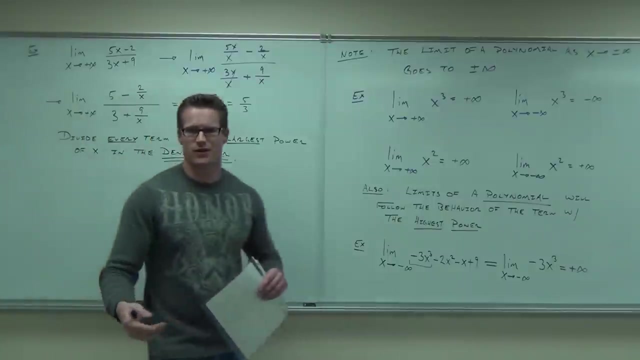 no x's here. x here. you're going to zero. That's one way you can look at that as well. So if the top still has an x, you're going to go to infinity. Let's try a couple more. You're going to start seeing this very easily. 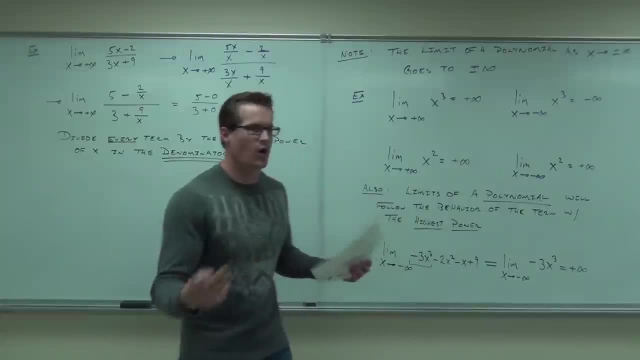 It's not going to be something super-duper hard. What's going to be super-duper hard is when we combine this with some other ideas in a little while. Actually, not even super-duper hard then, just super hard, not even duper. 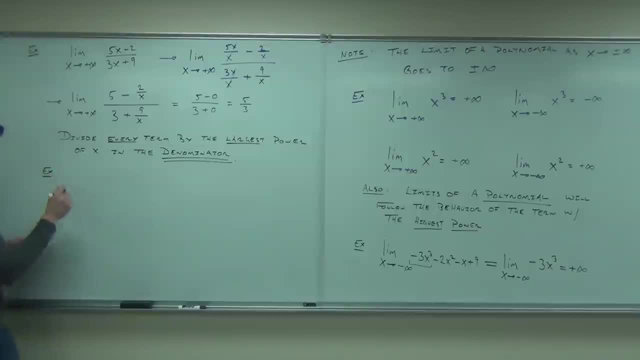 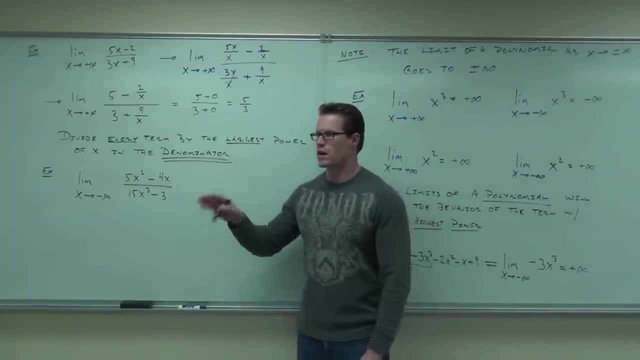 Don't worry about the duper, Come on. that was funny, Among others. If you were listening to what I was talking about, you could probably tell me where this limit is going. right off the bat: Zero, Not one third Zero. 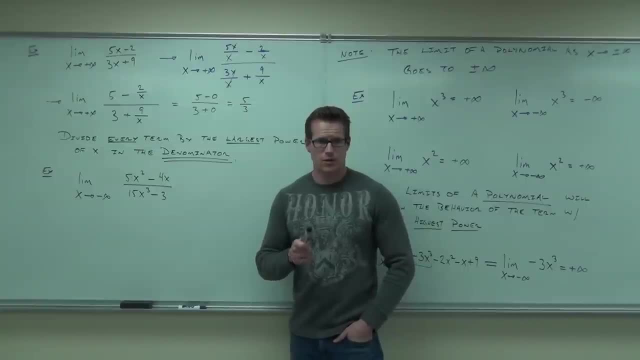 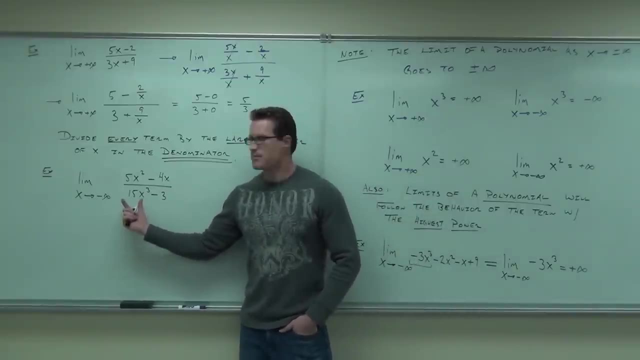 If the powers matched up, it would: Where's the power of the biggest There? That means what we're going to be doing here to show you work: you're going to be dividing everything not by x squared, but by x to the third power. 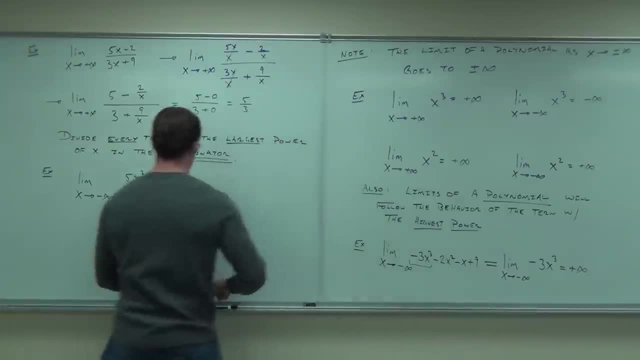 x to the third power. You follow me on that. So this would look just like this: You'd have 5x squared over x to the third, minus 4x over x to the third. All over, Everything is divided Everything. 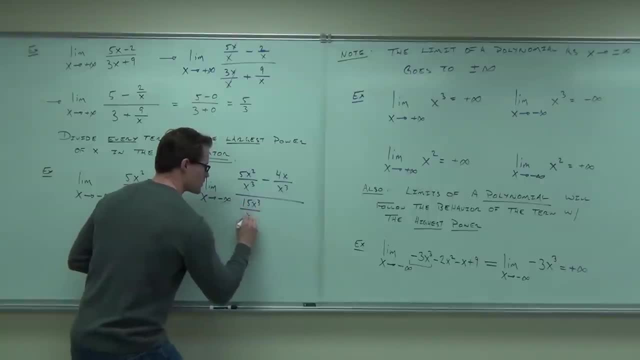 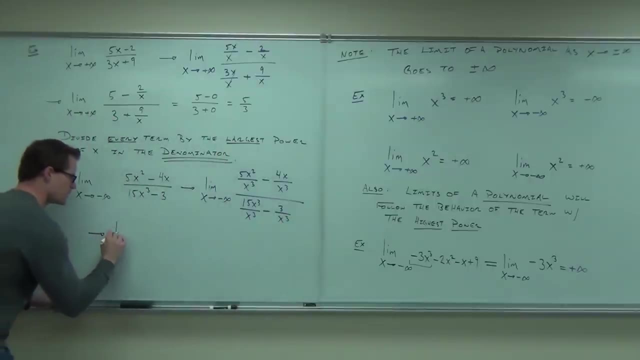 15x to the third over x to the third, Minus 3 over x to the third. If we do just a little simplification, well, look what happens. Do you see how? this power is still going to be 5 over x. 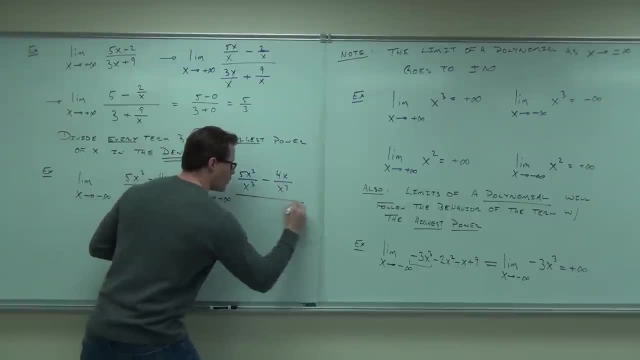 Minus 4x over x to the third. All over everything is divided everything: 15x to the third over x to the third, Minus 3 over x to the third. If we do just a little simplification. 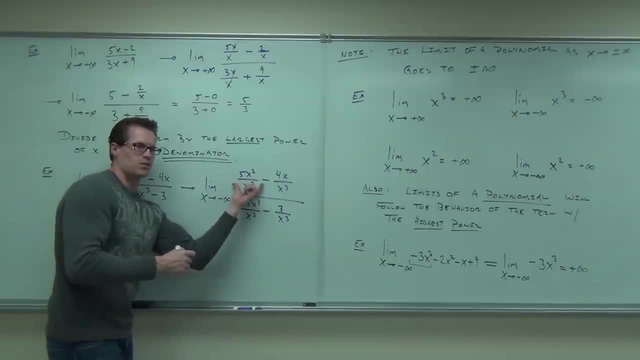 Well, look what happens. Do you see how? this power is still gonna be 5 over x And this is gonna be 4 over x squared. You see the x squared. This is gonna be 15, sure, But this is gonna be 3 over x. to the third. 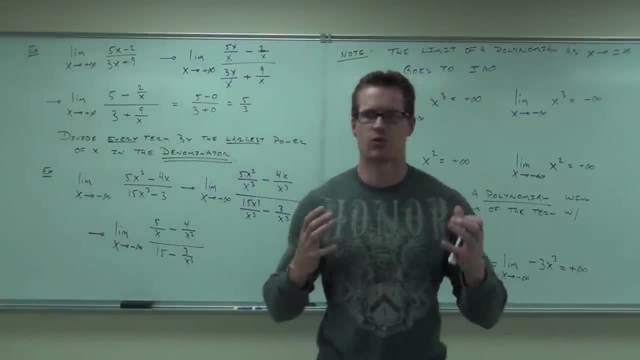 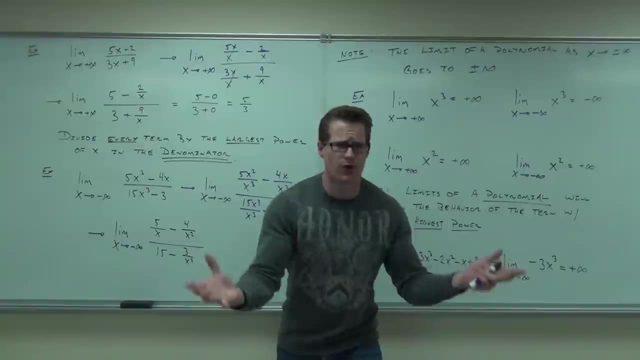 We had that. We had that, The principles of beginning class. for a reason, It said: any constant over any power of x, as x approaches any infinity, is going where folks Where Zero. So where's this going, Zero, Where's this going? 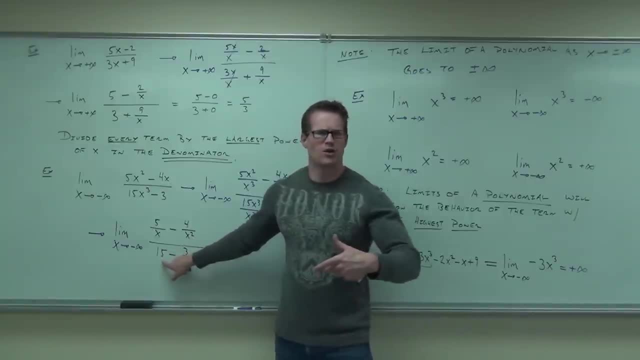 Where's this going? Oh, come on, come on, Everyone's gotta play along. Where's this going? Zero, Zero, zero, 15, zero. So this, after you stop running, the limit would be zero 0.. 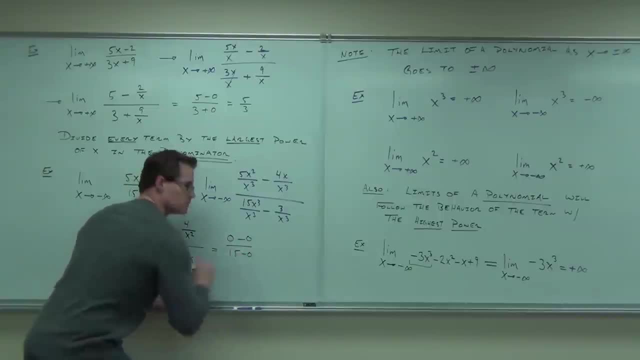 would be zero minus zero, over 15 minus zero. That's where these things are going. It's a constant over x as x approaches infinity, Negative infinity, but still an infinity Zero, zero, zero, zero. How much is that gonna be? 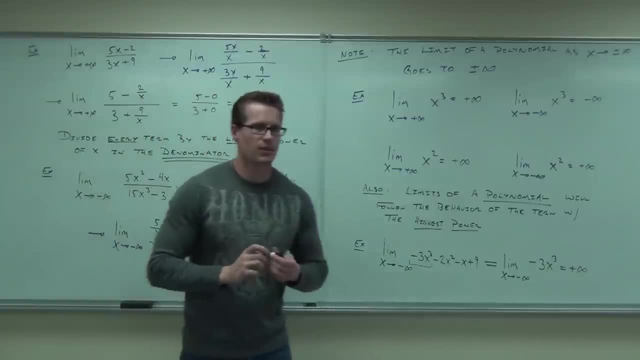 Zero, That's zero. That says a horizontal asymptote. That's what this is, by the way, a horizontal asymptote as you're going to the left. Are you following me on that? Now, if you did this, if you reciprocated this, 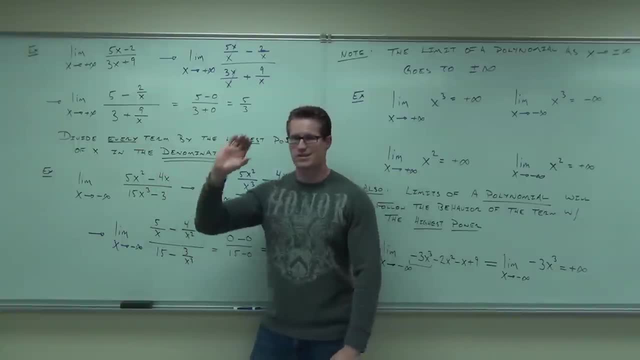 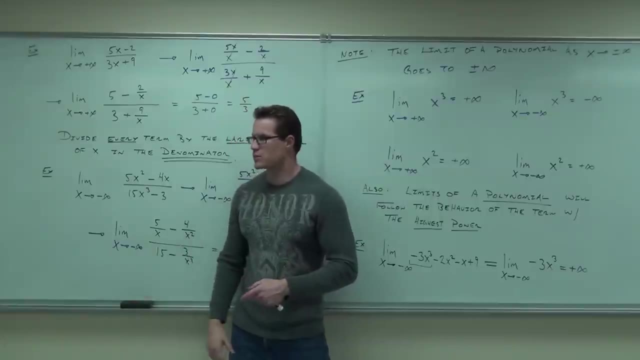 and you divided everything by x squared. do you see how you still have an x on the numerator? That would be saying you're going to positive or negative infinity, depending on what x is approaching. Let's do one more, and then next time. 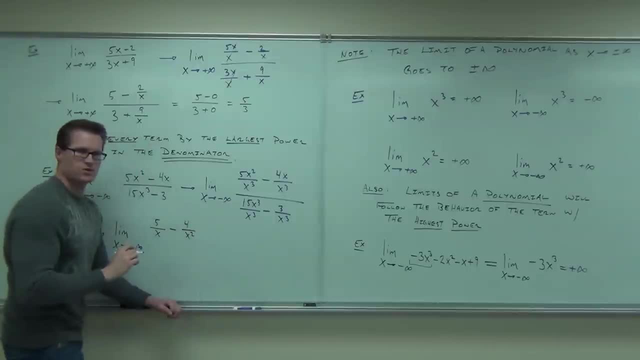 And this is going to be 4 over x squared. You see, the x squared. This is going to be 15, sure, But this is going to be 3 over x. to the third. We had the principles at the beginning of class. 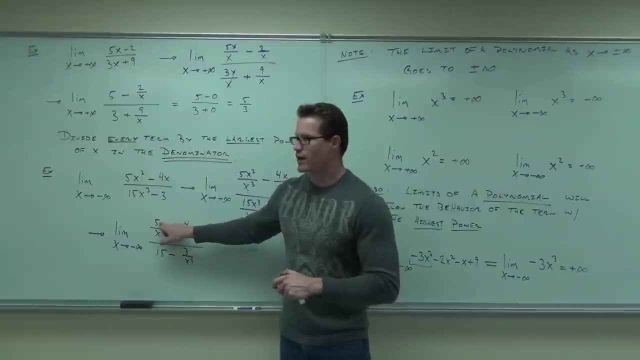 for a reason, It said: any constant over any power of x, as x approaches any infinity, is going where folks Where Zero. So where's this going? Zero? Where's this going? Where's this going? Oh, come on. 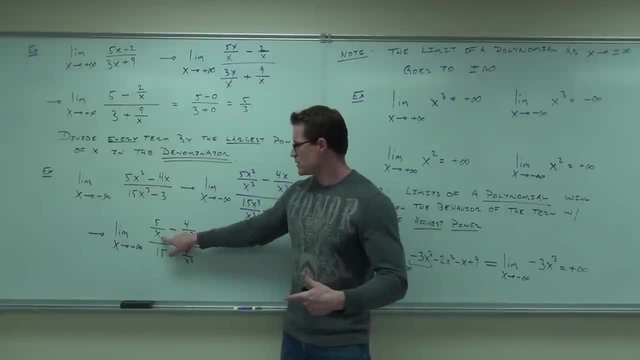 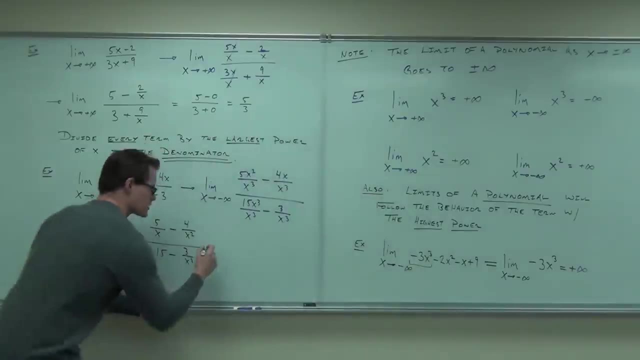 Come on, Everyone got to play along. Where's this going? Zero Zero, Zero, Zero, 15. 15. Zero. So this: after you stop running, the limit would be 0 minus 0 over 15 minus 0.. 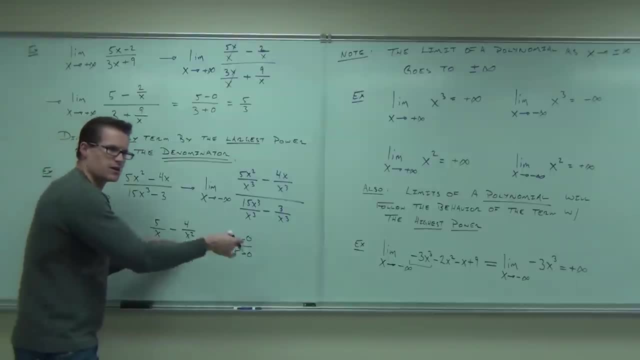 That's where these things are going. It's a constant over x as x approaches infinity, negative infinity, but still an infinity: 0, 0, 0, 0.. How much is that going to be Zero? That's zero. 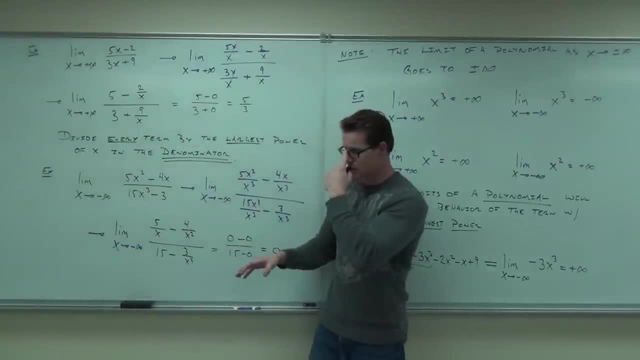 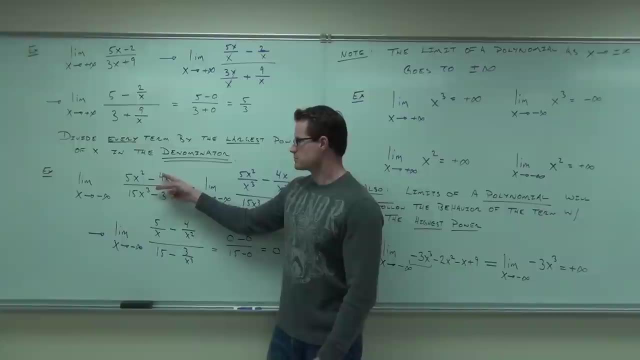 That says a horizontal asymptote. that's what this is, by the way, a horizontal asymptote, as you're going to the left on that. Now, if you did this, if you reciprocated this and you divide everything by x, squared. 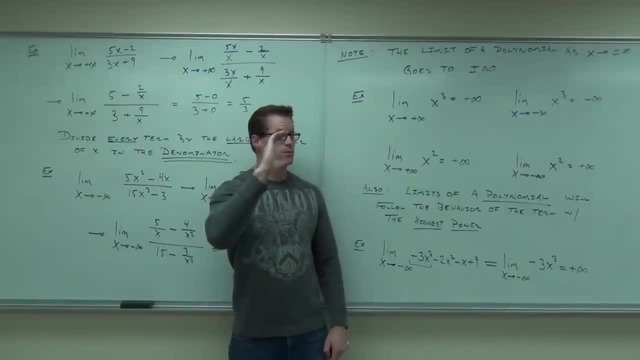 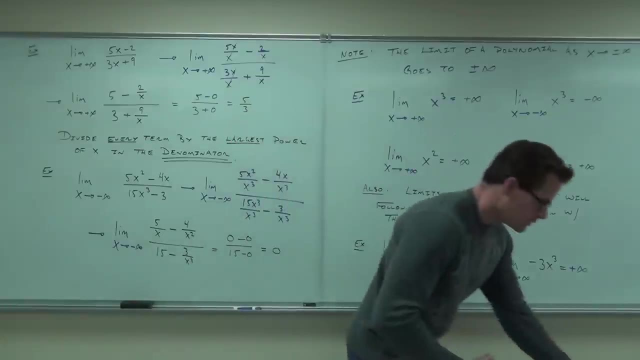 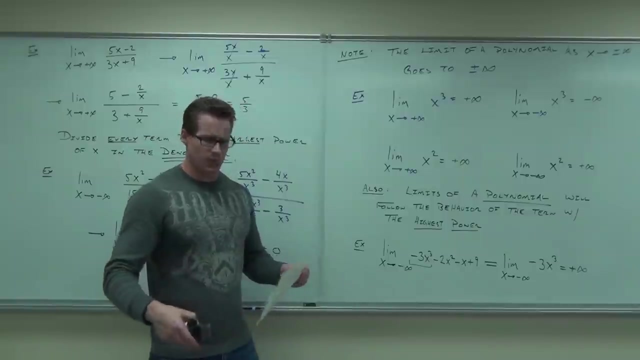 do you see how you still have an x on the numerator? That would be saying you're going to positive or negative infinity, depending on what x is approaching. Let's do one more and then next time we'll start building on this concept. Two more, two more. We've got. 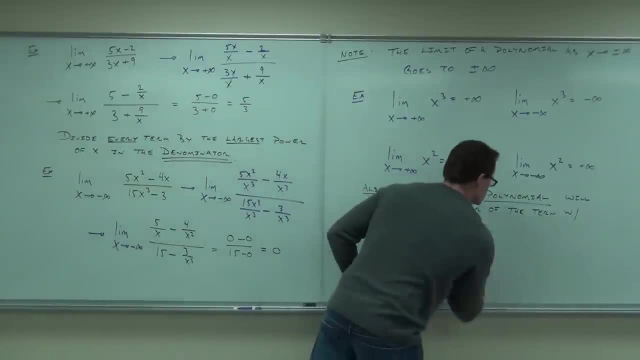 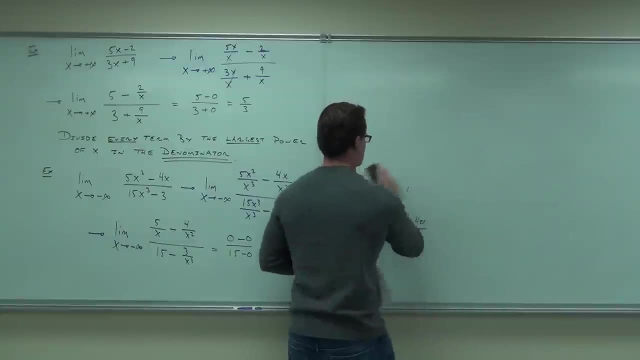 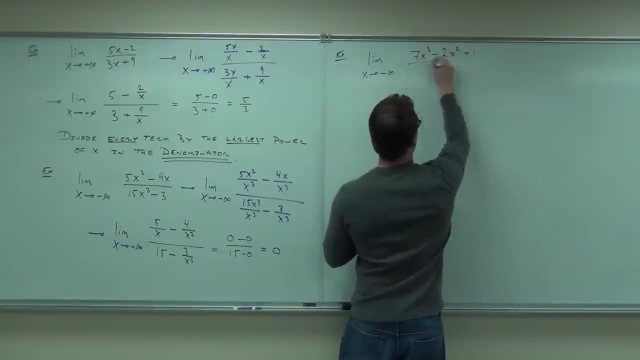 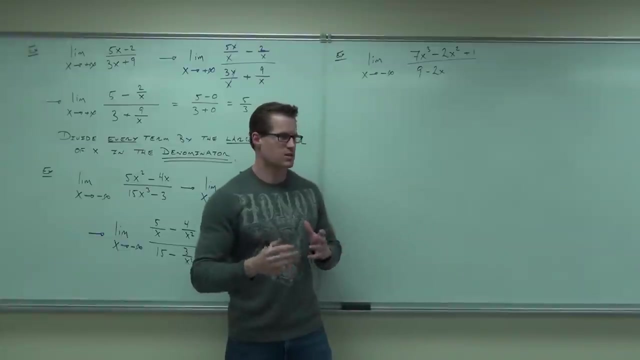 we'll start building on this concept. Two more, two more. We got three minutes. now There we go Again. some of you who kind of understand this concept right now should probably be able to tell me where this is going to approach. 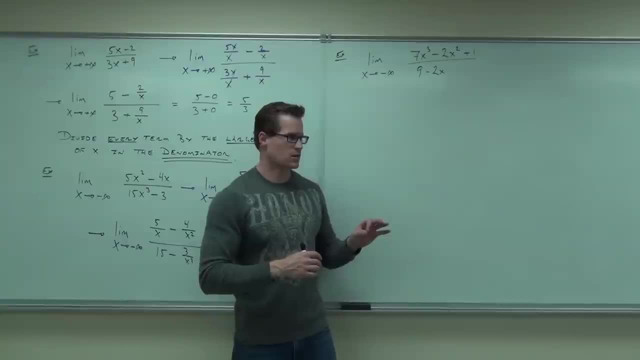 or at least have a guess what it's going to approach. Okay, okay, battle royale. Well, you might want to do the work to make sure, but you see it's not going to go to a constant, You see it's not going to go to zero. 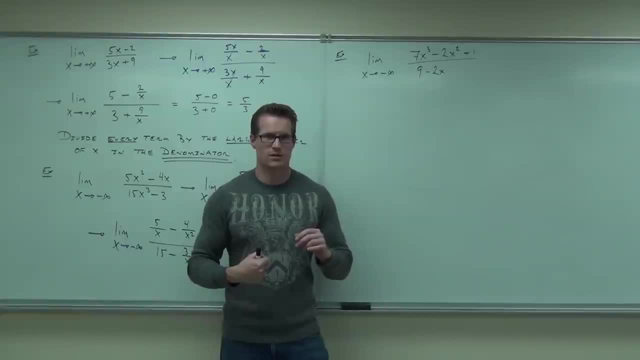 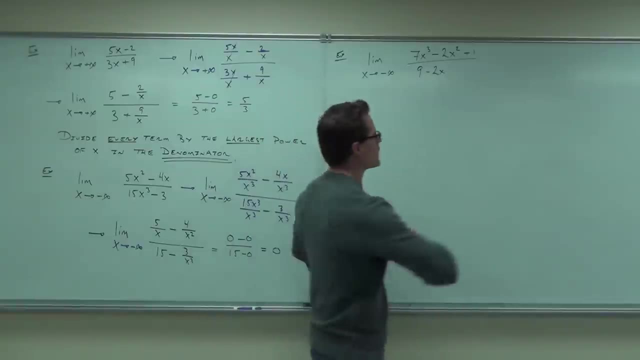 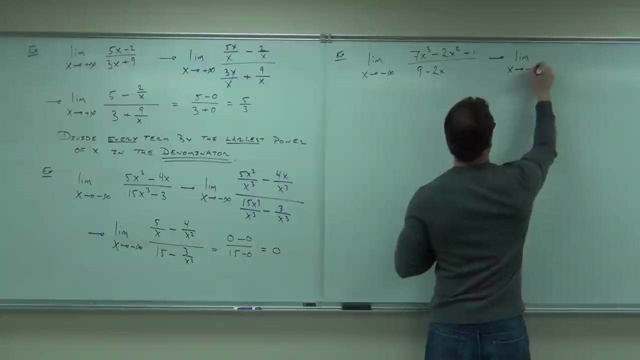 What are we going to divide by X cubed, X squared, or X, The largest power in the denominator? So show your work. don't get lazy on that. don't take a guess, because some of you are guessing right now. Don't take a guess, Show your work. 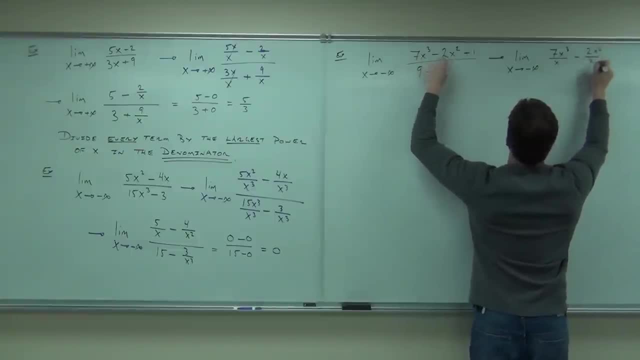 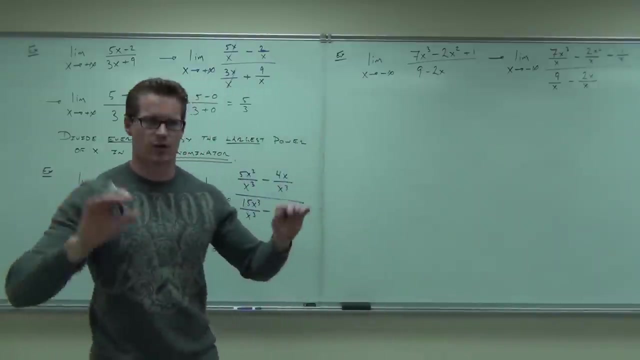 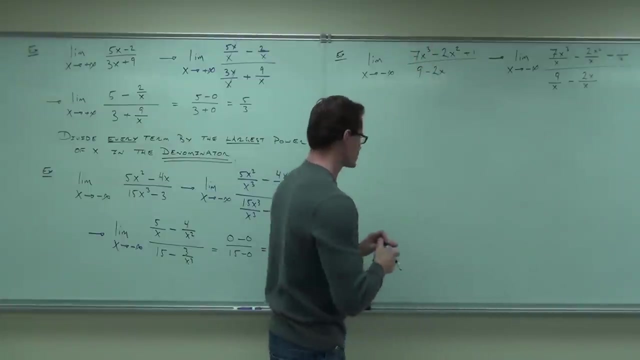 Over X, over X, over X, all over that. Divide everything by the largest power in the denominator, Not the numerator. That'll give you undefined spots. Do you see that If I divide it by X cubed, I get this whole bunch of undefined stuff? Can't have that, Can't do that. 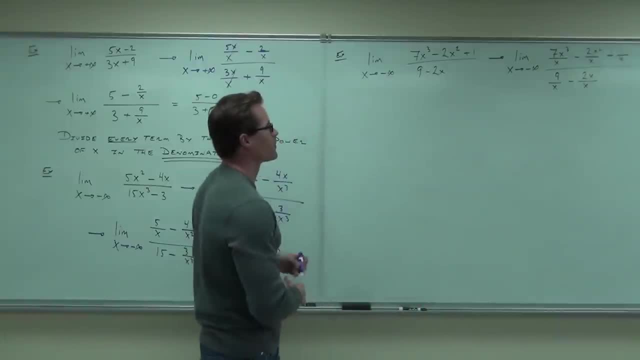 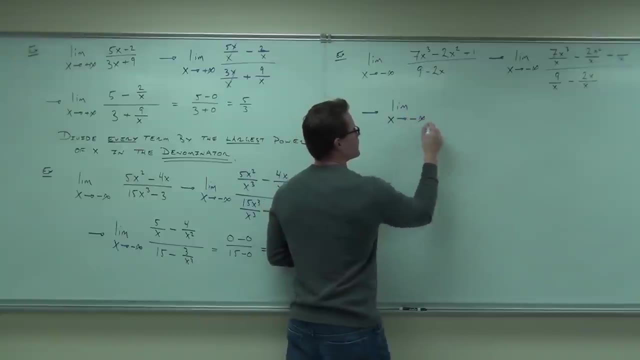 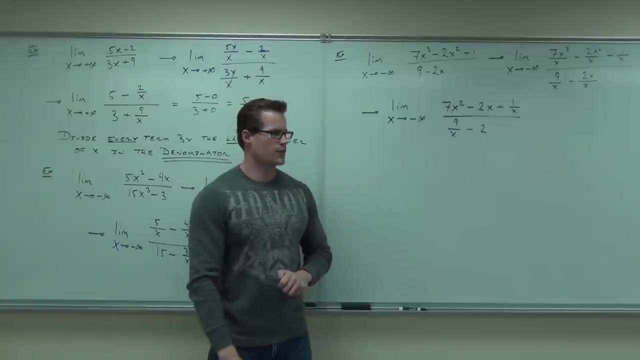 Are you alright with that one? so far, Simplify them. You're going to get 7X squared minus 2X plus 1 over X, All over 9 over X plus 1 over X Minus 2.. You follow me on that. Now let's kind of think carefully about what happens. 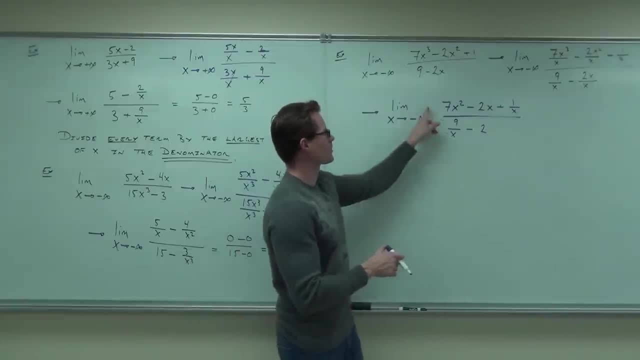 here. What happens? Where does that go? That goes to positive infinity. Does this stuff matter? No, That goes to positive infinity. Agreed, It's X squared. This is zero. This is negative infinity, But that is a negative 2.. Where's that going? Negative infinity. 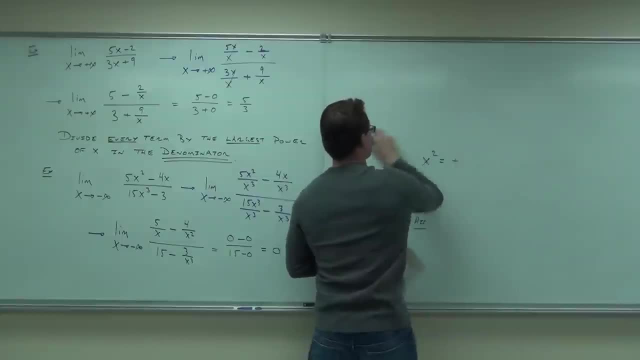 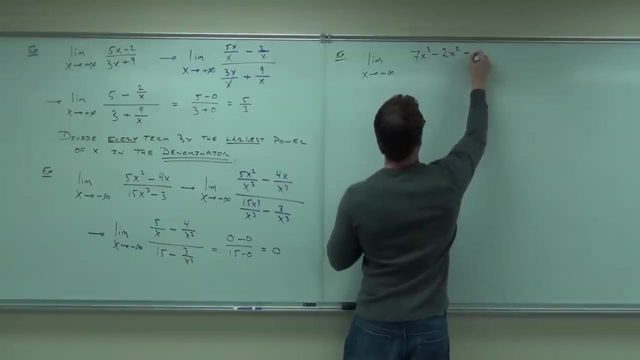 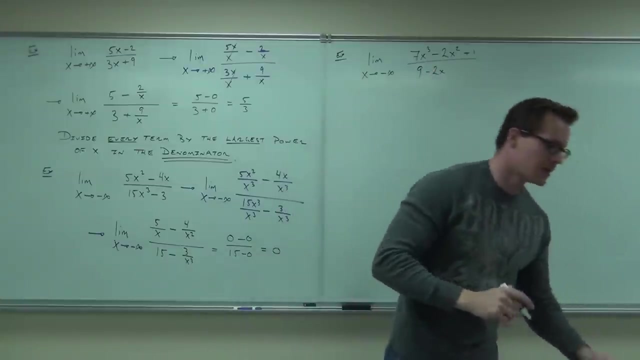 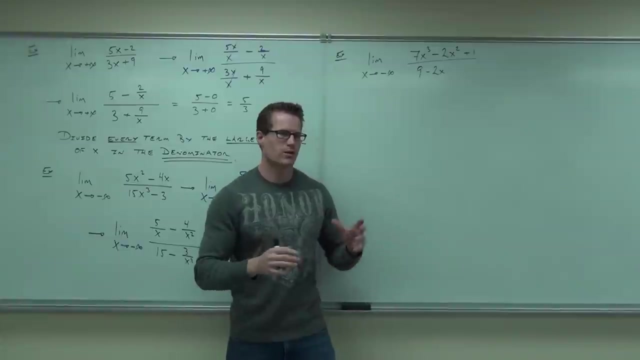 three minutes now. Again, some of you who kind of understand this concept right now should probably be able to tell me where this is going to approach, or at least have a guess what it's going to approach: Negative infinity, Oh, okay. 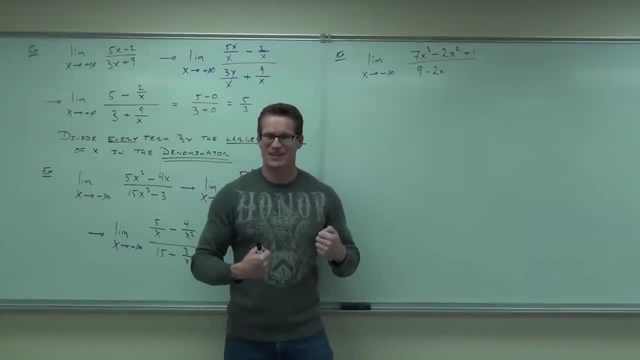 Positive infinity, Okay, Ooh, battle royale. Well, you might want to do the work to make sure, but you see, it's not going to be positive infinity, It's going to go to a constant. You see it's not going to go to zero. What are we going? 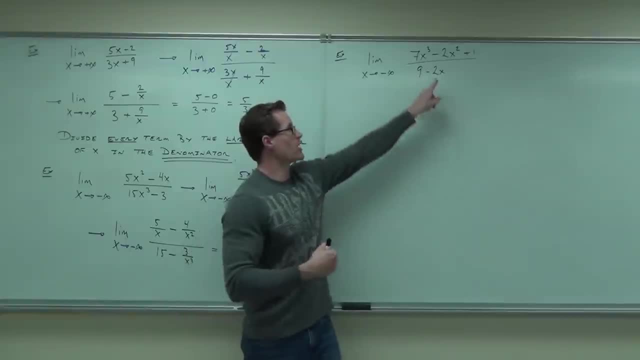 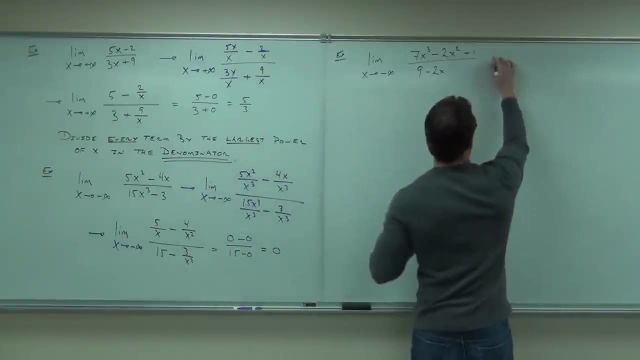 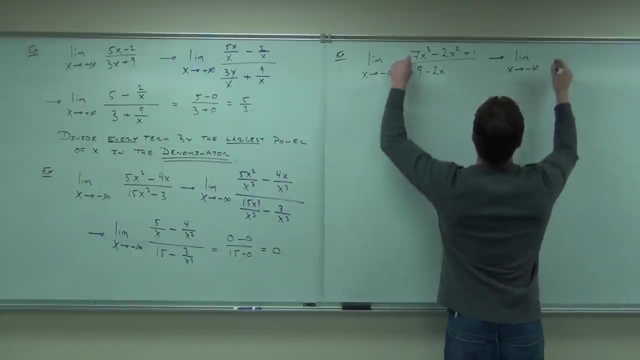 to divide by X cubed, x squared, or x- X, The largest power in the denominator. So show your work. Don't get lazy on that. Don't take a guess, because some of you are guessing right now. Don't take a guess, Show your work. 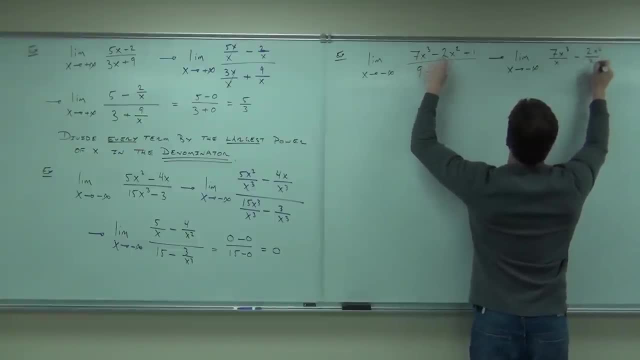 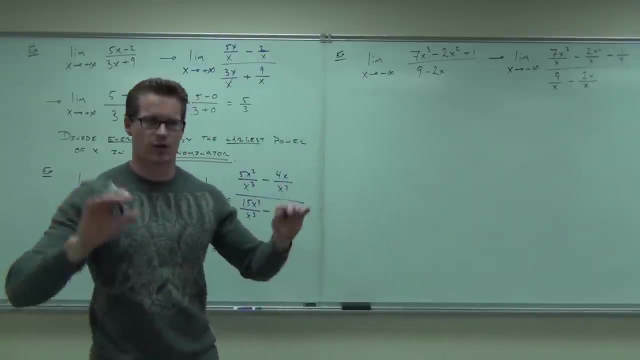 Over x, Over x, Over x, All over that. Divide everything by the largest power in the denominator, not the numerator. That'll give you undefined spots. Do you see that If I divide it by x cubed, I get this whole? 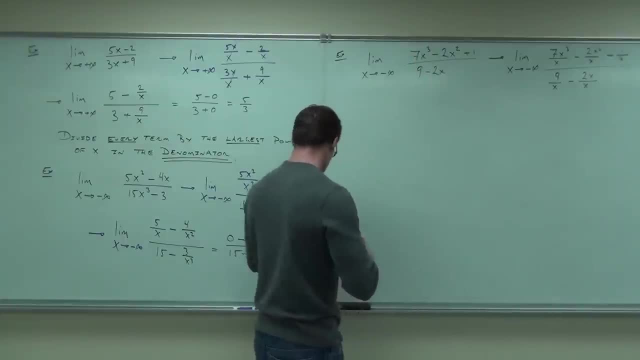 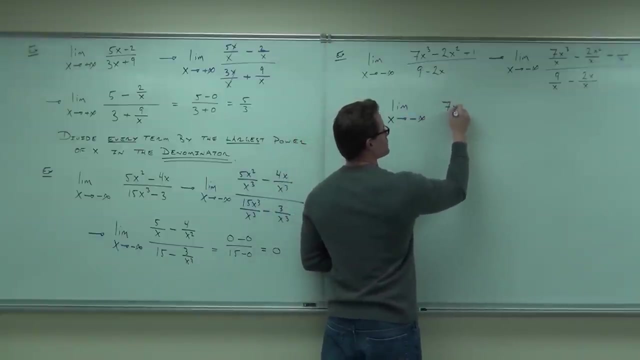 bunch of undefined stuff. Can't have that, Can't do that. Are you all right with that one? so far? Simplify them. You're going to get 7x squared minus 2x plus 1 over x. All over 9 over x minus 2.. 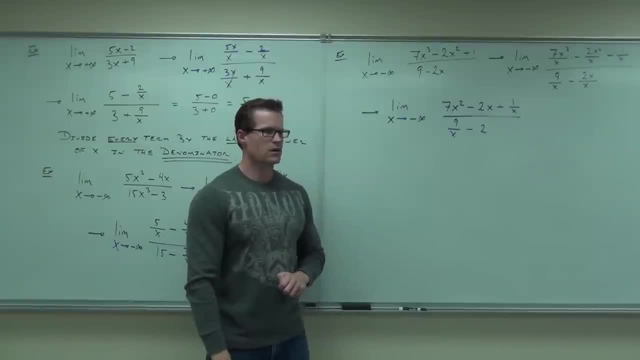 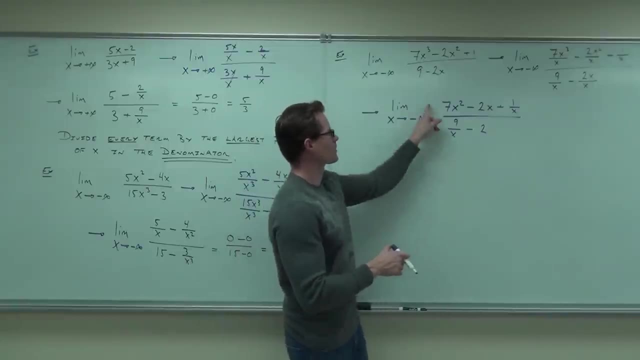 You following me on that? Now let's kind of think carefully about what happens here. What happens, Where does that go? That goes to Positive infinity. Positive infinity- Does this stuff matter? No, That goes to positive infinity, Agreed. 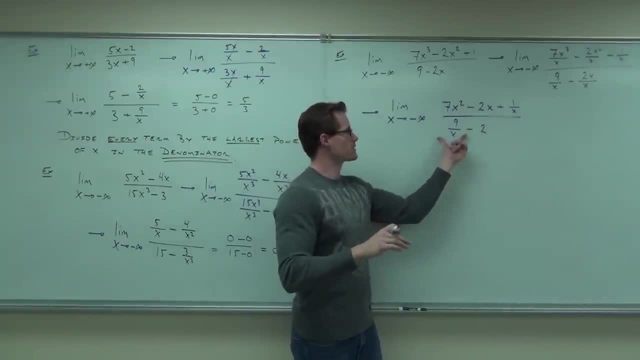 It's x squared, This is 0, but that is a negative 2.. Where's that going? Negative infinity, Negative infinity. In fact, if you really wanted me to show it to you this way, I could Couldn't you factor out a negative and get 2 minus 9 over x? Move the negative up top. 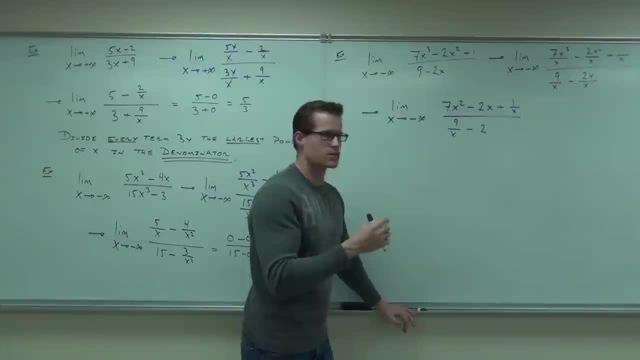 In fact, if you really wanted me to show it to you this way, I could. Couldn't you factor out a negative and get 2 minus 9 over X? Move the negative up top. Negative infinity. Bam Got it. Did you see it? Did I lose you? 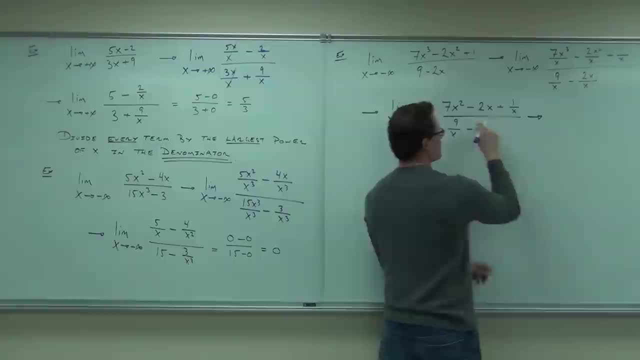 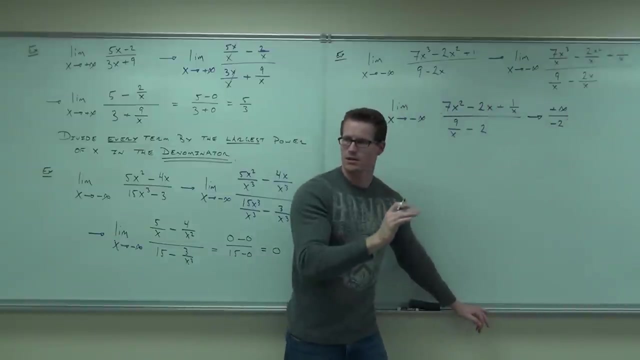 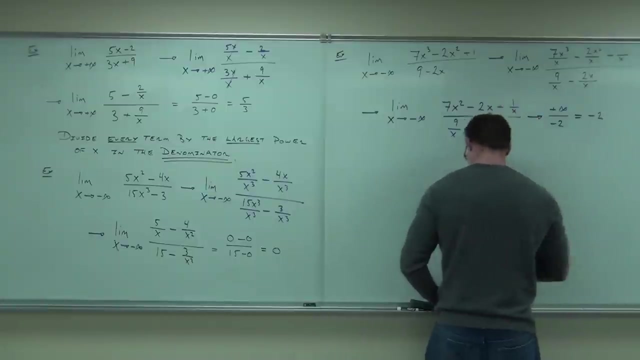 You understand that it went to positive infinity. A little unorthodox here, but you see, this goes to zero. Negative 2 doesn't change. Positive divided by negative is a Infinity. Infinity divided by 2? Still infinity? No, mathematically, Oh not that It doesn't do that Mathematically. 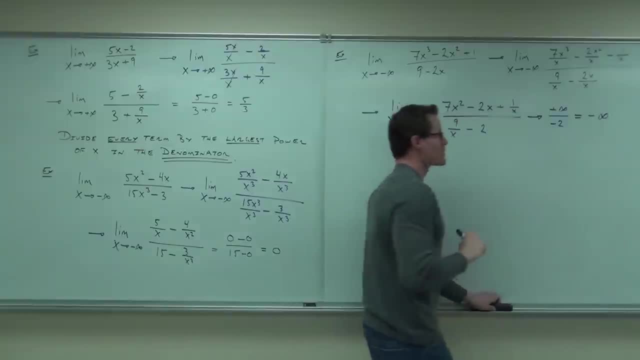 the way that you could show. this is the way I showed you. If you factored out the negative, it's negative. 2 minus 9 over X. Right, If you take that negative and move it to the top of your fraction, which is legal to do, it goes there. That becomes 2 minus 9 over. 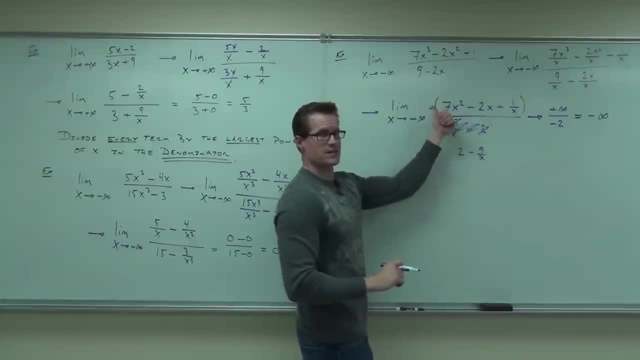 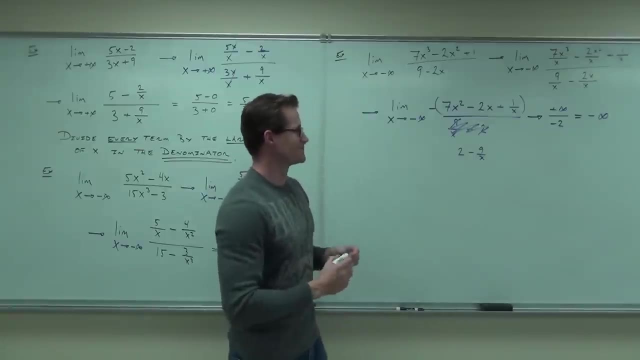 X That says this goes to infinity times the negative, That's negative infinity. That's negative infinity Divided by a positive. now that's negative infinity. That's what that means as well. Can we show it the way? it's unorthodox way. 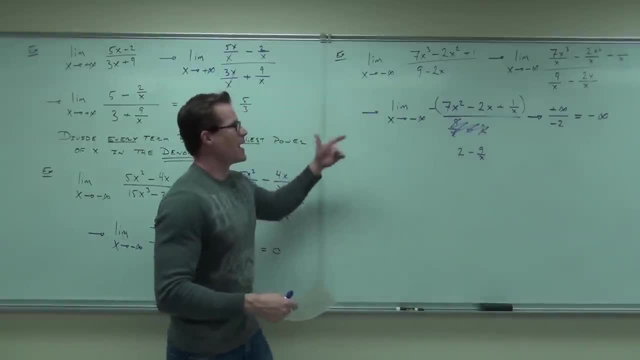 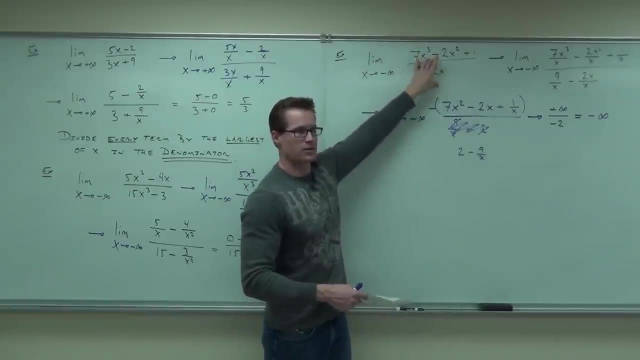 Yeah, By the way, did anything but the highest powers of X have anything to do with our problem here? This one and that one was really what caused this to be the way it was That. One last thing. I'll leave you with just this idea, Because I want you to. 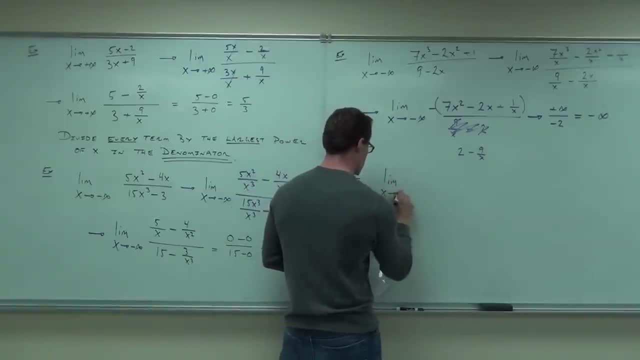 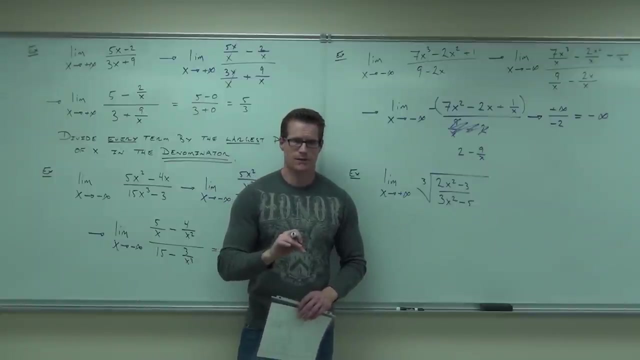 look at some of your homework tonight. but I don't want you to be completely afraid of it, Just a little afraid. That looks pretty nasty. but tell me something that I can do with exponents. What can you do? Divided by X? 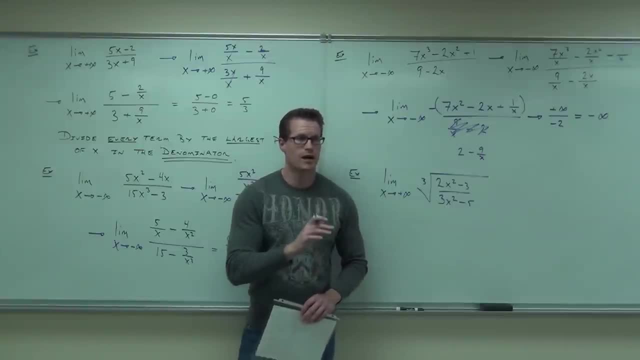 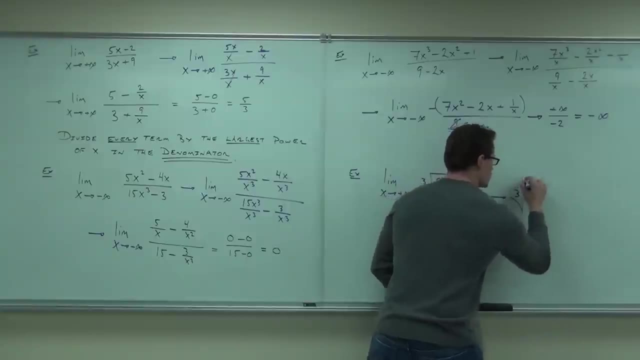 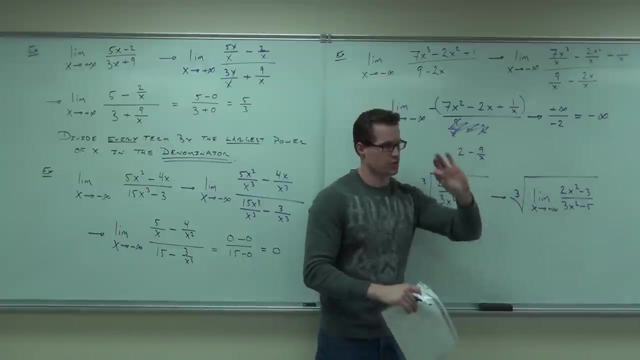 Not, yet. You can move them outside of the graph. I can move them outside, That's right. Is a root a type of exponent? Yes, Then look, You can take a cube root of the limit. Okay, Now ignore the cube root for a second. just for a second, though. Can you do this limit? 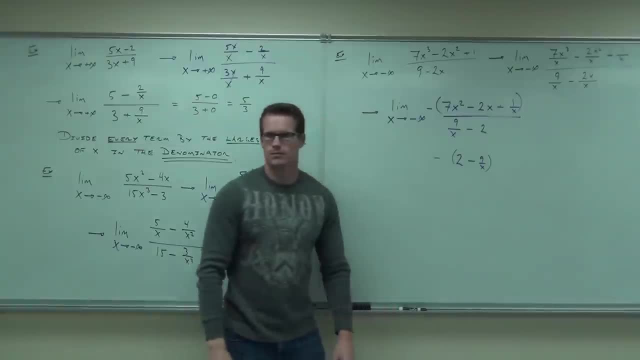 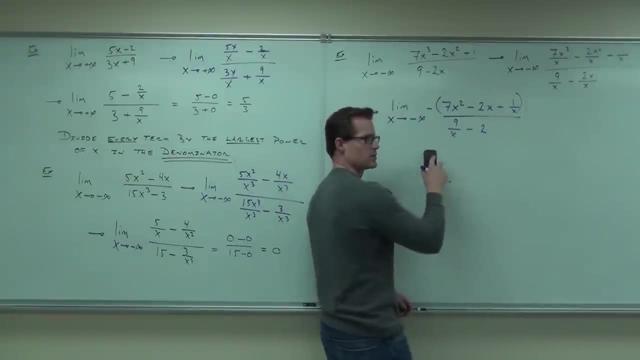 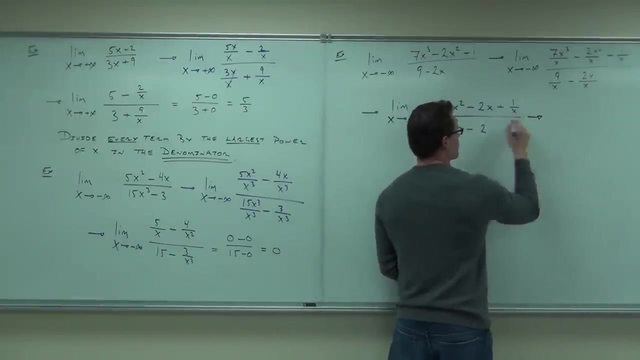 Move the negative up top Negative infinity. Bam Got it. Do you see it? Did I lose you? You understand that it went to positive infinity. A little unorthodox here, but you see this goes to 0.. Negative 2 doesn't change. Positive divided by negative is a. 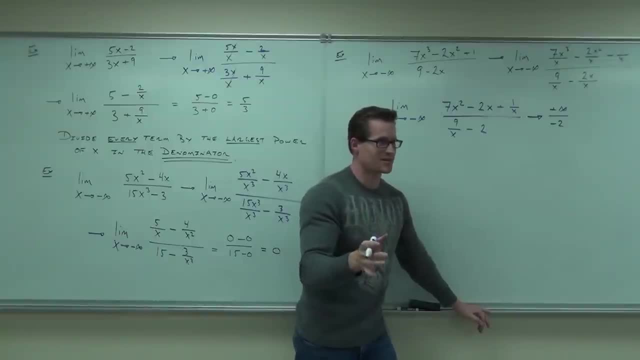 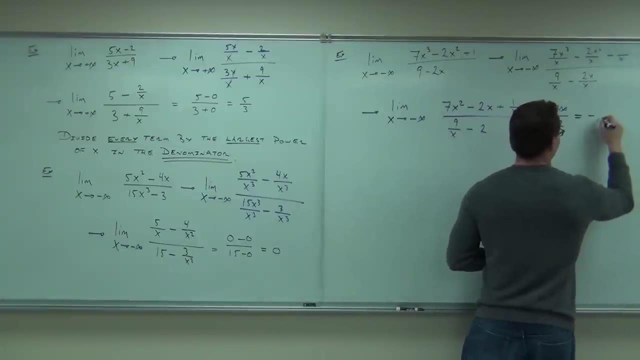 Infinity. Infinity divided by 2? Still infinity. Yeah, Now mathematically- oh, not that It doesn't do that Math- Yeah, Mathematically. the way that you could show. this is the way I showed you, If you factored. 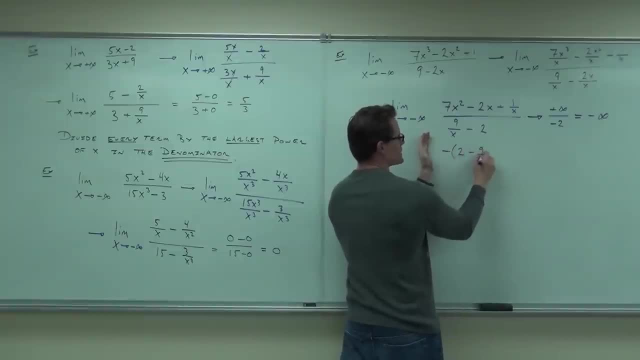 out the negative. it's negative. 2 minus 9 over x. Right, If you take that negative and move it to the top of your fraction, which is legal to do, it goes there. That becomes 2 minus 9 over x. That says this goes to infinity times a negative. That's negative. 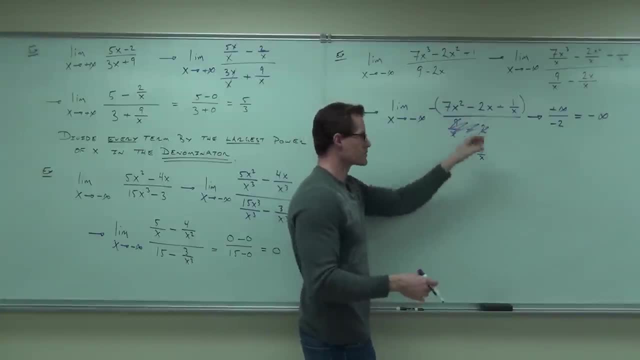 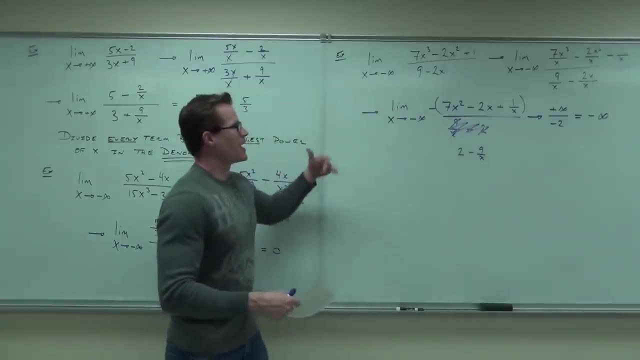 infinity Divided by a positive, now that's negative infinity. That's what that means as well. Can we show it the way? Yeah, By the way, did anything but the highest powers of x have anything to do with our problem here? 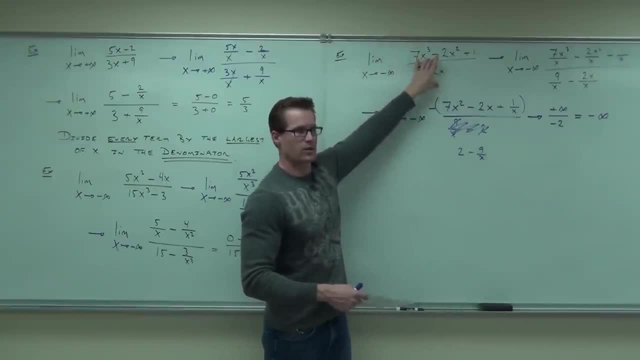 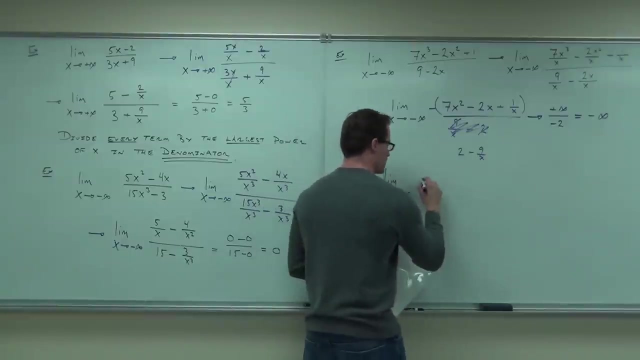 No, That one is really what caused this to be the way it was that? One last thing: I'll leave you with just this idea, Because I want you to look at some of your homework tonight, but I don't want you to be completely afraid of it, Just a little afraid, That looks. 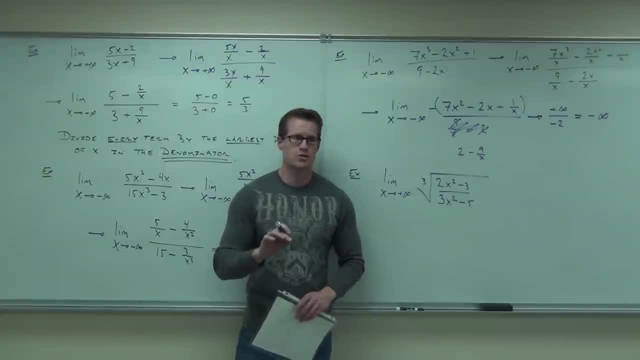 pretty nasty, but tell me something that I can do. Yeah, What can I do with exponents? What can you do Divided by x? Not, yet You can move them outside of the graph. I can move them outside. Is a root, a type of exponent. 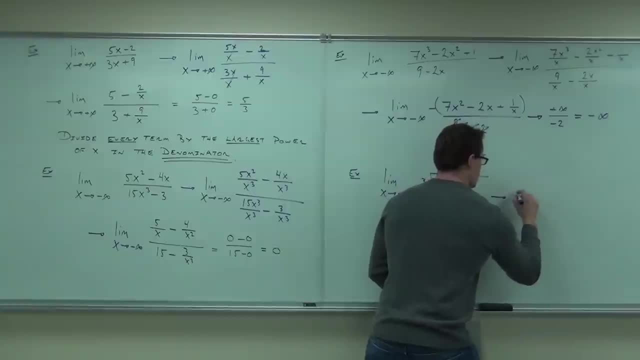 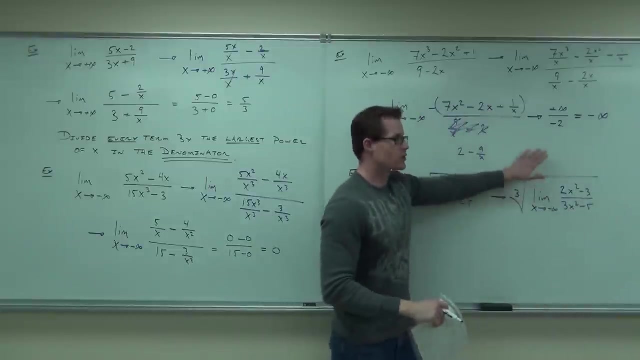 Yes, Then look, You can take a cube root of the limit, OK, Ah, Now ignore the cube root for a second, Just for a second. Can you do this limit? Yeah, Explain to me how you would do this limit. What would you divide by here? 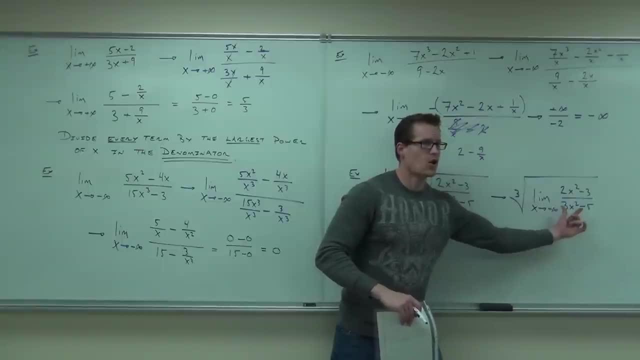 x, x. Which one? x squared, x squared. Hey, where is this limit going to go on the inside Two-thirds, Do you see the two-thirds, Two-thirds, Two-thirds, And then take a cube root of that. So our answer here, after you show the work: 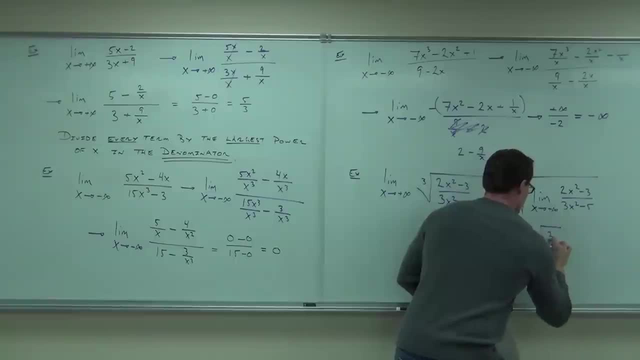 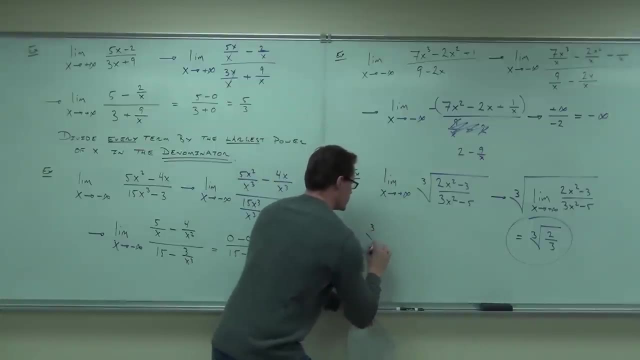 would be a cube root of two-thirds. The work you show is this: You show a cube root 2x squared over x squared minus 3 over x squared all over that. That's what you show, but that's the answer you get. 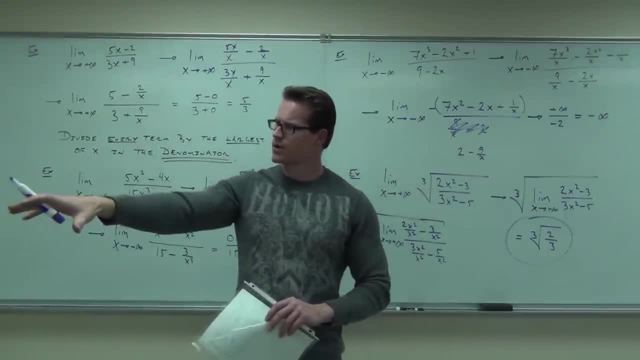 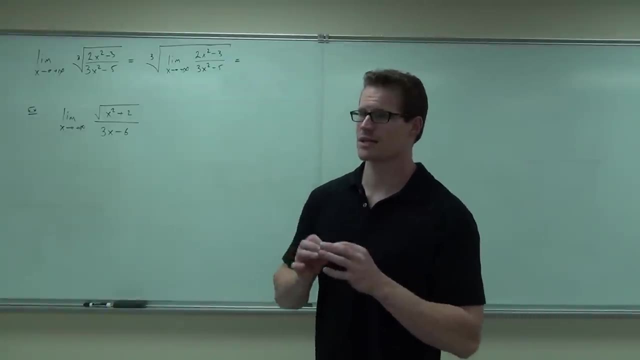 How many people understood today. I feel OK with it. Right side people: are you guys doing this so far? Yeah, OK, OK, so we're talking about how to do limits as x approaches infinity. Now the last example I gave you. I think I gave you that one, didn't I? 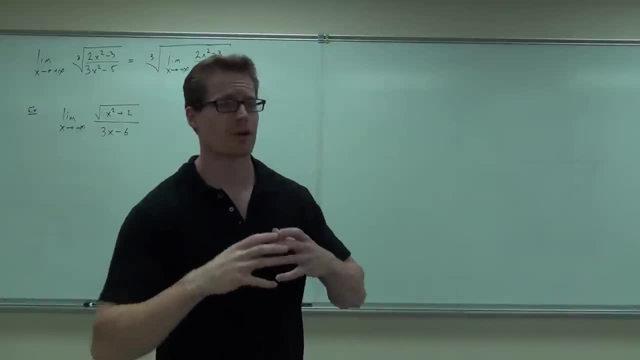 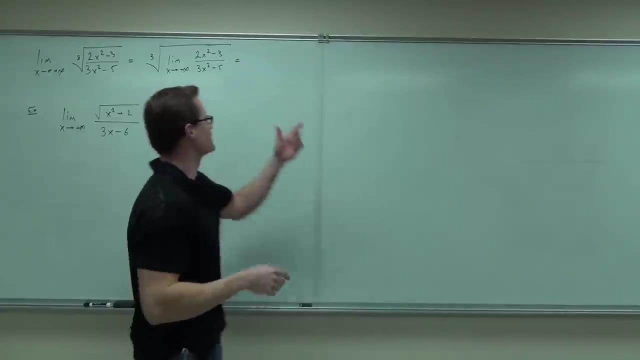 I said that when you have a cube root, it is a power. That means you can pull it outside of our limit and say, well, let's take the cube root of our limit itself. Now, when you do that, that's kind of nice, right, because we know how to take these limits. 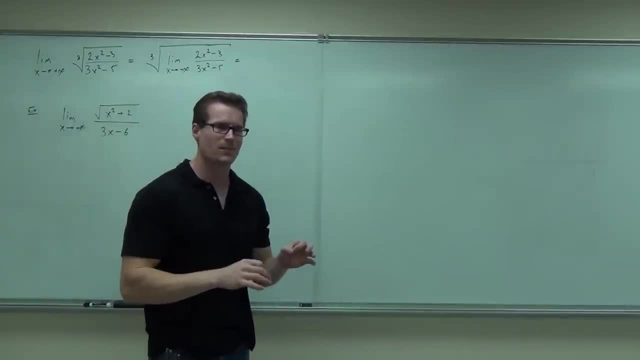 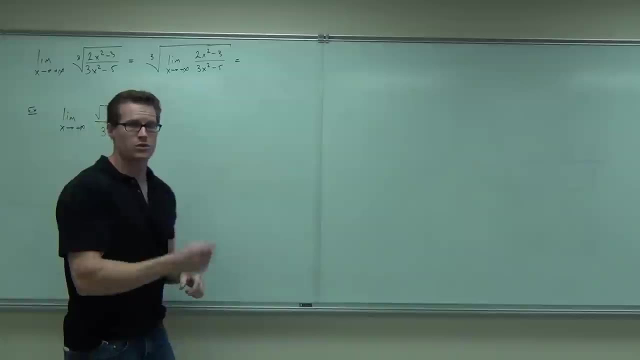 What we would normally do is divide everything by the largest power in the denominator. That's x squared, You would get 2.. That's going to be 0.. 3. That's going to be 0.. OK, 2 thirds You follow. 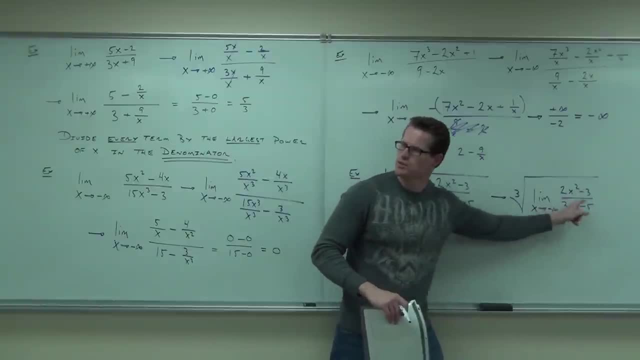 Yeah, Explain to me how you would do this limit. What would you divide by here? X, X, Which one? X squared, X squared? Hey, where is this limit going to go on the inside Two-thirds? Do you see the two-thirds? 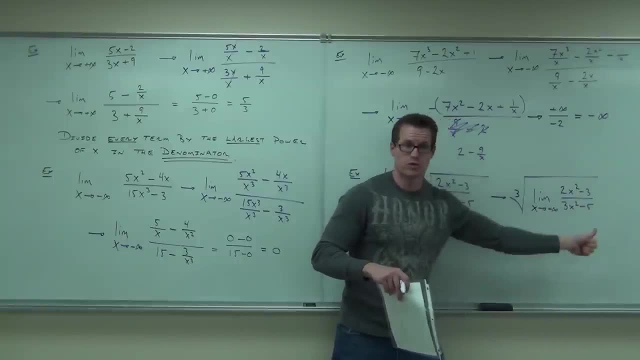 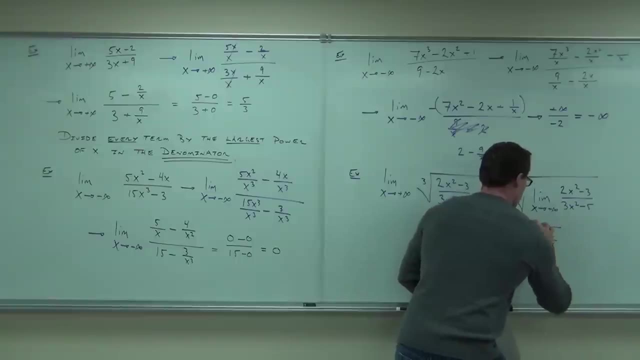 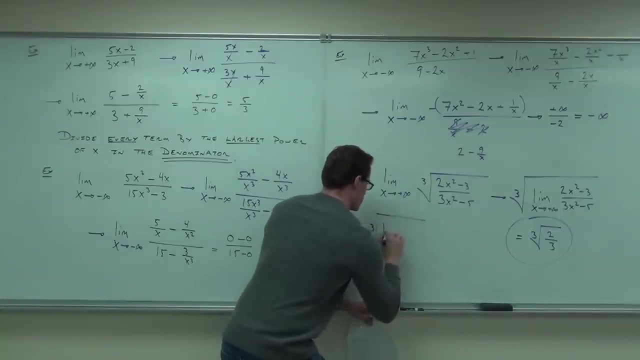 Two-thirds, Two-thirds And then take a cube root of that. So our answer here, after you show the work, would be: a cube root of two-thirds. The work you show is this: You show a cube root 2X. 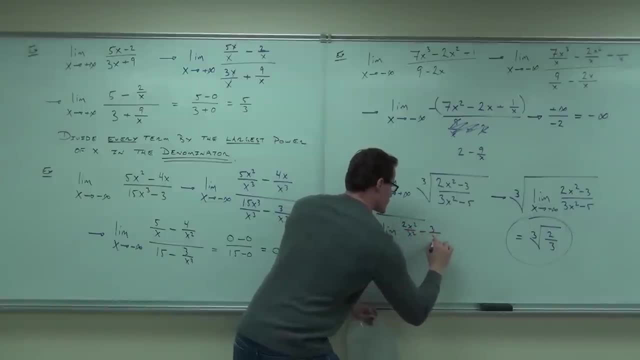 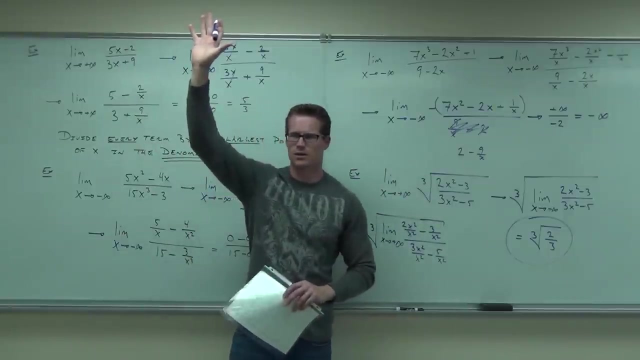 squared over X. squared minus 3 over X, squared, Okay, And then you show it here all over that. That's what you showed, but that's the answer you 're going to get. How many people understood today, if you're okay with it. 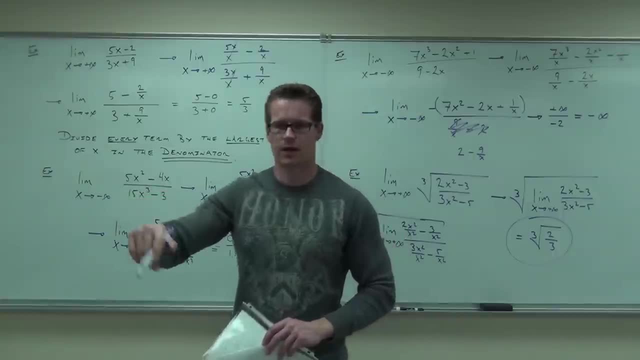 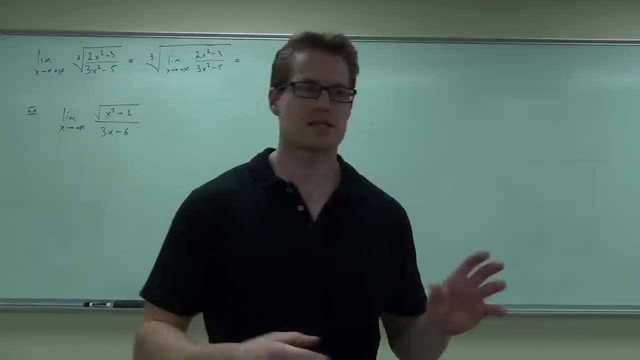 Here Right-side people are. you guys are understood so far, Yeah, Okay, Okay. so we're talking about how to do limits as X approaches infinity. Now the last example I gave you. I think I gave you that one, didn't I? 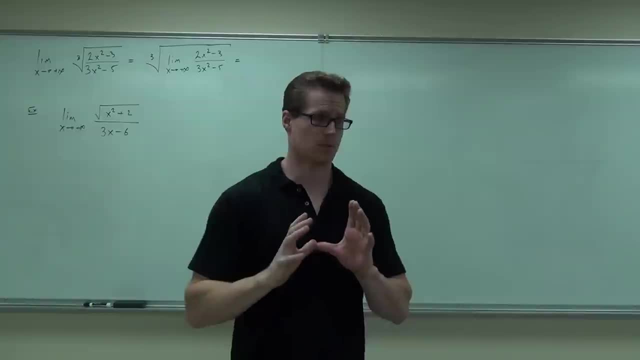 Uh-huh. I said that when you have a cube root, it is a power. That means that it's a power. Yeah, It is a power. That means you can pull it outside of our limit and say: well, let's take the cube root of our limit itself. 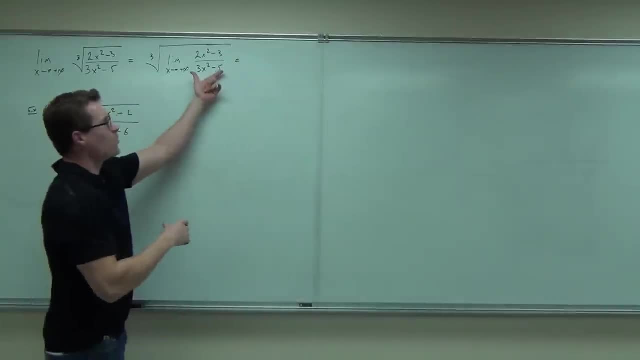 Now, when you do that, that's kinda nice, right, Because we know how to take these limits. What we normally do is divide everything by the largest power in the denominator. That's x squared, You would get two. that's gonna be zero. 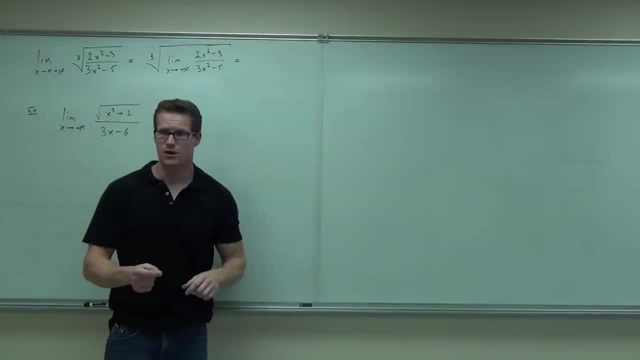 Three, that's gonna be zero. You're gonna get 2- 3rds. you follow- Don't forget about the cube root- but your answer is 2- 3rds with a cube root around it. That's it. 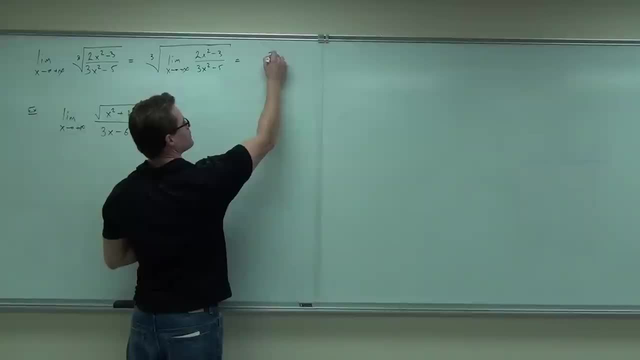 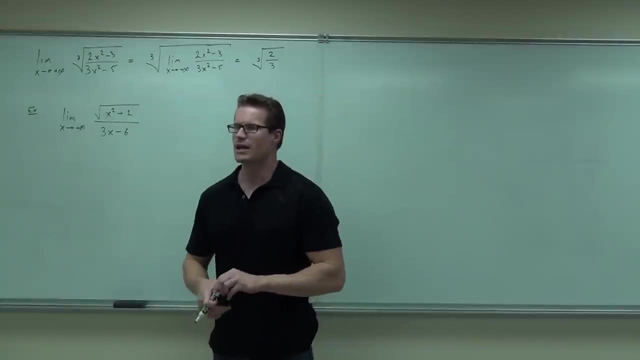 Don't forget about the cube root. but your answer is 2 thirds with a cube root around it. I think that's what I gave you last time. Were you OK with that one? Yeah, Now I showed you that one again because I want you to consider the problem that's just below it. 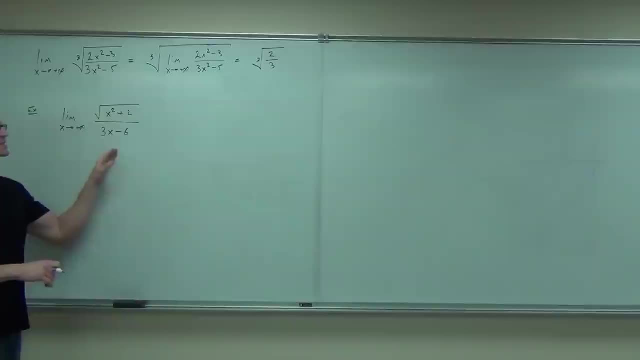 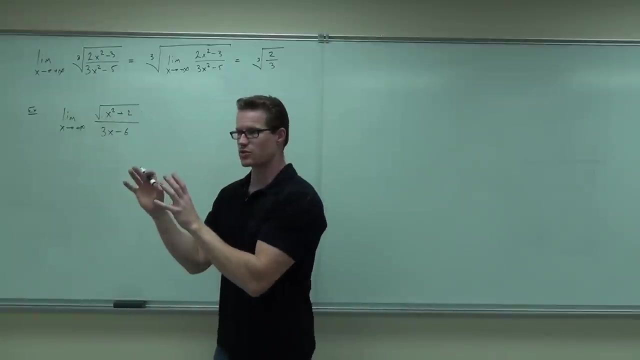 Can I do the same thing here? For instance, can I pull out the square root around the whole limit? No, No, because that square root is not around this whole function, It's just on the numerator. So, oh my gosh. Well, what do we do? 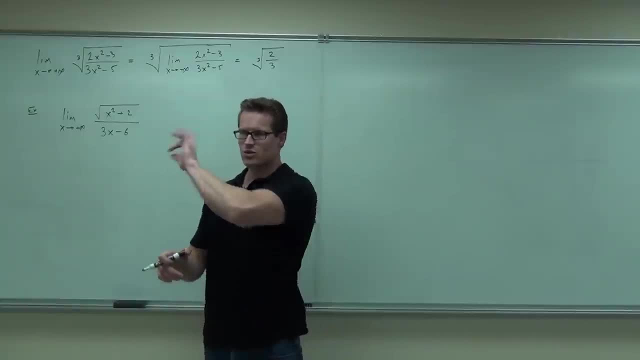 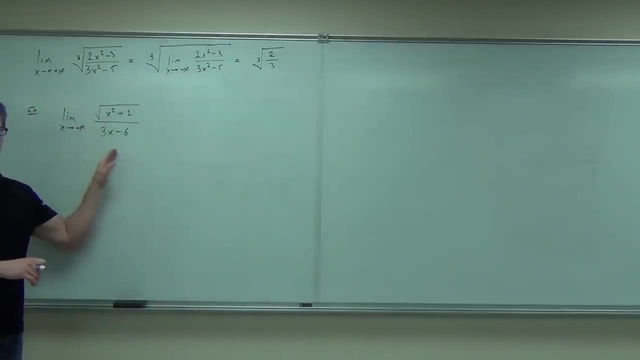 I think that's what I gave you last time. Were you okay with that one? Yeah, Now I showed you that one again because I want you to consider the problem that's just below it. Can I do the same thing here? For instance, can I pull out the square root? 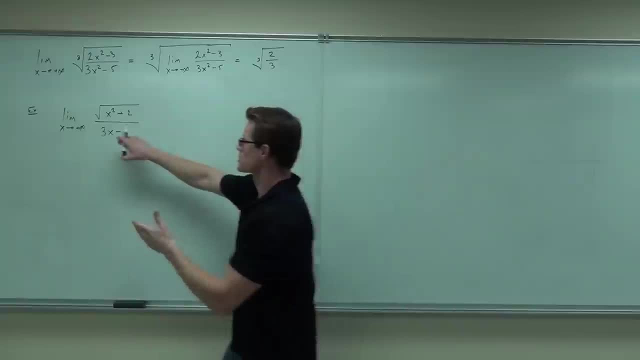 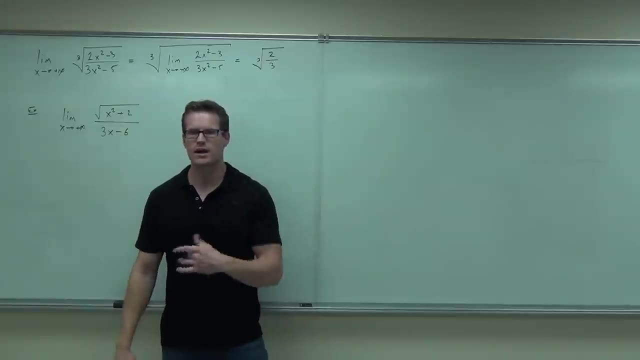 around the whole limit. No, because that square root's not around this whole function, it's just on the numerator. So, oh my gosh, well, what do we do? What do we do? Well, let's try to stick with the normal operation of this. 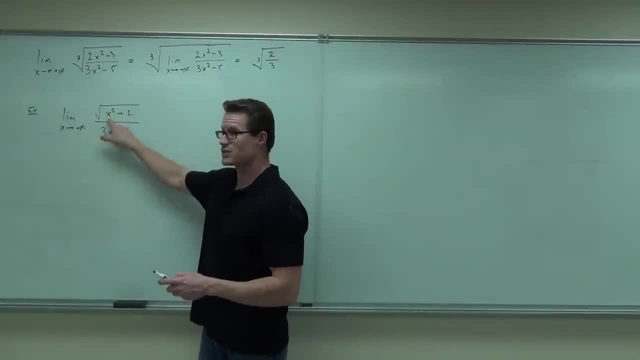 When you're taking x to infinity, we can't just go: well, that's infinity squared, Okay, that's still infinity Plus two, infinity square root's infinity over infinity One. we can't do that. But what we did say was: maybe we divide. 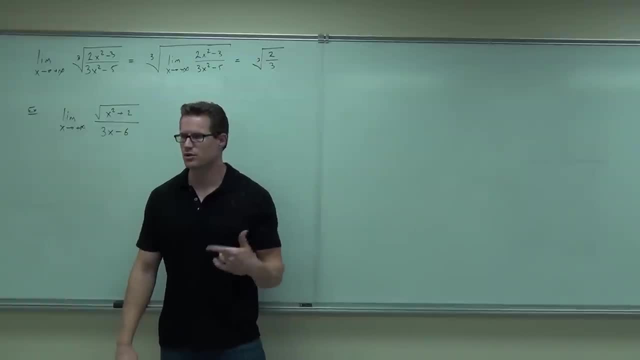 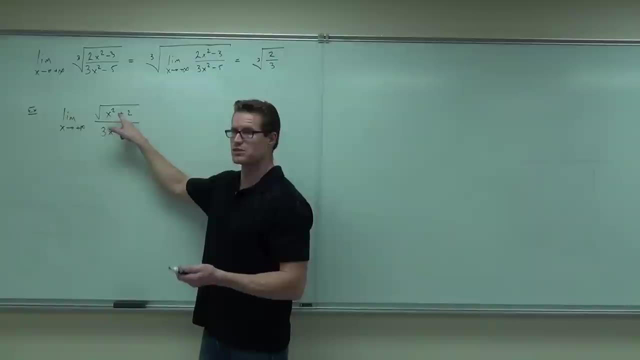 What do we do? Well, let's try to stick with the normal operation of this. When you're taking x to infinity, we can't just go. well, that's infinity squared, OK, that's still infinity Plus 2 infinity Square root is infinity over infinity. 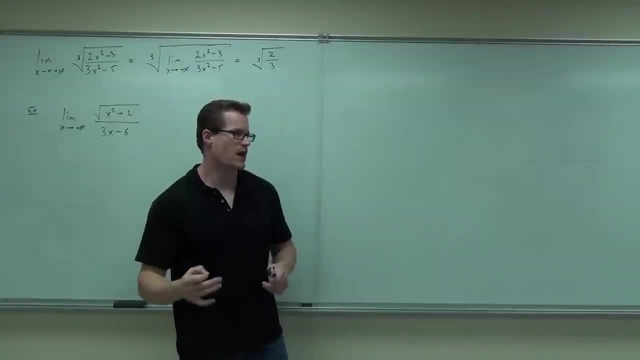 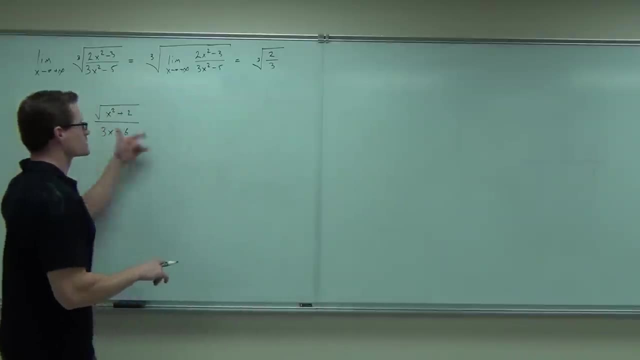 1.. We can't do that. But what we did say was: maybe we divide by the largest power of x in the denominator. So we're going to look down there What's the largest power of x in the denominator 1.. 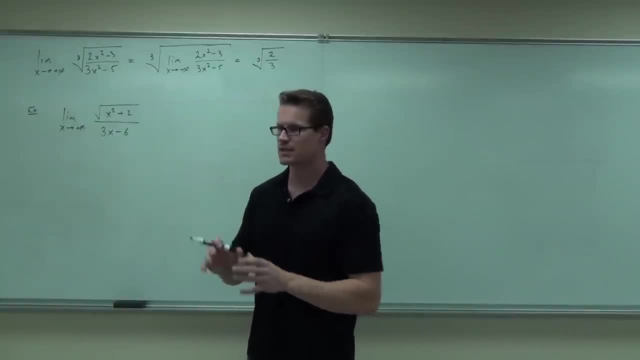 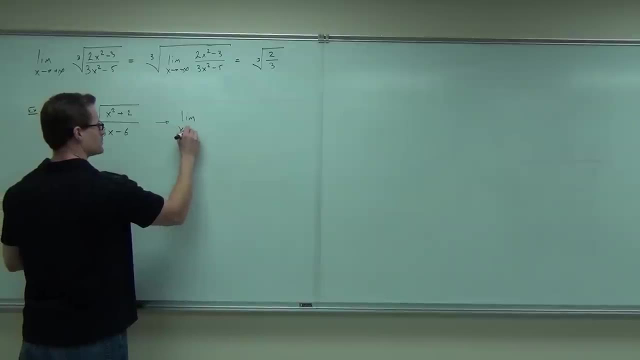 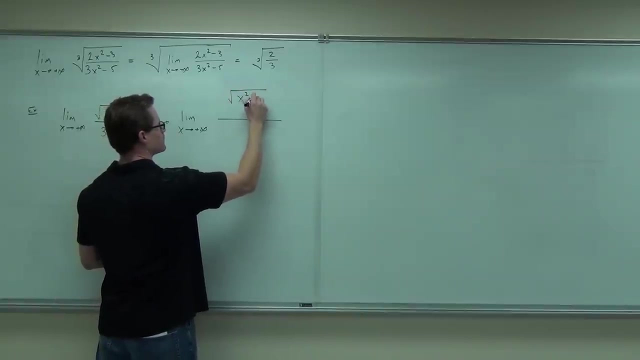 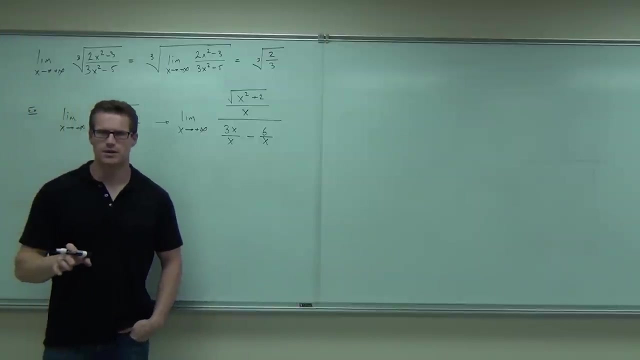 x to the first power. So let's divide the numerator and the denominator, And the denominator by x. Are you OK with that so far? Well, now here's the issue, And some of you might see this issue already. Can I just take this x inside that square root? 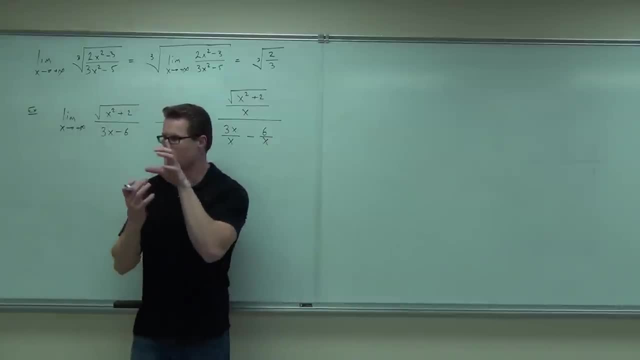 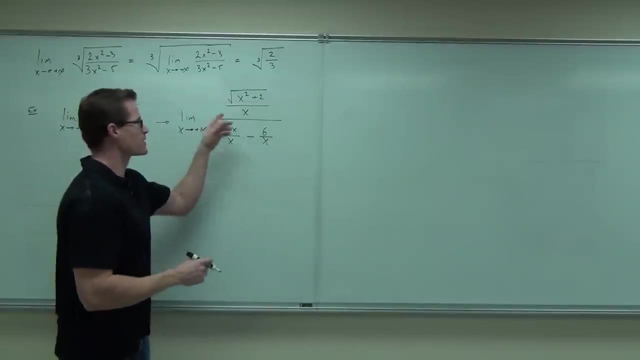 I can't, unless I have a square root. Remember: you can only combine things if you have the same exact type of root. Follow, Because it's an exponent. You can only put things together if you have the same type of exponent. Well, that's a problem. 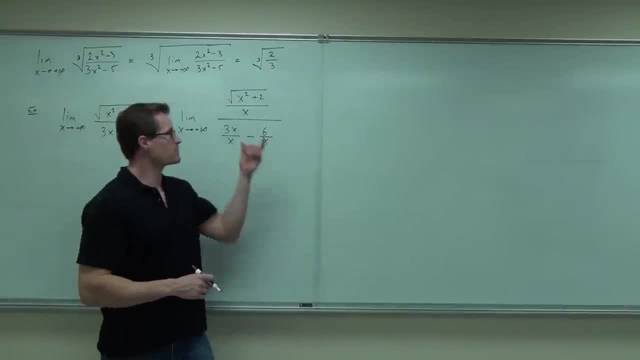 Does anyone know how to change x into something that I can take into that square root? Let's think about it for a second. Let's think about that x. What do you think? But if I do x squared, I have to change those to x squared, right? 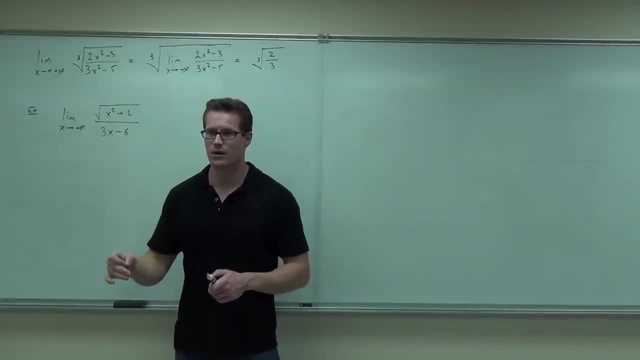 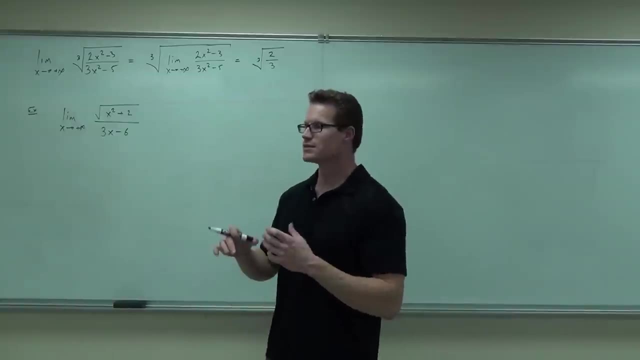 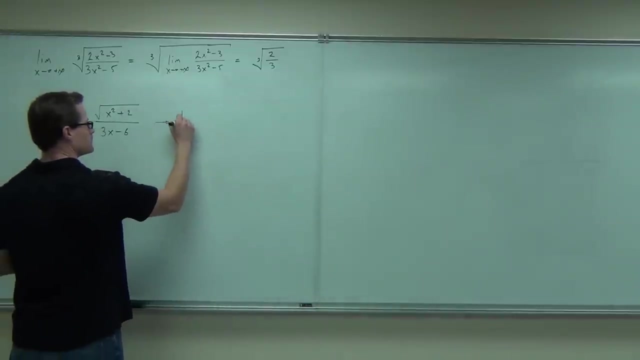 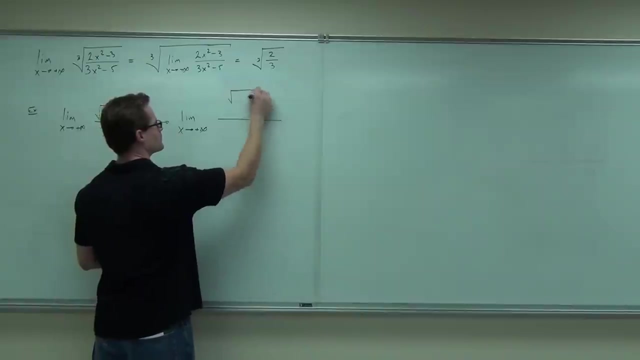 by the largest power of x in the denominator. So we're gonna look down there What's the largest power of x in the denominator: X to the first power. So let's divide the numerator and the denominator by x. Are you okay with that? so far, 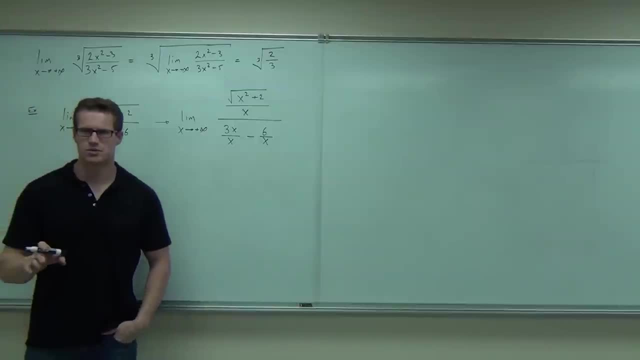 Well, now here's the issue, and some of you might see this issue already. Can I just take this x inside that square root? I can't, unless I have a square root. Remember, you can only combine things if you have the same exact type of root. 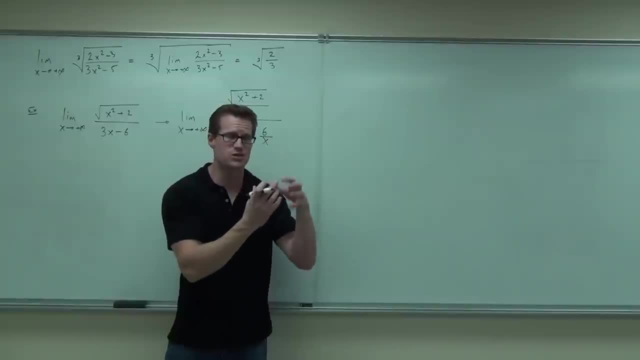 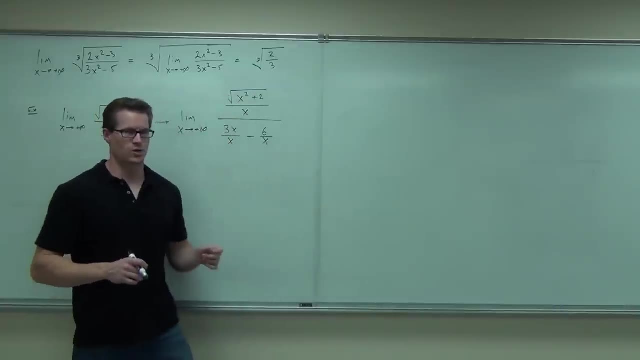 You follow Because it's an exponent. You can only put things together if you have the same type of exponent. Well, that's a problem. Does anyone know how to change x into something that I can take into that square root? Let's think about it for a second. 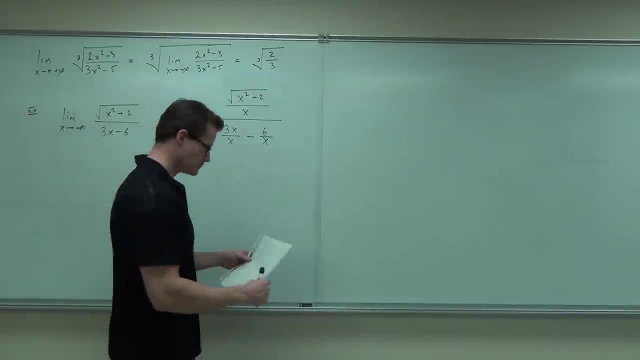 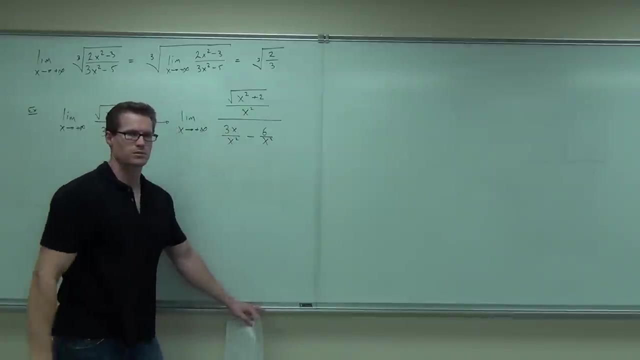 Let's think about that x. What do you think? But if I do x squared, I have to change those to x squared, right? Is that a problem? That would be zero and zero, That would be undefined. So I can't just arbitrarily change x squared. 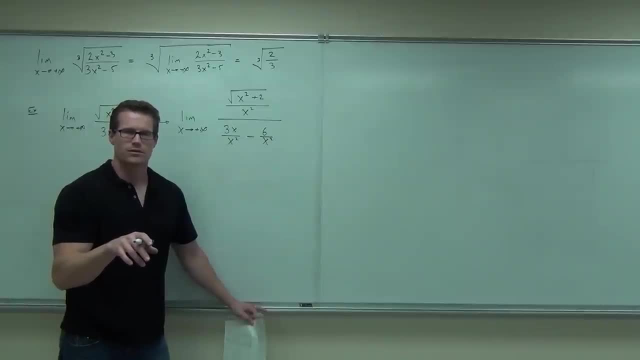 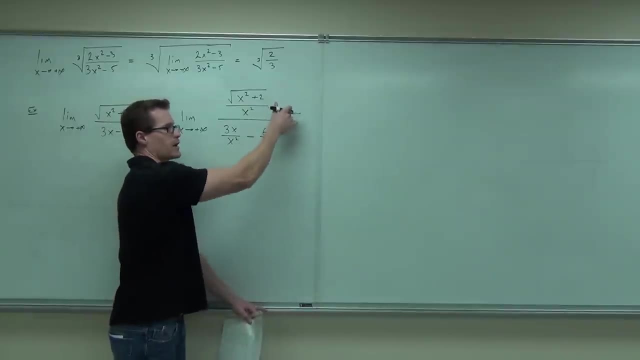 but you're on the right track, Going where Two over two. What's the two over two? Two over two is still one. What's y over x? x over y? I did one over x. I did that, So x squared down here. 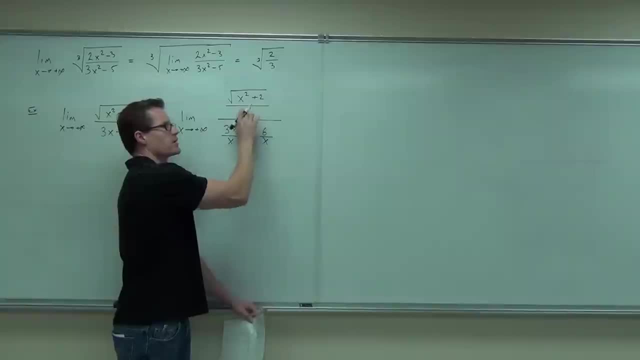 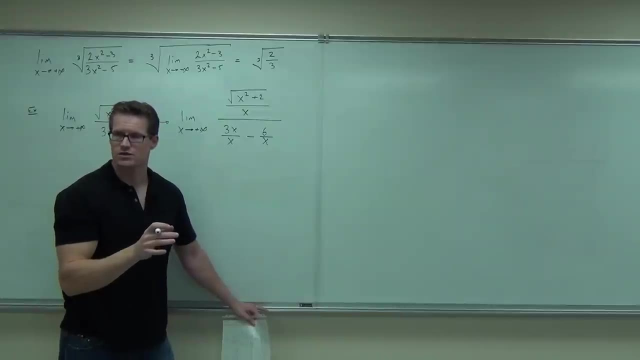 we can't have an x squared. I need this to still be a value of x. Make it a value of x squared's a great idea. x squared is x squared. x squared times. x squared is x squared If x is x to the fourth. that's too much. 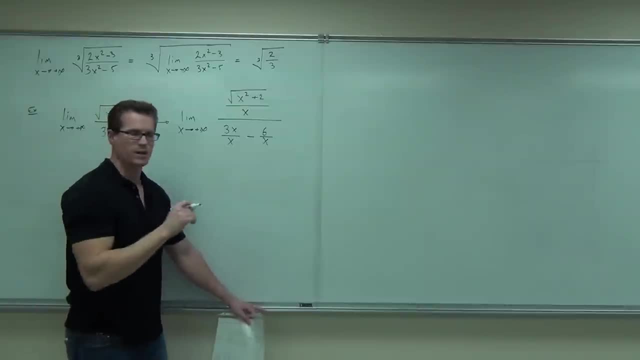 I mean x to the root of x. Say what now? Root of x times, root of x, Root of x times, root of x is still x. You're close, Oh, you're so close, You're so close. Put that together. 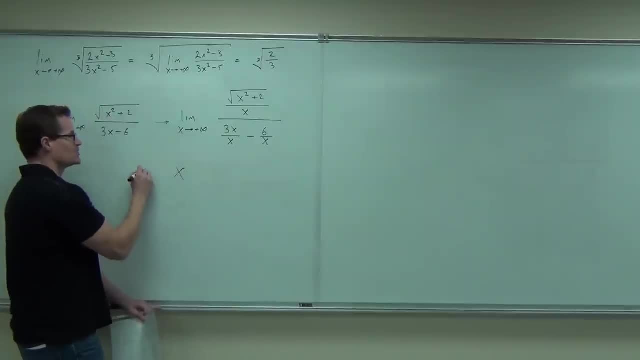 You want something that equals x, true? How do you make this equal x? Do that, And they are equal. Is that equal, Okay, No, no, but almost That's our idea, though I'm gonna fix this in a second. 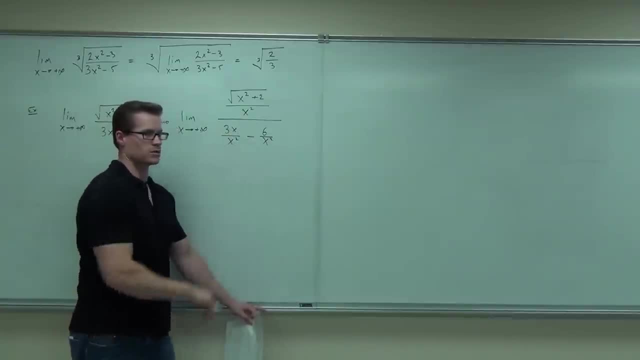 Is that a problem? That would be 0 and 0.. That would be undefined, So I can't just arbitrarily change x squared. But you're on the right track. 2 over 2 is still 1.. x over y. 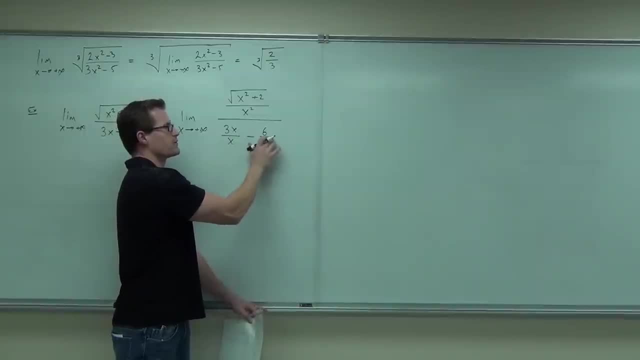 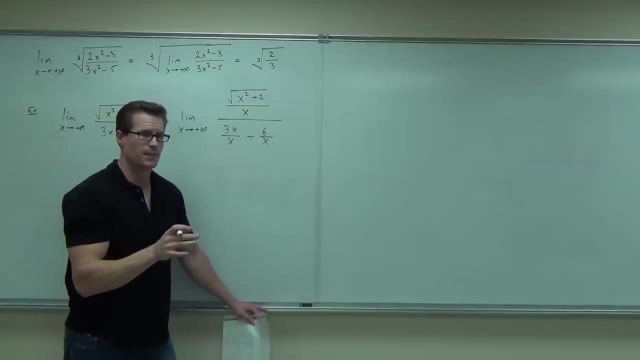 I did 1 over x. I did that, So x squared down here. We can't have an x squared. I need this to still be a value of x. Make it a value of x. X squared is a great idea. 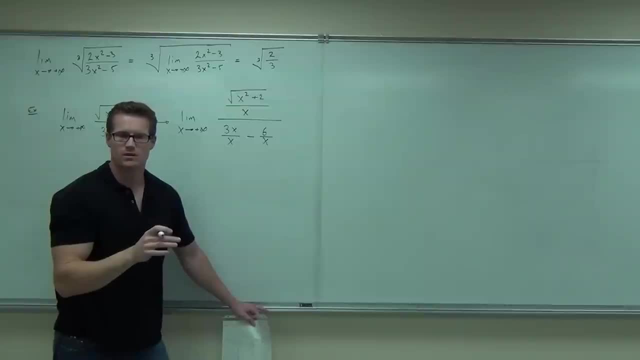 x squared times x squared is x to the fourth. That's too much. Say what now? The root of x times the root of x is still x. You're close, Oh, you're so close, You're so close. Put that together. 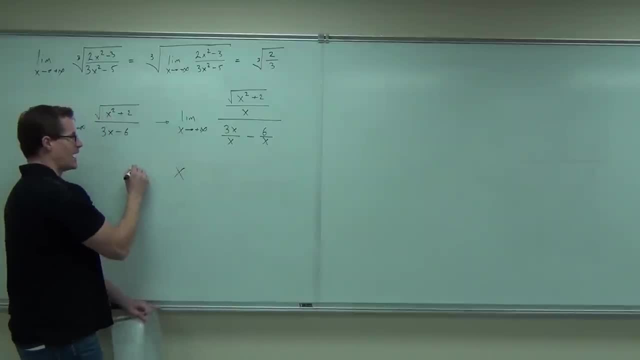 You want something that equals x. True. How do you make this equal x? Do that, And they are equal. Is that equal? OK, No, No, But almost That's our idea, though I'm going to fix this in a second. 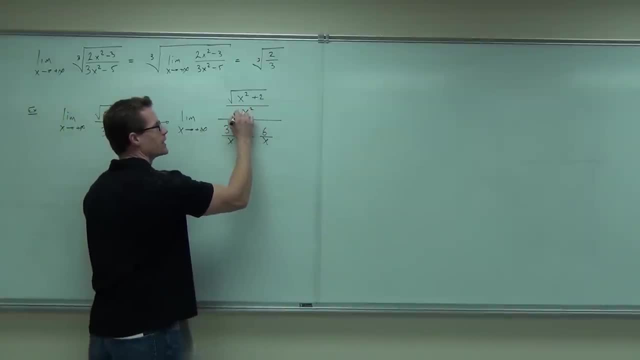 So here's the plan. I know that I need this. Do you see why I need that? That is still, well, pretty much x, Almost x, And that's going to allow me to take that into that square root. Do you follow me? 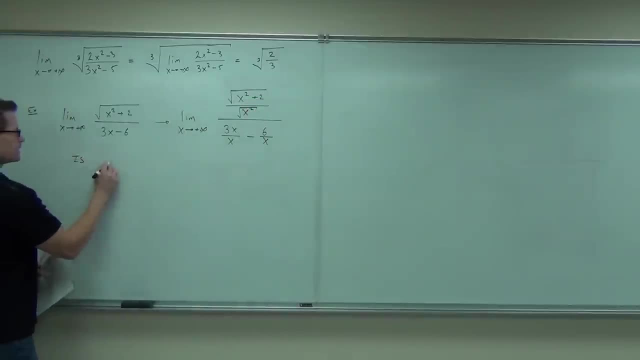 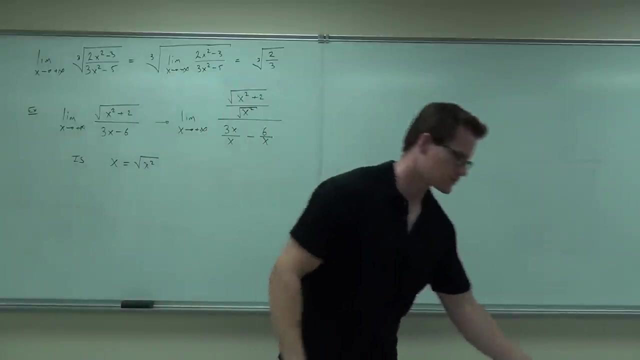 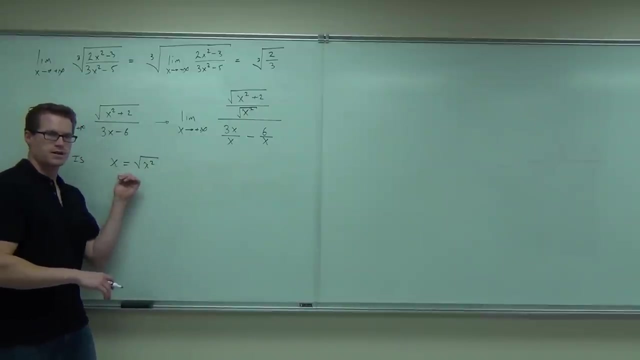 That's important. But the question is: is x equal to the square root of x squared? And the answer is no, Not really, Because if you think about it, why don't you take like a negative number, Negative 5.. Is negative 5 equal to the square root of negative 5 squared? 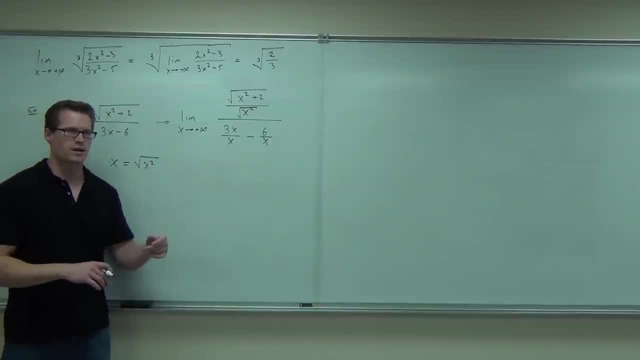 No, it's not, Because as soon as you square it, it becomes positive right. So this is not necessarily true. What is true is this: That's true. So if we have to have this, there's something that's wrong in our problem right now. 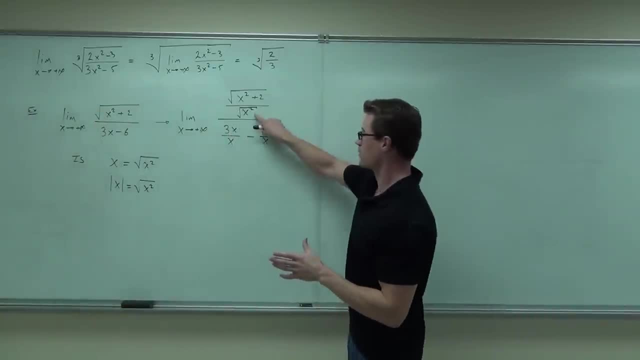 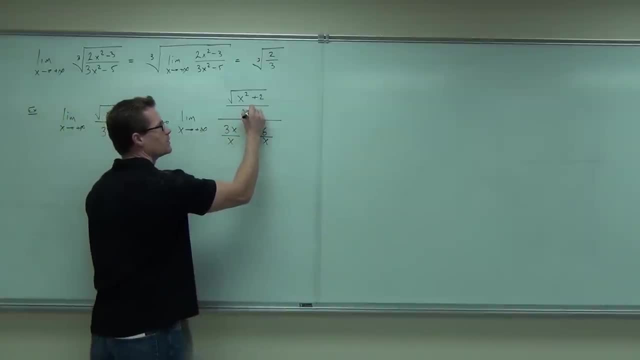 So here's the plan. Well, I know that I need this. Do you see why I need that? That is still, well, pretty much x, almost x, And that's gonna allow me to take that into that square root. 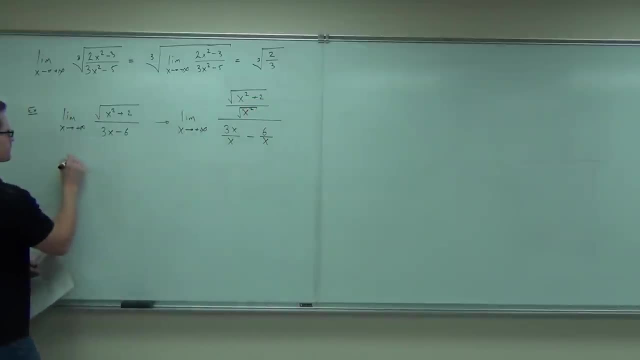 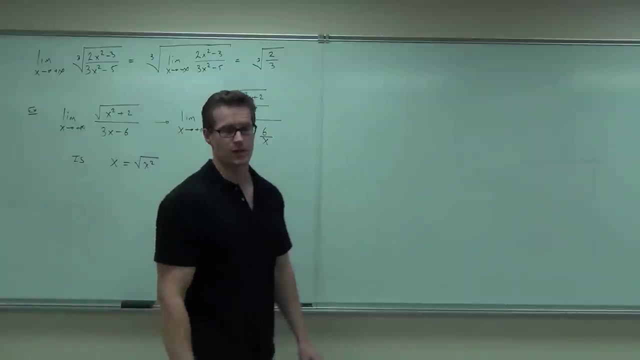 Do you follow me? That's important. But the question is: is x equal to the square root of x, The square root of x squared? And the answer is no, Not really. Because, if you think about it, why don't you take like a negative number? 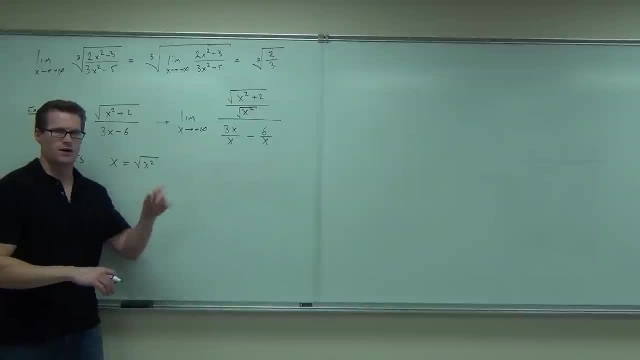 Negative five. Is negative five equal to the square root of negative five squared? No, it's not, Because as soon as you square it, it becomes positive right. So this is not necessarily true. What is true is this: That's true. 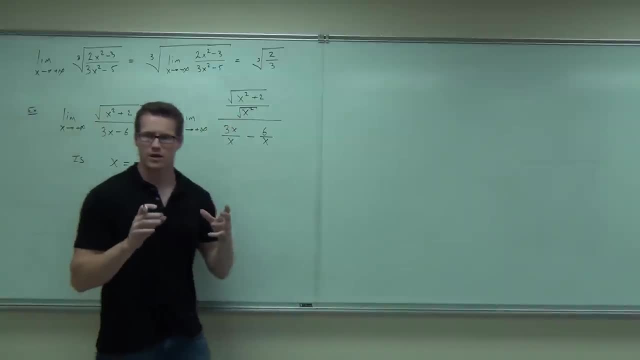 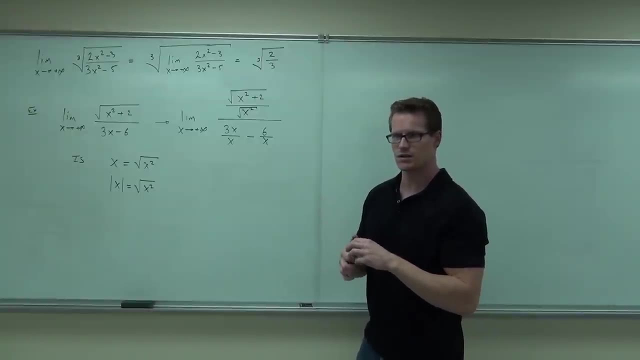 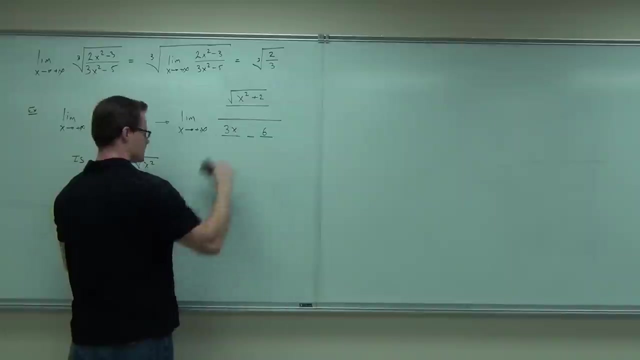 So if we have to have this, there's something that's wrong in our problem right Now. this is right. What is wrong? Do you see it? You don't see it. Let me go through the process one more time. 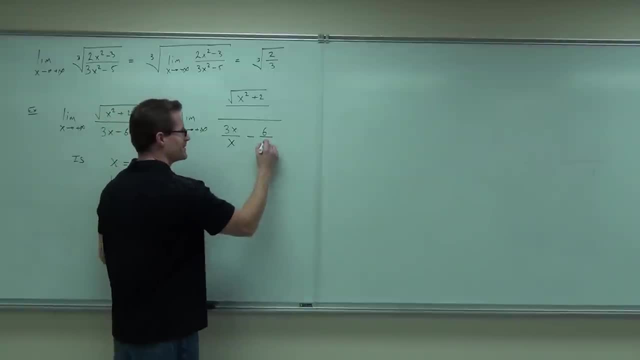 You knew, maybe if I draw in purple it'll make more sense. You knew if you you had to do that right, But you knew that this wouldn't work. So to try to make it equivalent, you did this. 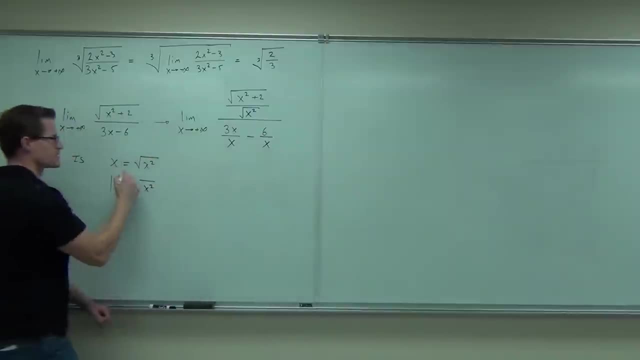 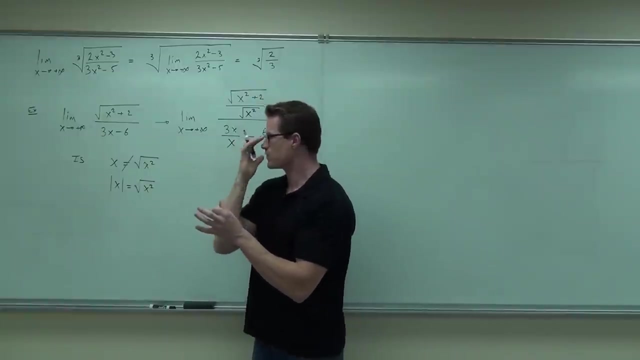 That would go into the square root. However, this fails now because this is not equal. That's not equal. Notice, you're trying to divide everything by the same thing, right, The same thing. So if you have divided by the same thing, 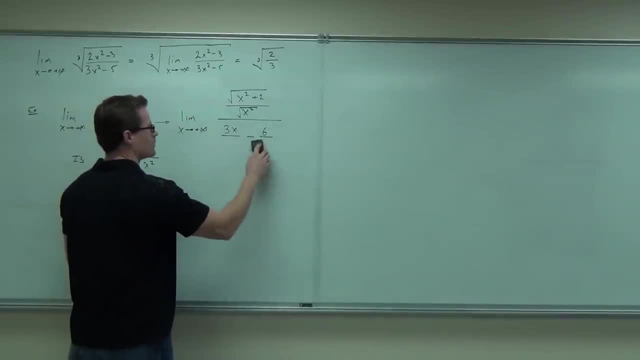 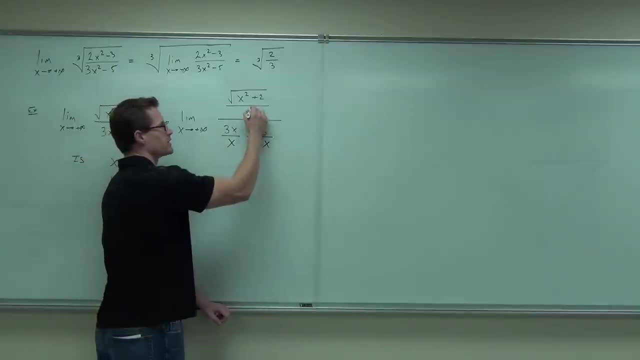 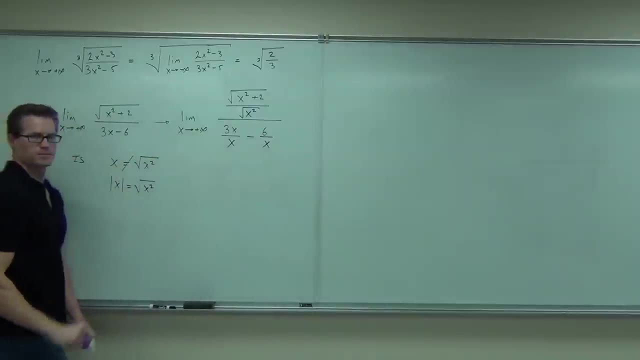 But you knew that this wouldn't work, So, to try to make an equivalent, you did this. That would go into the square root. However, this fails now because this is not equal. Notice: you're trying to divide everything by the same thing, right? 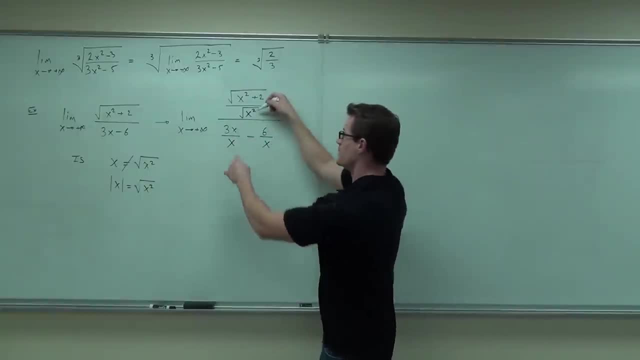 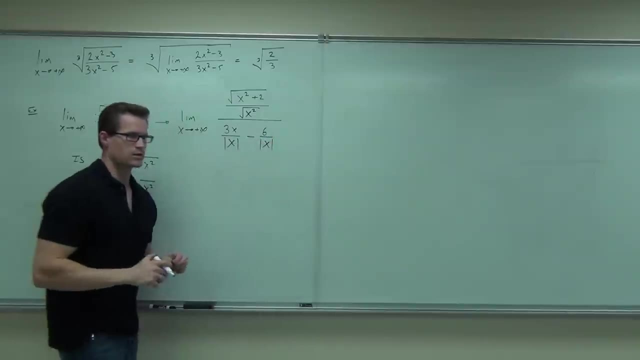 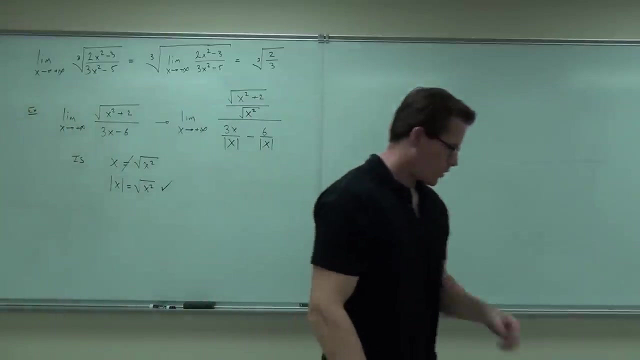 The same thing. So if you have divided by the same thing, these are not the same thing. This Is the same thing. that's true, This is true. yes, this is not true, not necessarily true. So are the absolute value important? 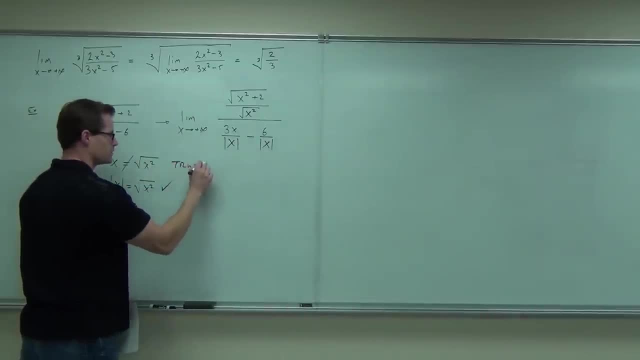 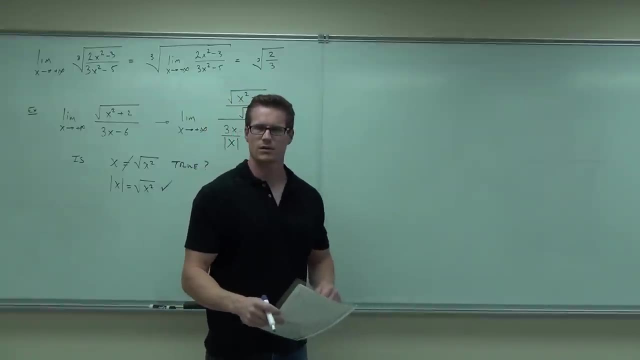 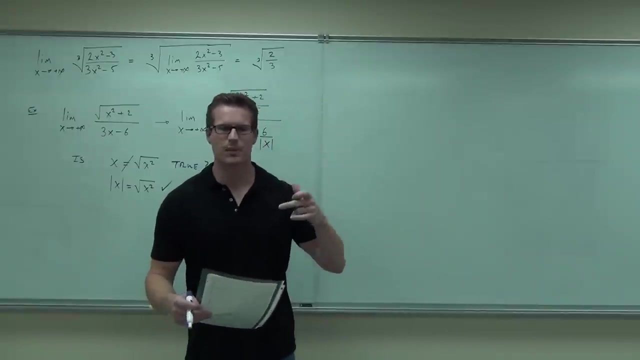 This is almost true. is this true? Well, no, almost, this is true. You ready to keep going? Did you understand that idea right now? You sure? Okay, so when we take the square root of x squared, we can't just have x. 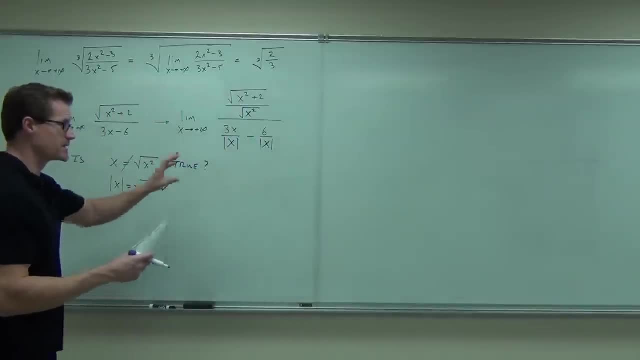 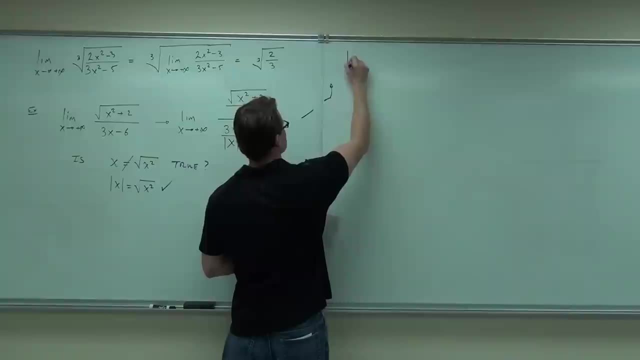 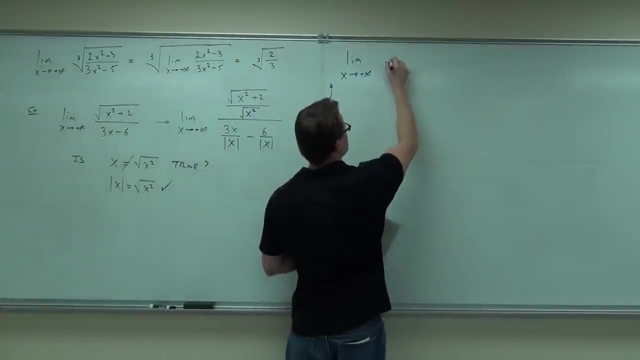 you have to have the absolute value of x, And I'll show you why it's important in maybe 10 minutes. For right now, let's continue working on this problem. When you have a square root over a square root, that says you can take a square root of the whole entire fraction. 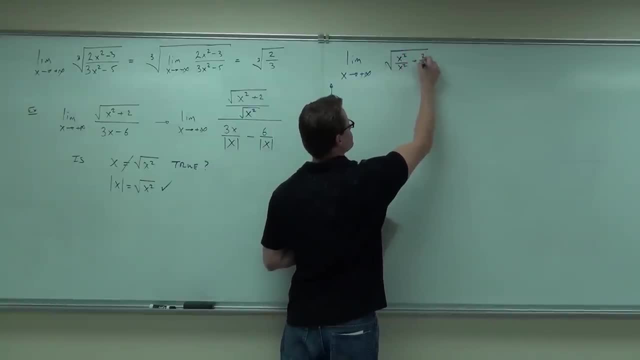 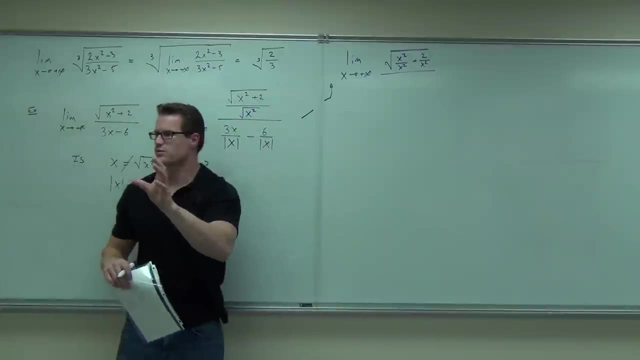 That's x squared over x squared plus 2 over x squared. Are you okay? You can't where the x squared over x squared and 2 over x squared are coming from. That's the sole reason why you did that right. Just to make that in there. 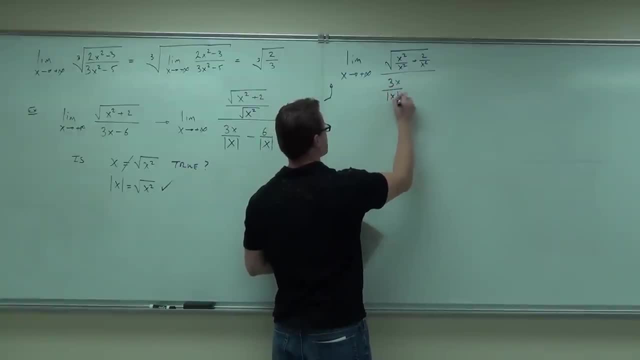 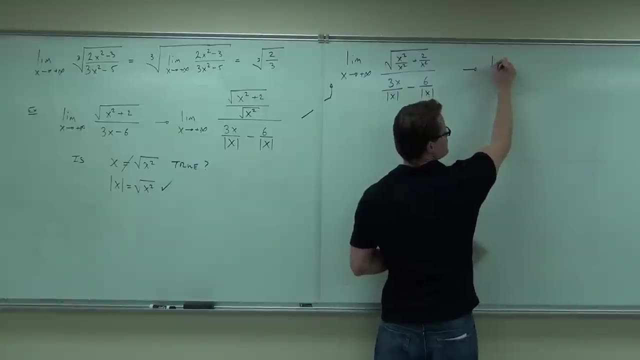 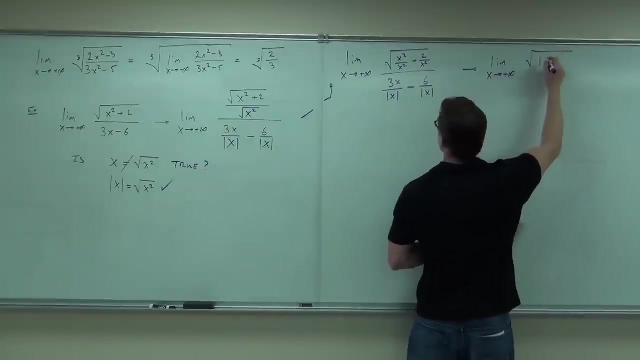 Over 3x over the absolute value of x, minus 6 over the absolute value of x. Well, that's a limit. x goes to positive infinity. You're going to have the square root of 1 plus 2 over x squared. 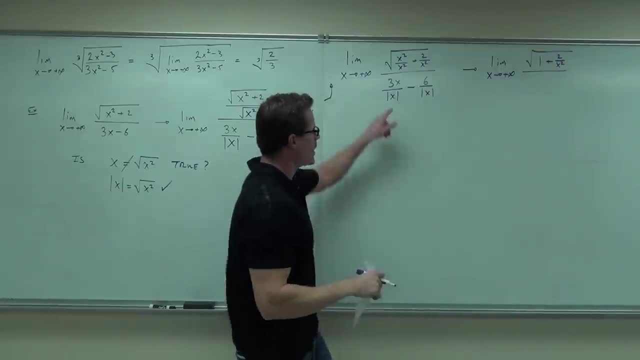 That's the sum of all the squared parts. Oh, okay, Okay, Now we got to deal with that. I need your minds to think back to what it means to be an absolute value. Absolute value is actually a piecewise function. The piecewise function says: if x is positive, you leave it alone. 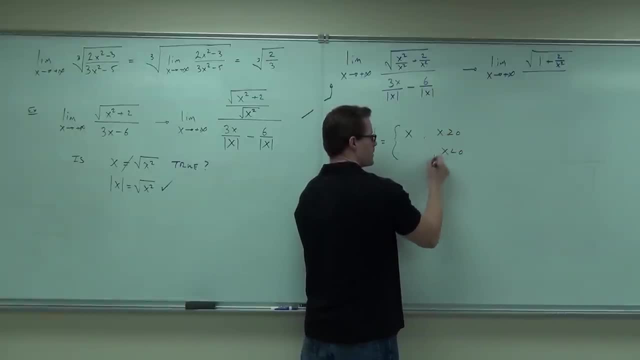 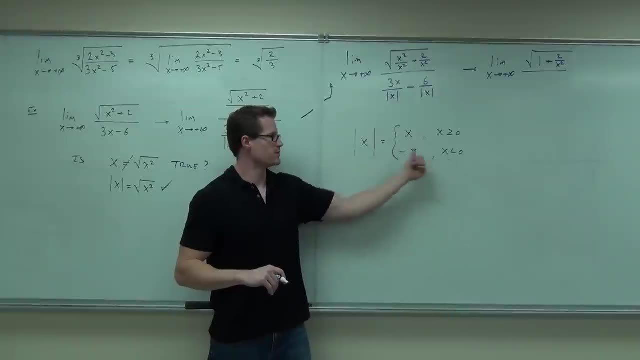 if X is negative, you change the sign. does that make sense to you? if X is positive, positive, you leave it alone. if X is negative, you change the sign. and that was the whole idea. that's the piecewise definition of absolute value. remember that I think we did in here, actually. well, this is how you apply that. 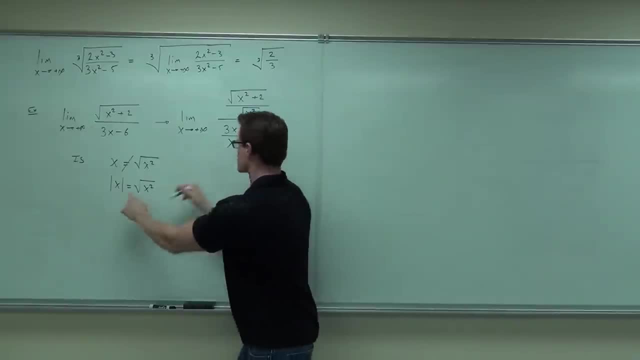 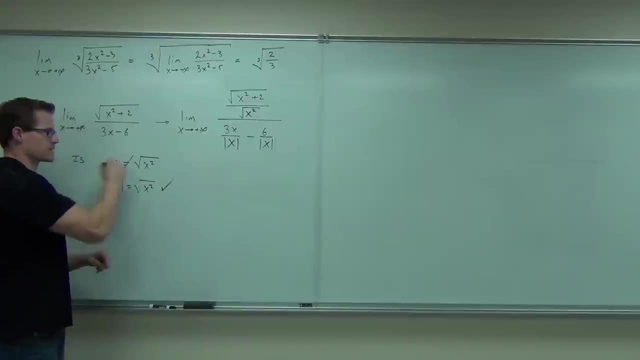 these are not the same thing. This is the same thing. That's true, This is true. Yes, this is not true, Not necessarily true. So are the absolute value important? This is almost true. Is this true? Well, no, almost. 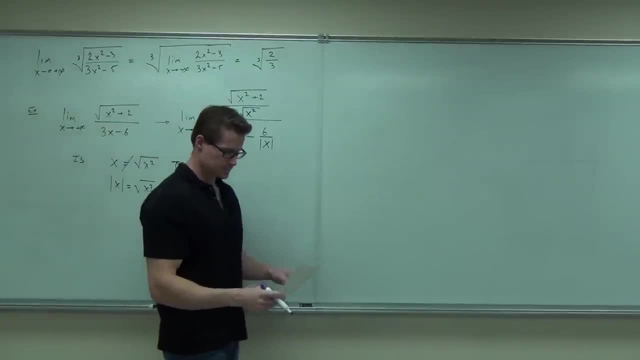 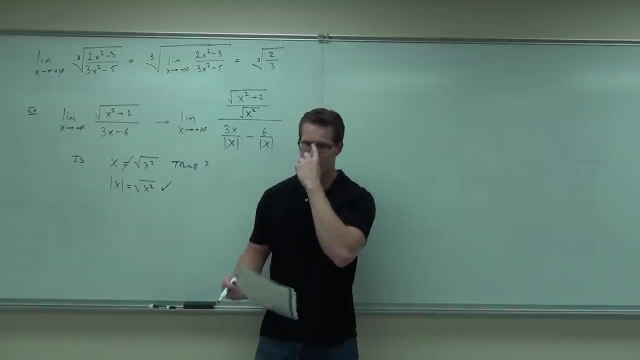 This is true. You ready to keep going? Did you understand that idea right now? You sure, Okay. so when we take the square root of x squared, we can't just have x, You have to have the absolute value of x. 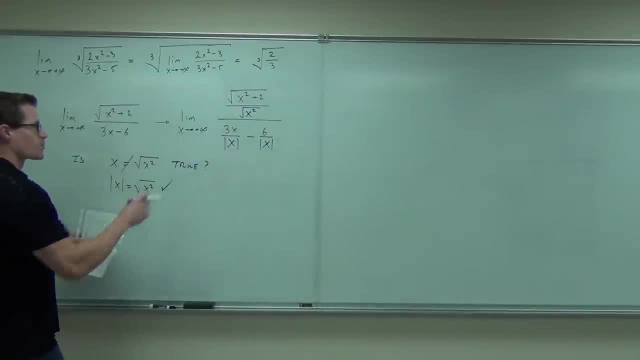 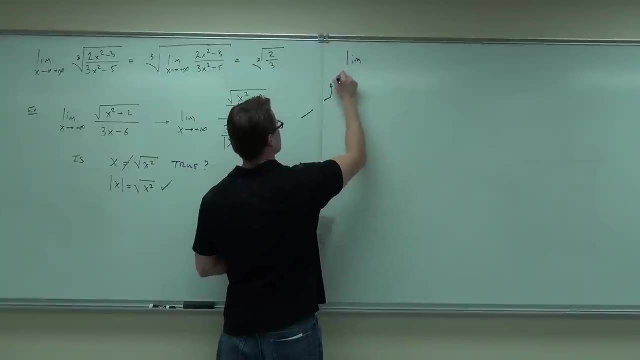 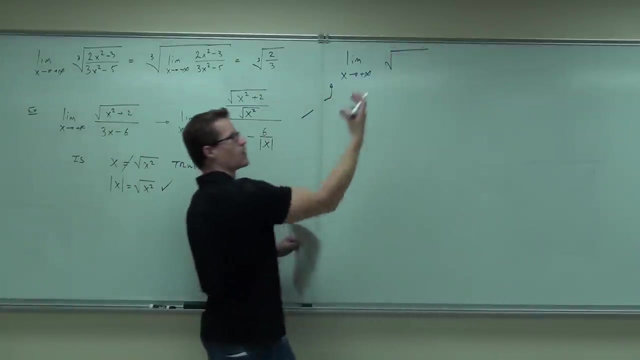 And I'll show you why it's important in maybe 10 minutes. For right now, let's continue working on this problem. When you have a square root over a square root, that says you can take a square root of the whole entire fraction. 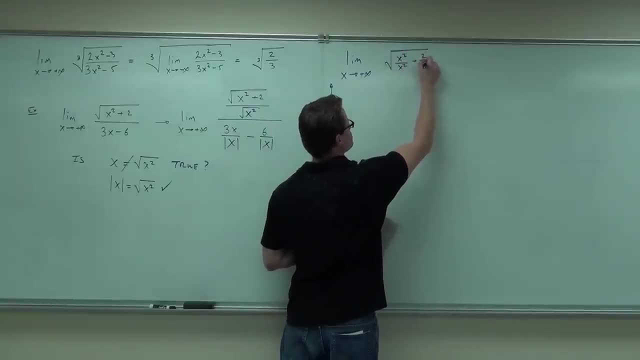 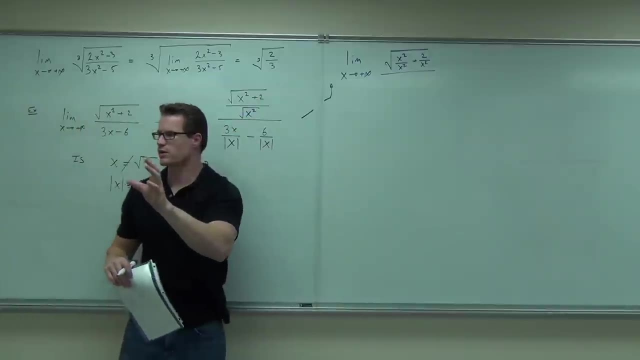 That's x squared over x squared plus two over x squared. Are you okay on where the x squared over x squared and two over x squared are coming from? That's the sole reason why you did that right. Just to make that in there. 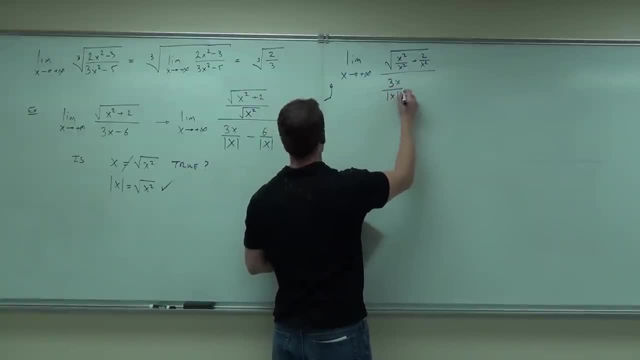 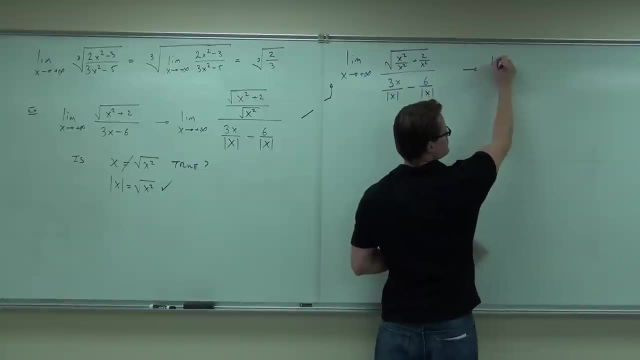 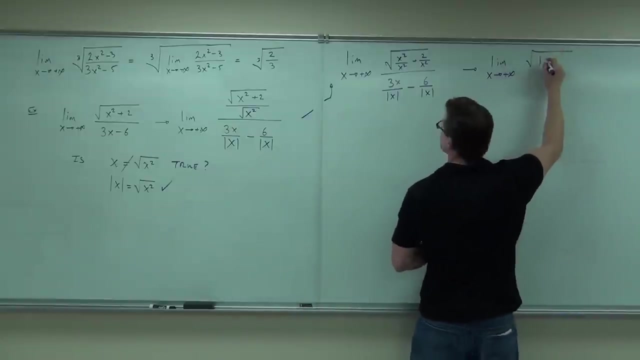 Over three, x over the absolute value of x, minus six over the absolute value of x. Okay, Okay. Well, that's a limit. X goes to positive infinity. You're gonna have the square root of one plus two over x squared. Oh, okay, okay. 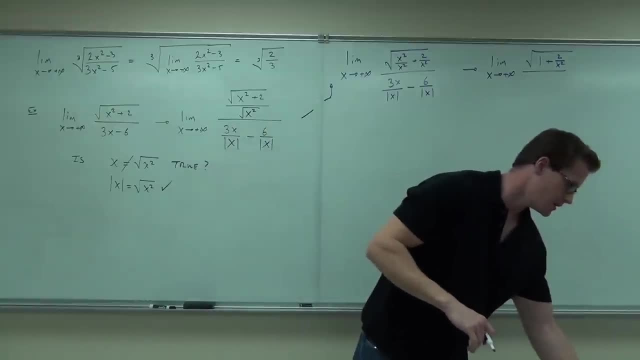 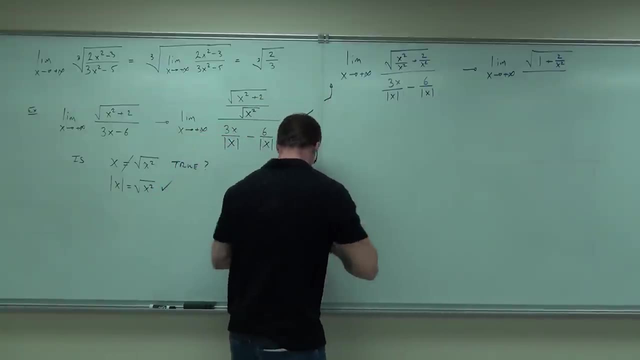 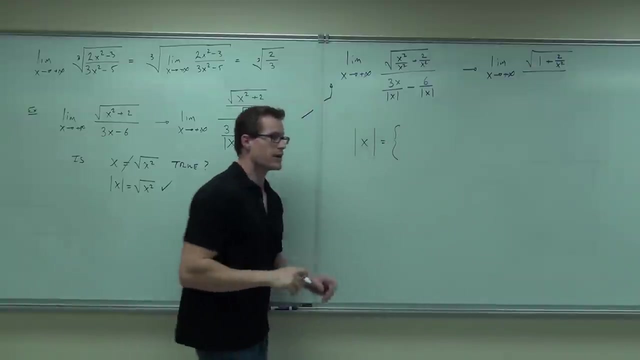 Now we gotta deal with that. I need your minds to think back to what it means to be an absolute value. Is an absolute value the value of a positive value? The absolute value is actually a piecewise function. The piecewise function says: if x is positive, 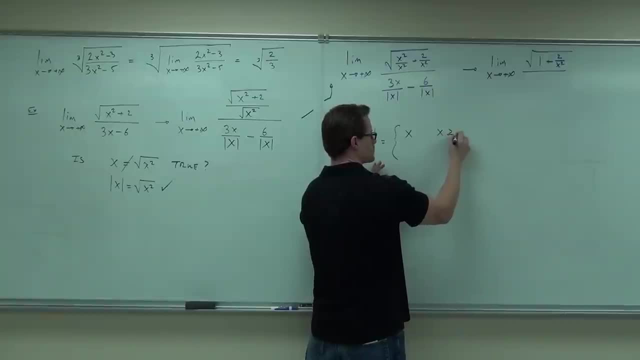 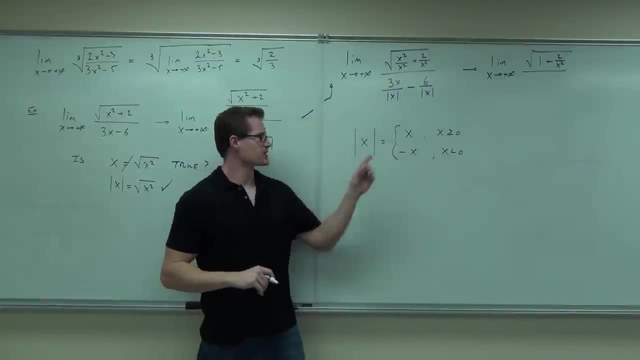 you leave it alone. If x is negative, you change the sign. Does that make sense to you? If x is positive, positive you leave it alone. If x is negative, you change the sign. And that was the whole idea. 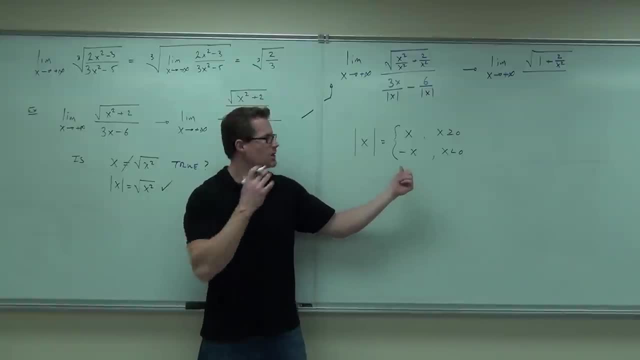 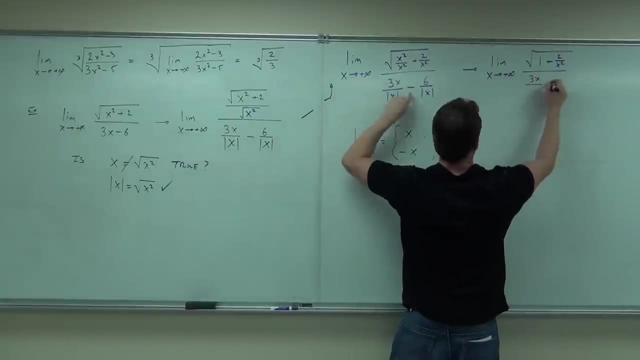 That's the piecewise definition of the absolute value. Do you remember that I think we did in here here actually? Well, this is how you apply that. We are going to have the 3x over minus 6 over. 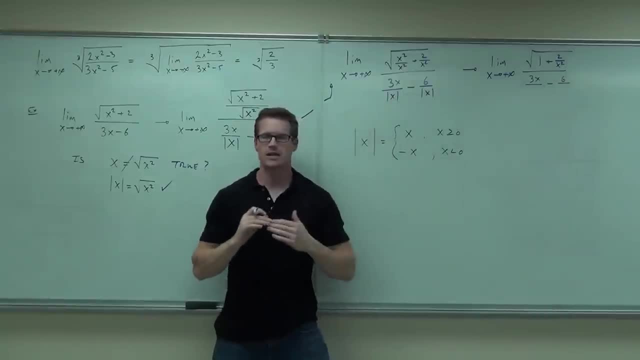 Now you get to change your absolute value of x depending on where you are going, whether you're going to positive infinity or negative infinity. Where are we going To positive numbers or negative numbers? Positive numbers- We're going to. positive numbers- say that absolute value of x equals x. 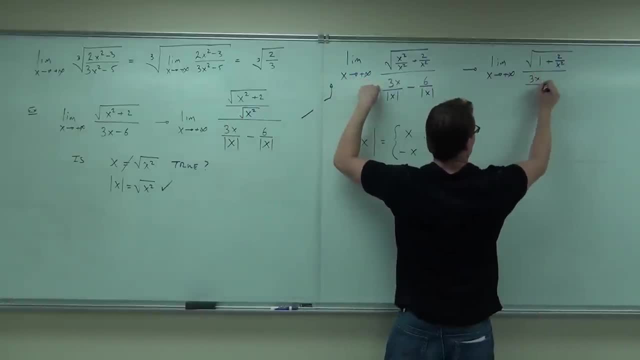 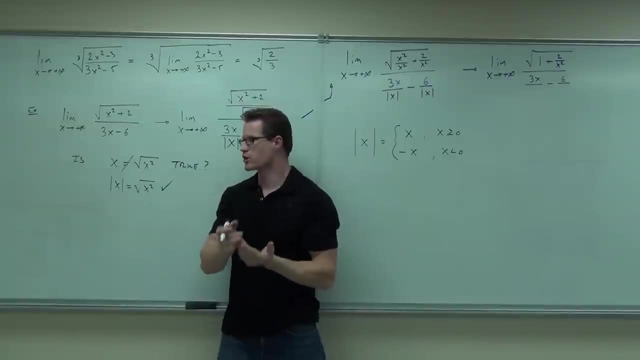 we are going to have the 3x over minus 6 over. now you get to change your absolute value X depending on where you are going, whether you go into positive infinity or negative infinity. where are we going to positive numbers or negative numbers? we're going to positive. no positive numbers say that absolute value. 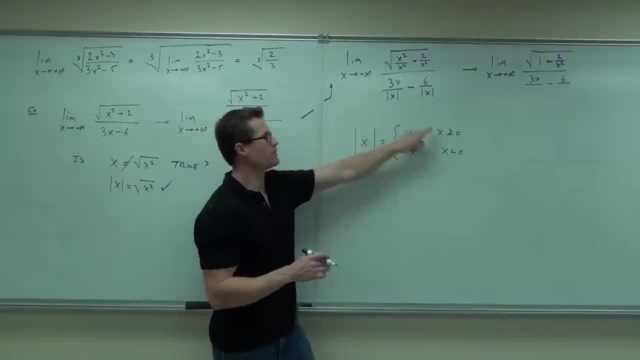 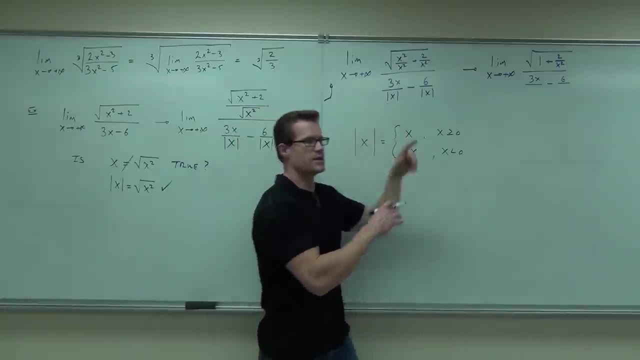 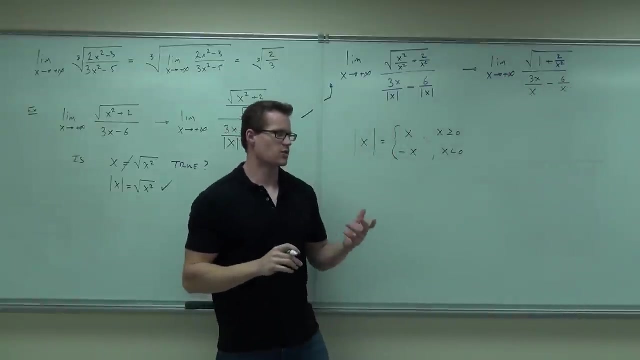 of X equals X. positive numbers. positive numbers say that absolute value of X equals X. are you with me on this? absolutely love X. you whom he doesn't I. you know that since I'm going to positive numbers, that can become the X. It might seem trivial like well. 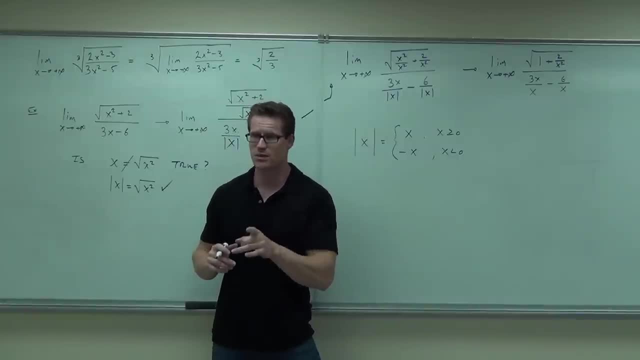 if it's just gonna change to x anyway, why do we need the absolute value? Trust me, you need them. I'll show you why in a couple minutes. okay, Yeah, in like five minutes, But you're gonna feel okay with that so far. 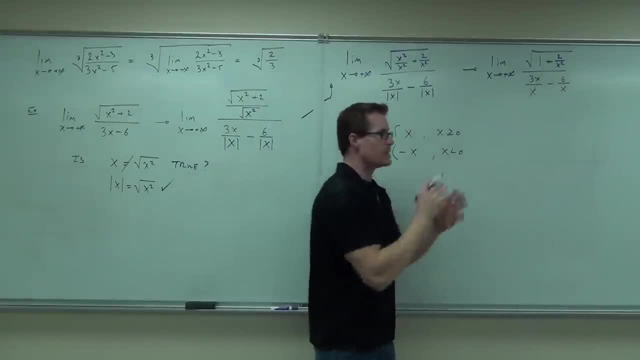 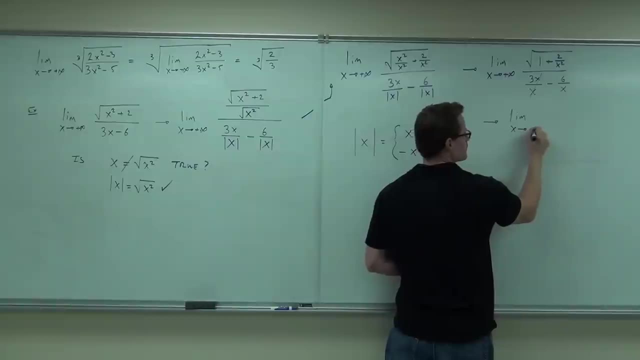 You see, now that we have that, those x's do match up, Those x's are gone. You get a limit to positive infinity. One plus two over x, squared all over three minus six over x. Tell me some nice things that happen. 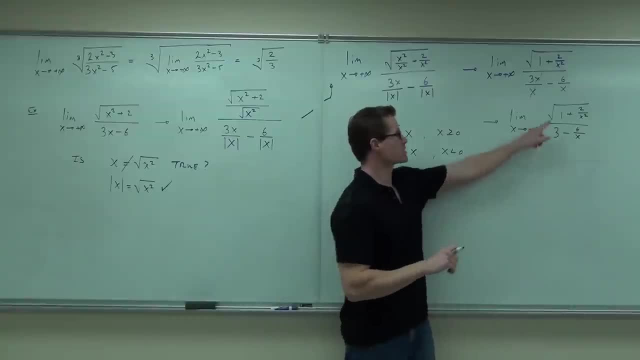 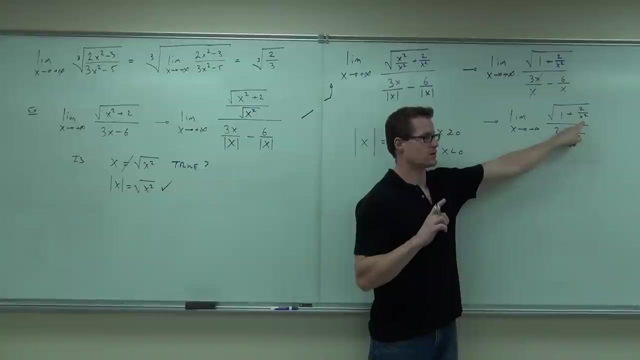 since x's go into a positive infinity. Tell me what happens. Where does this go? Not zero, This the one. The one goes to one. It's a constant. Do constants go anywhere? No, Where does this go? Where does the fraction go? 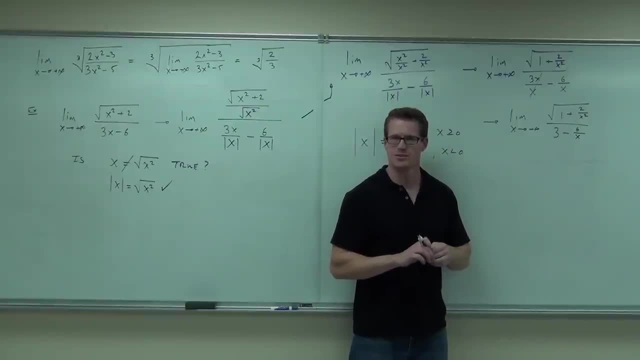 Have we lost it all? You're scaring me, Oh, you're scaring me here. Limits of constants are constants. Limits of this is not undefined. Where's x going? X is going to infinity. Where's this fraction going? 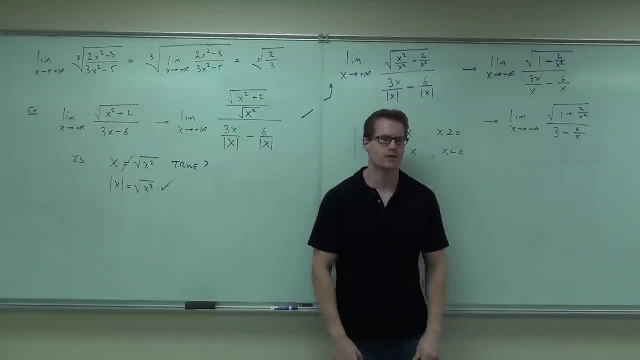 Zero. Constant over infinity is zero. Divide a constant by infinity, How much are you gonna get? Zero, Zero. Think about that. come on, Where's three going Nowhere? Three, okay, Where's this going Zero. 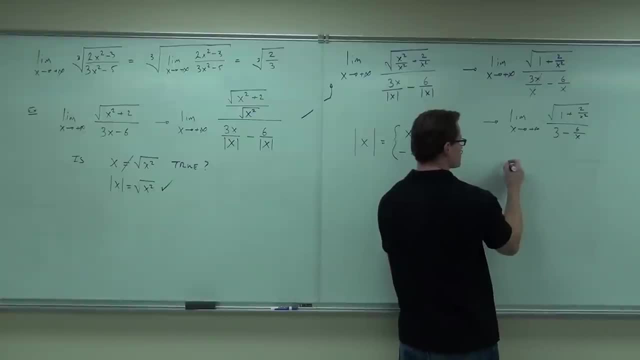 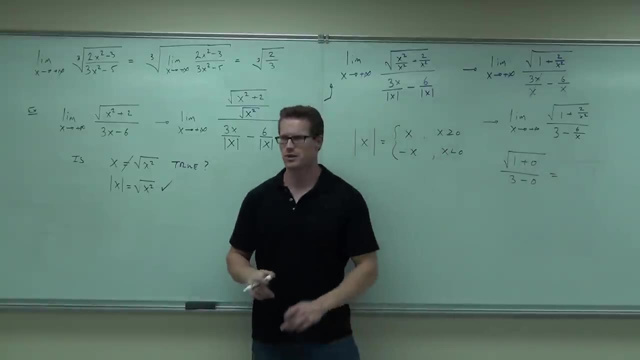 Zero. Don't forget what we did last time. This says you're gonna do one plus zero over three minus zero. Tell me my final answer please. What is that? One over zero. Are you okay in getting a zero in the zero? 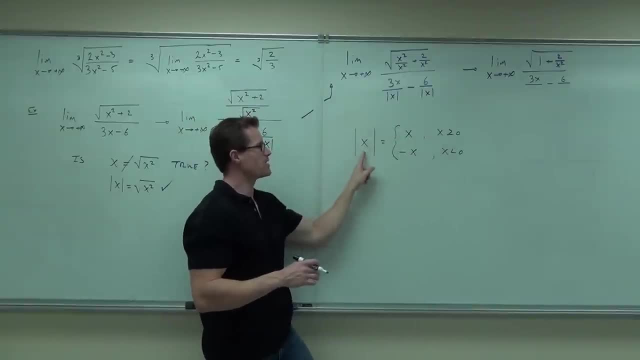 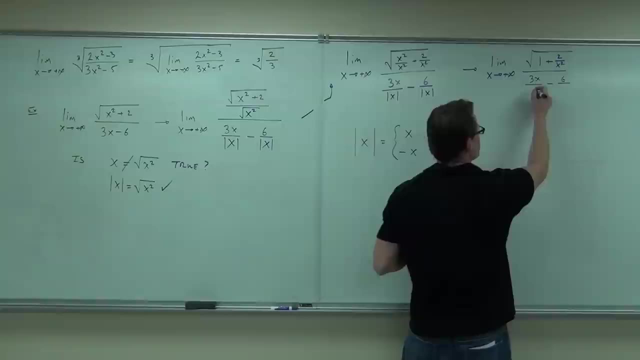 Are you with me on this Absolute value of x? Now, you don't need the absolute value. You just know that since I'm going to positive numbers, that can become the x, It might seem trivial: like well, if it's just going to change to x anyway, why do we need the absolute value? Trust me, you need them. 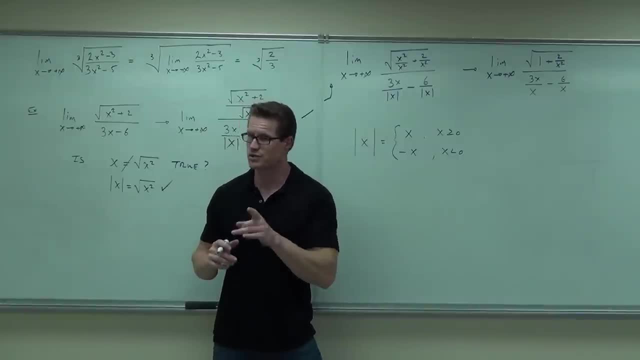 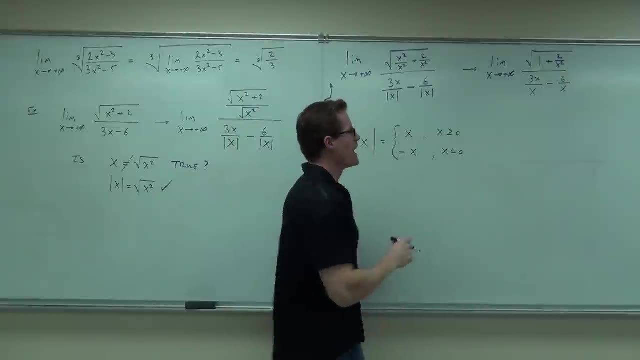 I'll show you why in a couple of minutes. okay, Now I'm like five minutes. Are you going to feel okay with that? so far, You see, now that we have that, those x's do match up, Those x's do match up, Those x's do match up. Now I'm going to show you why. 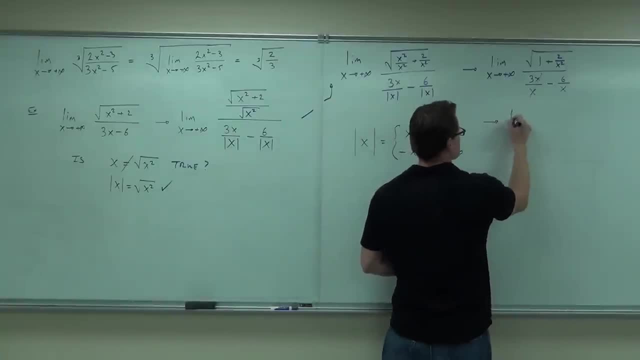 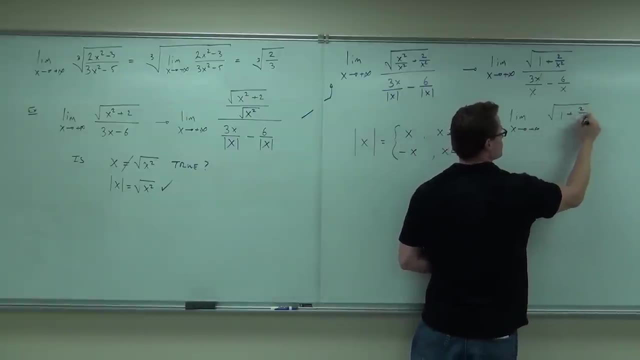 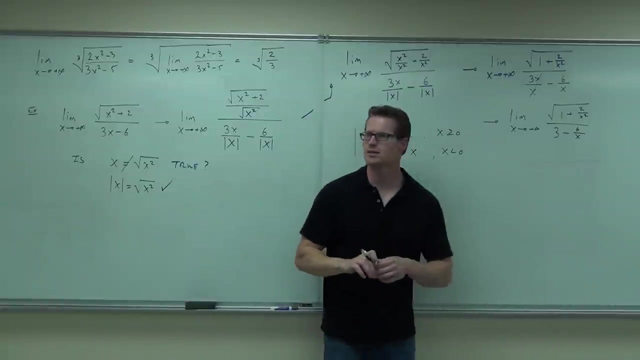 Since x's are gone, you get a limit to positive infinity. One plus two over x, squared all over three minus six over x. Tell me some nice things that happen since x's go into positive infinity. Tell me what happens. Where does this go? Zero, Not zero. One, This The one. 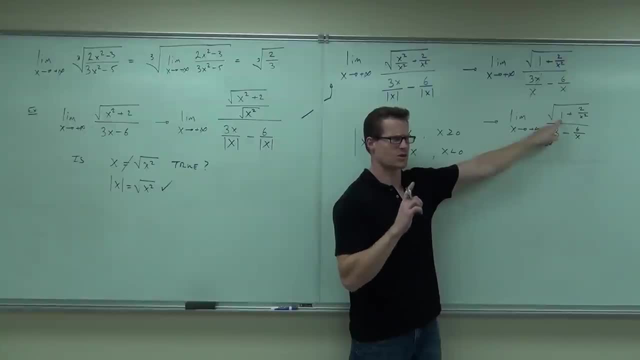 The one goes to one. It's constant. Do constants go anywhere? No, No. Where does this go? Where does the fraction go? Zero, Have we lost it all? Oh gee, You're scaring me, people, You're scaring me here. 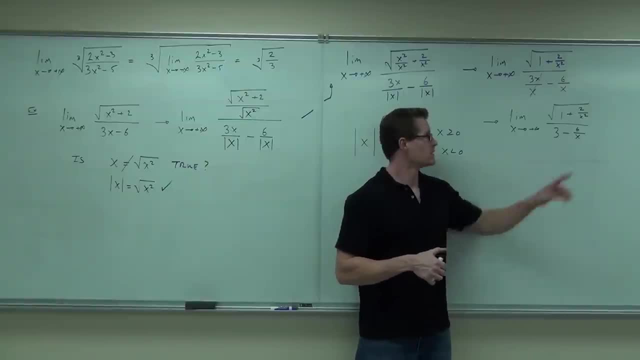 Limits of constants are constants. Limits of this is not undefined. Where is x going? X is going to infinity. Where is this fraction going? Zero, A constant over infinity is zero. Divide a constant by infinity, How much are you going to get? 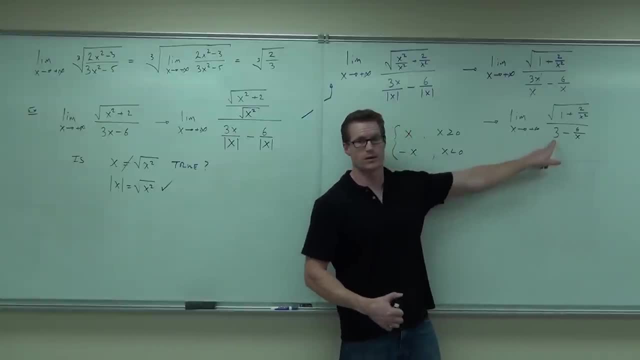 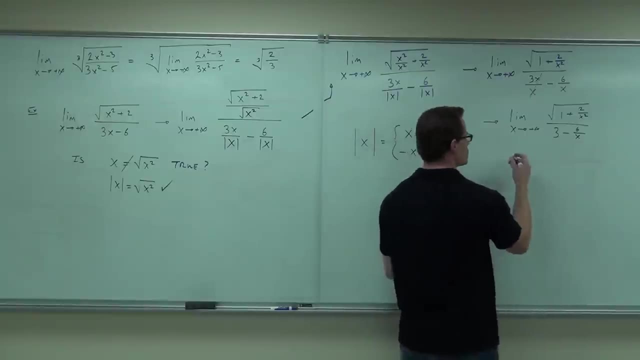 Zero, Zero. Think about that. Come on, Where's three going? Three, Three. Okay. Where's this going? Zero, Zero. Don't forget what we did last time. This says you're going to do one plus zero over three minus zero. 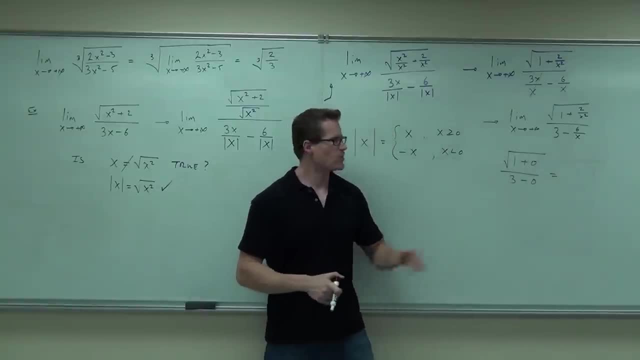 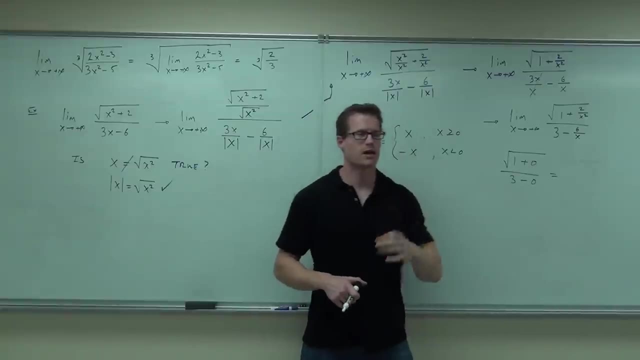 Tell me my final answer, please. What is that? One over zero? Are you okay getting the zero and the zero? I think we talked about that last time- A constant over any power of x. as x approaches infinity is going to be zero. 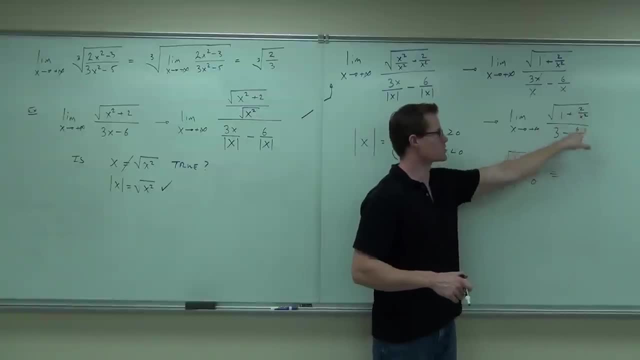 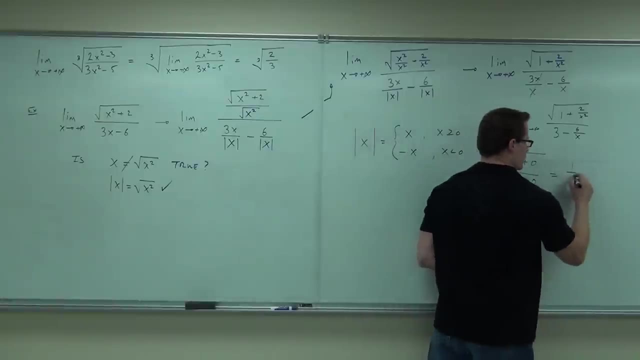 Because this number is getting huge And this number is getting huge And those numbers are staying the same. That means you're going to have a number over huge. A number over huge is zero, One third, Not the square root of one. 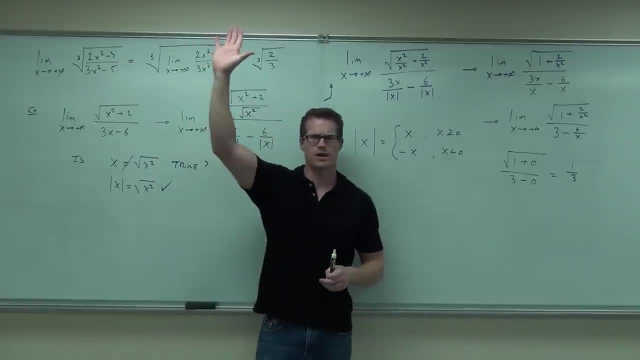 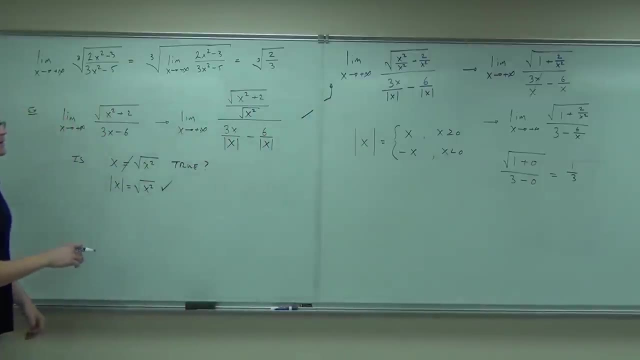 Okay, One third Show of hands. how many of you feel okay with that? Now I want you to consider this: Why this is important. Think about it. You can change your problem if you want to. I'm not going to do the whole example over again. 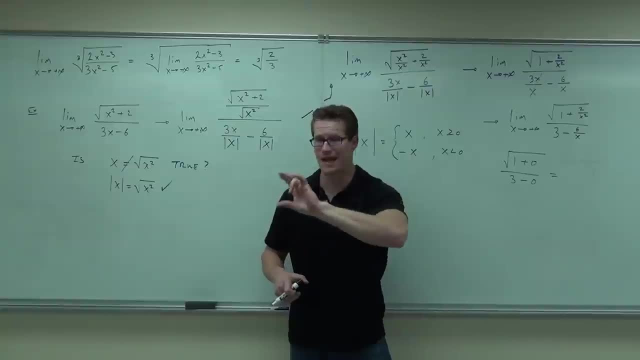 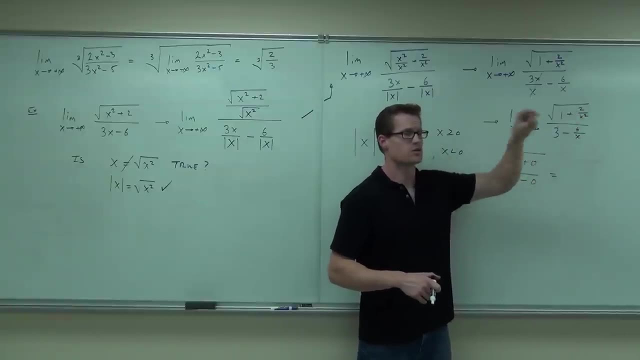 I think we talked about that last time. A constant over any power of x as x approaches infinity is gonna be zero, Because this number's getting huge and this number's getting huge and those numbers are staying the same. That means you're gonna have a number over huge. 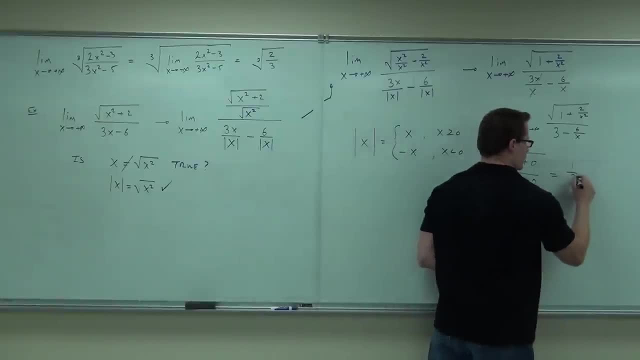 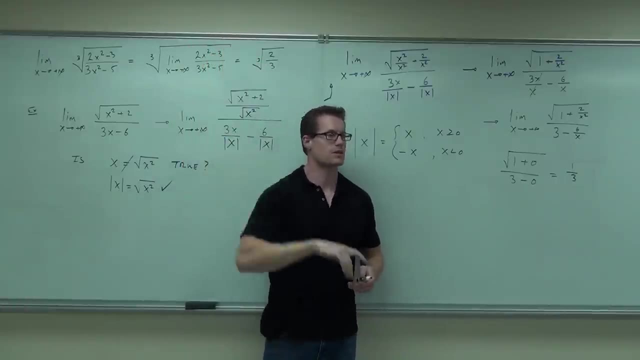 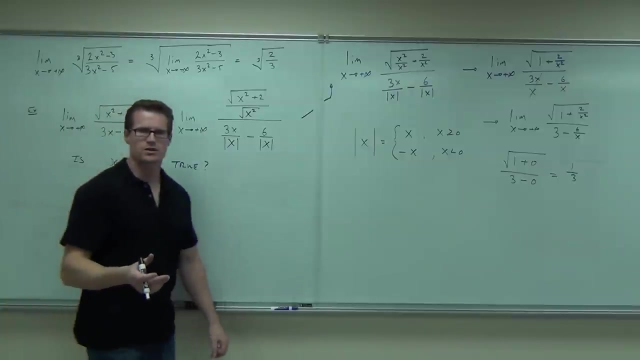 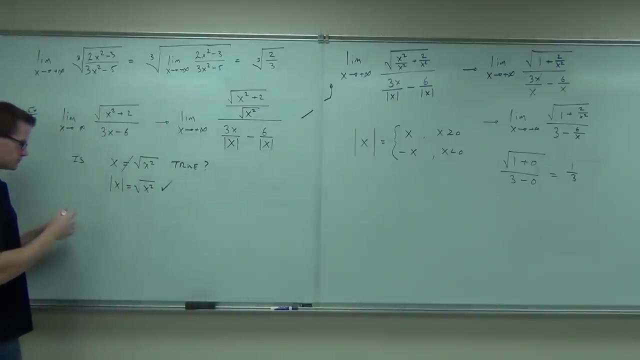 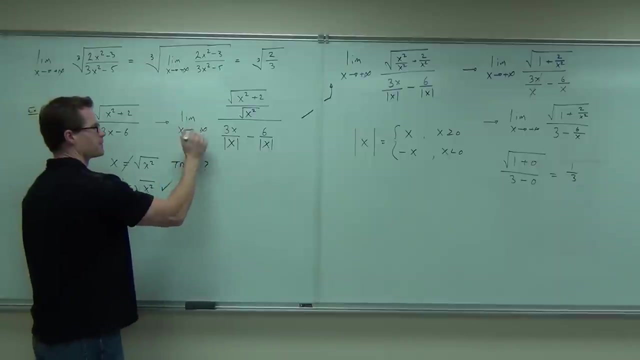 A number over huge is zero, One-third, Not the square root of one. 1 through Show of hands. how many people feel okay with that? Now I want you to consider this. Why this is important. Think about it. You can change your problem if you want to. I'm not going to do the whole example over again. I'm not going to give you two examples. I'm going to show you this. Let's say that that is now negative. That means that's negative. Is this still possible? 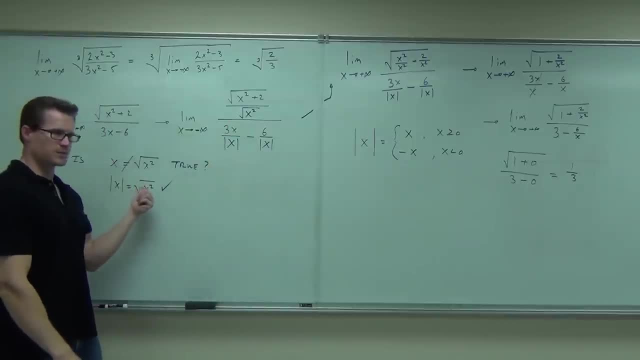 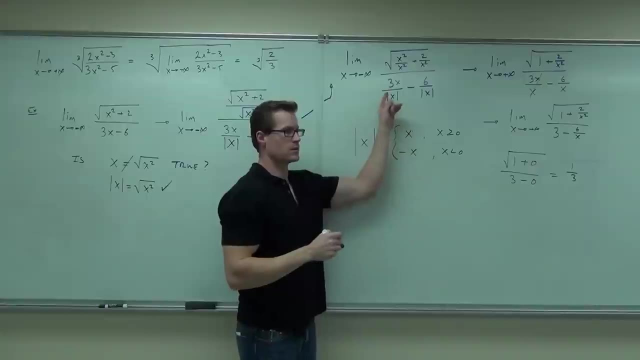 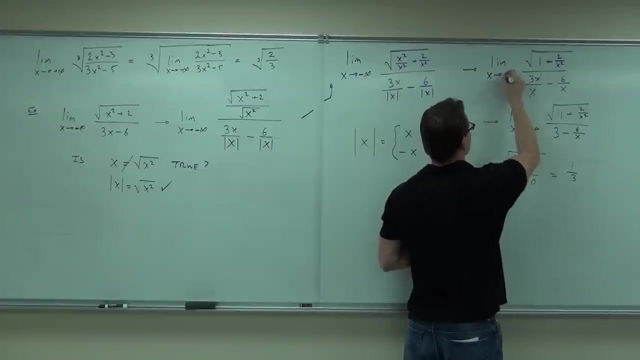 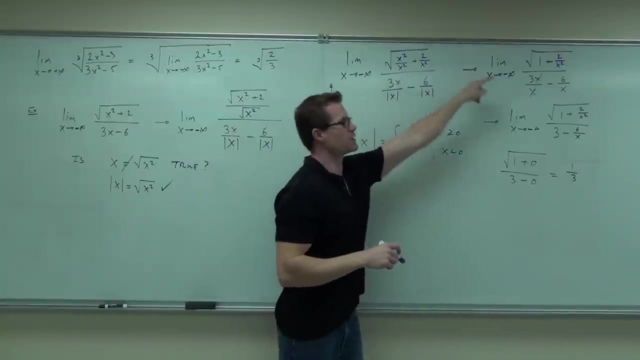 Absolutely, Is this still true? Absolutely, Is that still okay? Yes, Now, at this point, something different would happen At this point, from here to here. You see, if we're going to negative infinity, that means that for our absolute value of x. 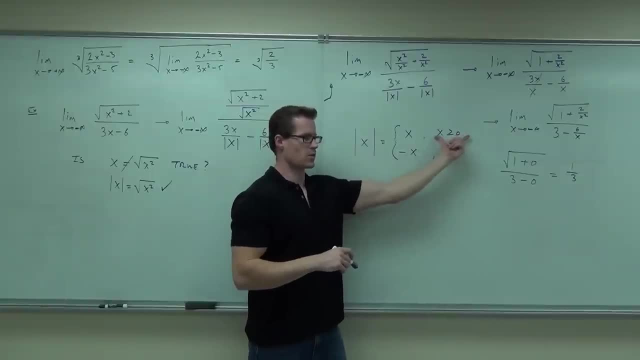 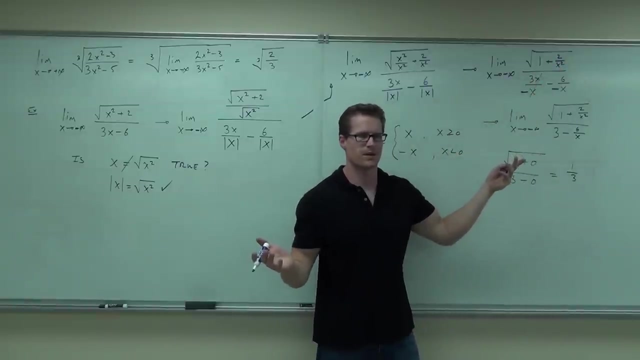 where are we going? We're not going here anymore. We're not dealing with positive numbers, We're dealing with negative numbers. That means, instead of absolute value of x equaling x, absolute value of x would equal negative x. That means that this and that would be there. Do you see the change? This would be okay. Square, right. Square is going to be positive, no matter what. That's where our definition came from. But this would be different. 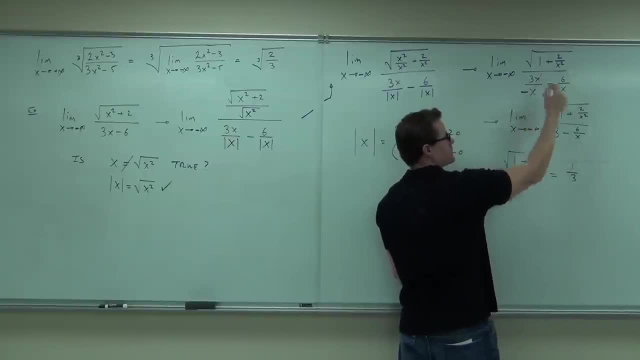 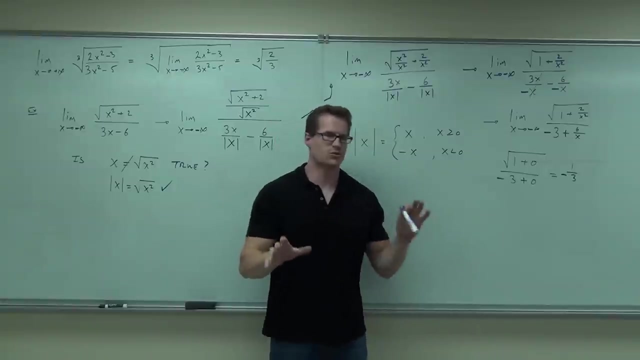 So what's negative? x Minus 6 over negative? Well, that's a plus. That's not really an effect. It's because that's being plus 0. But this definitely affects us, doesn't it? That's negative 3 plus 0. That's negative 1 third, not positive 1 third. What this says is- this is interesting, The first time we've had this, because if you've been thinking about it, you might have said: well, why do we even take positive infinity and negative infinity? Why don't we just do one infinity and consider it a horizontal asymptote the whole way? Well, it doesn't work. Look at that. 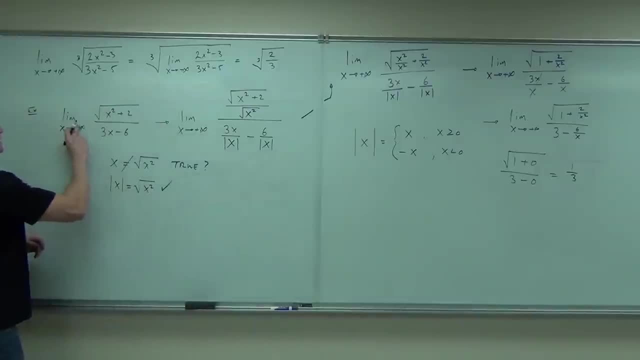 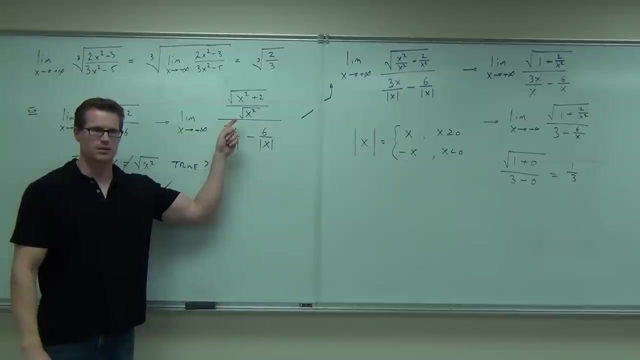 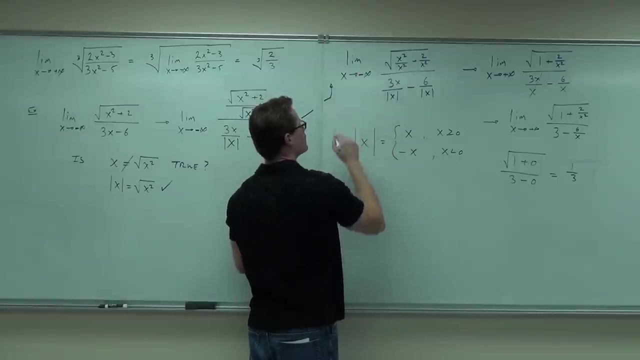 I'm not going to give you two examples. I'm going to show you with this. Let's say that that is now negative. That means that's negative. Is this still possible? Absolutely, Is this still true? Absolutely, Is that still okay? 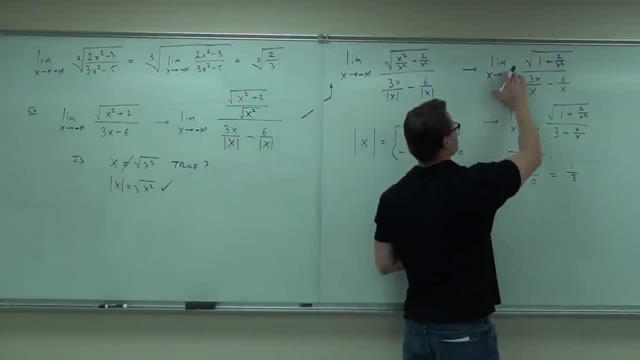 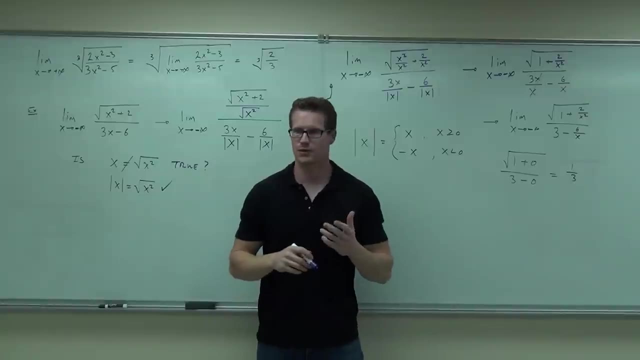 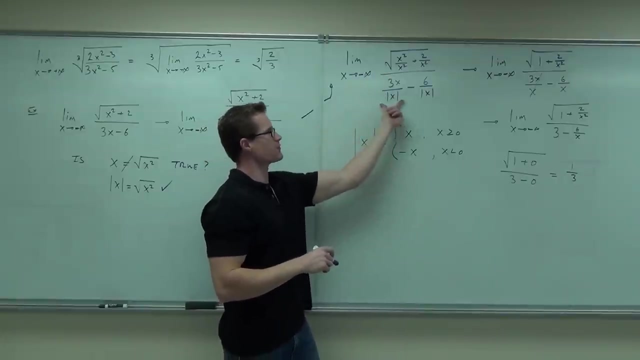 Yes, Now, At this point, something different would happen At this point, From here to here. You see, if we're going to negative infinity, that means that, for our absolute value of x, where are we going? We're not going here anymore. 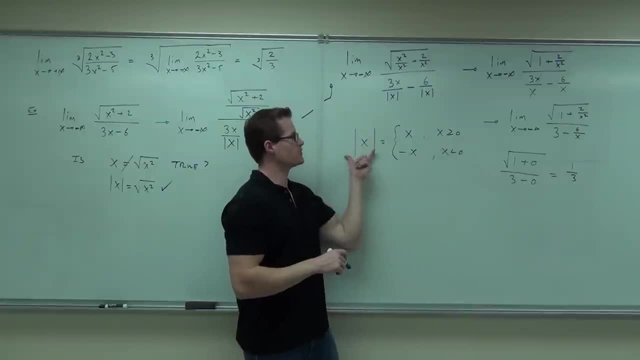 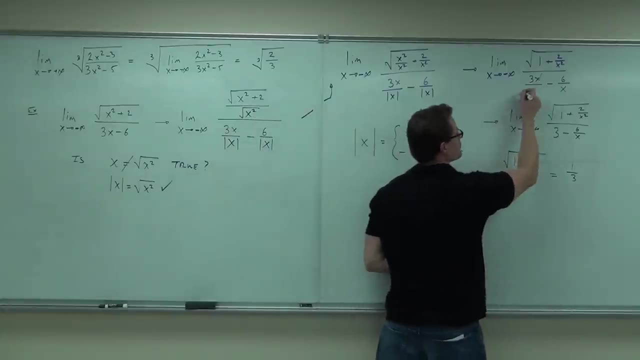 We're not dealing with positive numbers, We're dealing with negative numbers. That means, instead of absolute value of x equaling x, absolute value of x would equal negative x. That means that this and that would be there. Do you see the change? 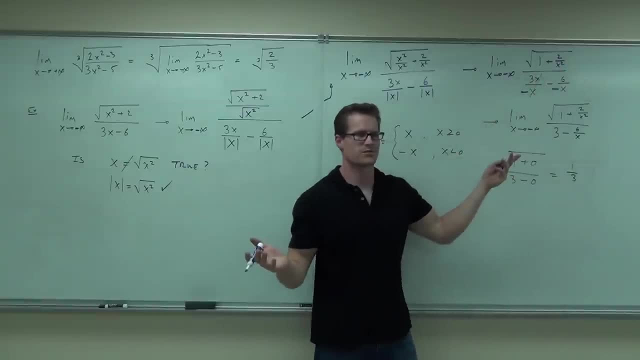 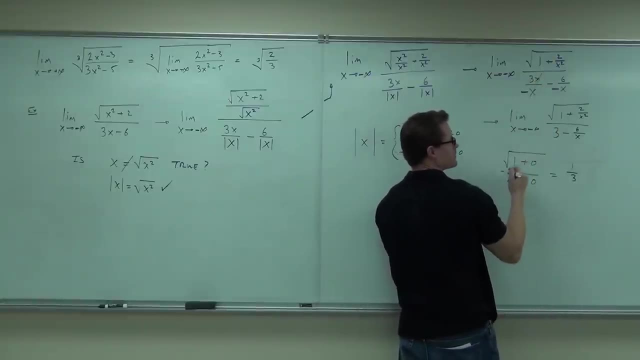 This would be okay. Square, right. Square's going to be positive, no matter what. That's where our definition came from, But this would be different. What's 3x over negative? x Minus 6 over negative? Well, that's a plus. 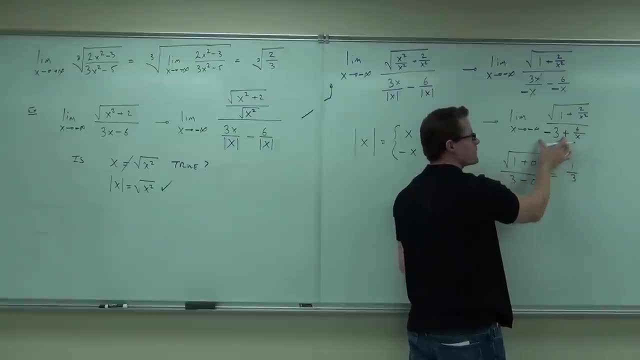 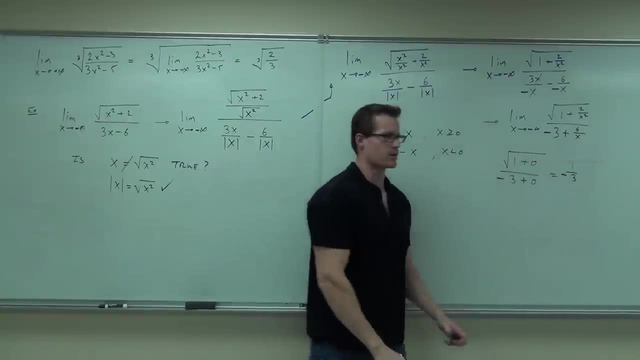 That's not really going to affect us because that's being plus 0. But this definitely affects us, doesn't it? That's negative 3 plus 0. That's negative 1 third, Not positive 1 third. What that says is: 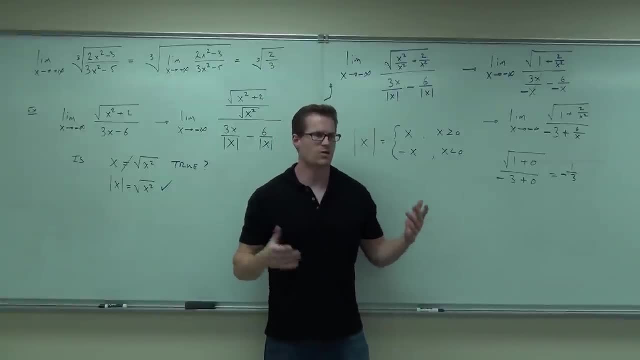 This is interesting. This is the first time we've had this, because if you've been thinking about it, you might have said: well, why do we even take positive infinity and negative infinity? Why don't we just do one infinity and consider it a horizontal asymptote the whole way? 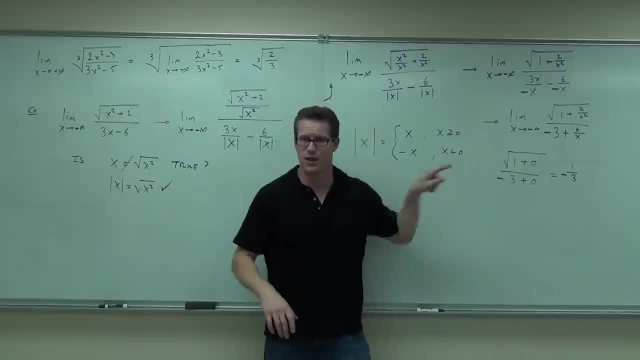 Well, it doesn't work. Look at that. Our first example was positive infinity, right, That's that way. That was at a horizontal. Remember what these are? A horizontal asymptote. That's a horizontal asymptote at 1 third. 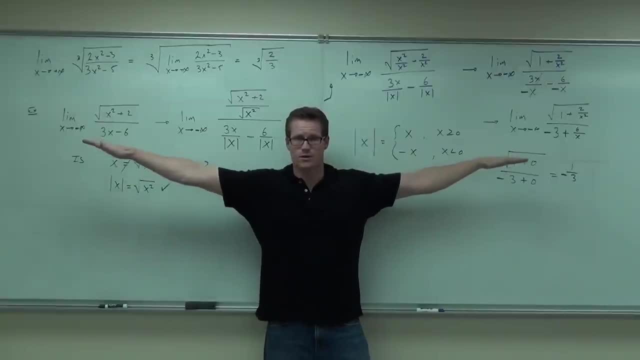 If you go to the left, negative infinity- is it at 1 third? No, it's at negative 1 third. So our horizontal asymptotes can be different as you go to positive infinity and negative infinity. That proves it. That's different, right there? 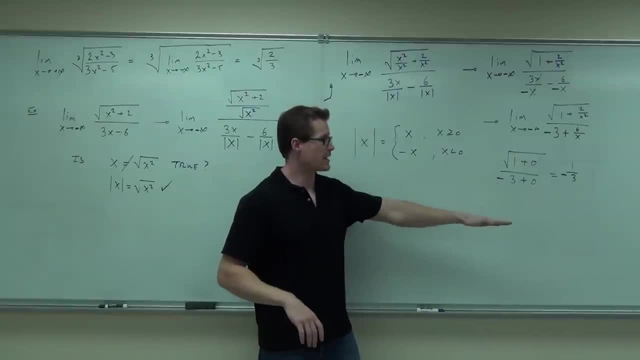 Our first example was positive infinity. right, That's that way. That was at a horizontal. Remember what these are? A horizontal asymptote, That's a horizontal asymptote at 1 third. If you go to the left, negative infinity- is it at 1 third? No, it's at negative 1 third. So our horizontal asymptotes can be different as you go to positive infinity and negative infinity. That proves it. That's different, right there. 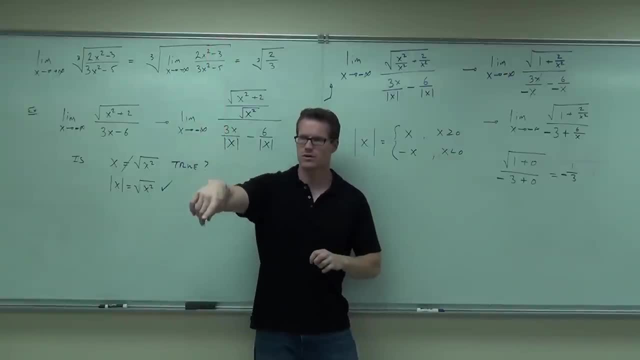 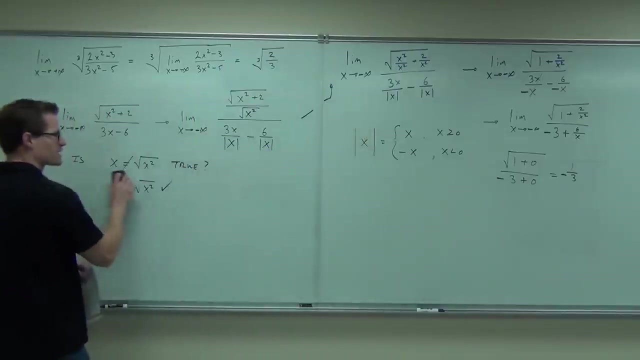 A lot of people understood that. Cool, This really is right with that. Hopefully that made sense to you. We're going to do one more example, maybe two, just to start it off. Let's try that. I'll show you something kind of cool, interesting, that you can do. 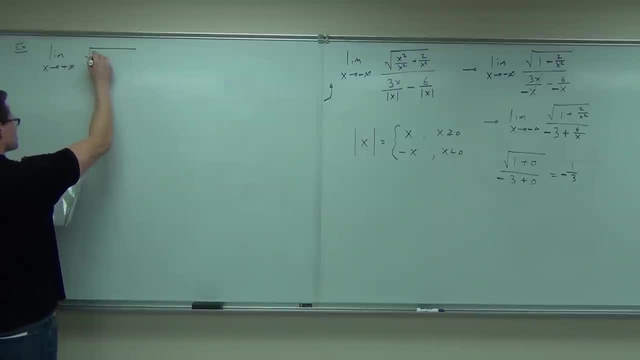 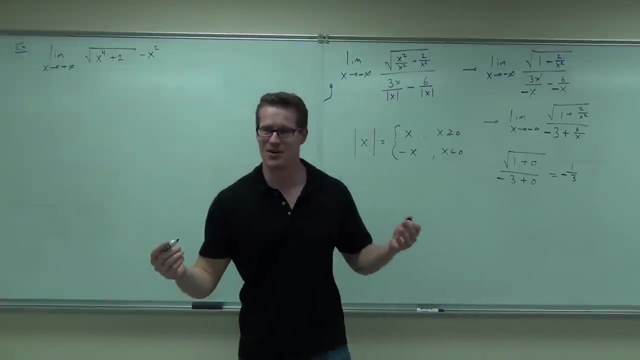 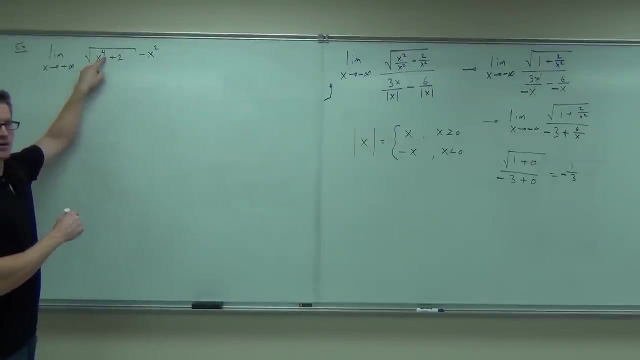 So we give it a try. Looks awesome to me. I don't know about you. Looks awesome to me, Let's try Ready. What's infinity to the fourth power? Infinity, Okay, cool, Plus 2?. And the square root of that. 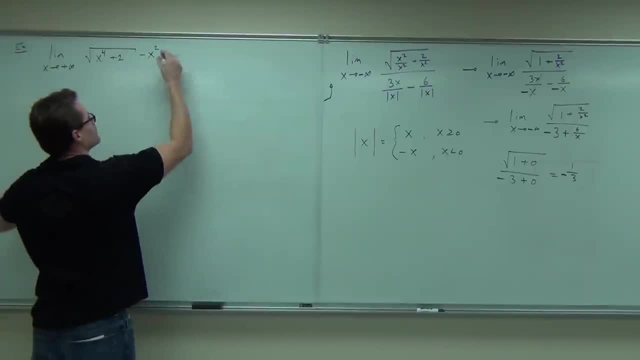 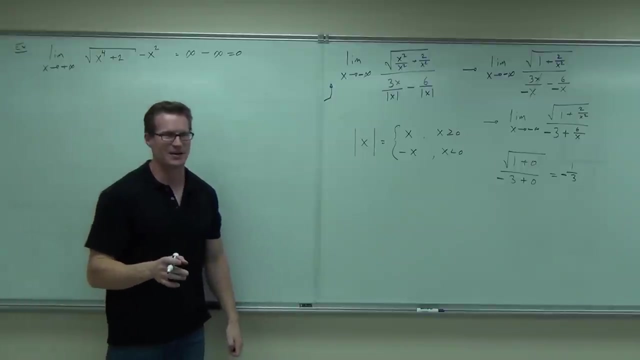 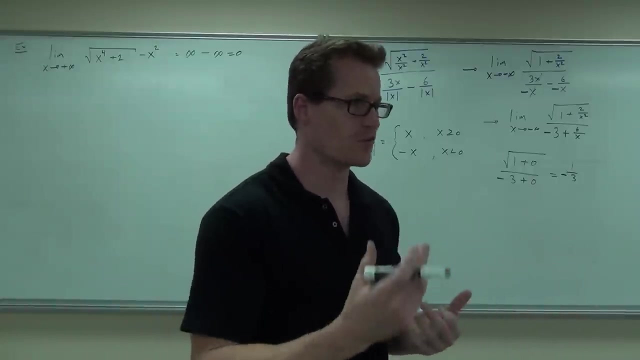 2. And then minus, so infinity. how much is infinity squared? Zero, All right, done. I love that. Easy problems, Yeah, No, Maybe coincidentally, but I really doubt it. We can't do that. You can't just plug in infinities Whenever you get a case where you're like infinity minus infinity or infinity over infinity, something like that. you know, something bad's happening. 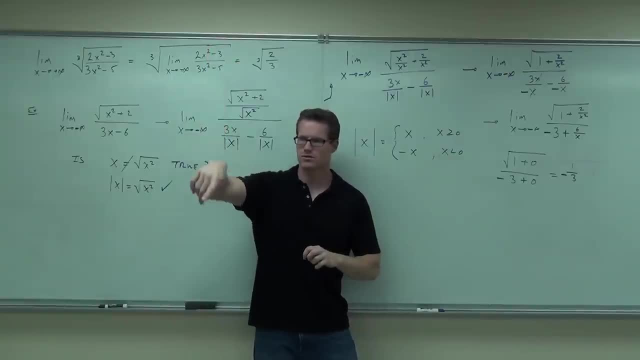 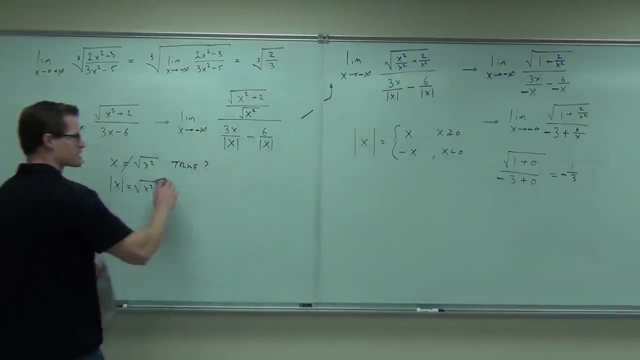 How many people understood that Cool? This really is a really good thing. Hopefully that made sense to you. We're going to do one more example, maybe two, just to start it off. Let's try that I'll show you something kind of cool. 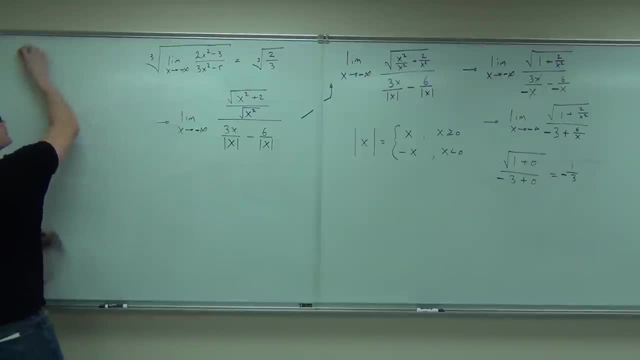 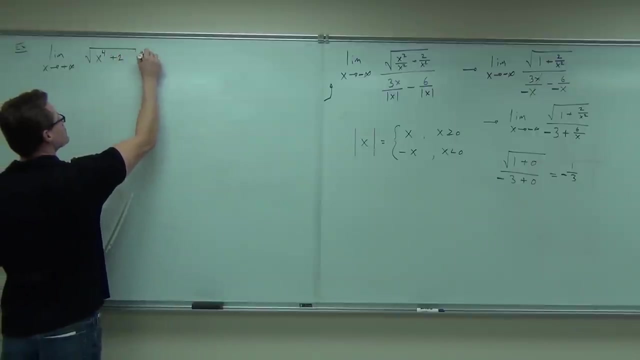 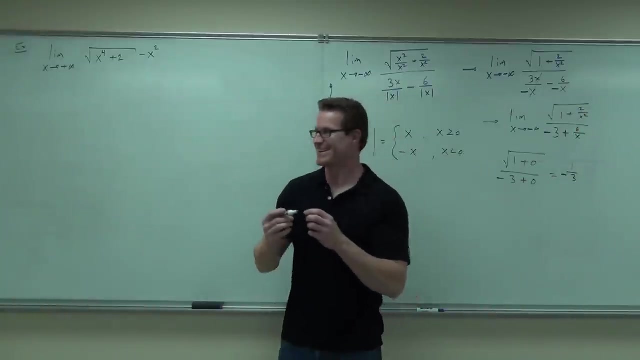 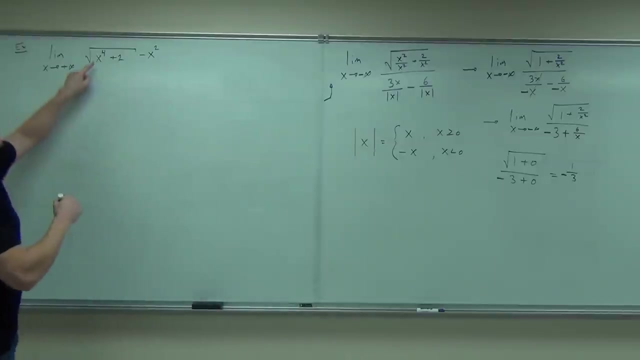 interesting that you can do, So we give it a try. It looks awesome to me. I don't know about you, It looks awesome to me. Let's try it Ready. What's infinity to the fourth power, Infinity, Infinity. 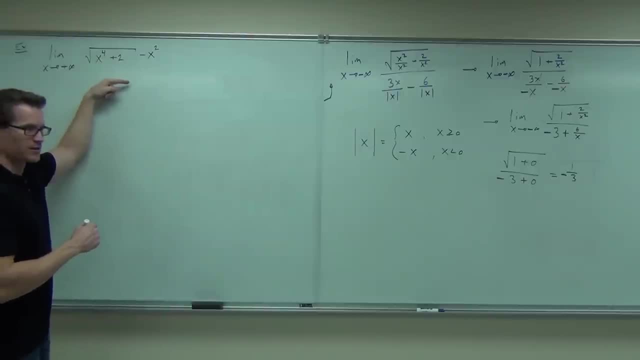 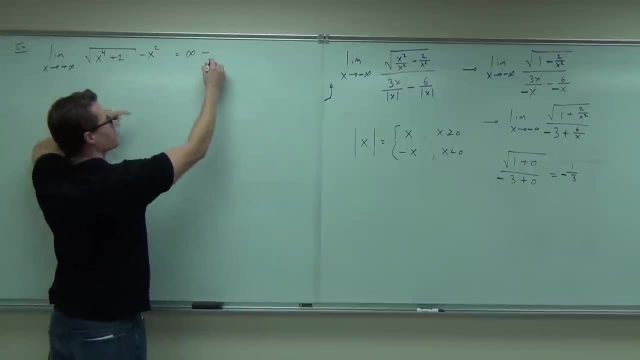 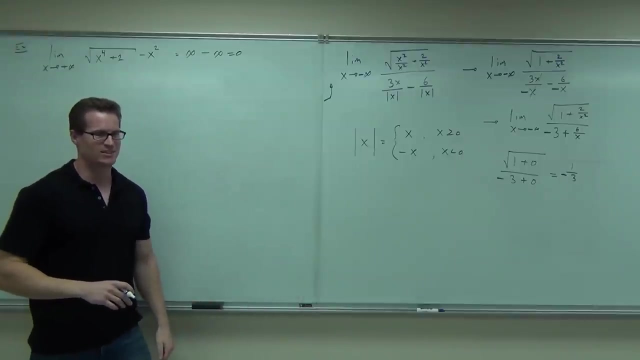 Okay, cool, Plus 2? Infinity And the square root of that, And then minus, So infinity. How much is infinity squared? Zero, Zero, All right done. I love that. Easy problems, Yeah, No, Maybe coincidentally, but I really doubt it. 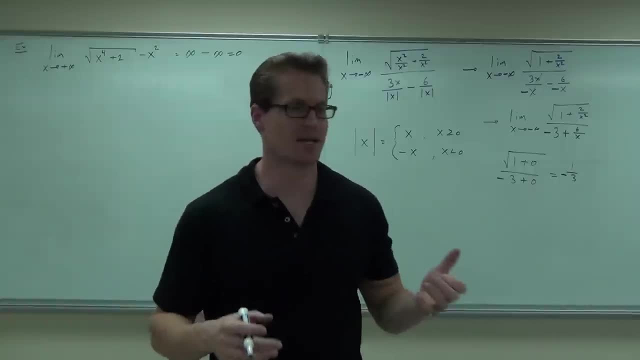 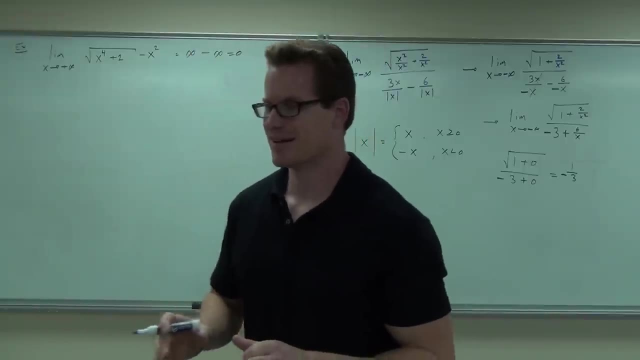 We can't do that. You can't just plug in infinities. Whenever you get a case where you're like infinity minus infinity or infinity over infinity, something like that, you know something bad's happening. all right, You're not doing something, right. 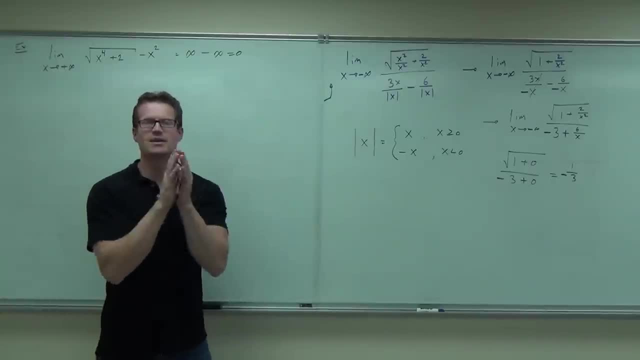 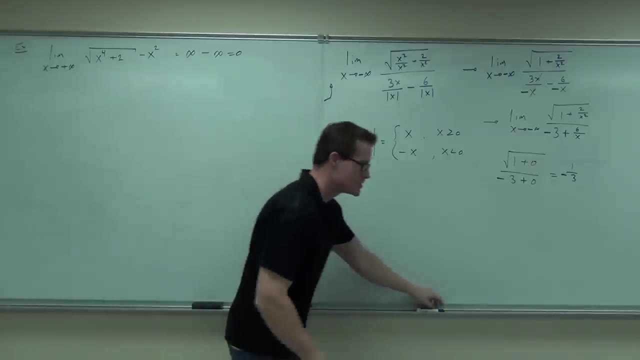 So you can't ever do that. If you get infinity over infinity, please, for heaven's sakes, don't put 1. Because that would have been 1, right? We can't do that. What we do have to do is manipulate the problem somehow. 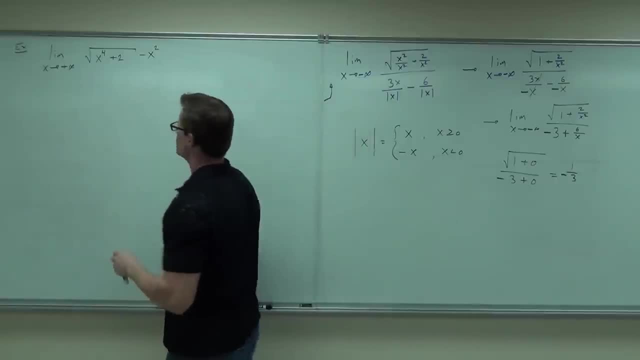 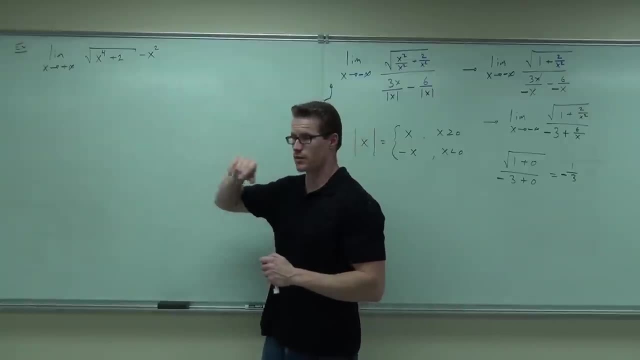 Now, in this case, you have a root. You have a root minus something. What's one thing we like to do with roots minus something when we can't work on them any other way. We usually try to rationalize something. all right. 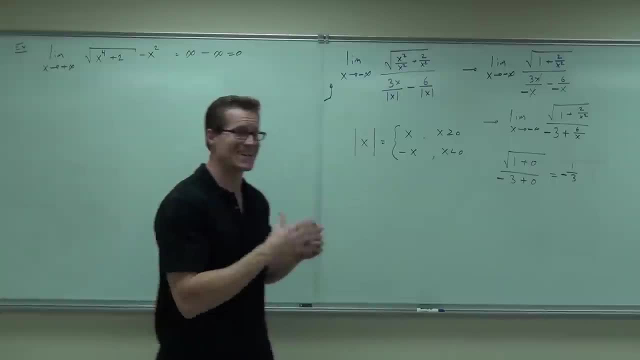 Yeah, you're not doing something right, So you can't ever do that. If you get infinity over infinity, please, for heaven's sakes, don't put 1,, because that would have been 1, right? We can't do that. 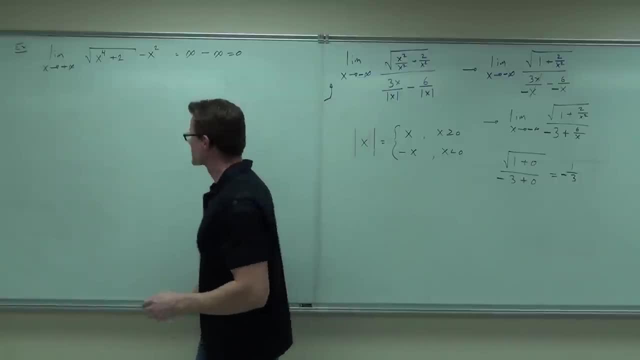 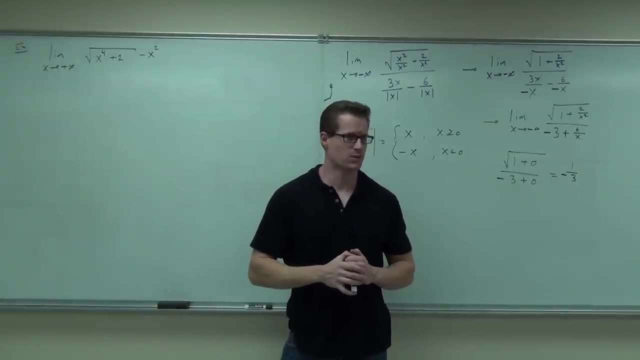 What we do have to do is manipulate the problem somehow. Now, in this case, you have a root. You have a root minus something. What's one thing we like to do with roots minus something when we can't work on them any other way? 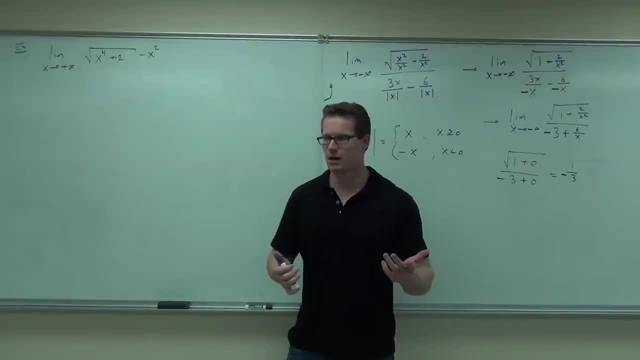 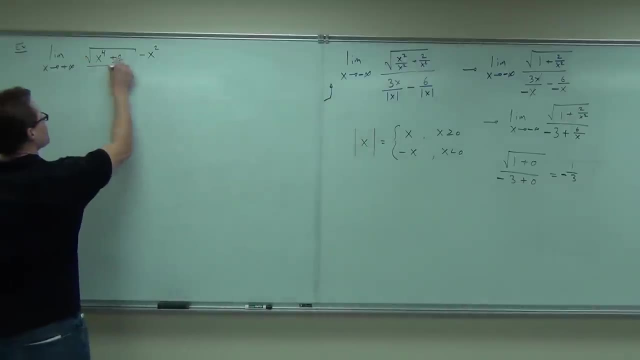 We usually try to rationalize somehow. right Now, this doesn't have a denominator, so make one: Put it over what? 1. Put it over 1. Get yourself a denominator, Then you're going to try to rationalize. 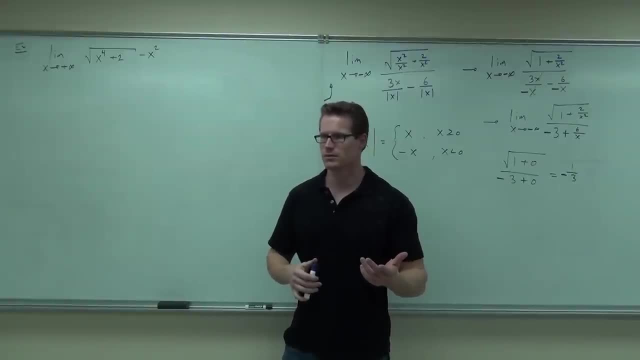 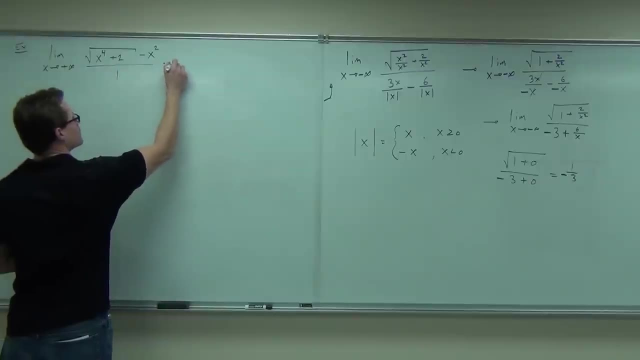 Now, this doesn't have a denominator. so make: 1. Put it over what, Put it over what, Get yourself a denominator. Then you're going to try to rationalize: Conjugate, Conjugate, Very good, Conjugate. 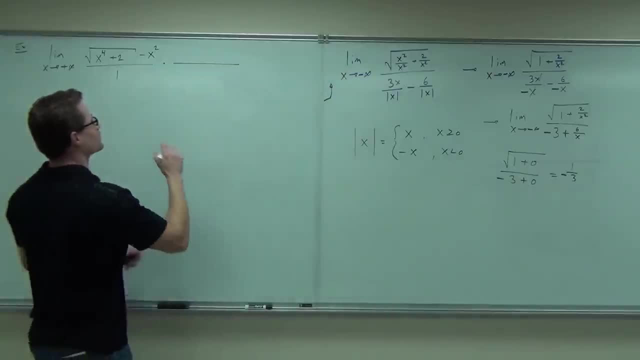 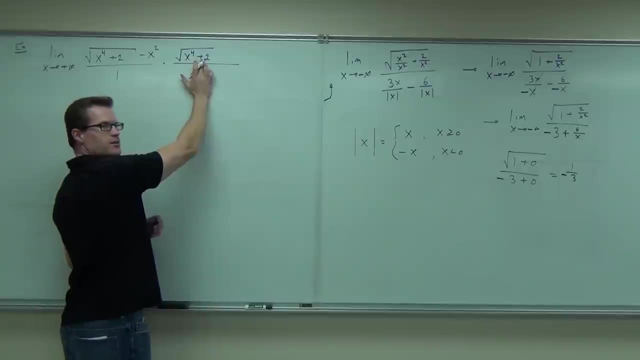 Conjugate, Conjugate. Very good, Conjugate. You don't want to be fancy about it. Is it plus 2 or minus 2 there, by the way, Plus 2.. Good, So this sign doesn't change. This sign does change And it's over exactly the same thing. 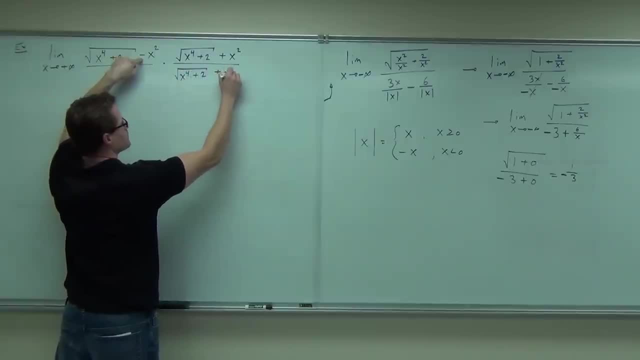 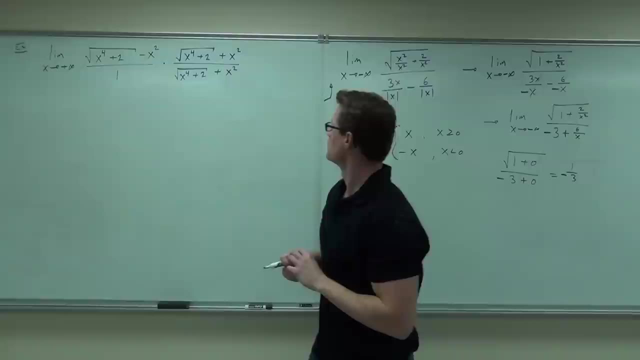 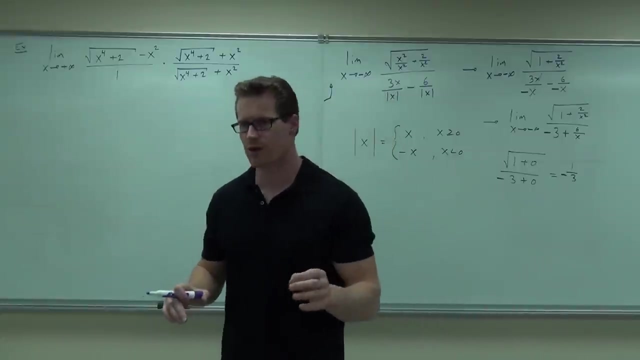 Are you okay with that so far, Yes or no? Well, the denominator has nothing to distribute, which is really nice. We don't have to do any work up there. The numerator just distribute it carefully. You know, with conjugates, your middle term should be bye-bye. 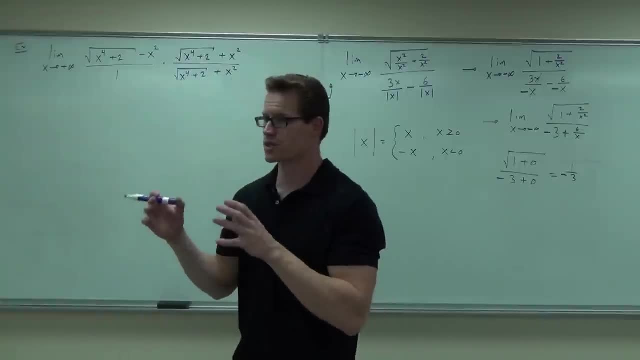 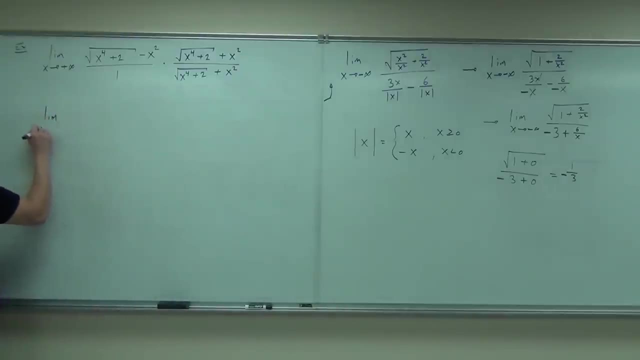 right, your middle term should be gone. We know also that conjugate works this way because you have a square root. times a square root gives you the radicand that's inside. That's nice. So our limit to positive infinity becomes something over the square root of x to the fourth, plus 2 plus x squared. 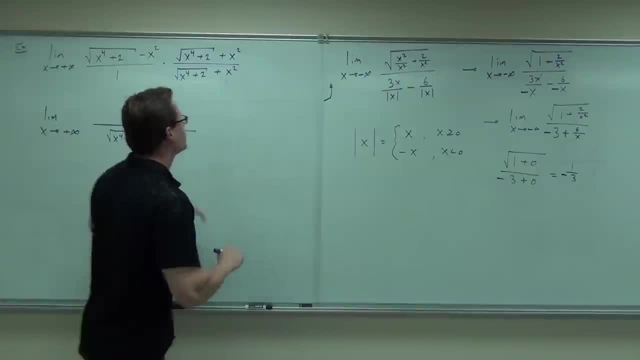 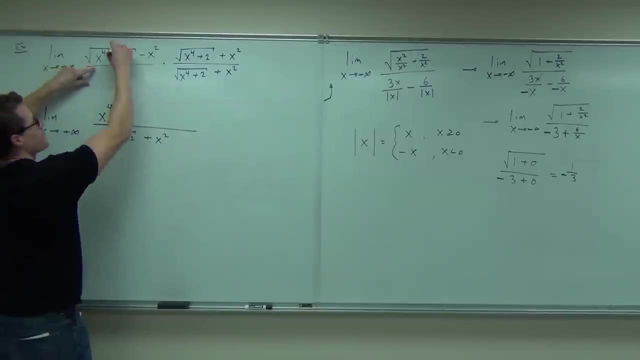 The numerator becomes: oh, what's the numerator become Minus x to the fourth. Distribute right. Do you see that On your distribution? Yeah, Do you see that distribution? because you should have those X to the fourth plus 2.. 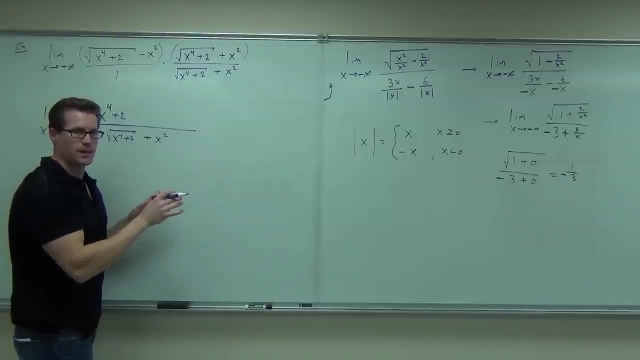 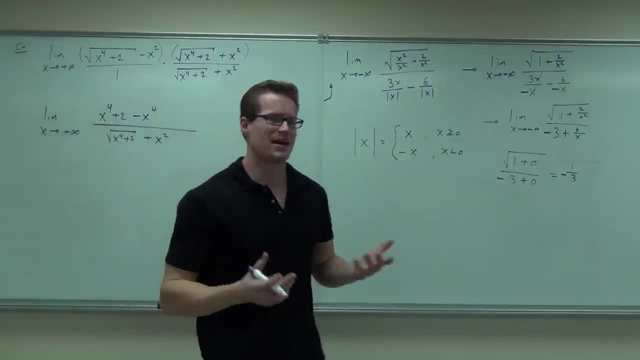 We're going to have plus and minus the same exact thing, and then we're going to get what's the last thing? You see, the minus x to the fourth too. Don't forget about the exponent. If you make the exponent incorrect, it's not going to come out right. 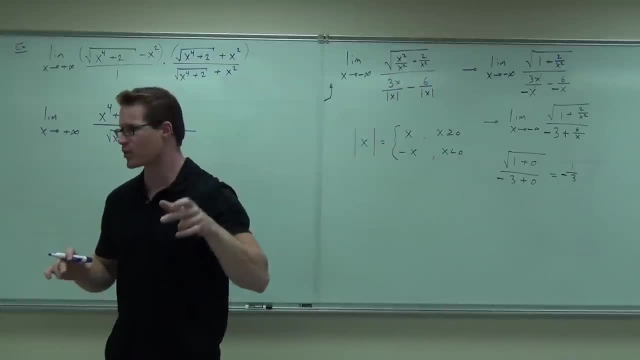 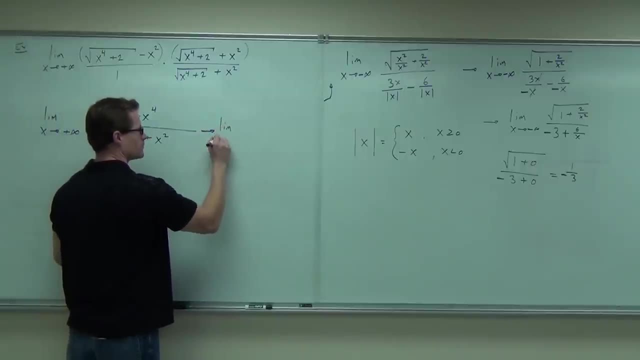 So you got to really be careful about your distribution. Don't forget to distribute that last part. You got me What happens here. that's nice, I think. I think that's what you're looking for. Yeah, oh, that's great. 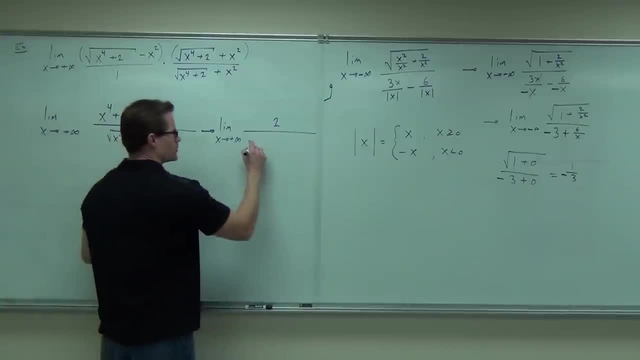 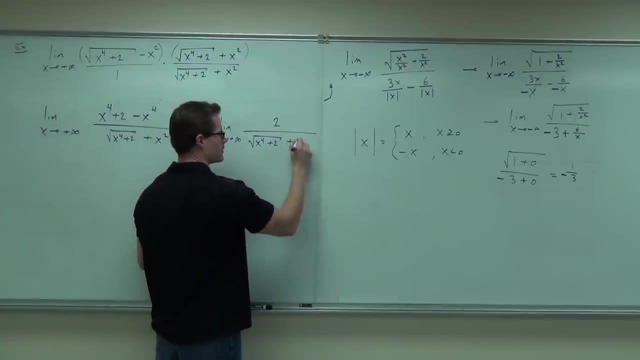 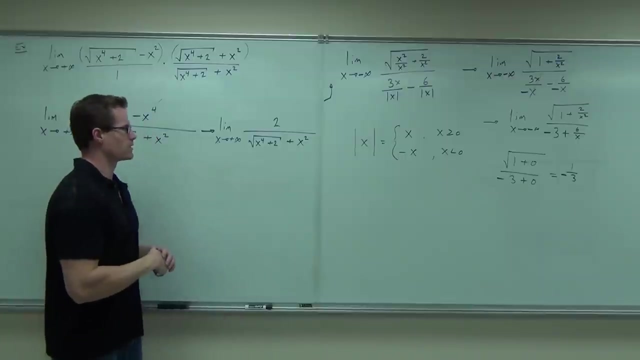 I love that. Two Square root of x to the fourth plus 2 plus x squared. So far, so good. Mm-hmm, Okay, Looks to me like it's going to zero. Can we do that legally? Can we just say 2 over? well, I don't know. 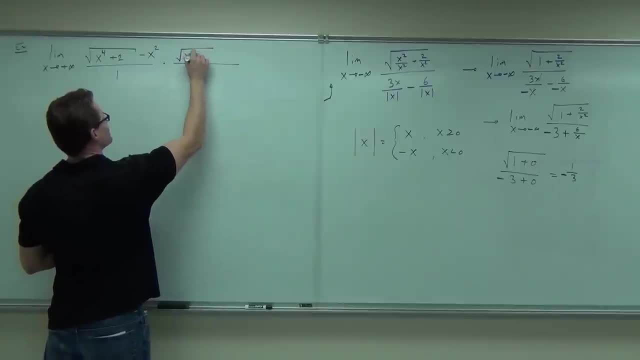 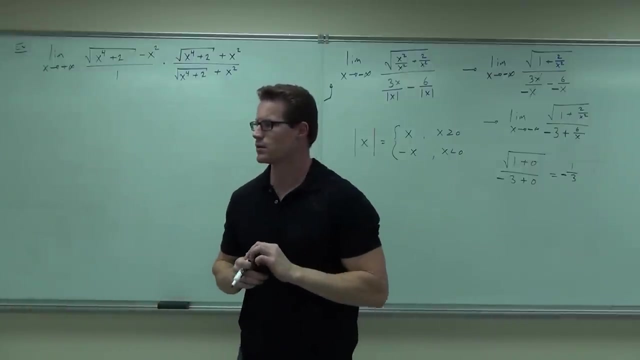 Let's see about it. Is it plus 2 or minus 2 there, by the way, Plus 2.. Good, So this sign doesn't change. This sign does change And it's over exactly the same thing. Are you OK with that? so far? 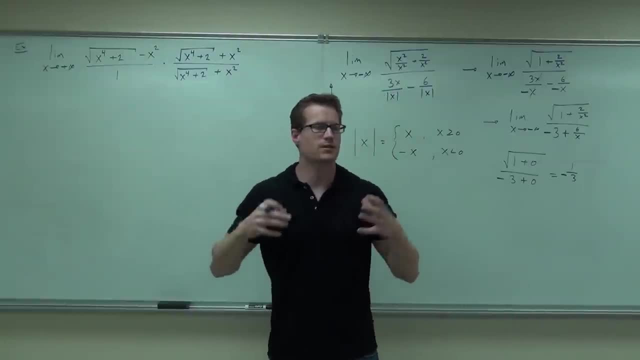 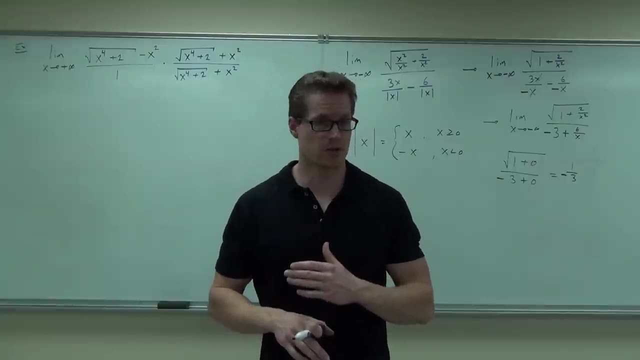 Yes or no. Well, The numerator has nothing to distribute, which is really nice. We don't have to do any work up there. The numerator just distribute it carefully. You know, with conjugates, your middle term should be bye-bye, right. 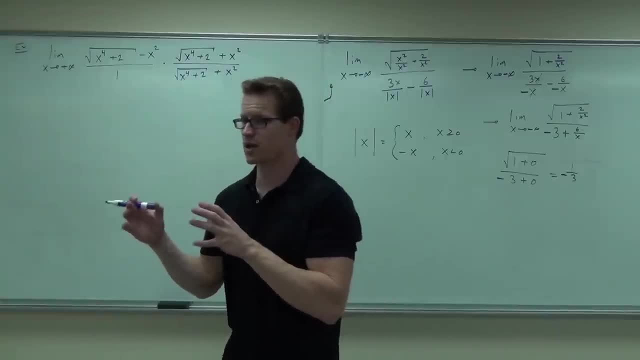 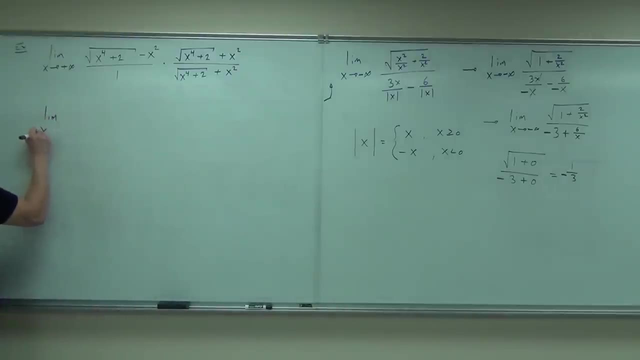 Your middle term should be gone. We know also that conjugate works this way because you have a square root. times a square root gives you the radicand that's inside. That's nice. So our limit to positive infinity becomes something over the square root of x to the fourth plus 2. 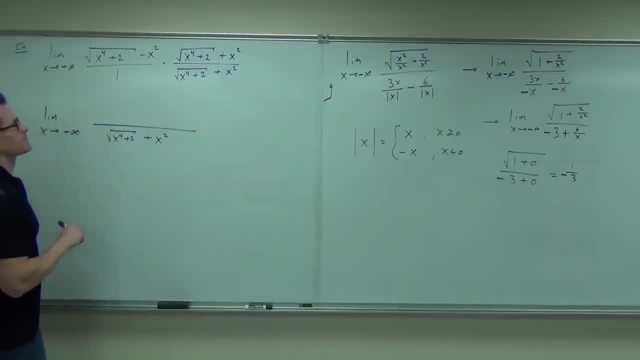 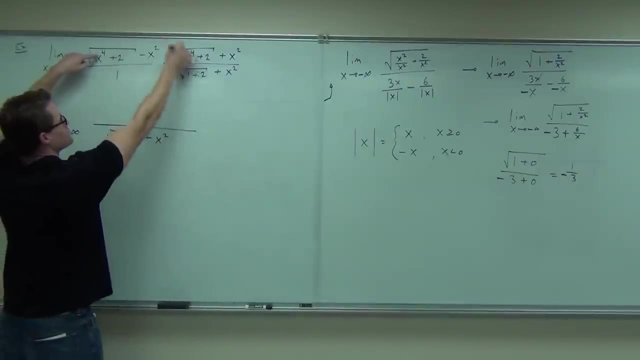 plus x squared, The numerator becomes: Oh, what's the numerator become Distribute, right? Do you see that on your distribution? because you should have those x to the fourth plus 2.. We're going to have plus and minus. 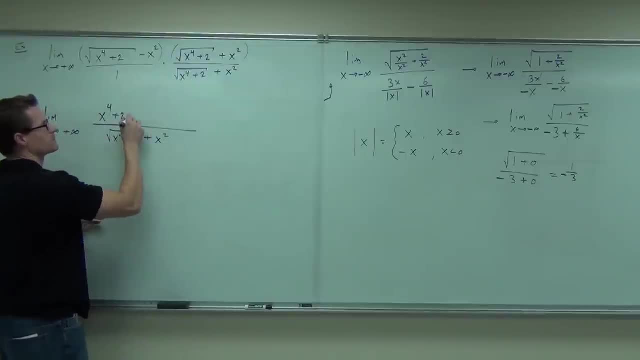 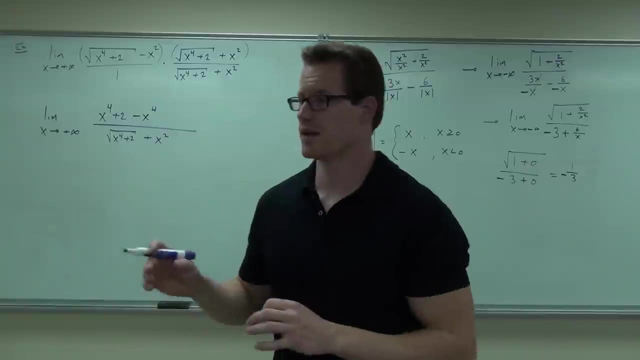 the same exact thing, And then we're going to get What's the last thing? You see? the minus x to the fourth 2?? Don't forget about the exponent. If you make the exponent incorrect, if you make the exponent incorrect. 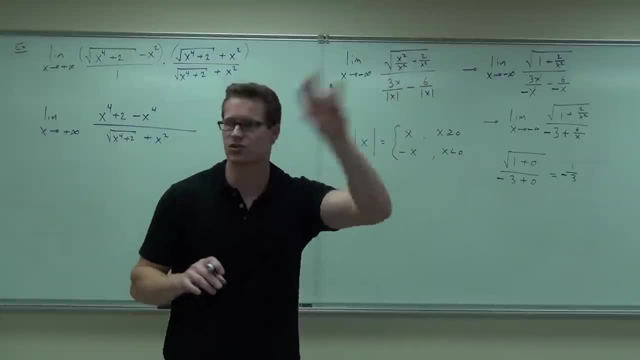 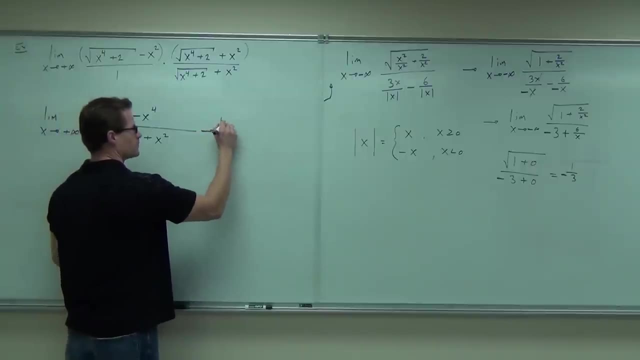 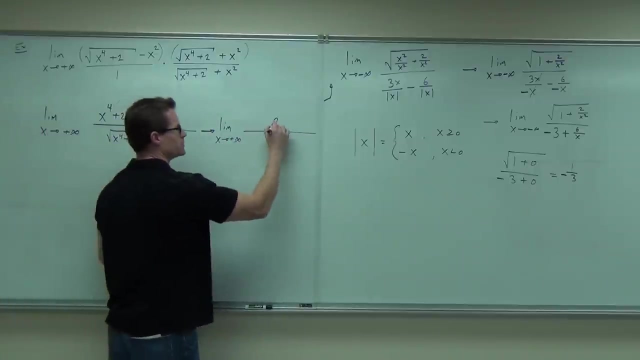 it's not going to come out right. So you really need to be careful about your distribution. Don't forget to distribute that last part. You got me What happens here. that's nice. Yeah, Oh, that's great, I love that. 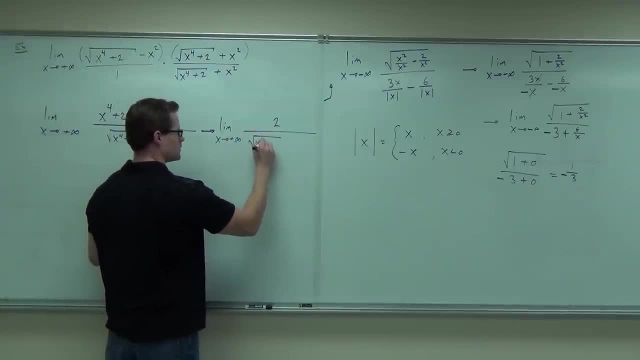 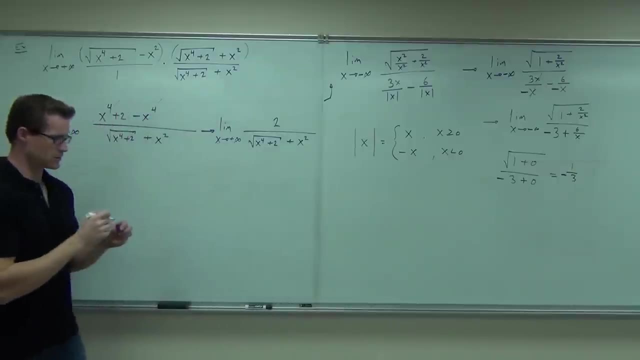 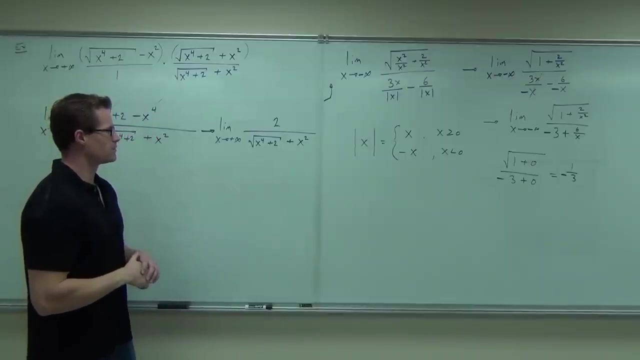 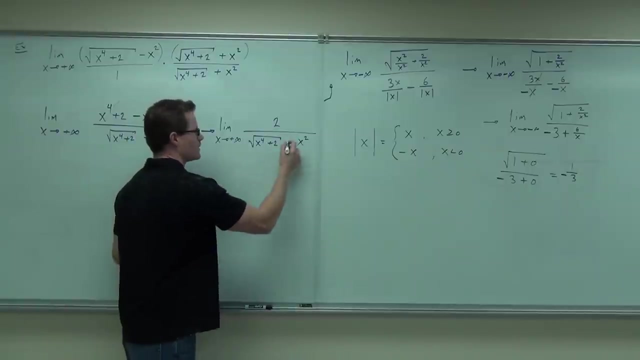 2 square root of x to the fourth plus 2 plus x squared. So far, so good. Okay, Can we do that legally? Can we just say 2 over? Well, I don't know, Especially if this is a, Especially if you did this. 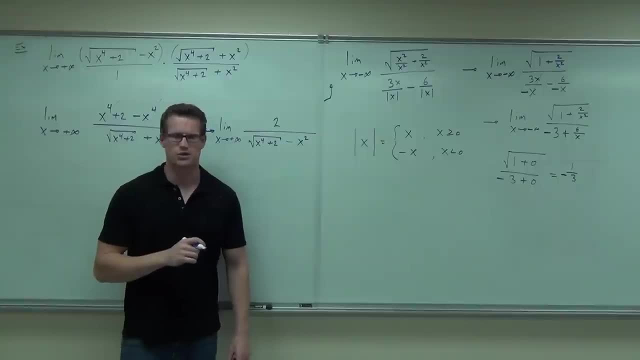 Especially if you did that, that would be a big problem. Can you do that? That would be an issue. So what we're going to do is make sure about it. You're going to start dividing by the largest power in the denominator. 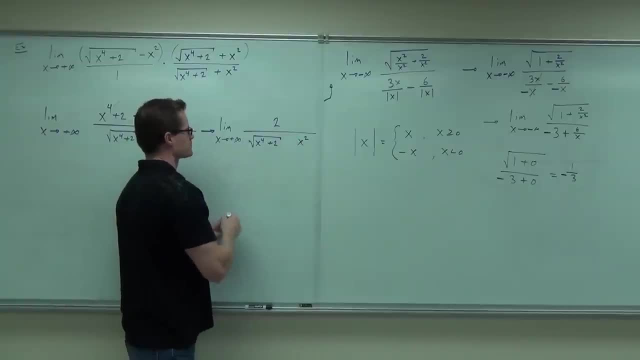 Especially if this is a especially if you did this, Especially if you did that, that would be a big problem. Do you see that? That would be an issue. So what we're going to do is make sure about it. You're going to start dividing by the largest power. 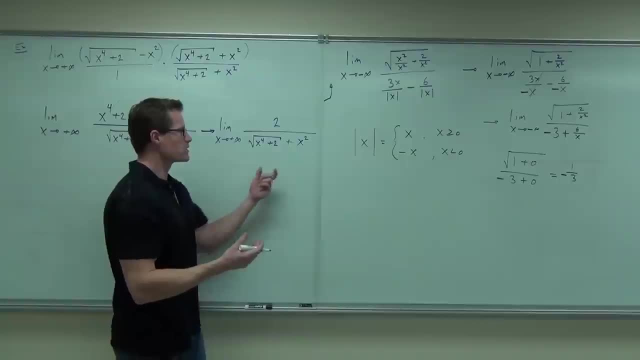 in the denominator again, just like you normally would. So what's the largest power in the, especially if I give you this one? okay, What if that was 2x? That would be a big problem. This one, yeah, Scott's right. 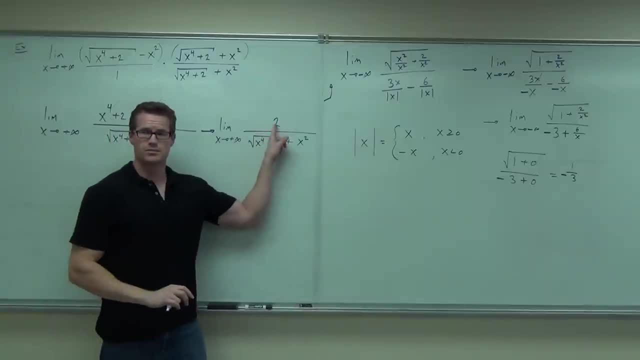 You probably could look at this and go: that's 2.. That's infinity plus that's infinity. There's no way that that's not going to be infinity. You got me This is going to go to zero. He's right. 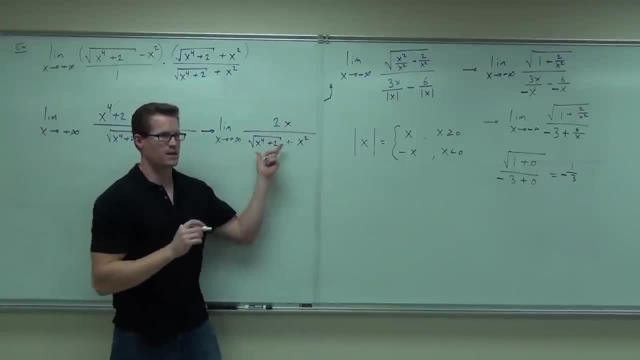 But to check your work, especially if you have something like this that might not go to infinity, That definitely wouldn't go to infinity- Okay, That wouldn't. So to check your work to show that what you're going to do is go all right. 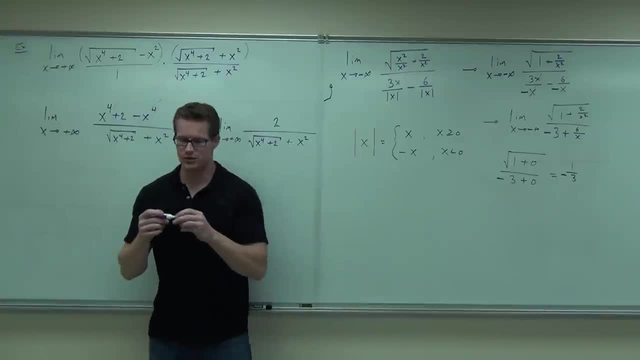 well, let's divide everything by the largest power in the denominator. Now, don't trick yourself here. The largest power in the denominator is 1.. The largest power in the denominator is not x to the 4th, It's not x to the 4th. 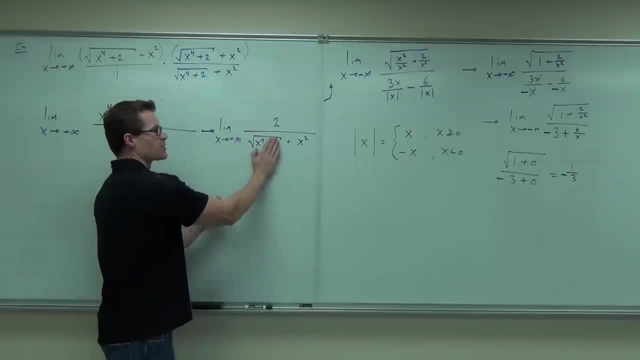 What is it? Yeah, the way you can think about it. Cover up the rest of it. Look at the largest term. What's the square root of x to the 4th? It's x squared. That's your largest power. 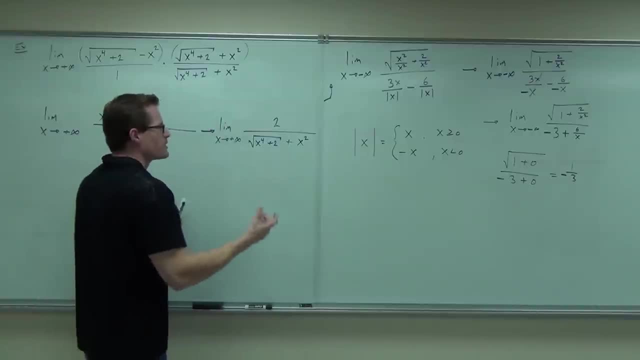 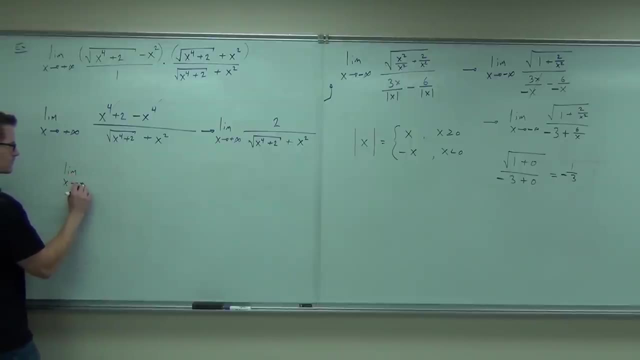 It's the square root of that, Because it's inside a square root, So divide everything by that. Now I'm making you do this because I want you to see one more time this setup. Notice: we're dividing by x squared. If I divide this by x squared, is that going to work here? 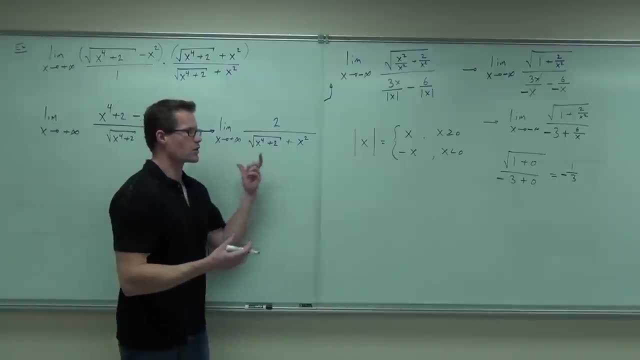 Again, just like you normally would. So what's the largest power in the, Especially if I give you this one? okay, What if that was 2x? That would be a big problem. This one, yeah, Scott's right. 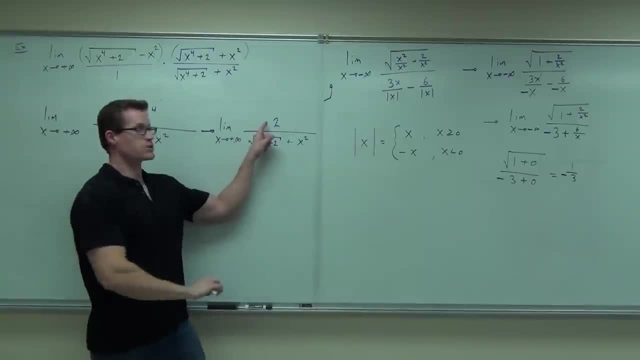 You probably could look at this and go: that's 2.. That's infinity plus That's infinity. There's no way that that's not going to be infinity. You got me This is going to go to 0.. He's right. 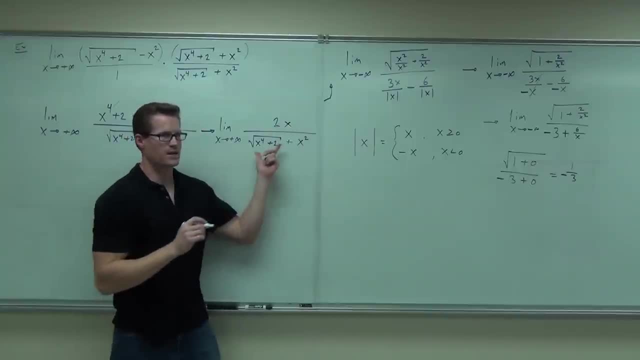 But to check your work, especially if you have something like this that might not go to infinity, That definitely wouldn't go to infinity, Okay, That wouldn't. So to check your work, to show that what you're going to do is go. 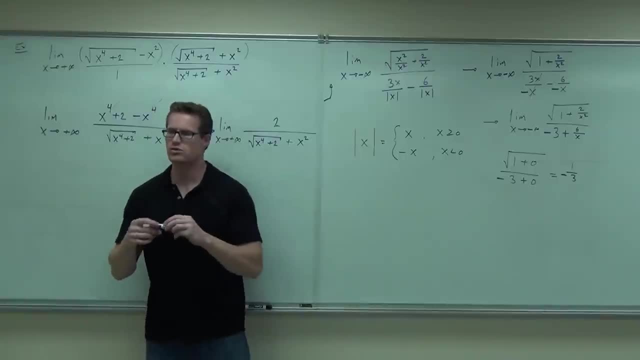 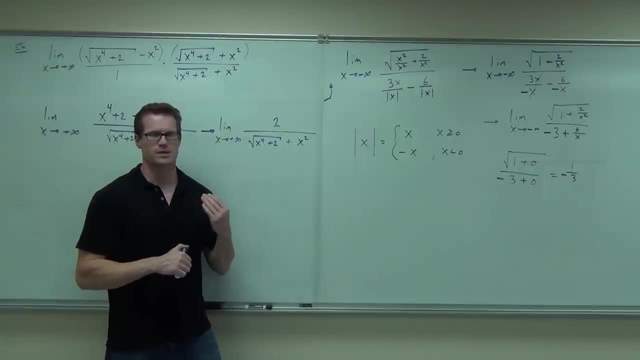 all right. well, let's divide everything by the largest power in the denominator. Now, don't trick yourself here. The largest power in the denominator is not x to the fourth. It's not x to the fourth. What is it? The square root of x to the fourth? 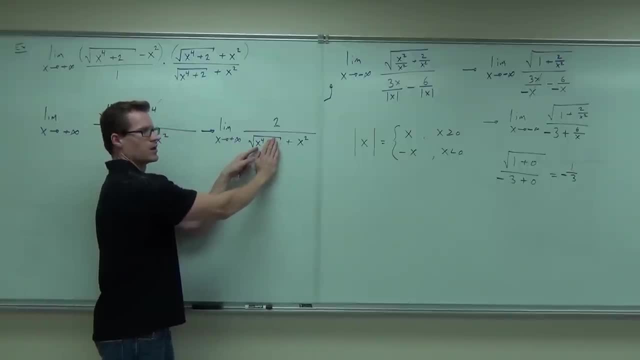 Yeah, the way you can think about it. Cover up the rest of it. Look at the largest term. What's the square root of x to the fourth? It's x squared. That's your largest power. It's the square root of that. 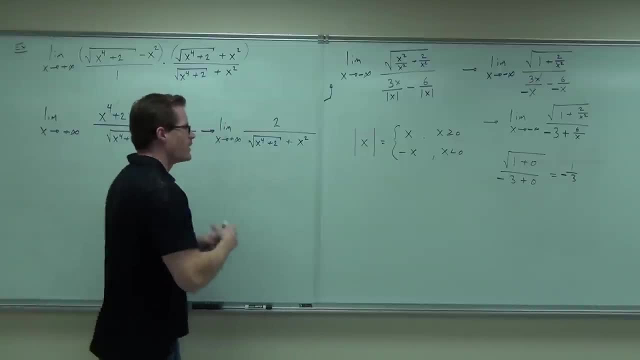 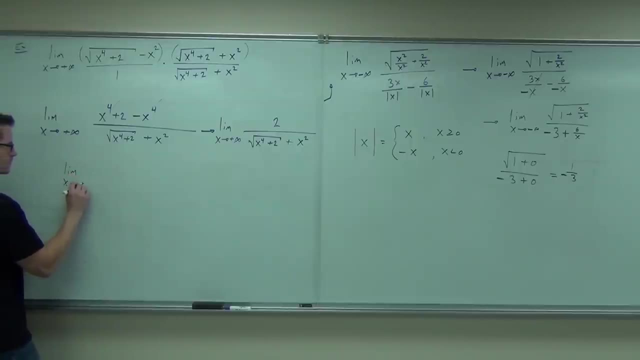 It's inside the square root, So divide everything by that. Now I'm making you do this because I want you to see one more time this setup: Notice we're dividing by x to the fourth. Notice we're dividing by x, squared. 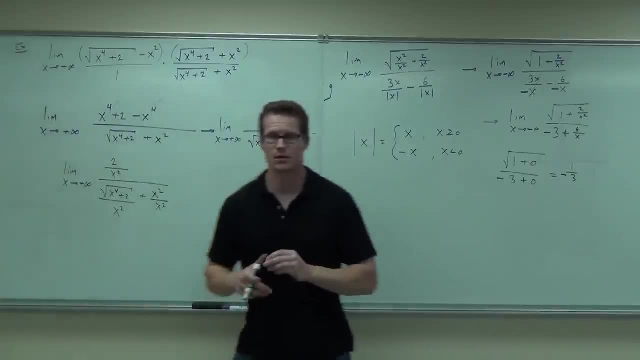 If I divide this by x, squared, is that going to work here? Is this okay? No, Can I take that inside of that square root? Okay, so think back to what we did. This is fine, right? This is fine. that's great. that's what we like. 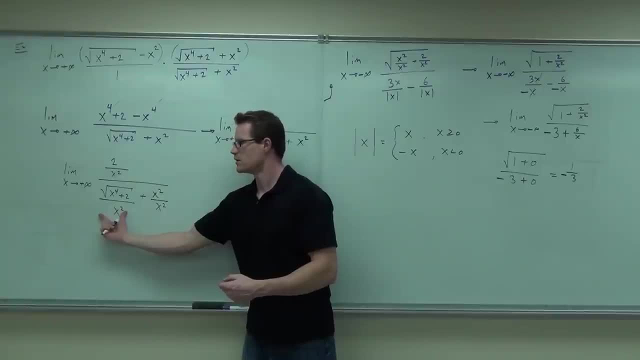 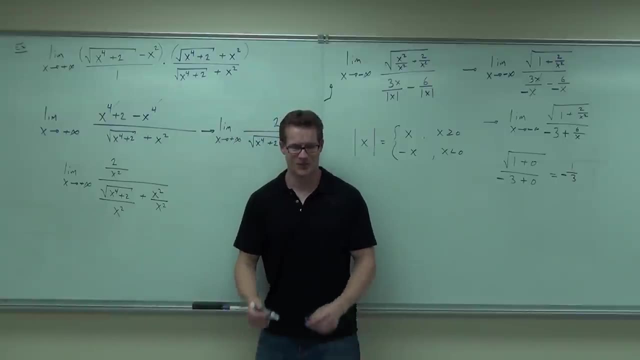 What does this do? What now? Uh oh, okay, did we get stuttered? Uh oh, Square root of x to the fourth. Square root of x to the fourth would be great. Did you see that already? Yeah, I was thinking. my mind was wandering. 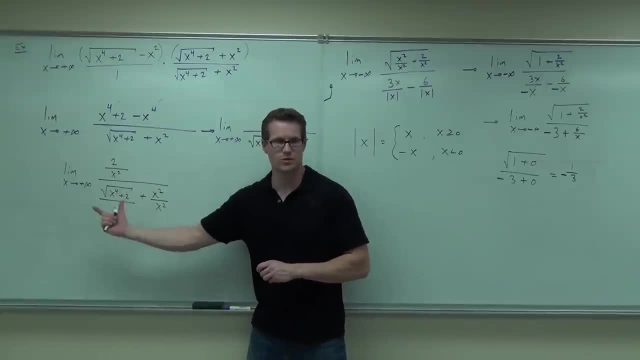 Is this okay? No, Can I take that inside of that square root? Okay, so think back to what we did. This is fine, right? This is fine, That's great, This is what we like. What does this do? 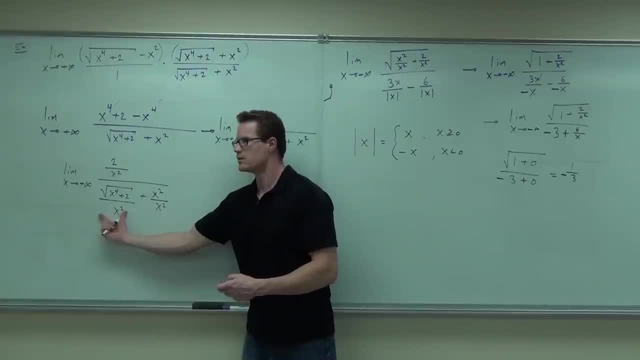 Square root of x squared over y. What now? Oh, oh, okay, We got stuck. Square root of x to the 4th. Square root of x to the 4th would be great. Did you say that already? Yeah? 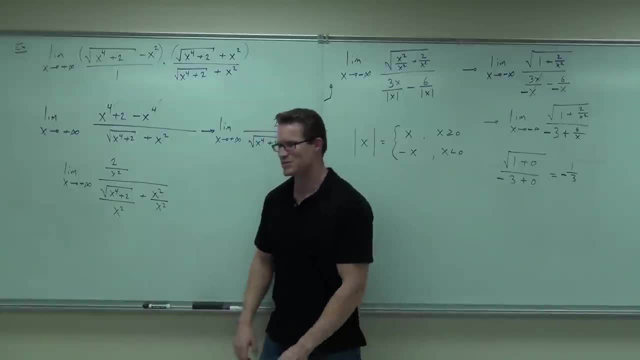 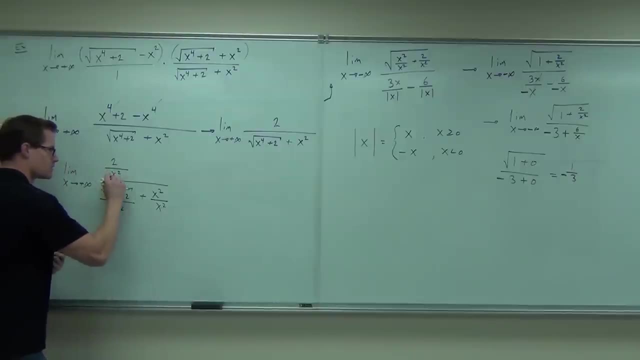 I was thinking, My mind was wandering. I was thinking about the Simpsons. So well, since this is x squared and this is x squared, we need to make this equal to x squared, but it also has to have a square root around it. 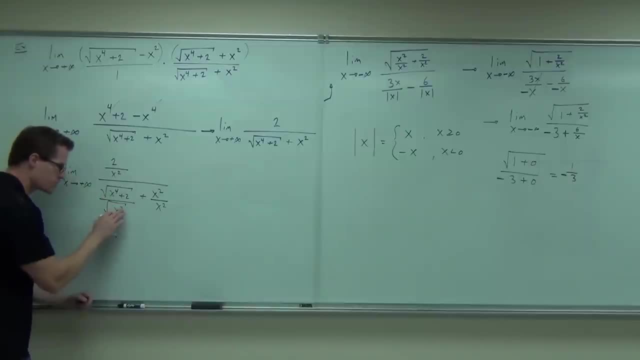 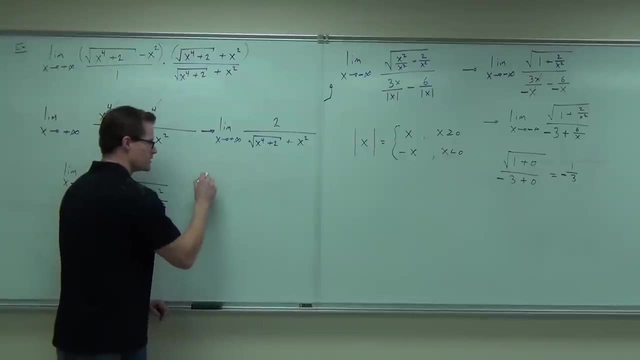 You follow. You can't just do this because that's x, so change the power. Is that true? Now some of you are going to ask me: well, wait a second, Mr Leonard, Don't you have to have some absolute value here? 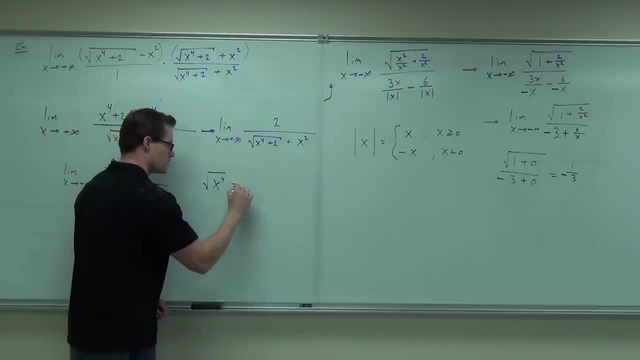 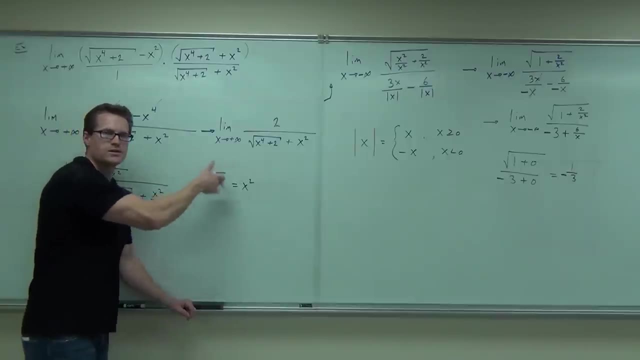 Let me ask you this question: Is this always true? That actually is always true. no matter what, No absolute value needed because you have all positive, all positive, It's always going to be the same. Does that make sense? So we don't even need that for this case. 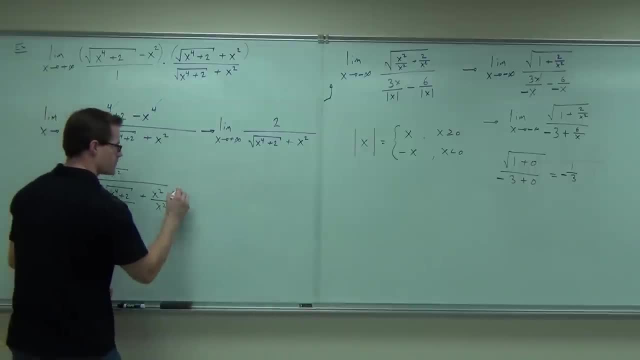 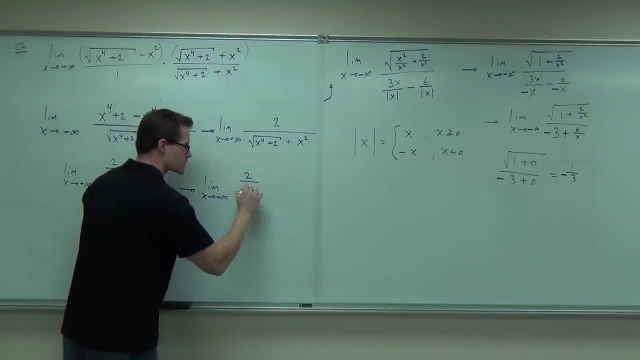 So here we're going to have- I just wanted you to see that one time- Two over x squared all over. We're going to have the square root. If you think about it, this is going to be 1 plus 2 over x to the 4th. 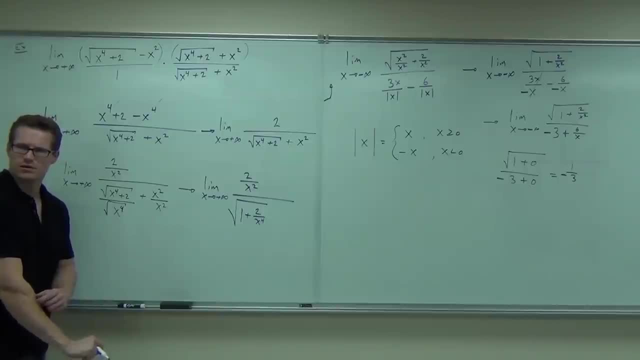 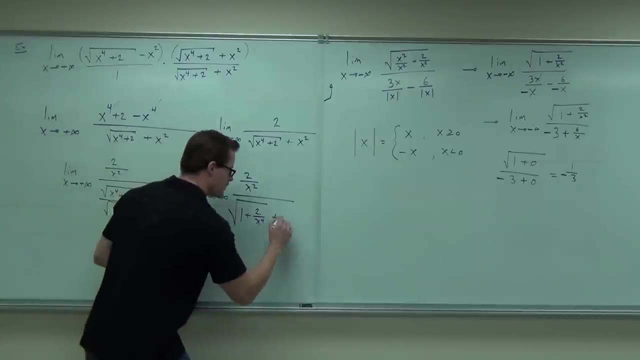 Do you see the 1 plus 2 over x to the 4th? Yes, no, Yeah, We get the 1x to the 4th over x to the 4th, plus the 2 over x to the 4th plus 1.. 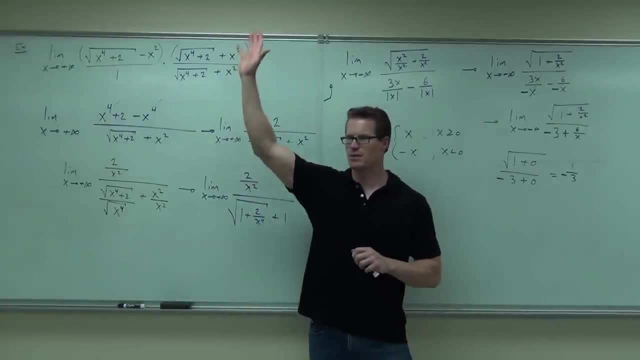 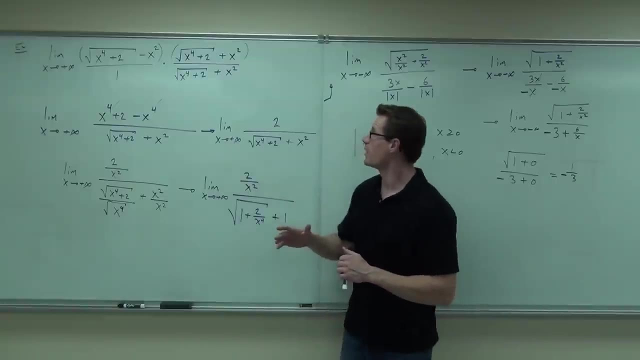 Yes, Yes. So how many of you feel okay getting down to that far? Well, that's not many. Let's have some questions, if you guys are not so okay on this. Are you okay on rationalizing? Yes, Are you okay on crossing those things out? 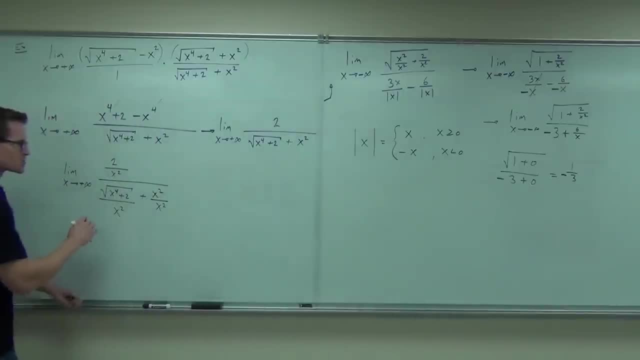 I was thinking about The Simpsons. So well, since this is x squared and this is x squared, we need to make this equal to x squared, but it also has to have a square root around it. You follow. You can't just do this because that's x. 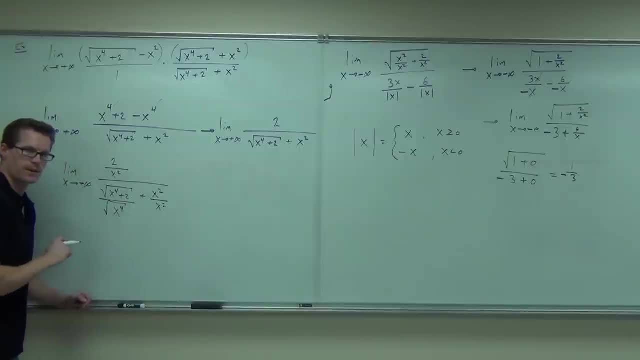 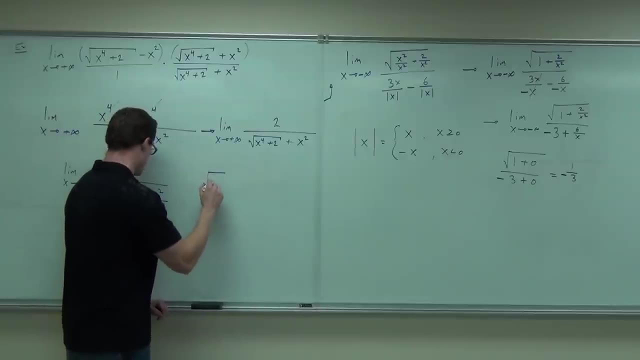 So change the power. is that true? Now some of you are going to ask me: well, wait a second, Mr Leonard, don't you have to have some absenteeism? What's the value here? Let me ask you this question. 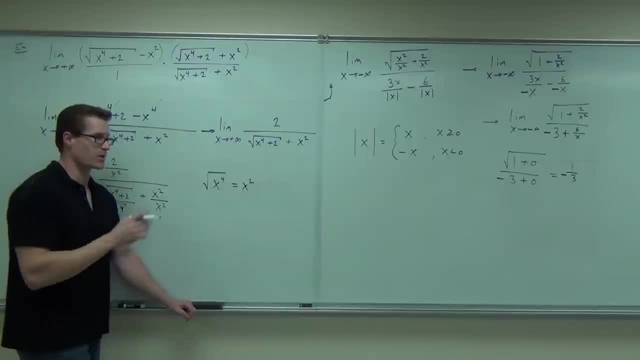 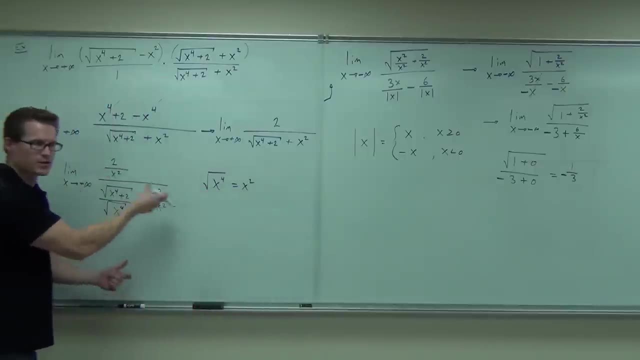 Is this always true? That actually is always true. no matter what, No absolute value needed because you have all positive, all positive. It's always going to be the same. Does that make sense? So we don't even need that for this case. 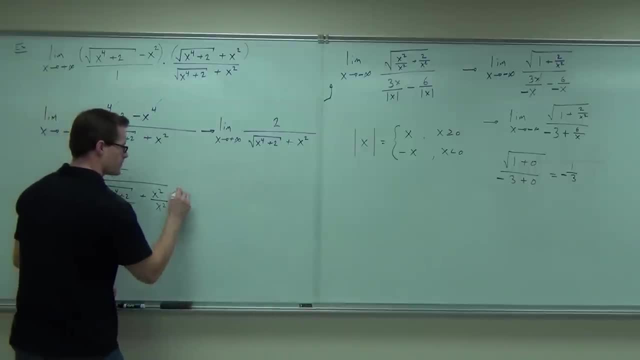 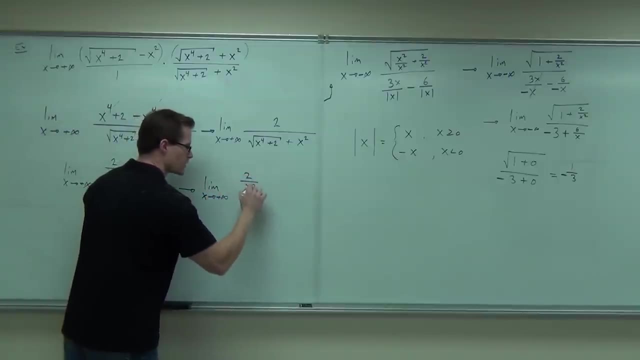 So here we're going to have. just wanted you to see that one time. Two over x squared all over, we're going to have the square root and, if you think about it, this is going to be one plus two over x to the fourth. 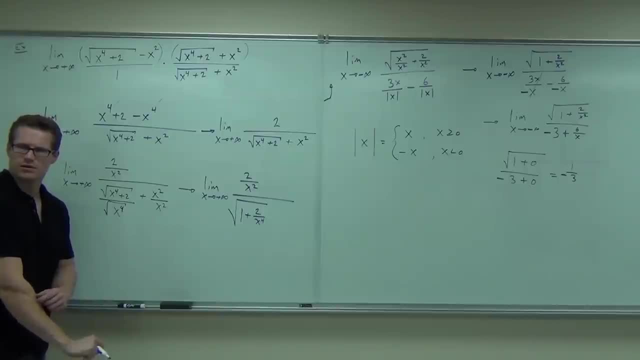 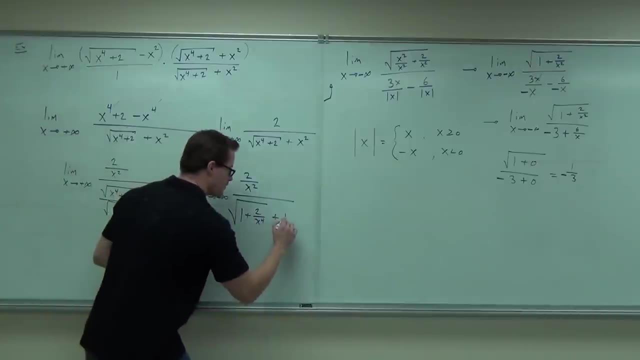 Do you see the one plus two over x to the fourth? Yes, no, We get the one x to the fourth over x to the fourth, plus the two over x to the fourth, plus one Show of hands. how many people feel okay? 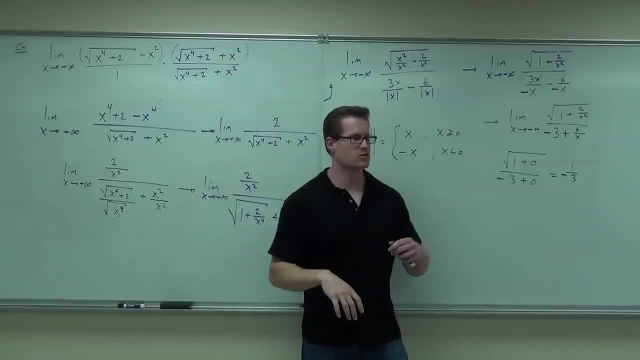 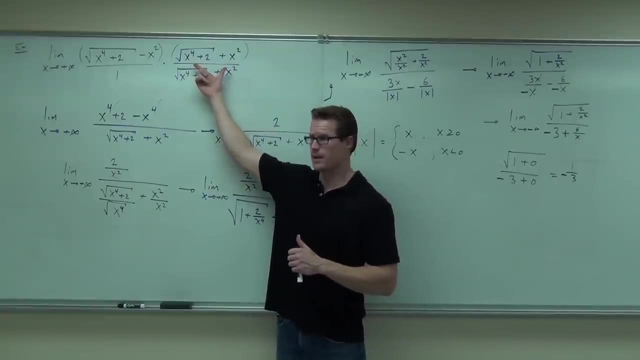 getting down to that far. Well, that's not many. Let's have some questions if you guys are not so okay on this, Are you okay on rationalizing? Yeah, Are you okay on crossing those things out? That should be easy. that's the fun part. 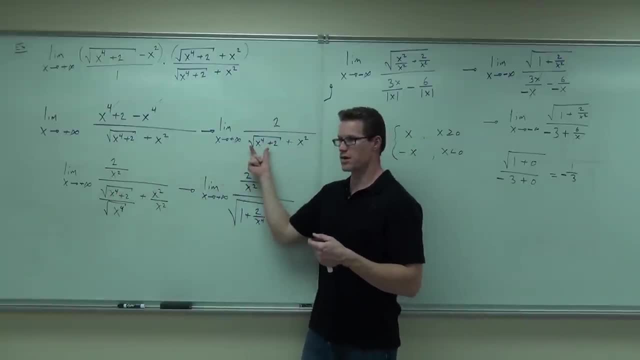 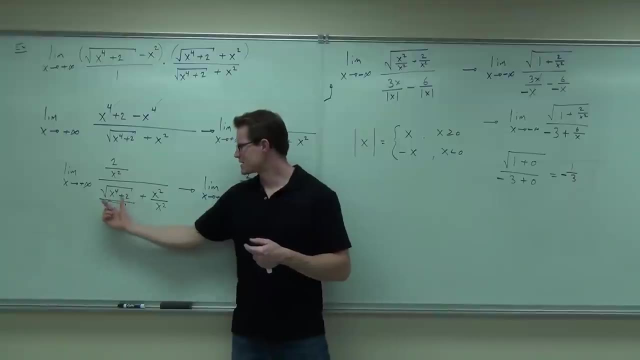 Are you okay on dividing by x squared, because that is the largest power in your denominator? You okay on doing the square root of x to the fourth, because that's still x squared? Then we take it inside, we have x to the fourth over x to the fourth. that's one. 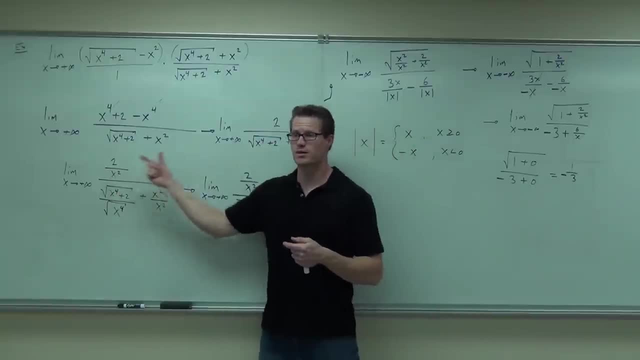 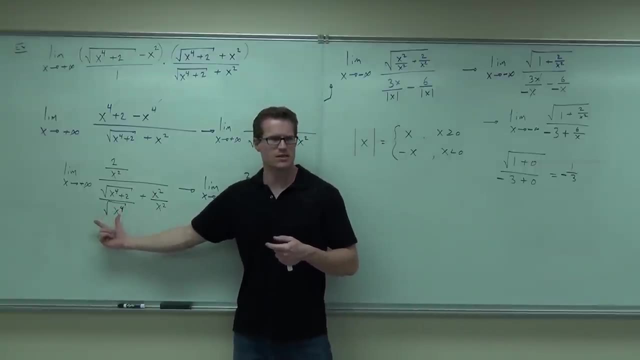 That should be easy. That's the fun part. Are you okay on dividing by x squared, because that is the largest power in your denominator? Are you okay on doing the square root of x to the 4th, because that's still x squared? 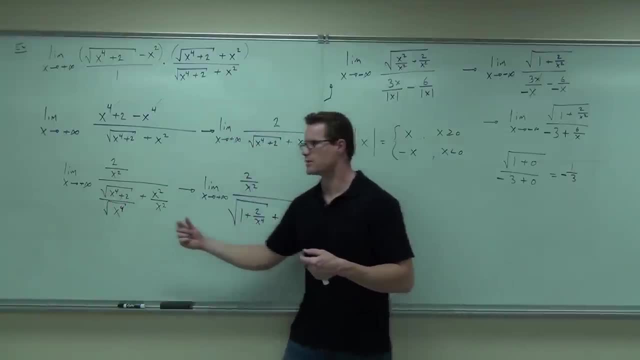 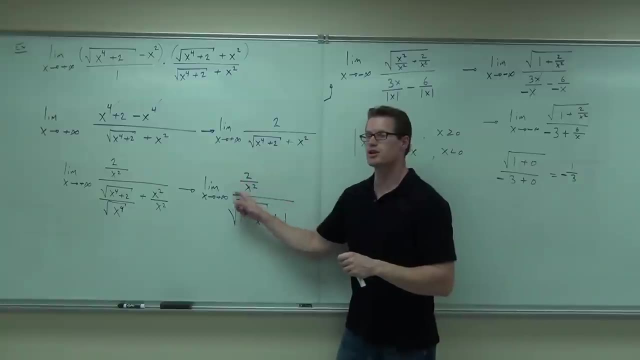 Then we take it inside, We have x to the fourth over x to the fourth, that's one. Two over x to the fourth, two over x to the fourth. x squared over x squared, that's one. Where does this go, ladies and gentlemen? 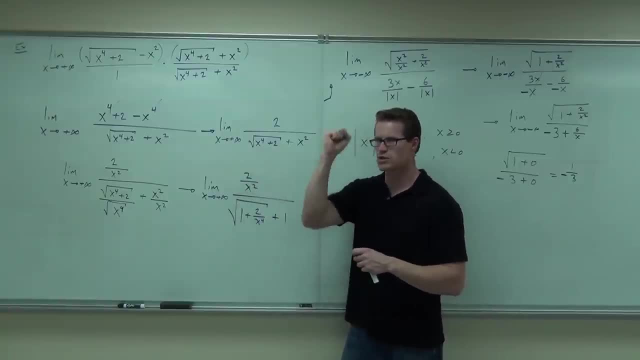 when we're taking it to infinity. where does that go? Is it okay to have zero on the top of the fraction? Where does this go? Where does this go? Where does this go? Would you agree that this denominator goes to two? 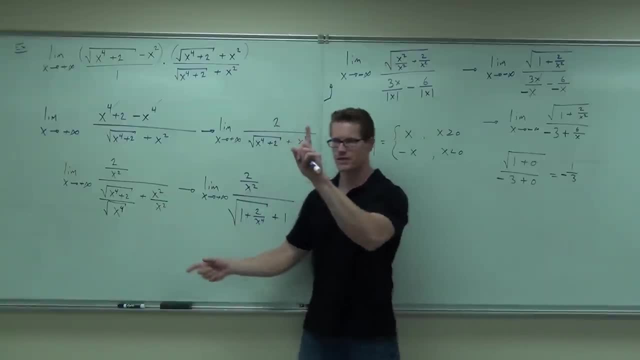 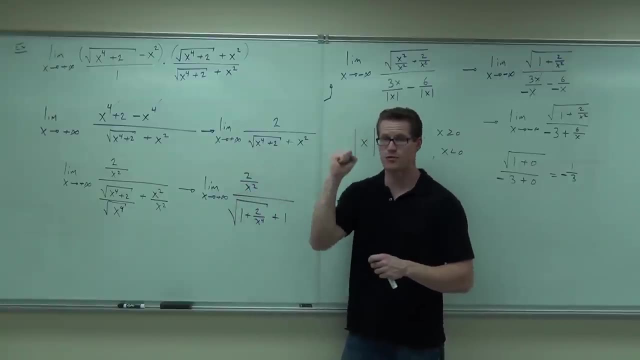 Two over x to the fourth, two over x to the fourth. X squared over x squared. that's one. Where does this go, ladies and gentlemen, when you're taking it to infinity? Where does that go? Is it okay to have zero on the top of a fraction? 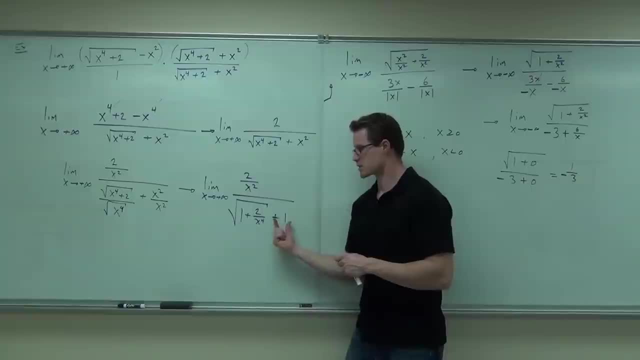 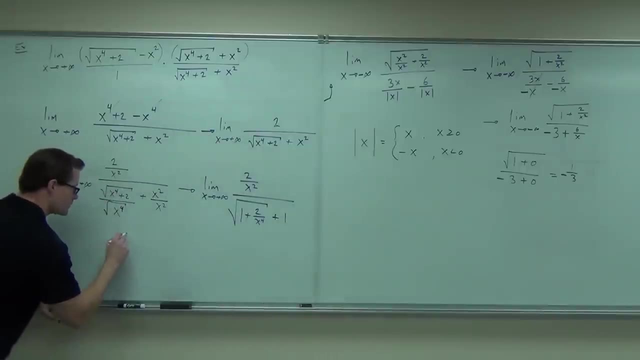 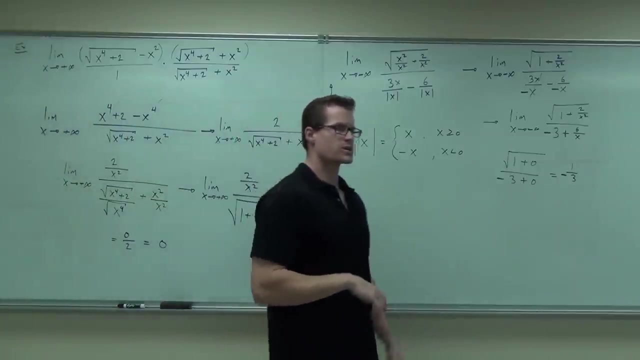 Where does this go? Where does this go? Where does this go? Would you agree that this denominator goes to two, So this equals zero over two or zero. You're gonna notice, in this case, if I change that to a negative, nothing about this changes. 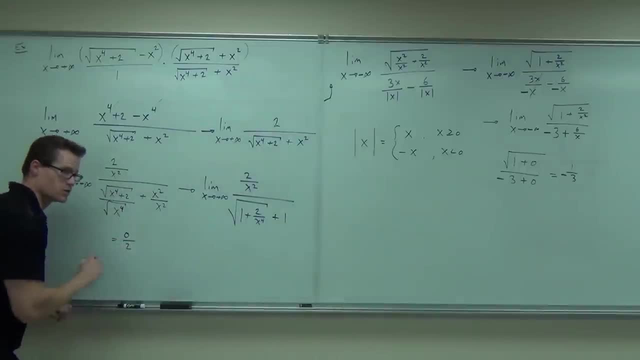 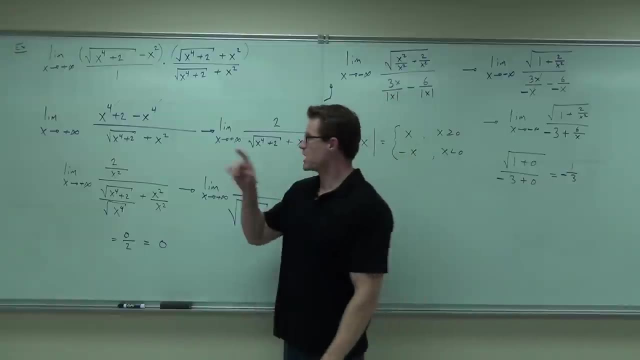 So this equals zero over two or zero Zero. You're gonna notice, in this case, if I change that to a negative, nothing about this changes. I don't have any absolute value. nothing changes. That says the horizontal asymptote in both directions is at zero. 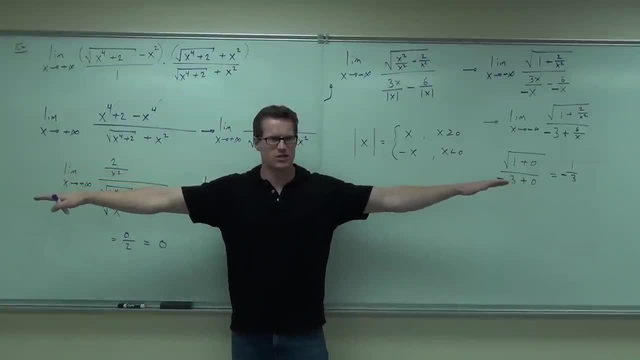 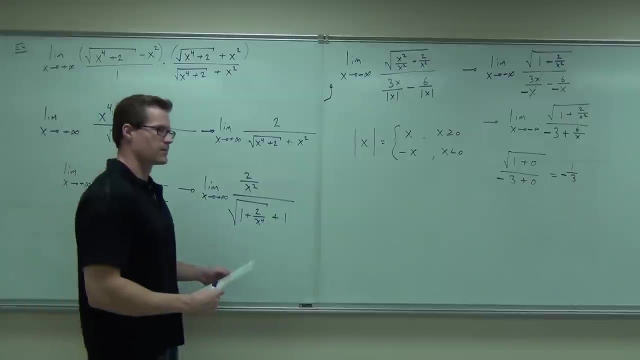 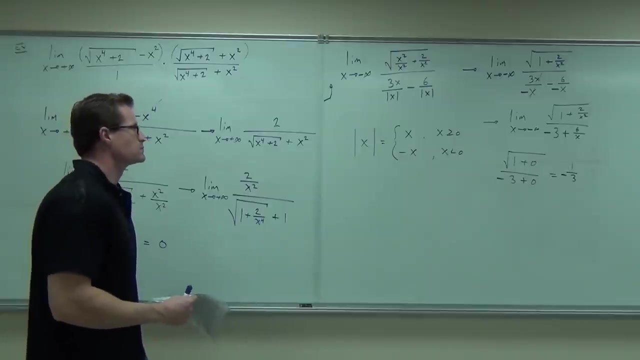 That's what it's gonna be, You following me on that one. Would you like to see one more case? Would that be all positive exponents, Or even exponents? Would that be the case? We didn't start with an even one there. 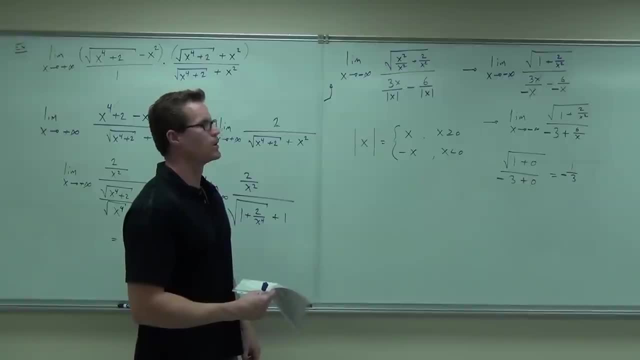 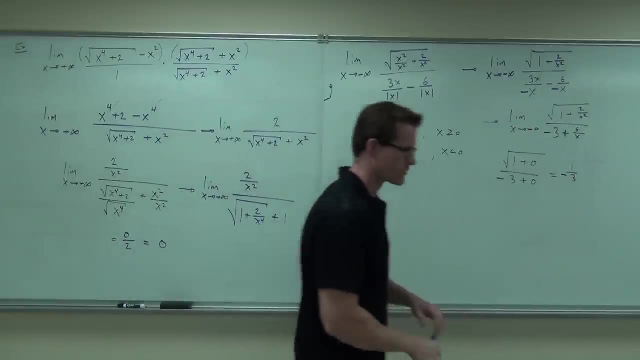 That was. I'm sorry, I don't know. that was even Divide and divide. Oh, I don't know. It really depends on what you have. I can't say a coverall situation for every time. Should we change the problem just a little bit? 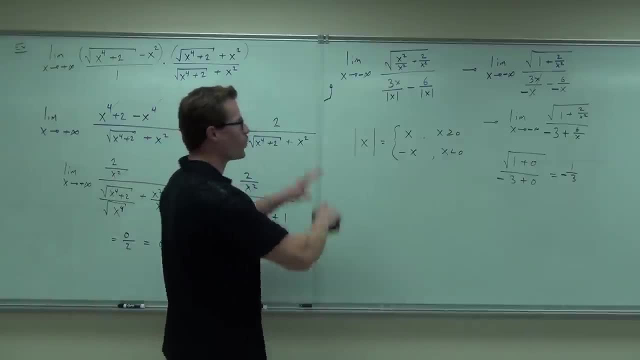 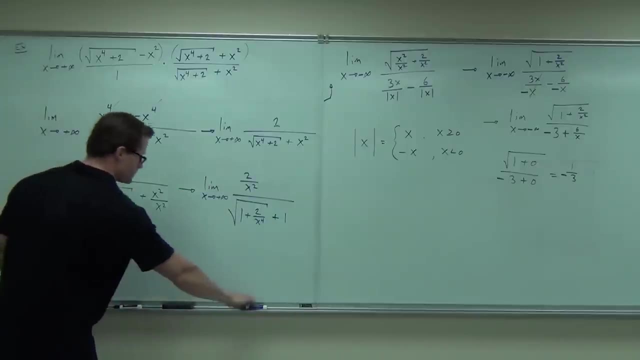 Change the problem just a little bit. all right, So what I'm gonna do instead of doing a whole, completely new one. Do you have any questions on this? We're gonna see how it changes if I do this little bit to it. 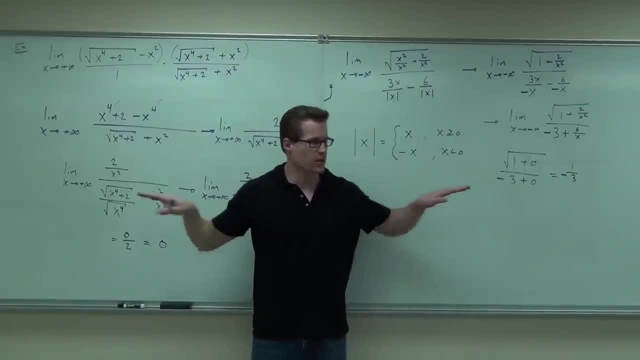 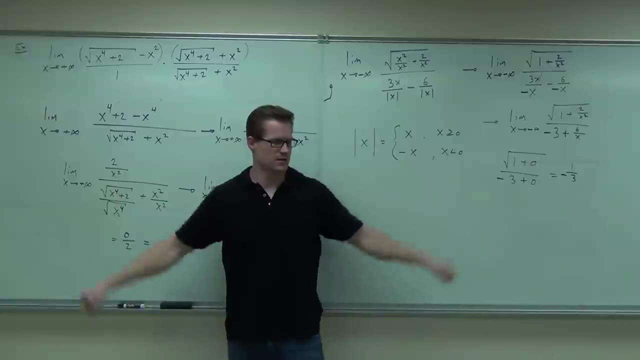 I don't have any absolute value. nothing changes. It says the horizontal asymptote in both directions is at zero. That's what it's gonna be. You following me on that one? Would you like to see one more case? Yeah, So would that be all positive exponents? 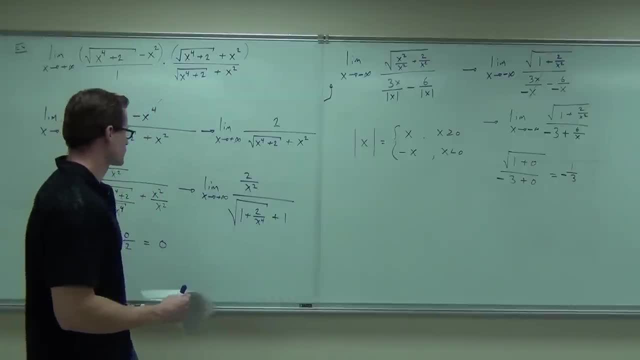 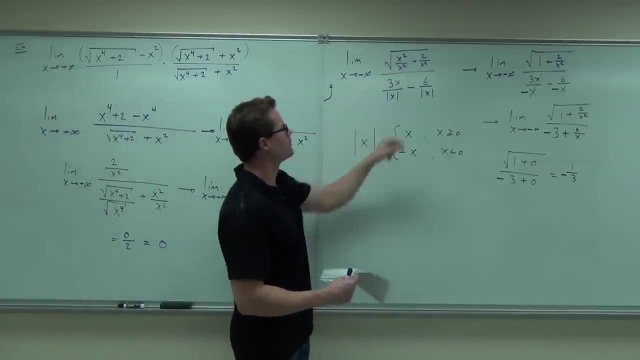 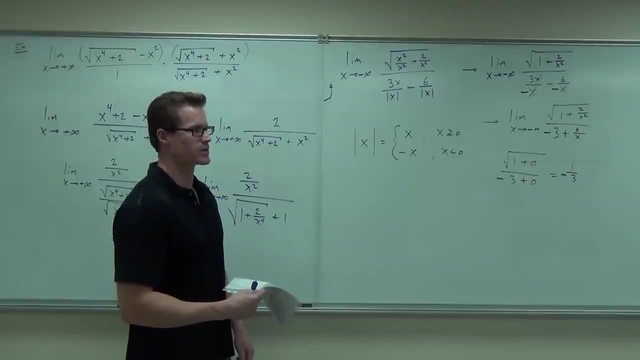 Or even exponents, right? Would that be the case? We didn't start with a new one there. That was- I'm sorry, I don't know. that was even Divide by five. Oh, I don't know. It really depends on what you have. 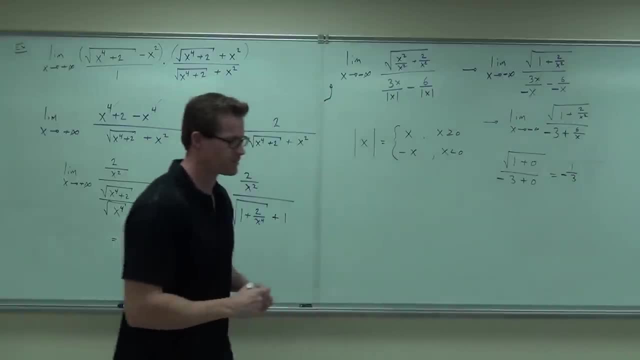 I can't say a coverall situation for every time. Should we change the problem just a little bit? Let's change the problem just a little bit, all right? So what I'm gonna do, instead of doing a whole completely new one? 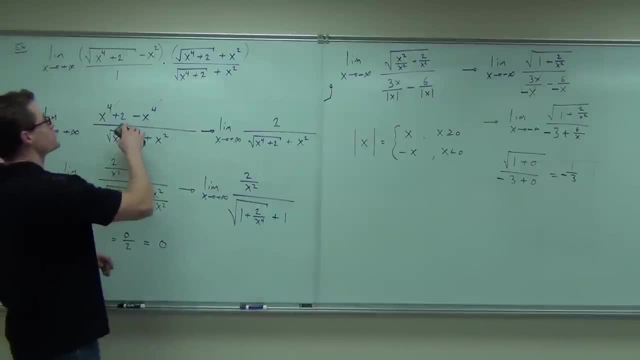 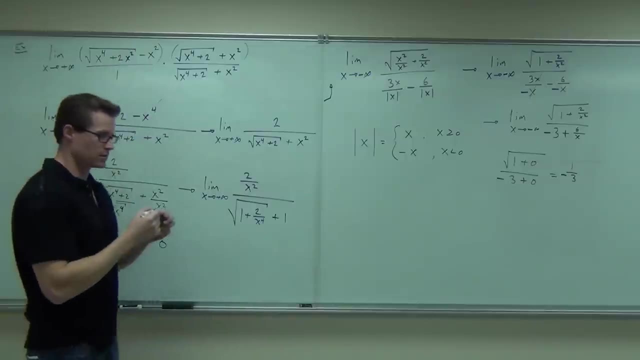 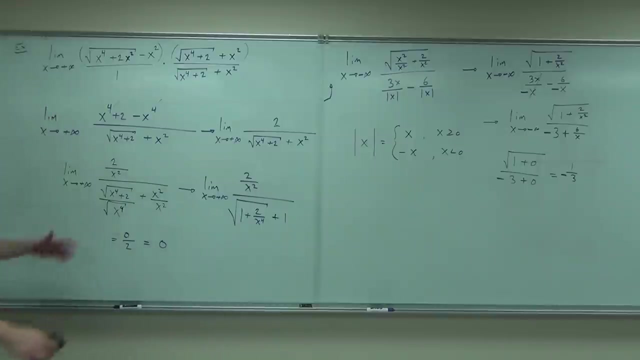 do you have any questions on this? We're gonna see how it changes if I do this little bit to it. That Okay, Let's see if that changes our problem at all. Let's see the things that change. Let's go through our problem. 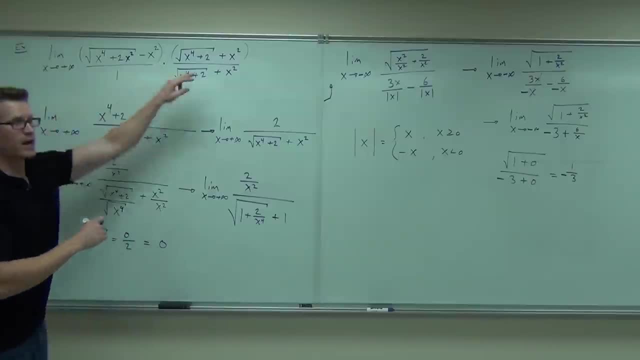 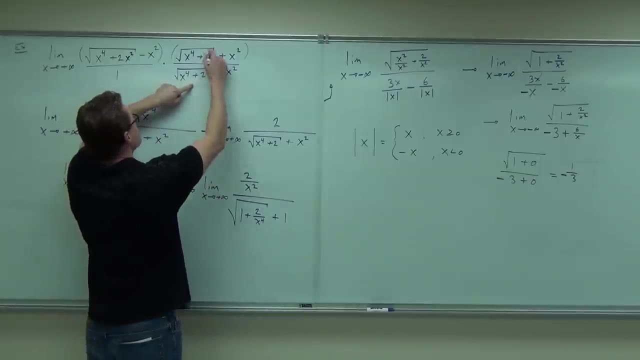 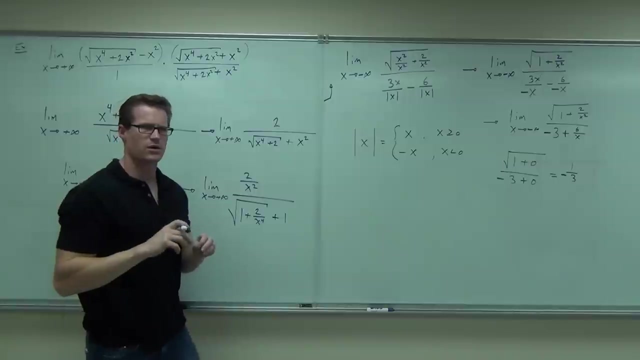 I'll try to use a different colored pen, so you see the differences. Can you still rationalize? What's the only thing that changes about our rationalization? That's gonna be an x squared. An x squared. Are you aware of that so far? 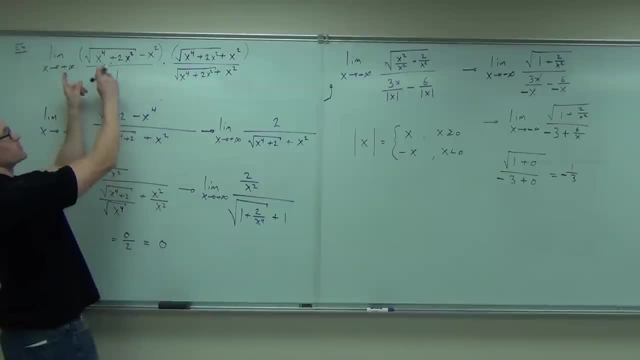 Okay, What changes here? ladies and gentlemen, when I distribute, What changes? Just an x squared, Just an x squared. You see it, It'd be kind of silly to do the whole example again. right, It's pretty much the same thing. 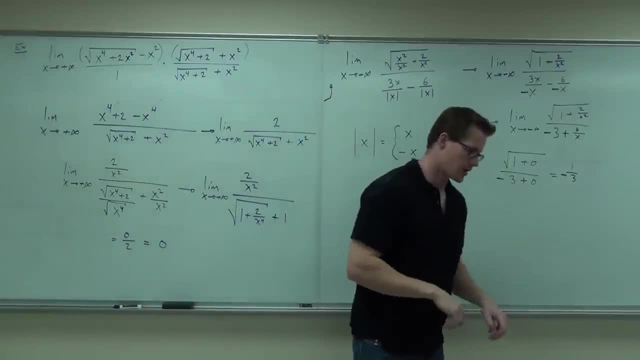 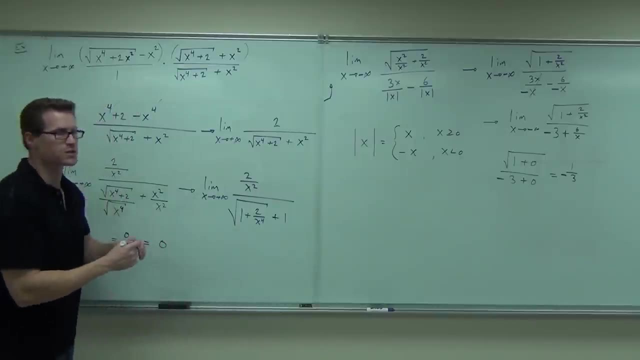 That Okay, if that changes our problem at all. Let's see the things that change. Let's go through our problem. I'll try to use a different colored pen so you see the differences. Can you still rationalize? What's the only thing that changes? 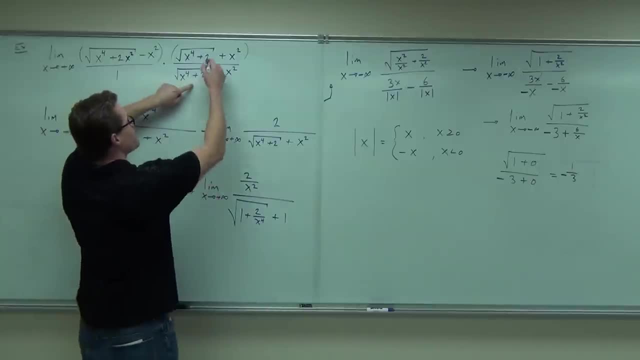 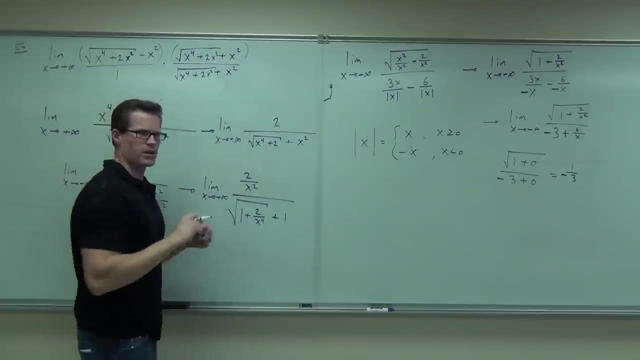 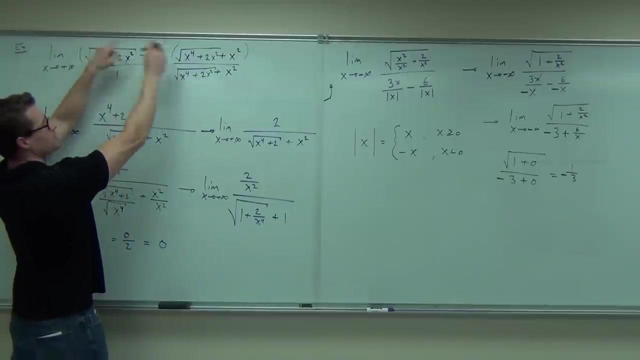 about our rationalization. That's going to be an x squared, an x squared. Are you aware of that? so far, Okay. What changes here? ladies and gentlemen, when I distribute, What changes? Just add an x squared, Just an x squared. 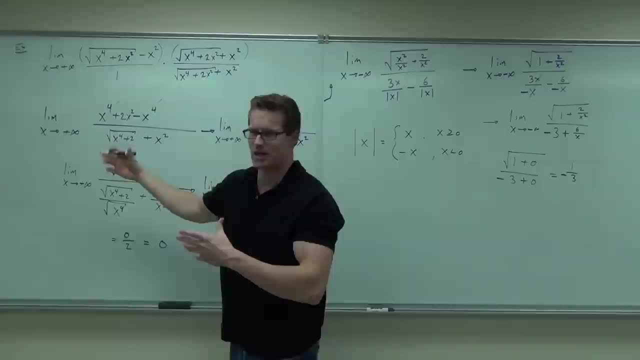 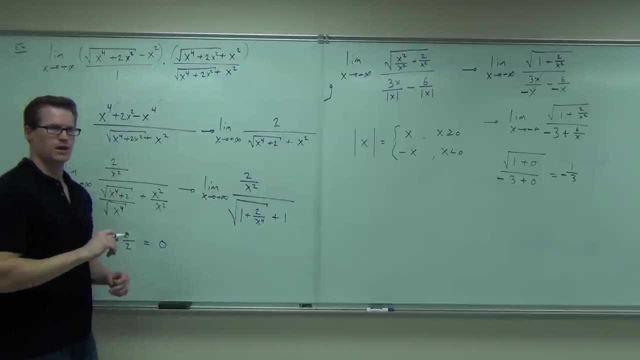 You see it, It'd be kind of silly to do the whole example again. right, It's pretty much the same thing. That would be an x squared and this would be an x squared. You still okay? Well, what happens here, then, is this is an x squared. 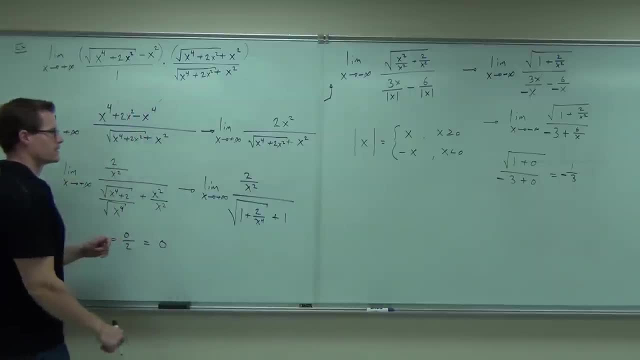 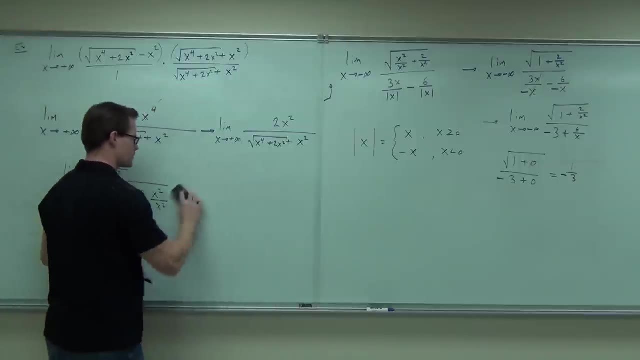 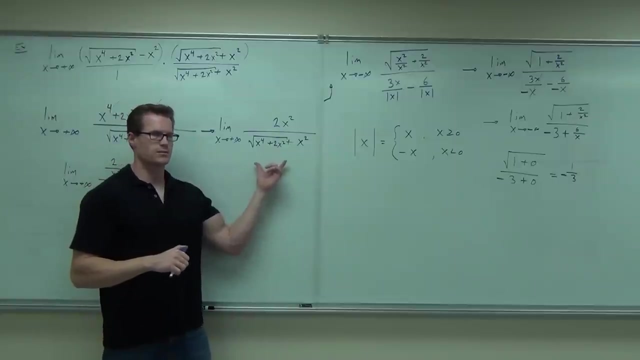 and that's an x squared, True, Okay, So okay, well, hang on a second then. Well, if that's the case, are we still going to be dividing by x squared down here? Yeah, because that's still the largest power. 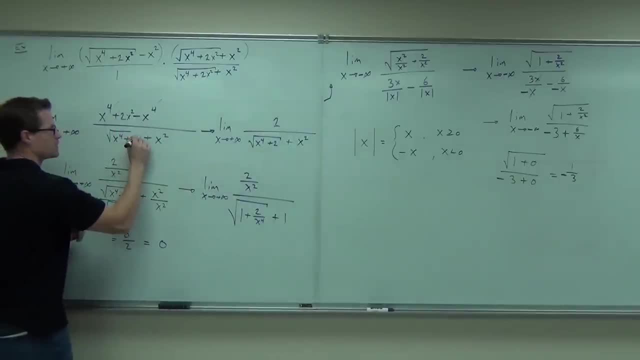 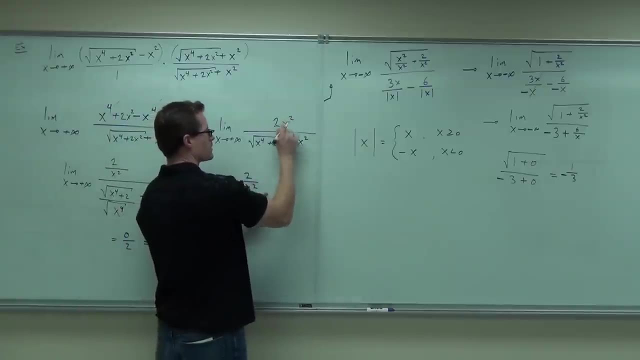 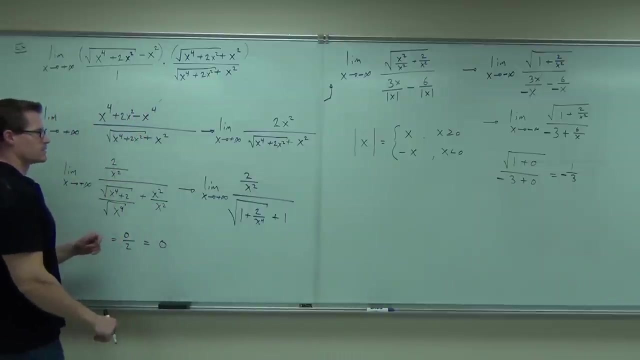 That would be an x squared, and this would be an x squared. You still okay? Well, what happens here, then, is: this is an x squared and that's an x squared, True, Okay, So okay. Well, hang on a second then. 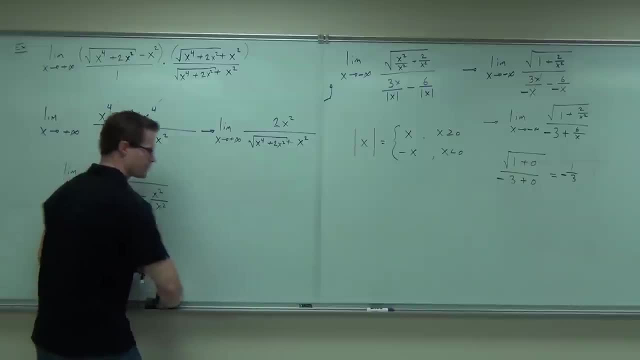 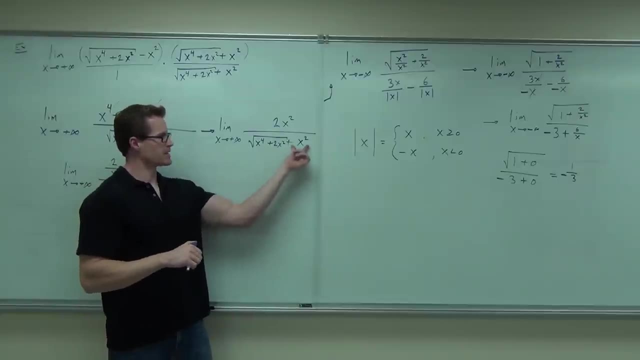 Well, if that's the case, are we still gonna be dividing by x squared down here? Yeah, because that's still the largest power. That's not That. actually, if you looked at, it would be x. The square root of x squared is x. 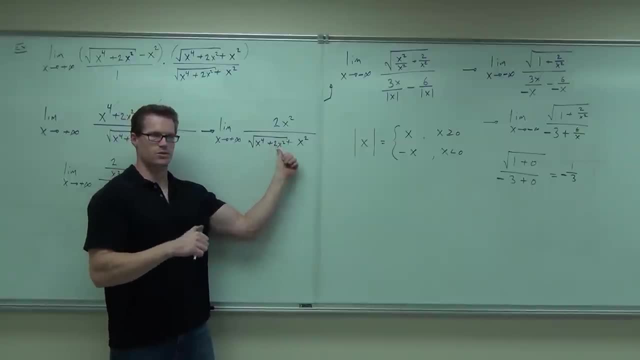 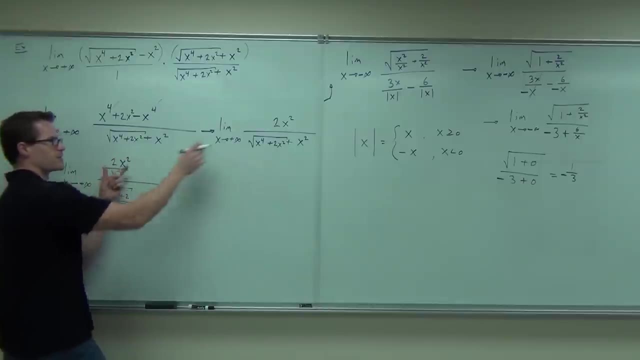 That's not That. actually, if you looked at it would be x squared over x, So that wouldn't be the largest power. We'd still divide by x squared. we'd still divide by x squared. but now I have an x squared right there. 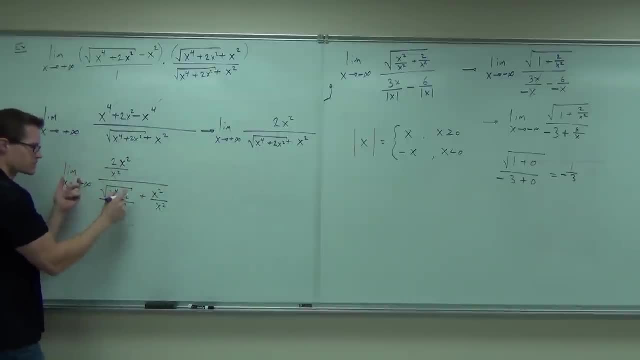 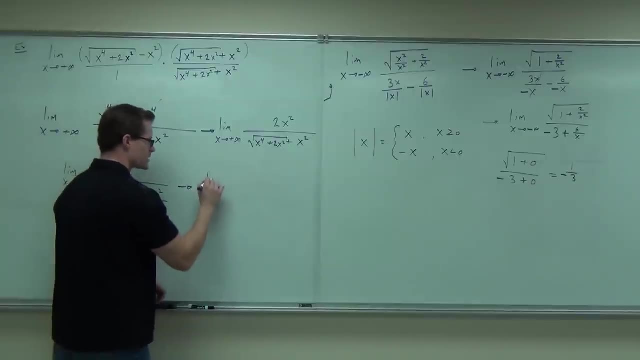 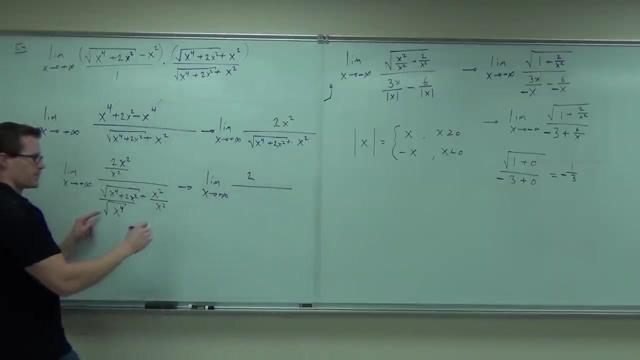 That 2x squared. that's right there. This would look almost the same, except I have an x squared there. What that means is I'll have a limit as x approaches positive infinity, of 2 over. this is going to give you 1, plus 2 over x squared. 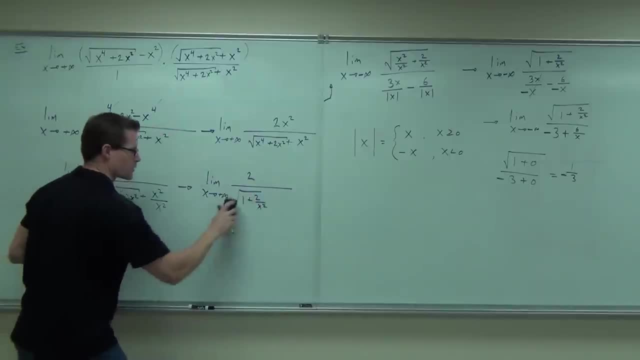 So that's going to be the largest power. So that's going to be the largest power. So that's going to be the largest power over x squared. You know, I'll show all the work for you in case you're having trouble following me. 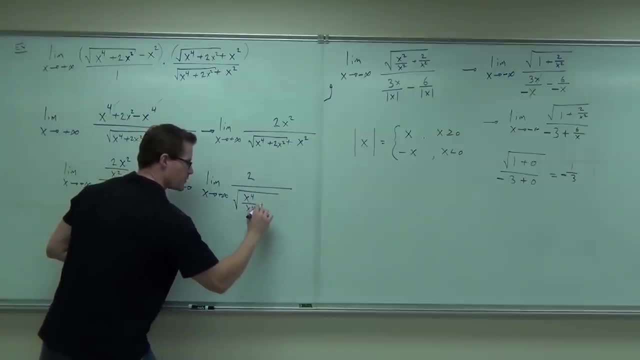 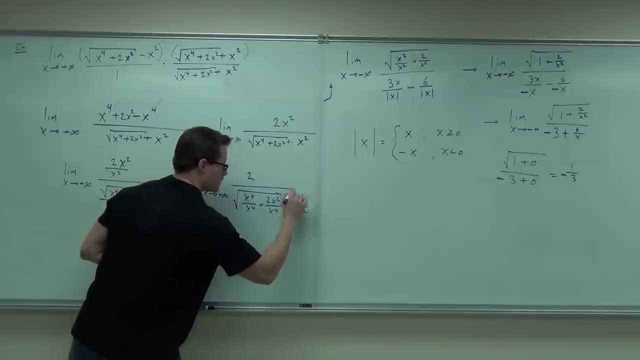 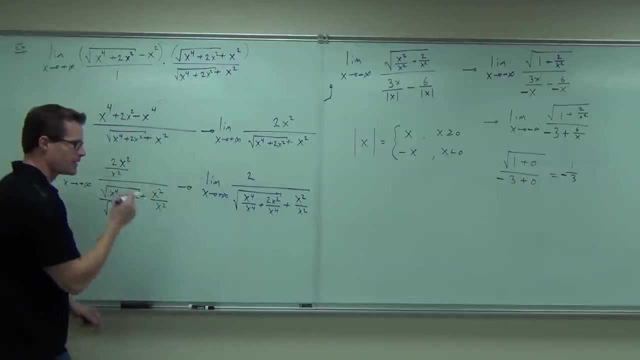 x to the 4th over x to the 4th, plus 2x squared over x to the 4th, x squared over x squared. Are you guys satisfied? with that one, Hopefully, Yeah. Okay, good, This gives you 1.. 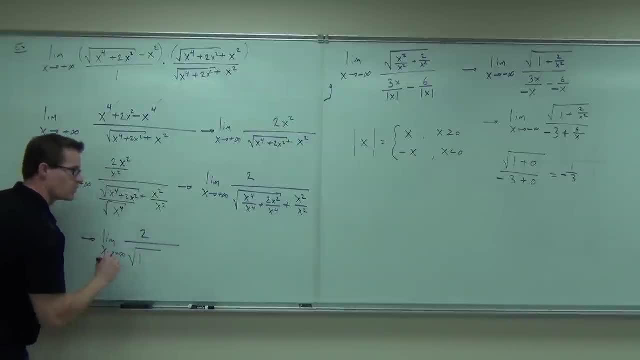 So we're still at 2.. That gives you 1.. This gives you 2 over x squared and that gives you 1.. We're now ready to take the limit, ready to let the x go to infinity? What happens to our 2?? 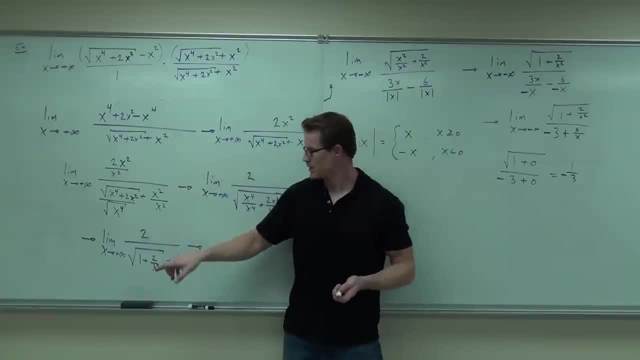 Does it go to 0?? It didn't last time because we had an over x. Where does that go? Where does that go? Where does that go? 1.. What is it? 1.. 2. We've got a 2 over the square root. 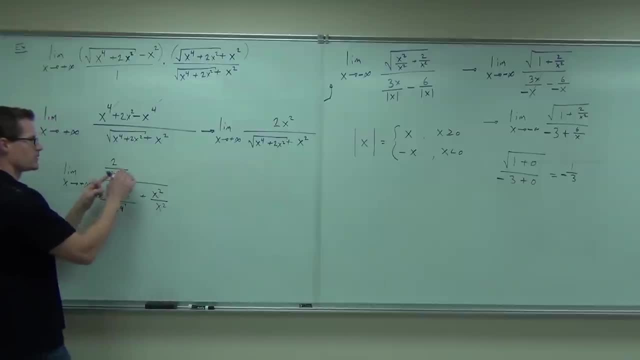 so that wouldn't be the largest power, We'd still divide by x squared. We'd still divide by x squared. but now I have an x squared right there, That 2x squared, that's right there. This would look almost the same. 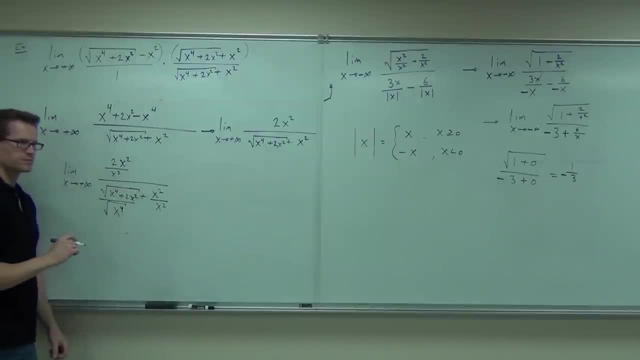 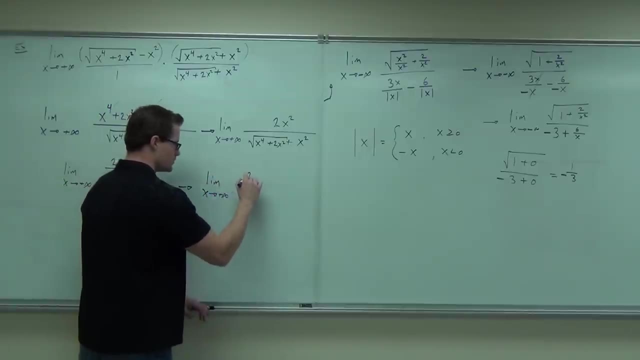 Except I have an x squared there. What that means is I'll have a limit as x approaches positive infinity of 2 over this is gonna give you 1, plus 2 over x squared. You know what? I'll show all the work for you. 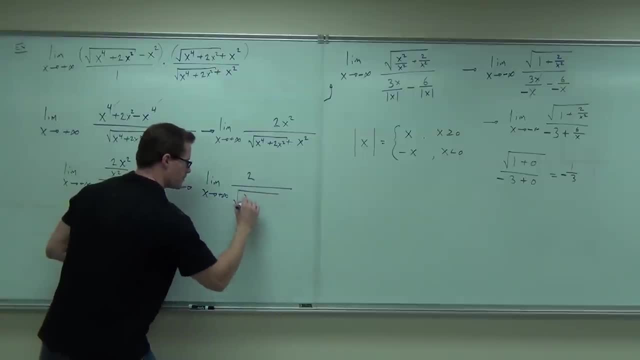 in case you're having trouble following me: x to the fourth over x to the fourth, plus 2x squared over x to the fourth. x squared over x squared. Are you guys satisfied with that one? Hopefully, Yeah, Okay, good. 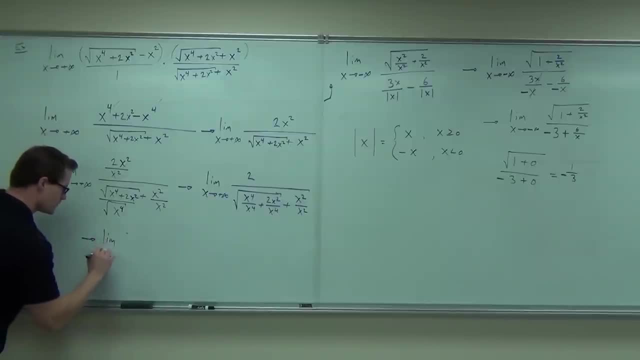 This gives you 1.. So we're still at 2.. That gives you 1.. This gives you 2 over x squared, And that gives you 1.. We're now ready to take the limit, Ready to let the x go to infinity. 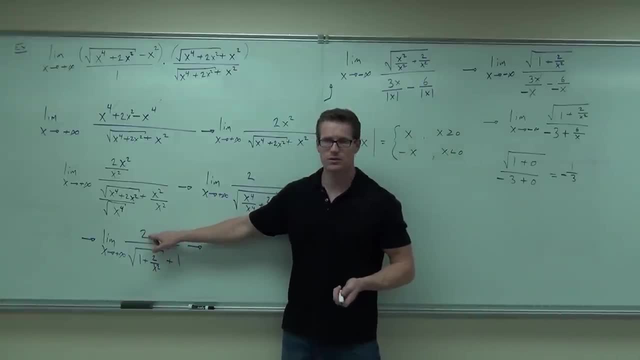 What happens to our 2? Does it go to 0? It didn't last time because we had it over x. Where does that go? Where does that go? Where does that go? What is it? We've got a 2 over the square root. 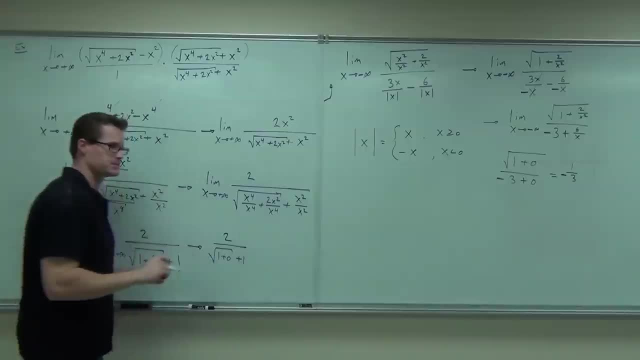 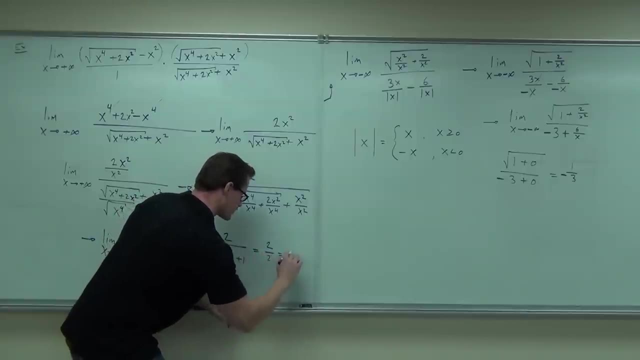 of 1 plus 0 plus 1.. 1 plus 0 plus 1.. That's the square root of 1.. That's 1.. 1 plus 1 is 2.. That's going to be a 2 over 2.. 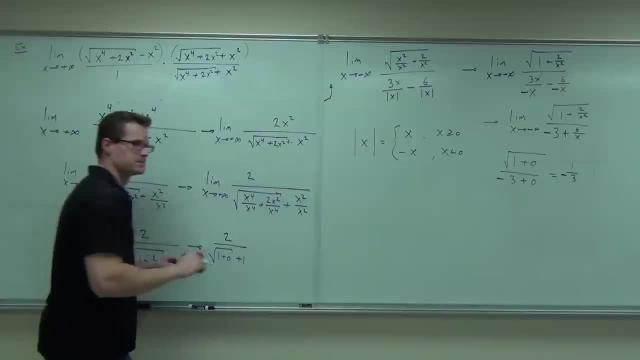 of x squared over x squared 1.. 1. 1 plus 0 plus 1.. 1 plus 0 plus 1. That's the square root of 1.. That's 1.. 1 plus 1 is 2.. 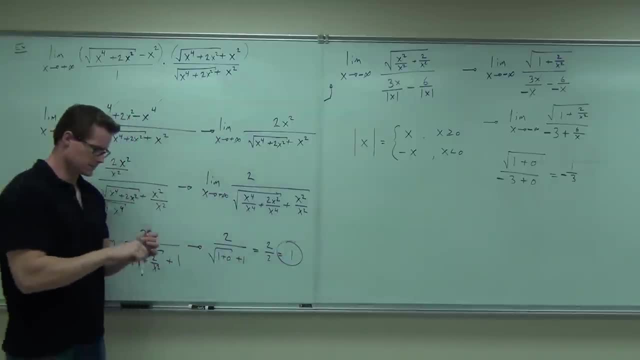 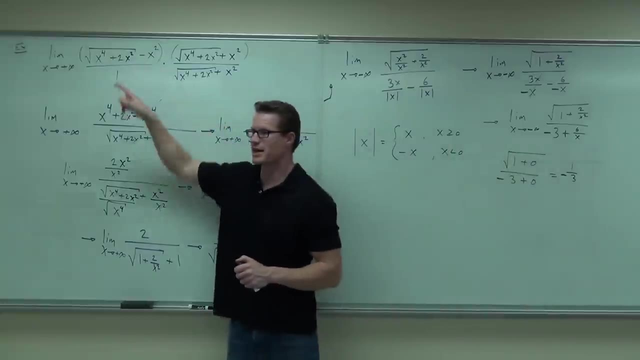 We get 2 over 2. Or 1.. Did it change So a little bit? Yeah, a little bit. So that little change there said we're not at 0 anymore, We have a horizontal asymptote at now 1.. 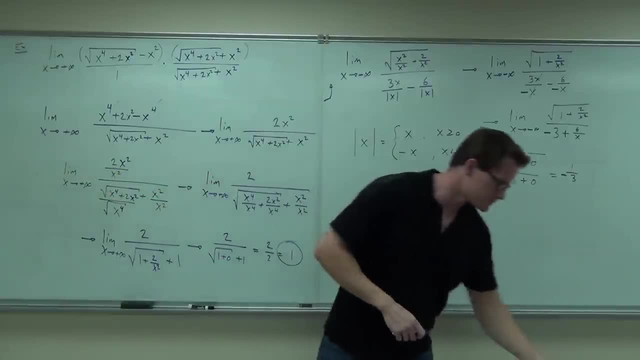 So we're going at 1, or when we get to infinity. How do you feel okay with what we've talked about so far? I'm not sure. I'm just going to say that's what I would like it to be. 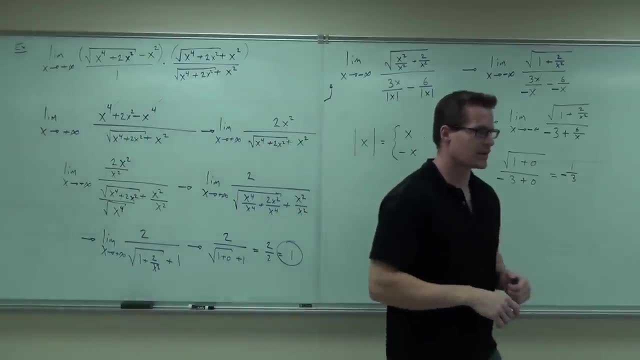 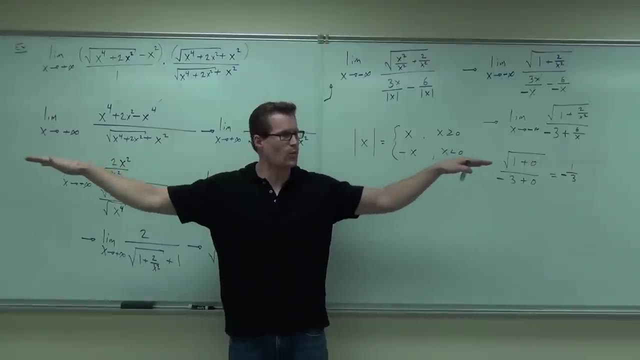 Did it change? So a little bit, Yeah, a little bit. So that little change there said: we're not at 0 anymore. We have a horizontal asymptote at now, 1.. So we're going at 1 when we get to infinity. 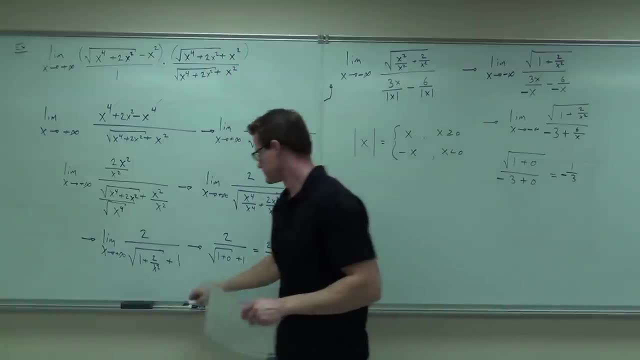 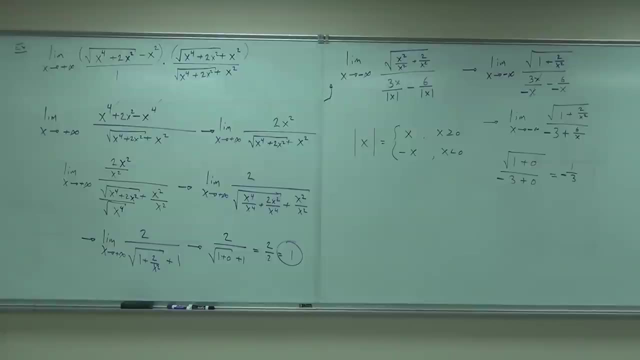 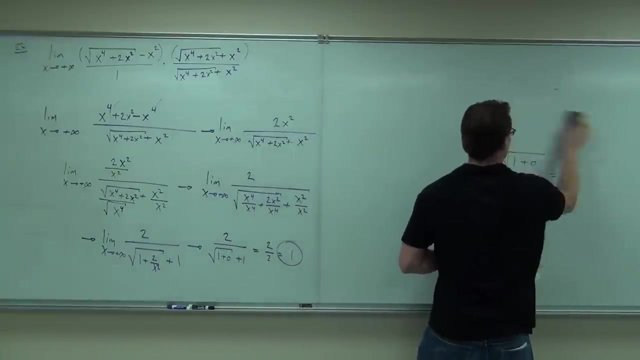 How many of you feel okay with what we've talked about so far? Allergies, Allergies are getting to me OK. last one: Is it making sense so far? Can you follow that, Shane? you, okay, Yeah. 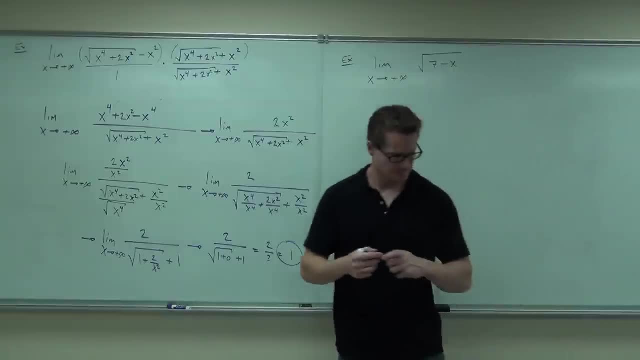 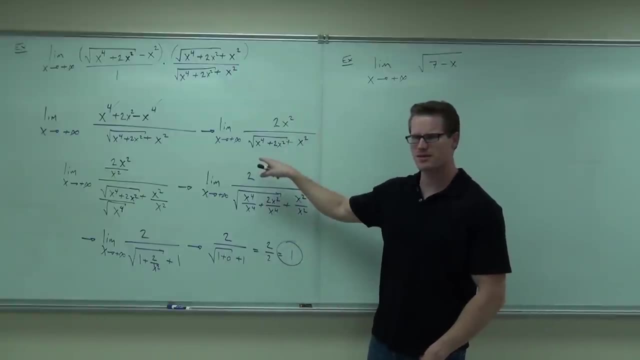 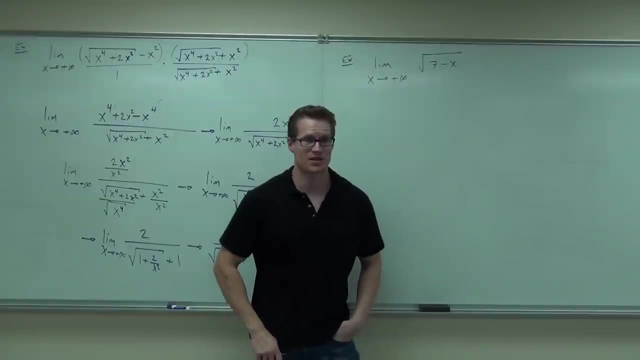 Ooh, that's nasty. Still sure you're okay with that one. Yeah, How about that one? No, no, no. Conjugate A little tougher, Conjugate. There's nothing to sing as conjugate Here. 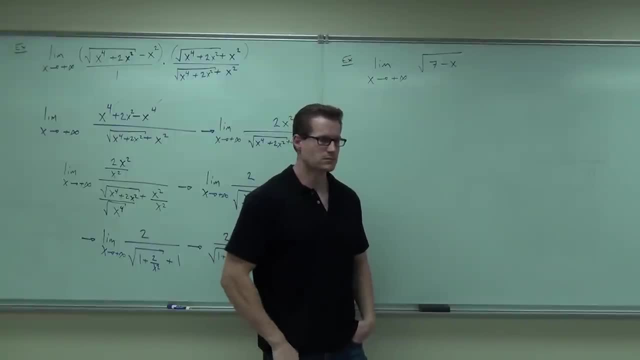 There's nothing to distribute. No, On the top and the bottom. you're still. I don't need to explain. Can't you just take it for a minute? Just think about it? for a second Derivative: No derivatives. Oh, good try though. 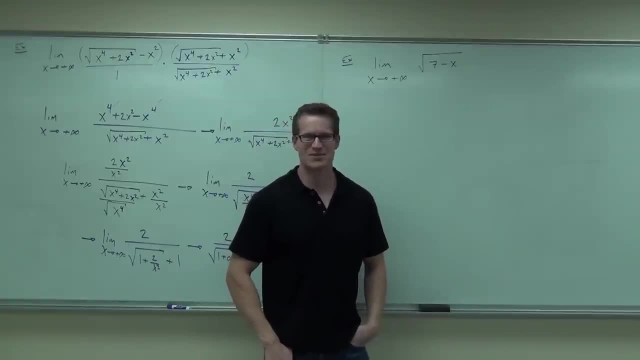 When you don't really know the answer, just derivative, that Good try. That's one of those 5% that doesn't work. Oh man, Yeah, close. No, It doesn't exist. Why It's going to. 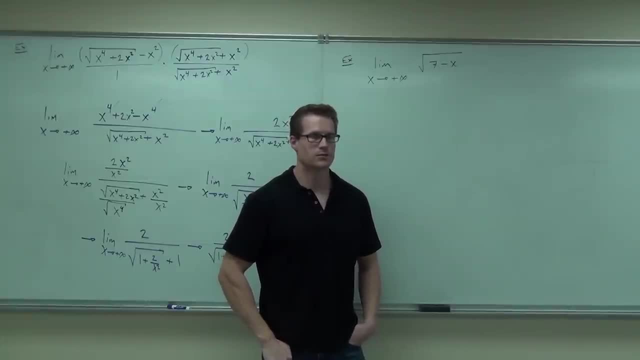 You have a negative under the square root. Ah, So if I take really big positive numbers, subtract them from 7, are they going to be positive or negative? And they're under a square root Define. It doesn't exist. Oh. 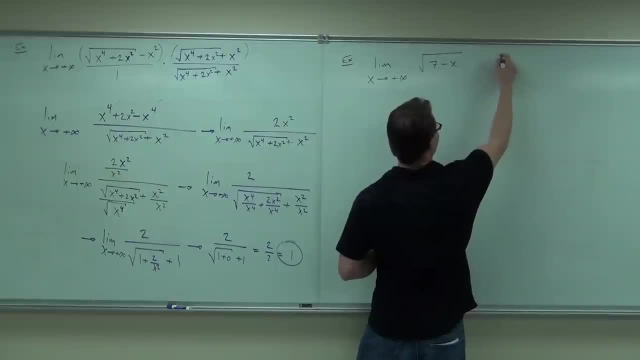 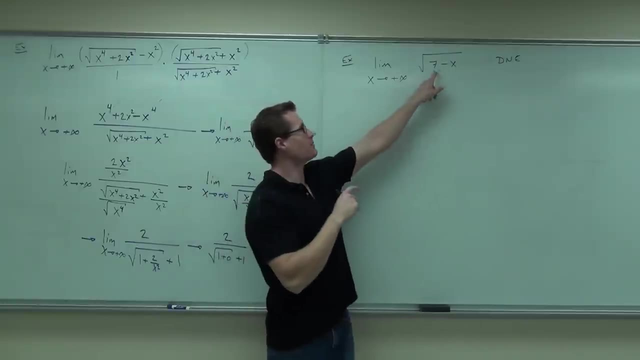 That was the easiest problem of the day. Come on, No, it doesn't exist. So think about your limits. I mean, you can think of them like that You have a 7 minus something huge. 7 minus something huge is something really negative. 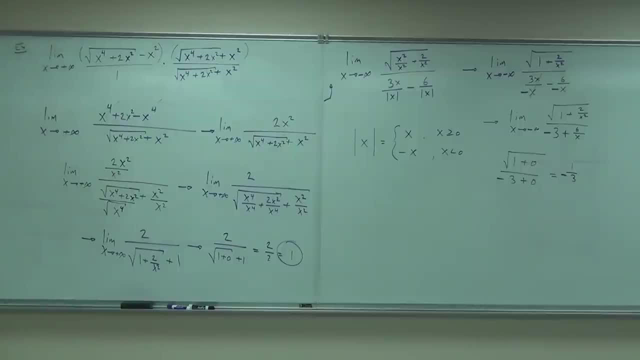 You know we've got a 2 here. I'm just going to keep telling you of It's the same stuff. And here's what I'm going to do. I'm just going to keep telling you of It's the same stuff. 1., 2., 3., 4., 5., 6., 7., 8., 7., 8., 9., 10., 11., 12., 13., 14., 15.. 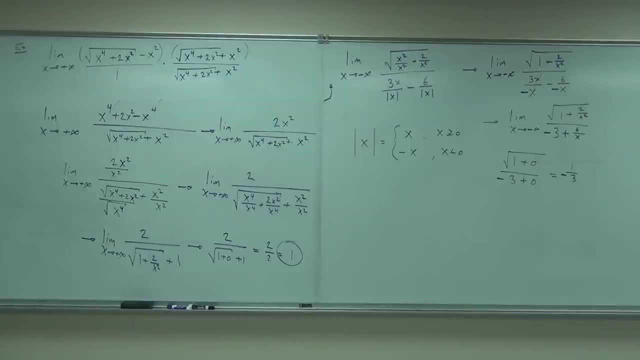 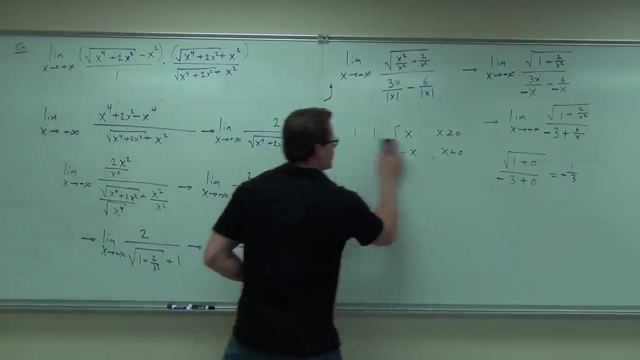 16., 17., 18., 19., 20., 21., 22., 25., 23., 24., 27., 28., 29., 30., 31., 32.. Okay, last one, is it making sense so far? 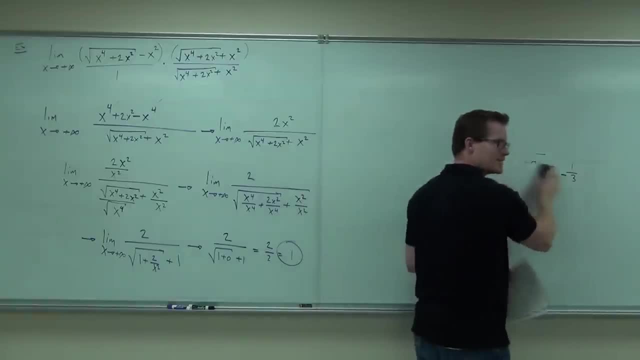 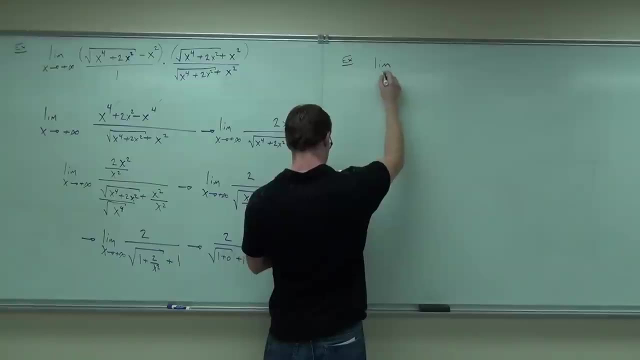 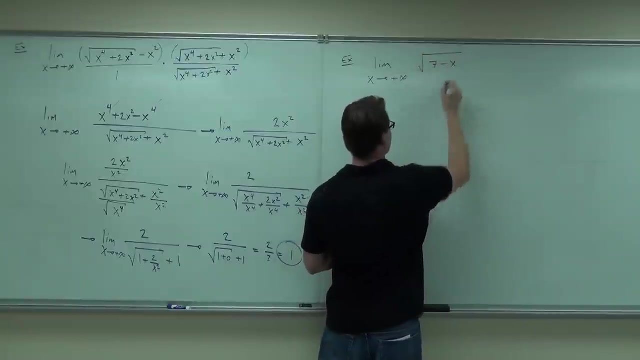 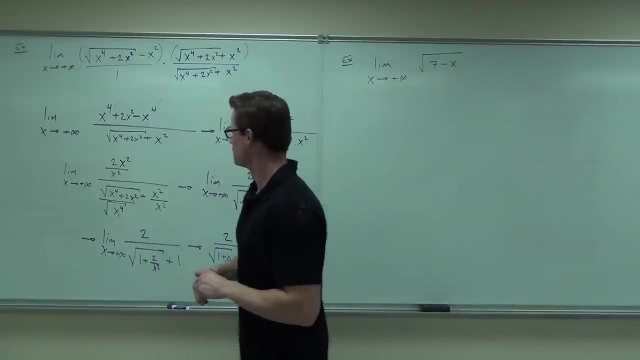 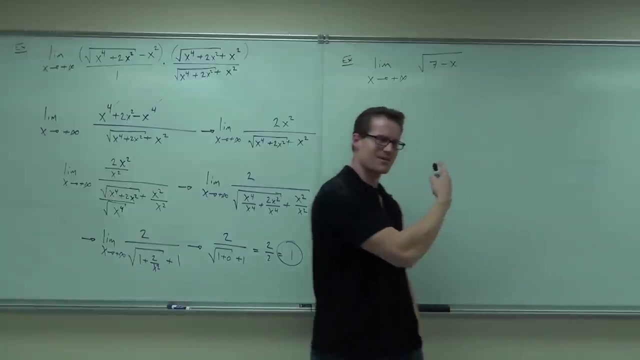 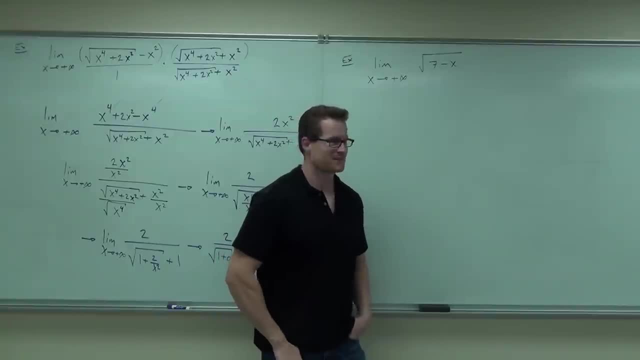 A little tough conjugate. there's nothing to sing as a conjugate here. This is nothing to distribute On the top and the bottom. you're Just think about it for a second. No derivatives. Oh, good, try though. 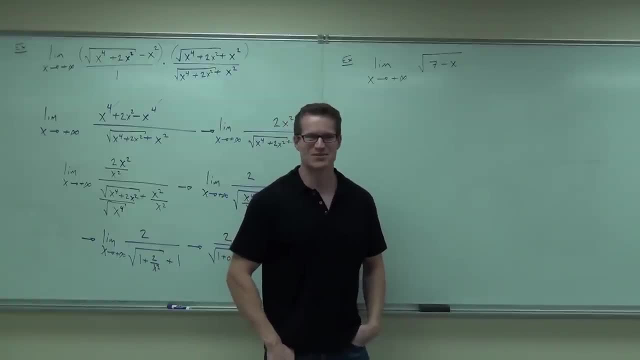 When you don't know the answer, just derivative. that Good try, That's one of those five percent. Oh man, Yeah, close, No, Huh, It doesn't exist Why It's going to. you have a negative under the square root. 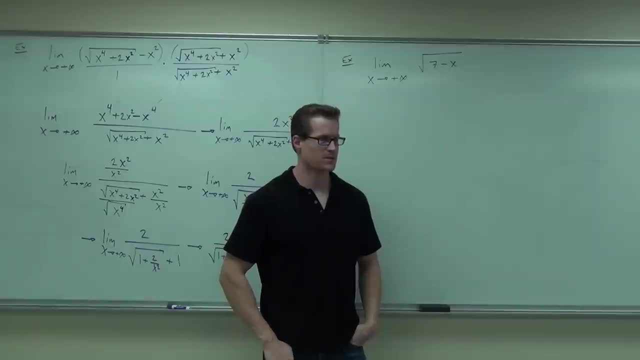 Ah. so if I take really big positive numbers, subtract them from seven, are they going to be positive or negative? And they're, under a square root, Undefined. It doesn't exist. Oh, That was the easiest problem of the day. 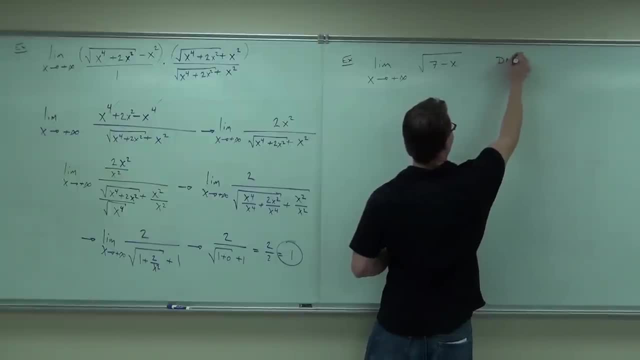 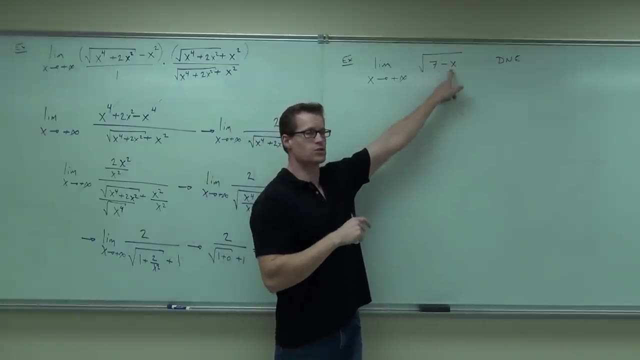 Come on. No, it doesn't exist. So think about your limits. I mean, you can't think of them like that. You have a seven minus something huge. Seven minus something huge is something really negative. Square root of something negative is undefined. 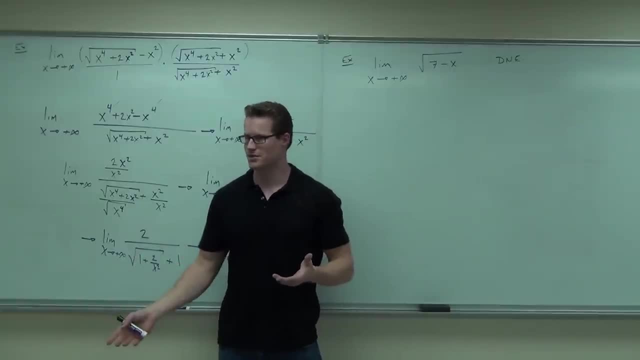 Square root of something negative is undefined. Therefore, a limit does not exist. Does that make sense? Now, if I did this, it's not harder. It's the same idea. You have 7 plus a really big number. Square root of that is still a really big number. 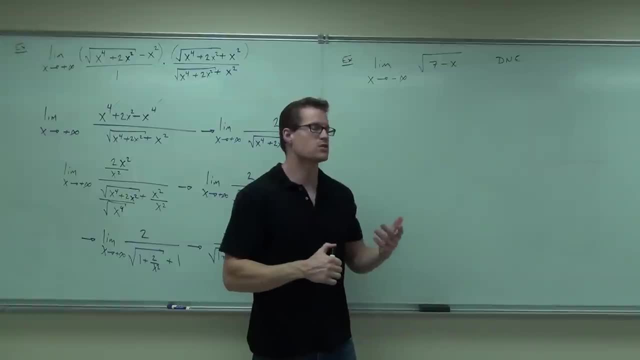 It's infinity, All right, So you can think of that. The only problems you really come up with is when you do things like infinity plus or minus infinity, infinity over infinity. That sort of thing gets you. You can't do those. 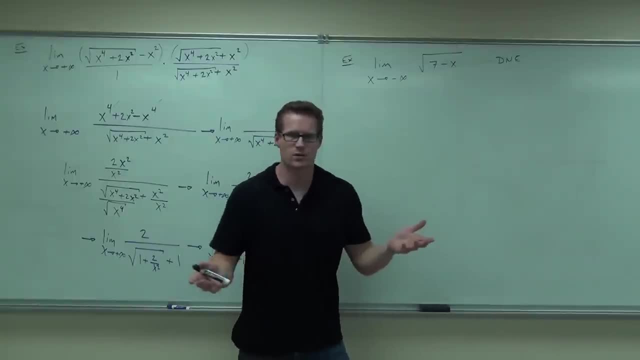 But if you know it's going to infinity or it's not going anywhere, that's fine, That's OK. You can consider things like that. There's no denominator, Nothing to divide by, You're good. Does that make sense? So negative infinity. 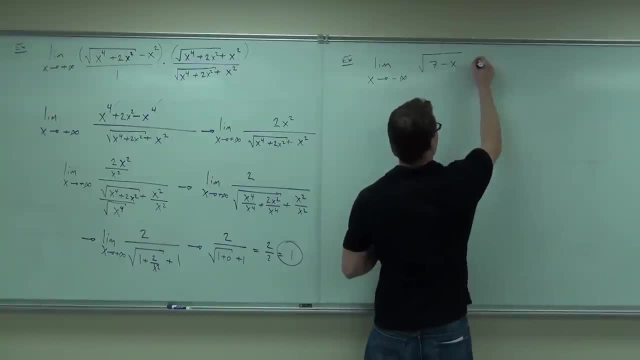 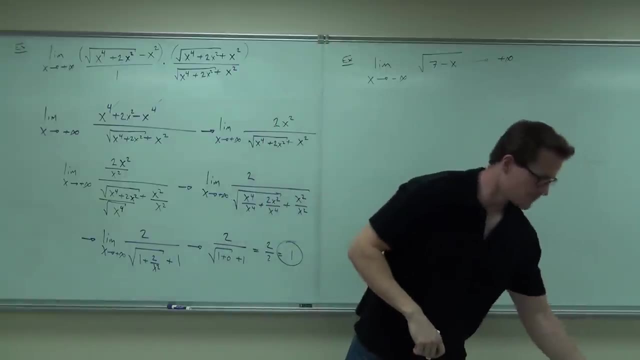 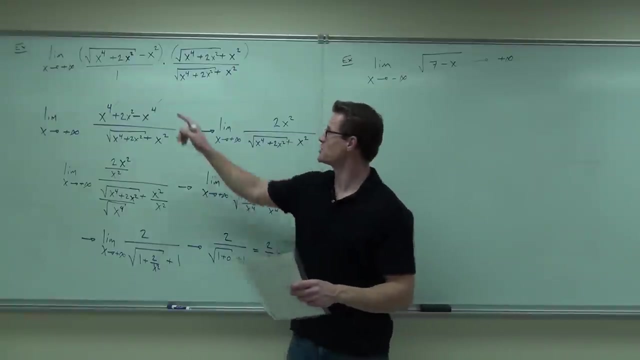 This, No, This is actually positive. Oh, it's positive, Yes. Do you feel OK with our limits? Have I blown your minds yet today? So when you have issues where you're subtracting infinities, rationalize them. 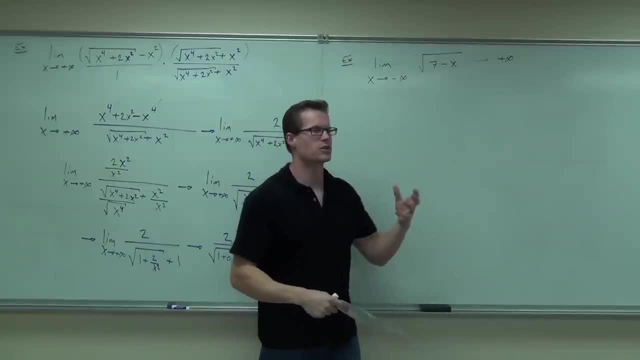 If you have a square root, rationalize them. If you don't think through the limit and what it means to go to infinity, consider the type of problems you have. You already know polynomials. Any polynomial is going to go to the positive. 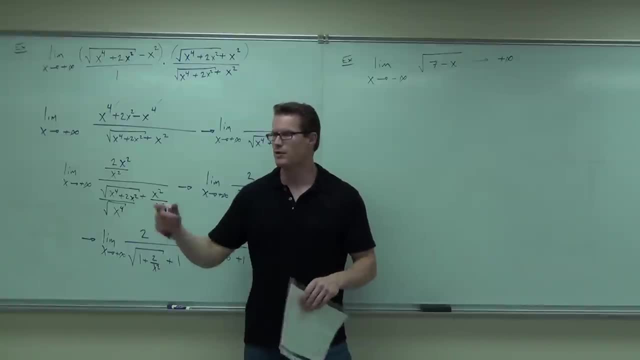 It's positive for negative infinity. right? We talked about that last time. We said: well, it follows really the leading coefficient or the leading term, Sorry, the power of the leading term. So x cubed is going to go up. 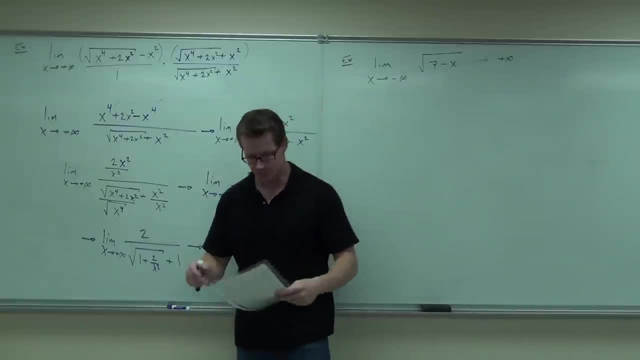 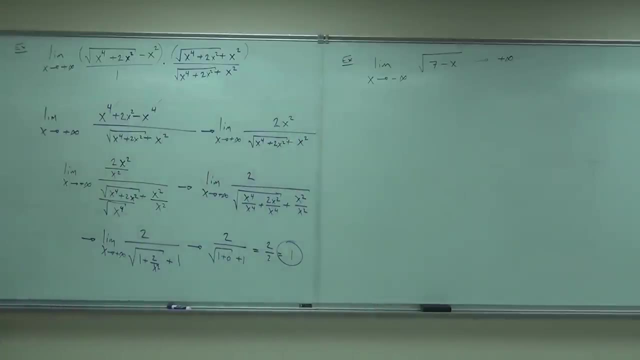 Or if it's negative, x cubed, it's going to go down And things like that happen. So be prepared for those limits. Are there any questions before we continue? All right, 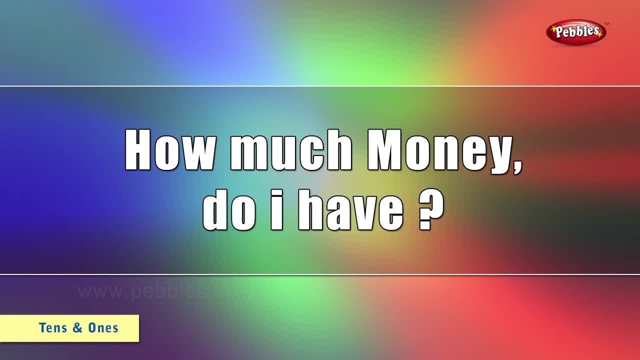 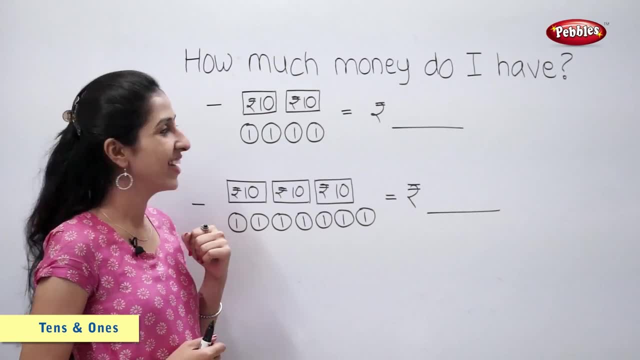 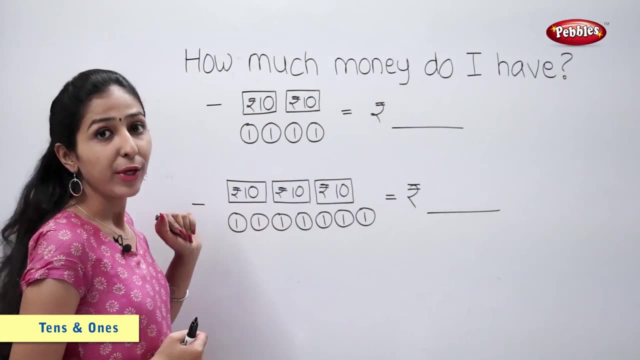 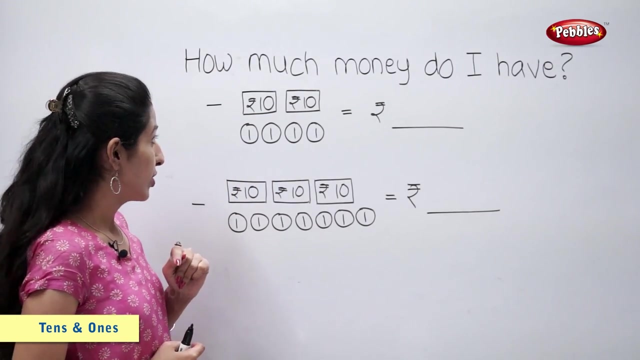 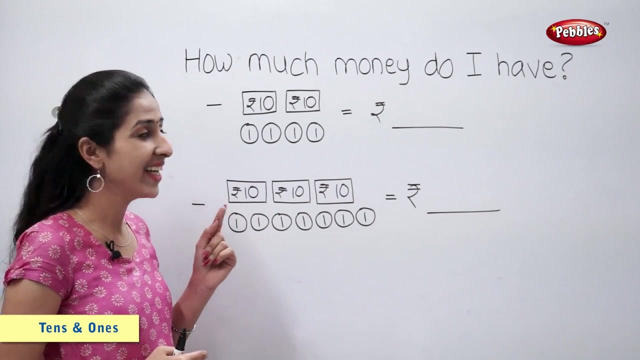 How much money do I have, Students? now let us find out how much money do I have. First example: we have 2 10 rupee notes and 4 1 rupee coins. So 10 plus 10 is equal to 20, and 20 plus 4 is equal to how much? 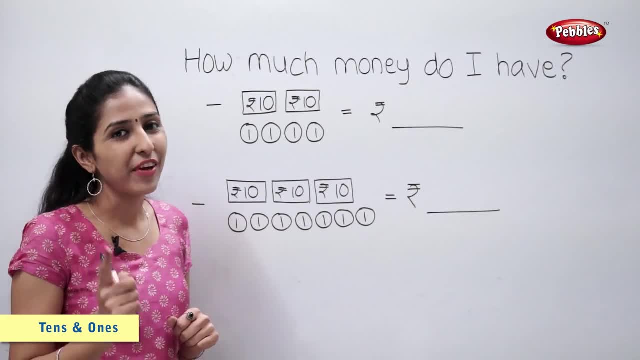 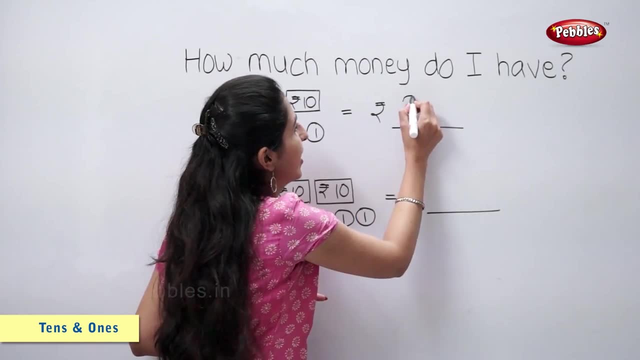 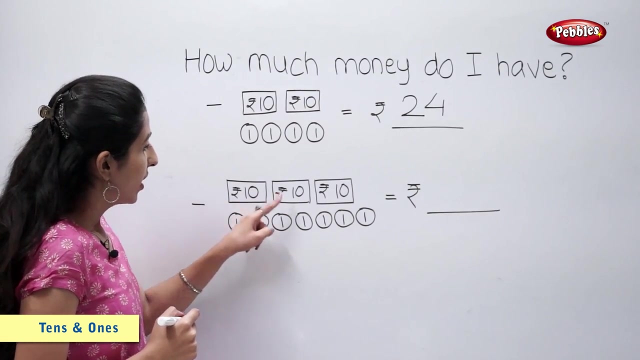 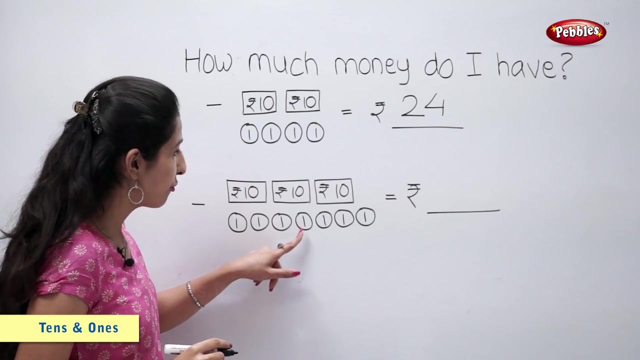 You count and tell me: Very good, that is 24.. So total I have rupees 24.. Next, 3, 10 rupee notes and 1, 2,, 3,, 4,, 5,, 6, 7..